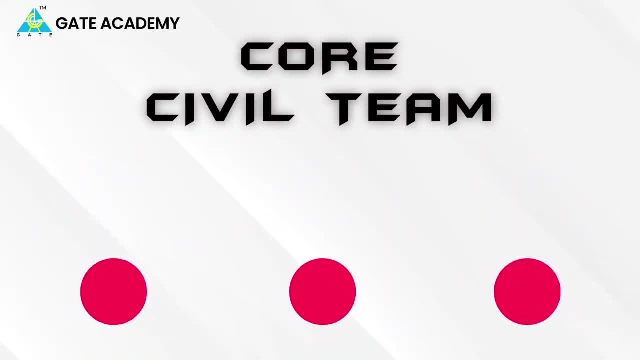 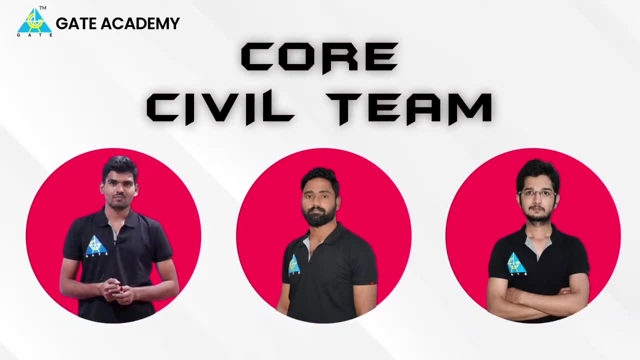 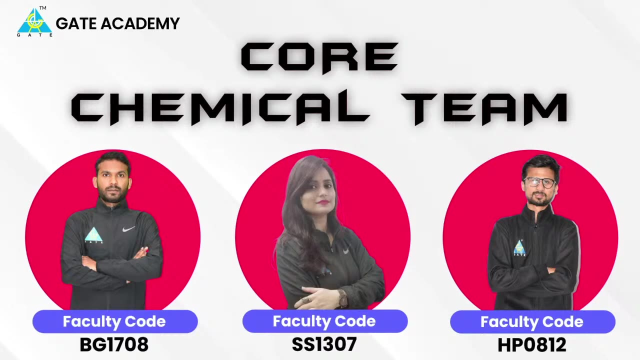 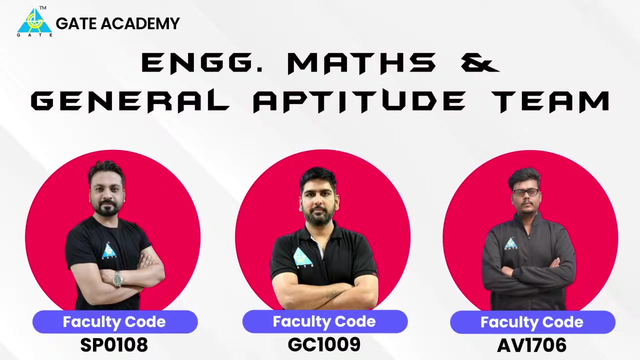 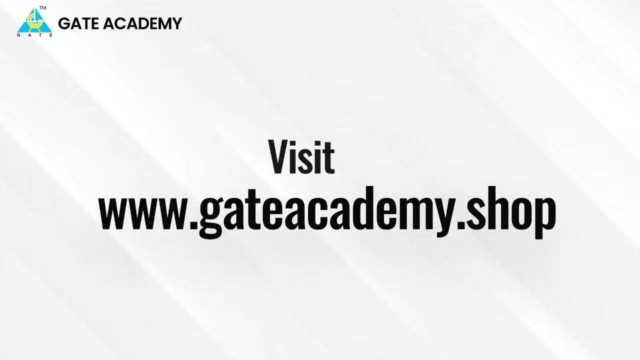 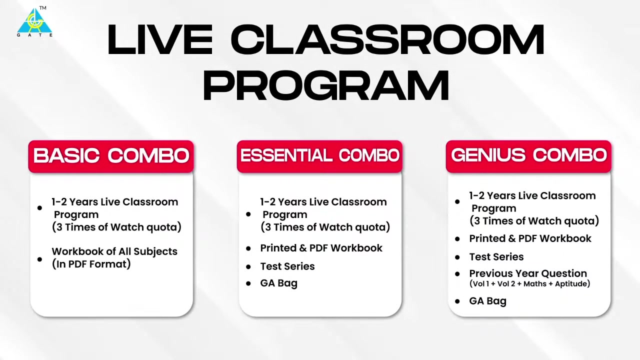 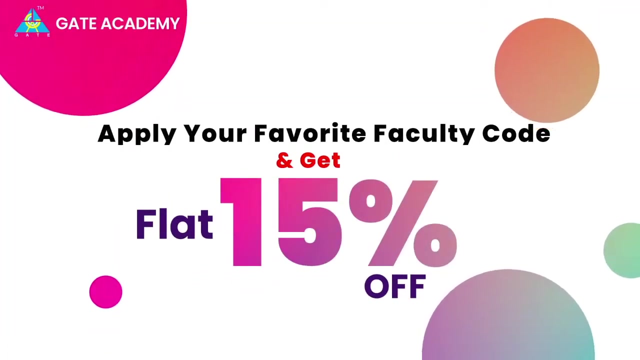 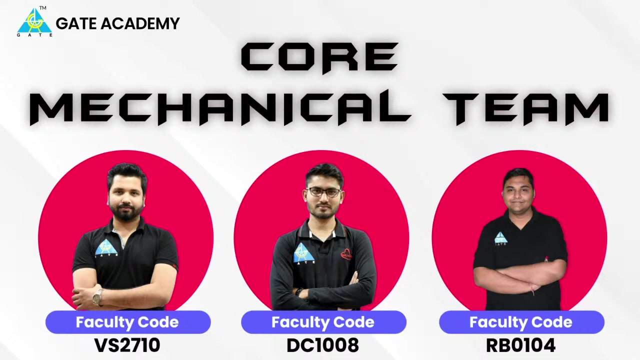 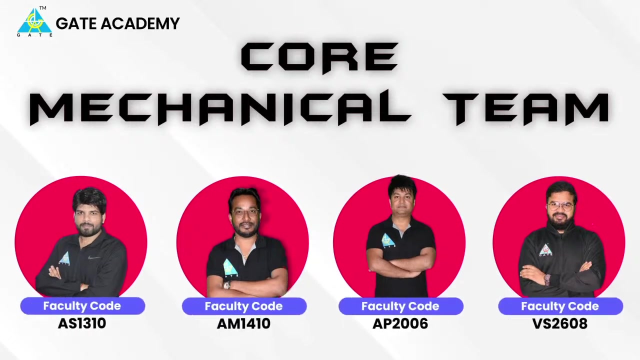 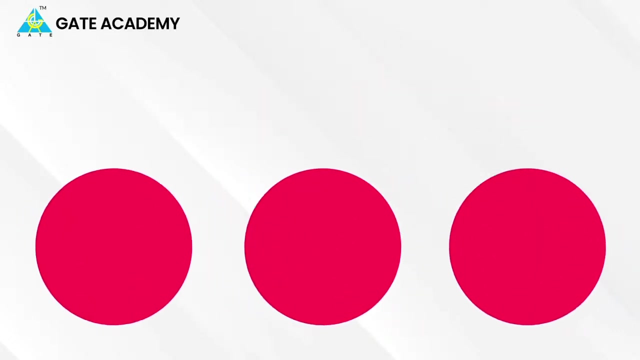 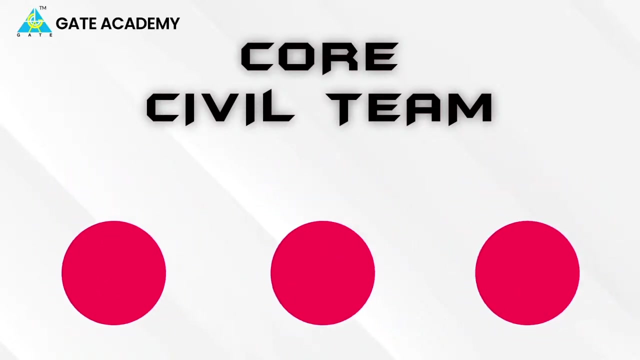 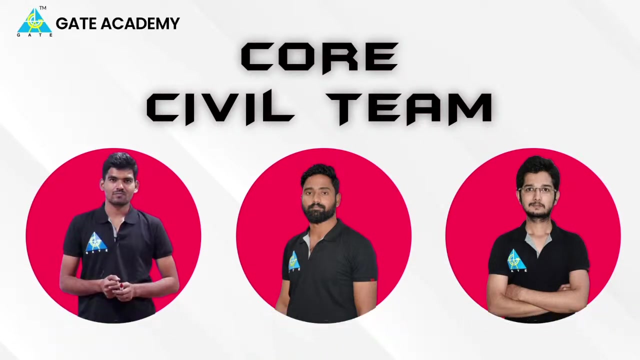 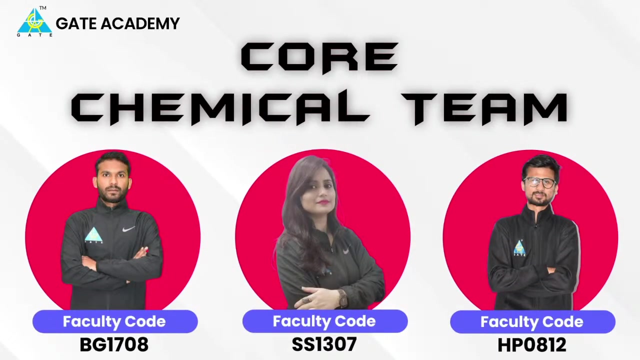 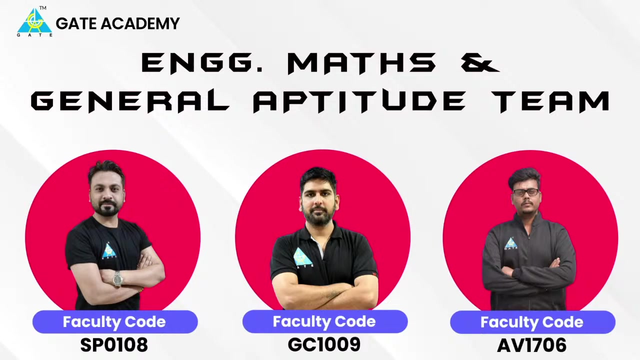 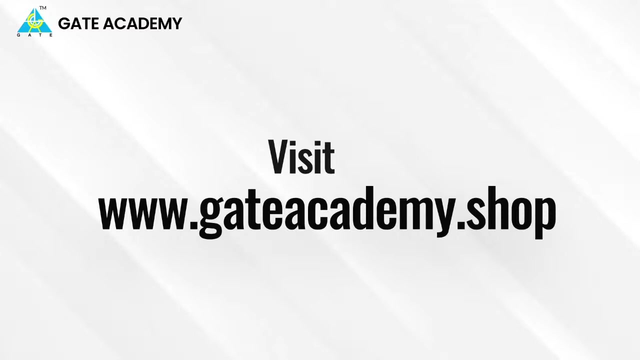 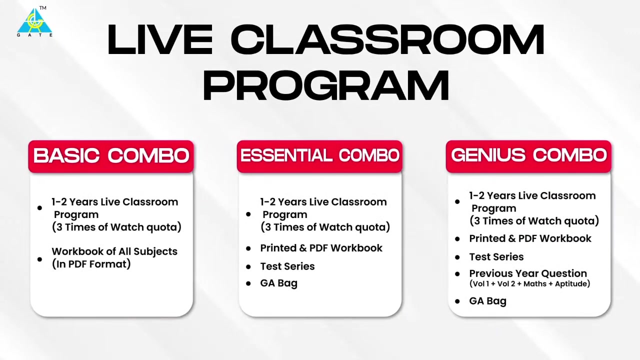 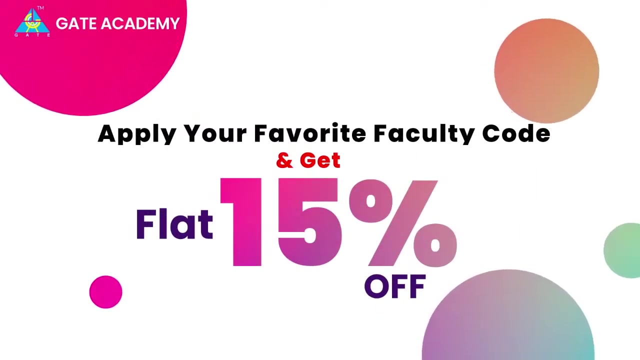 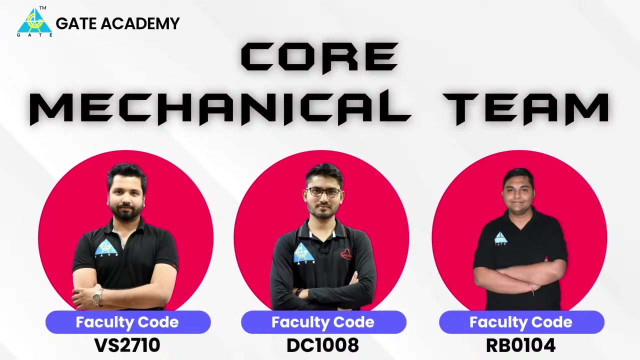 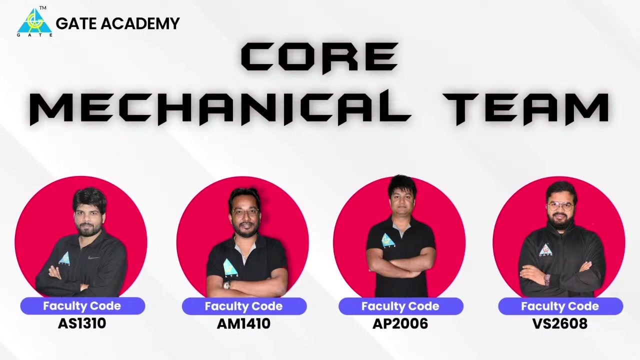 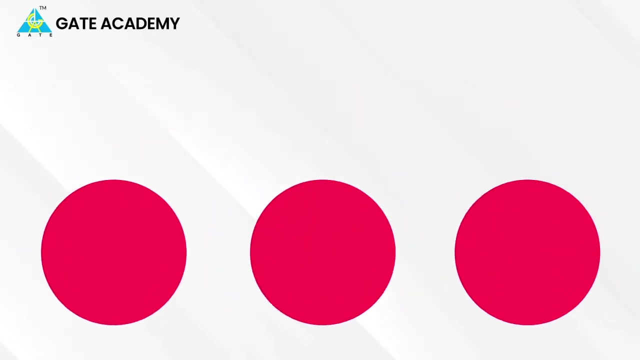 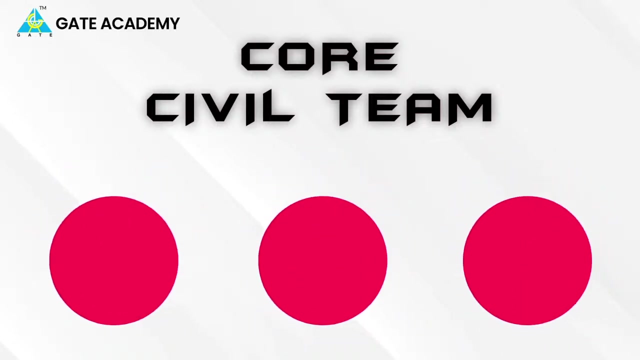 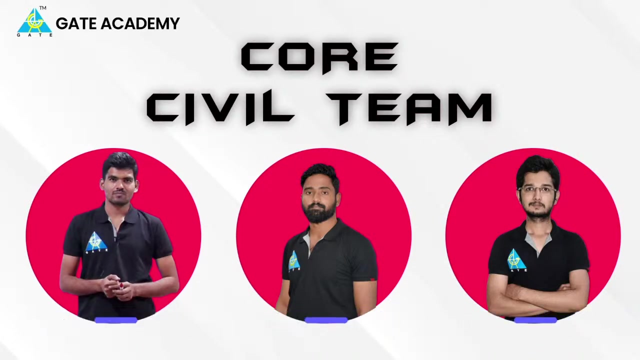 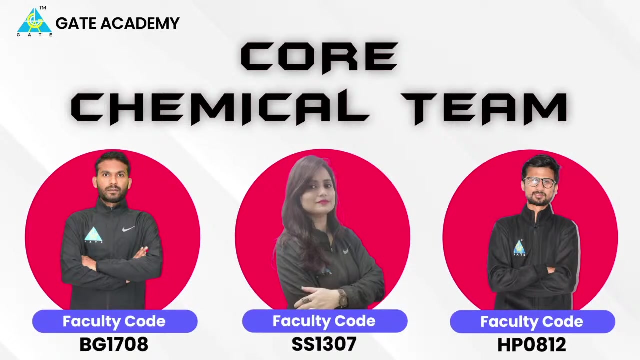 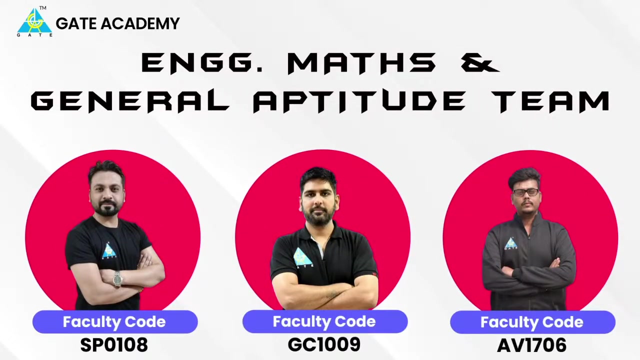 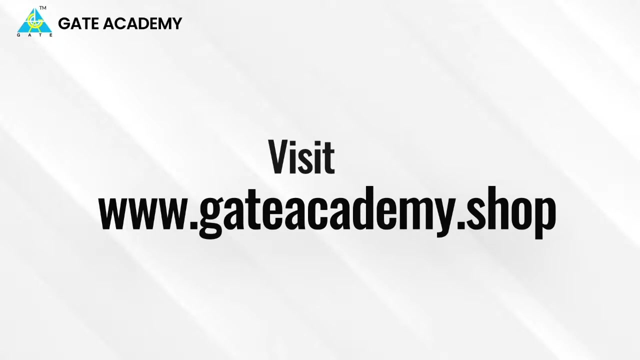 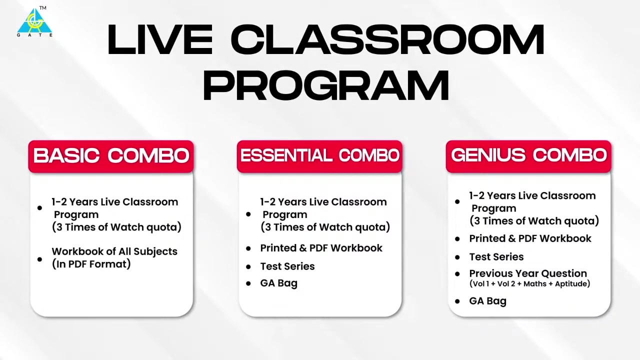 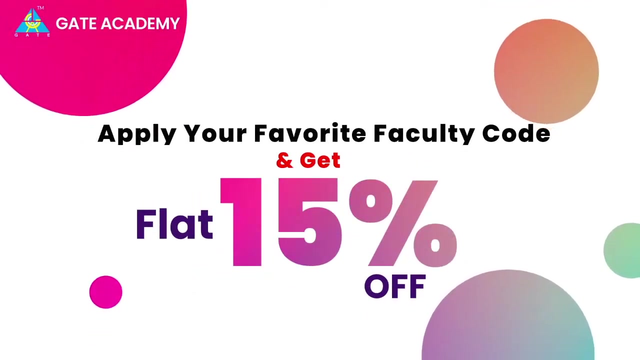 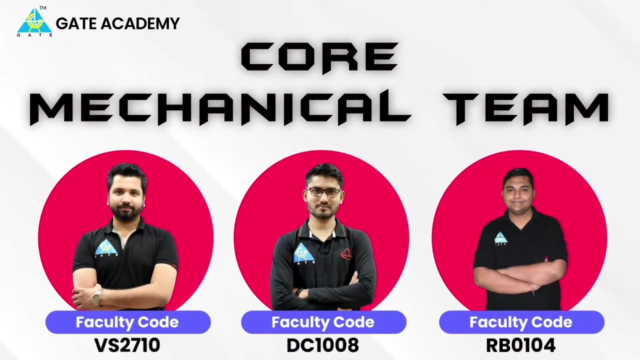 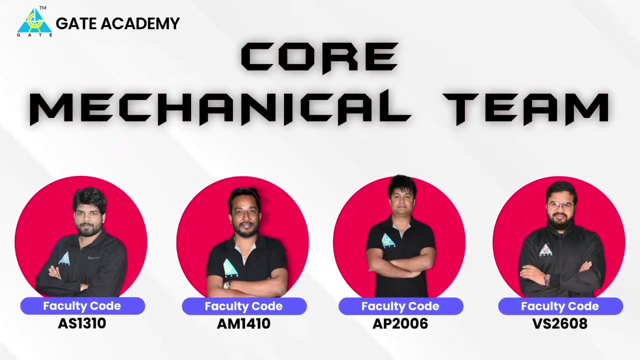 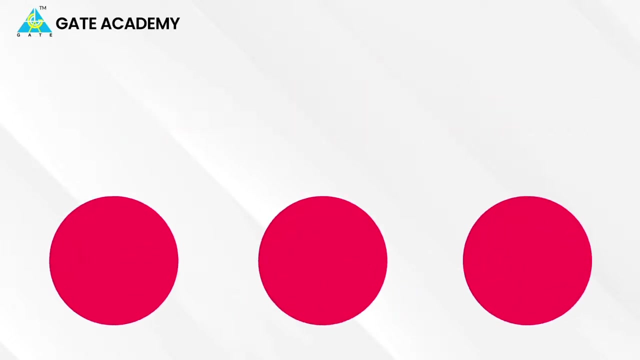 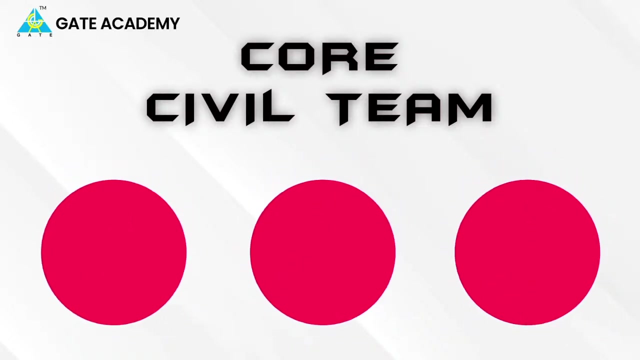 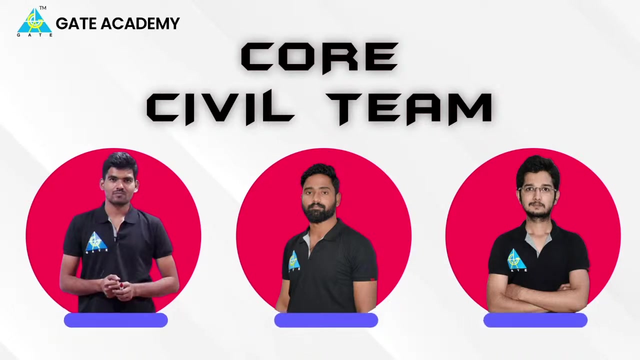 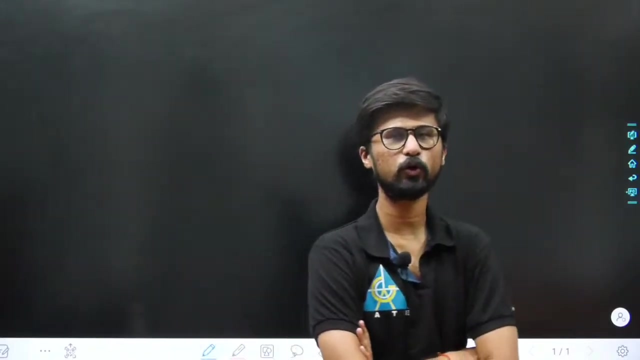 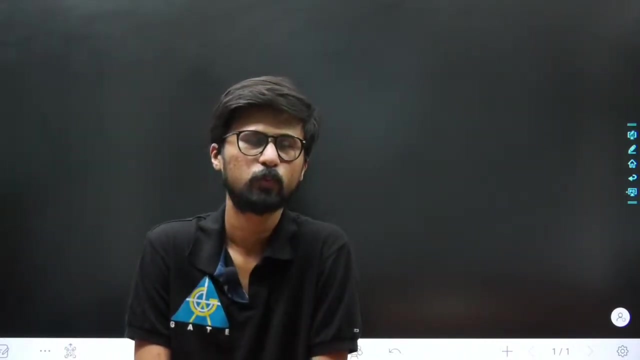 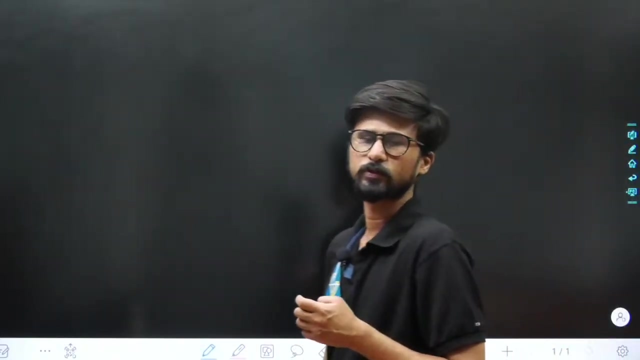 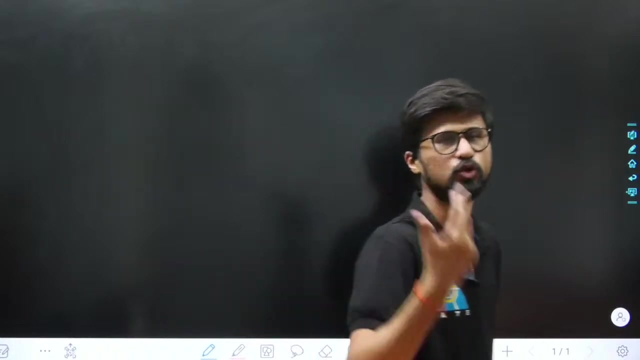 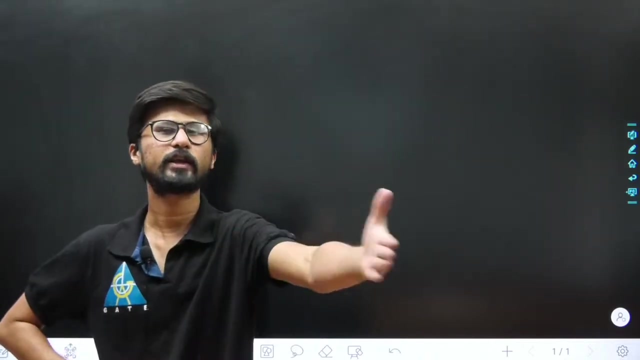 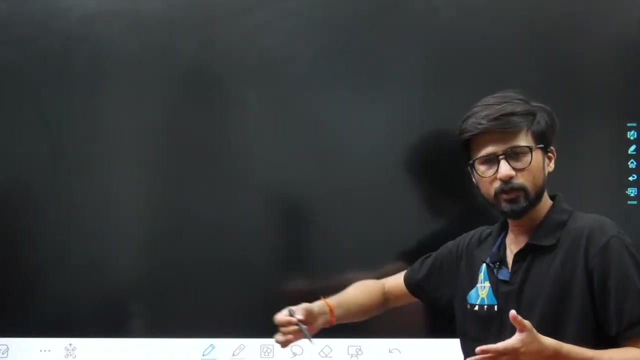 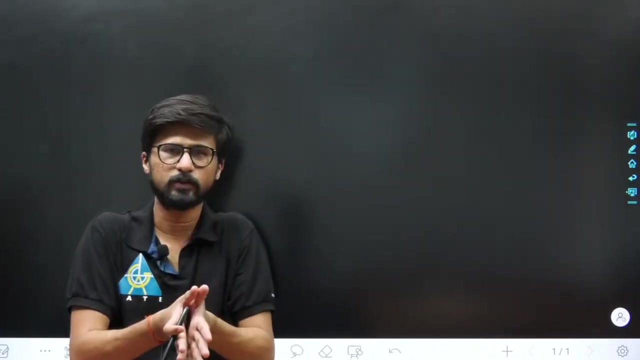 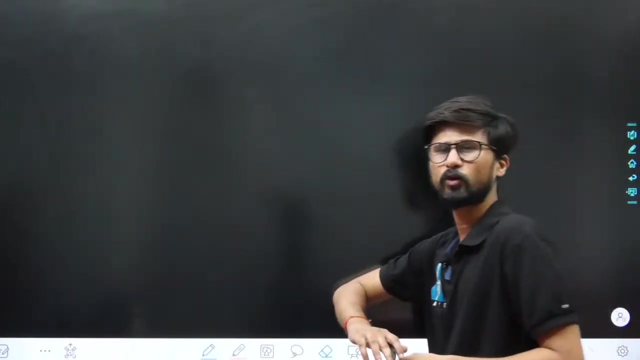 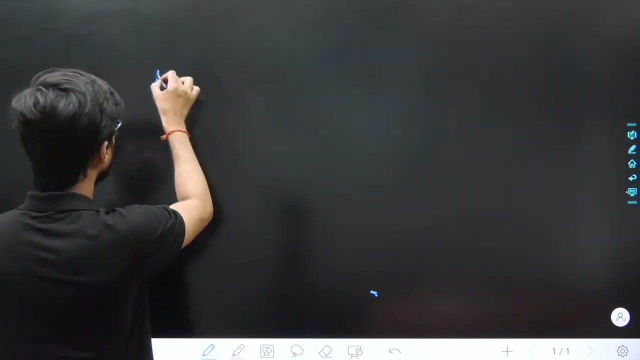 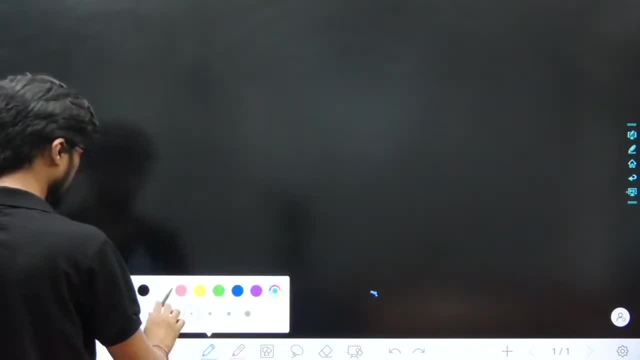 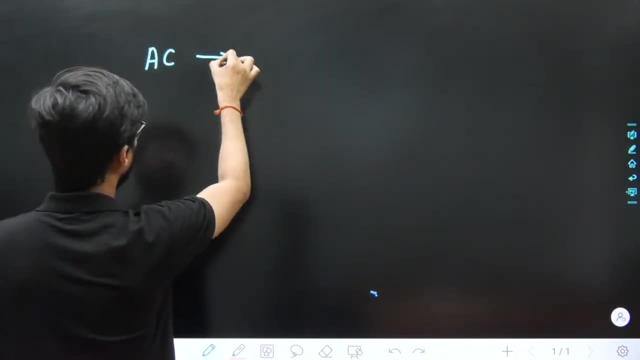 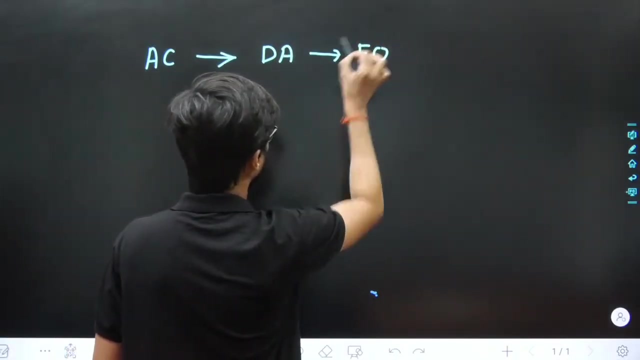 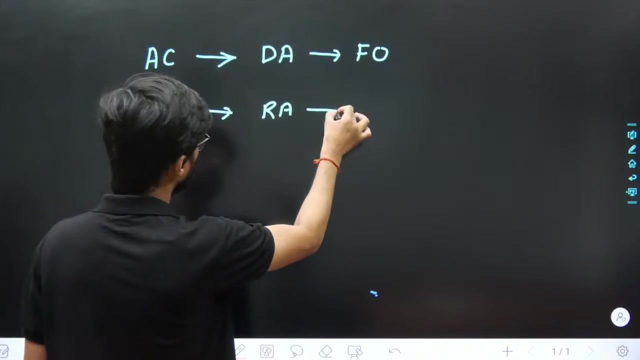 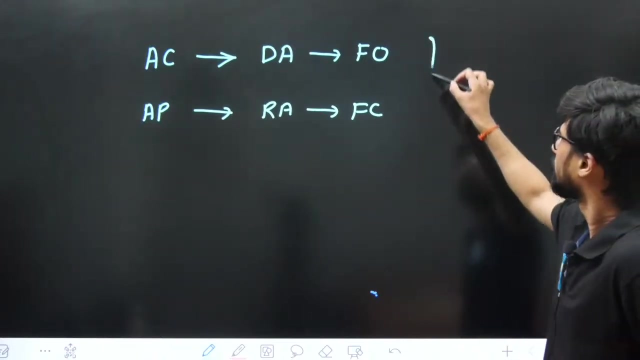 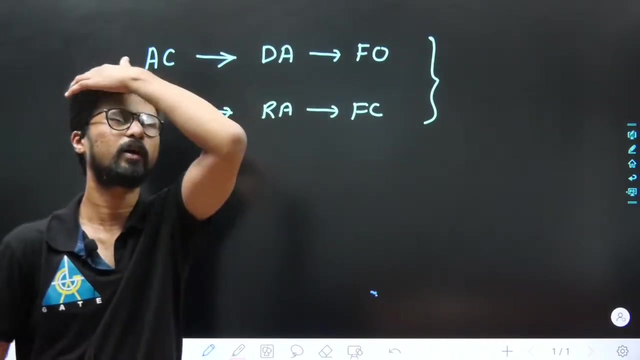 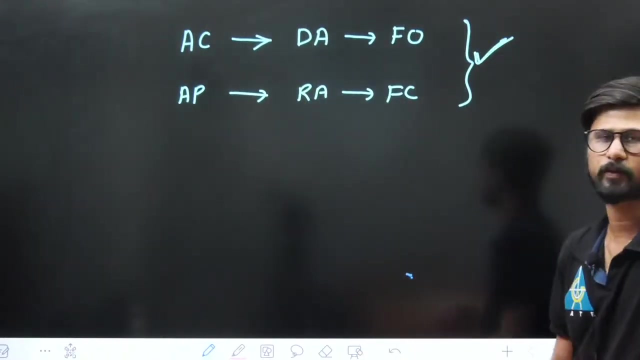 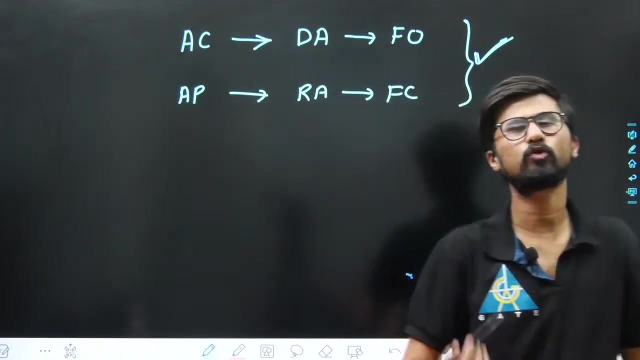 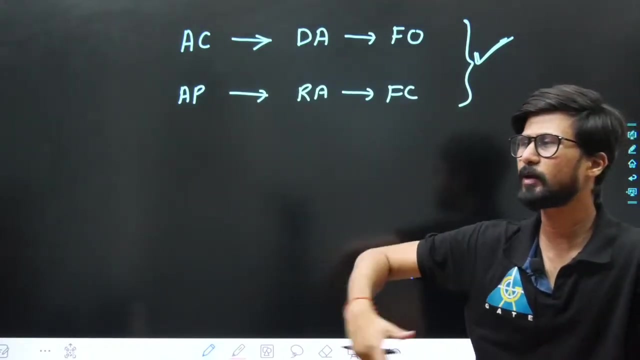 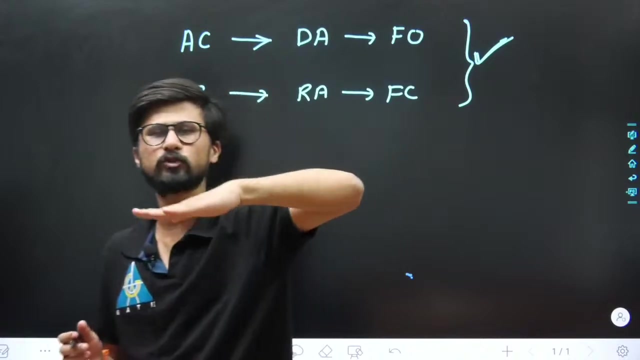 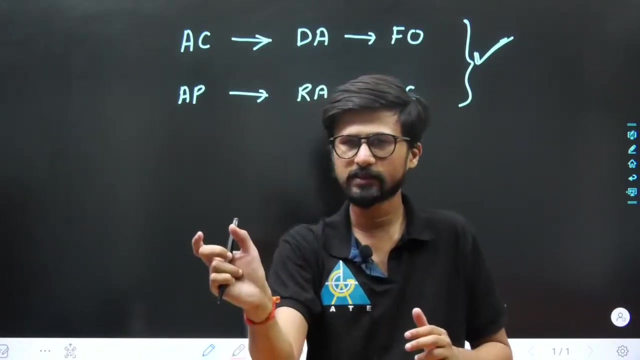 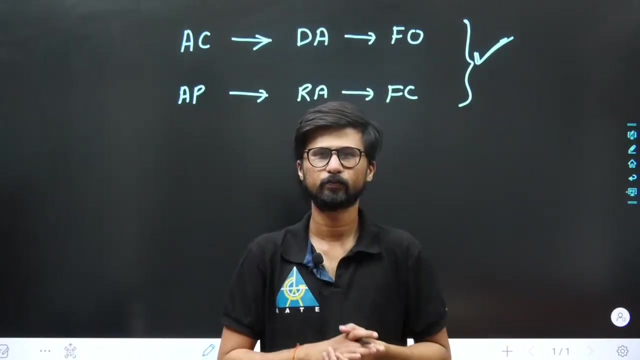 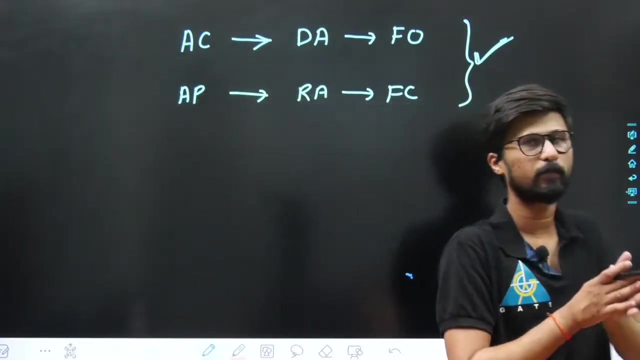 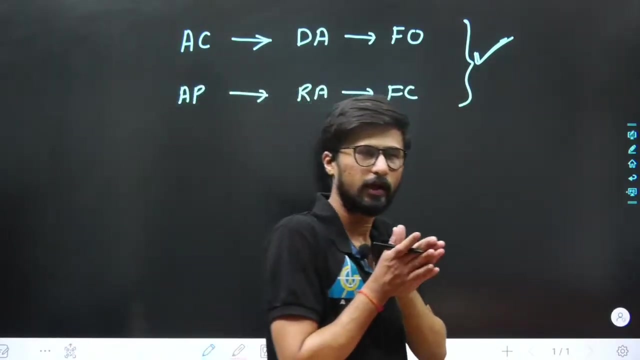 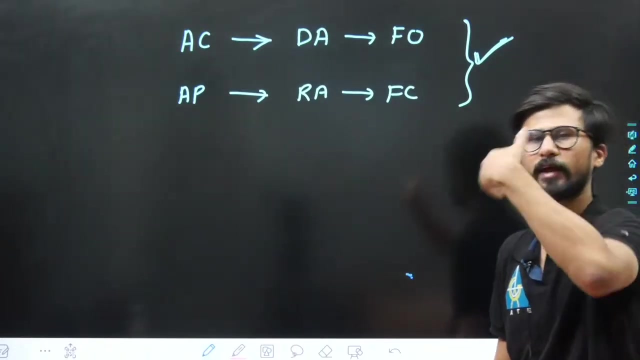 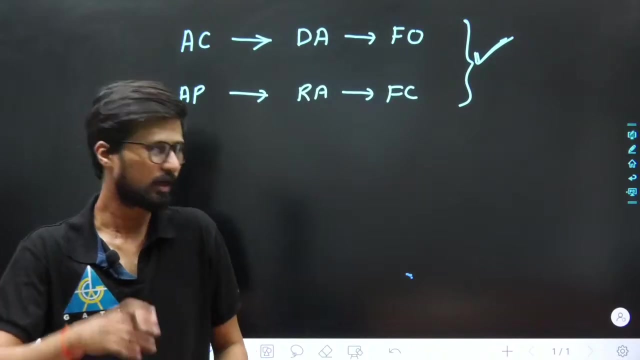 Bye-bye, Bye-bye, Bye-bye. Next thing we saw was inverse response. What is inverse response? Inverse response means two mechanisms are competing in the same process. I gave you the boiler example. How will you recognize the inverse response? by looking at the transfer function, By looking at the 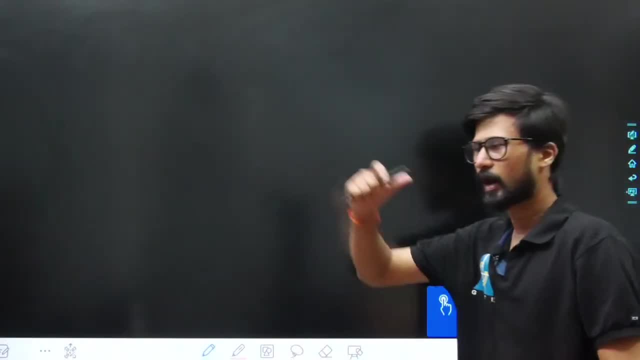 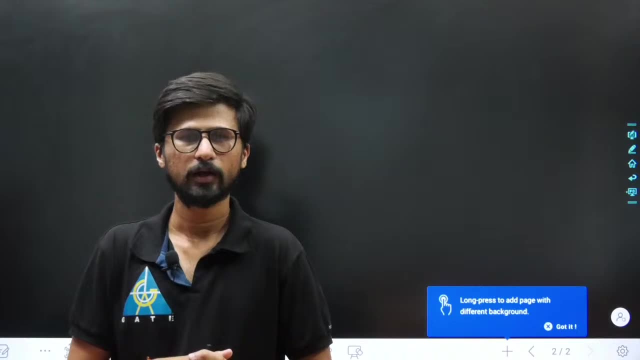 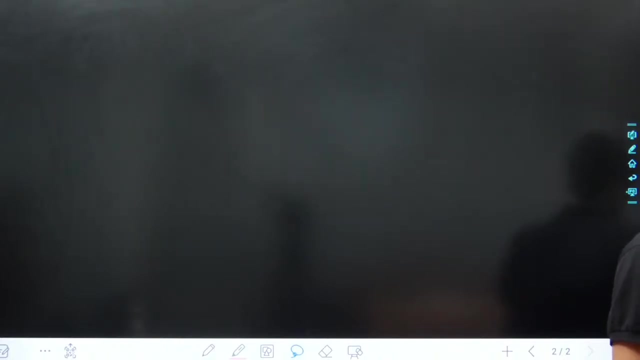 transfer function. you will recognize that if the right half plane 0 is present in the opposite direction, it will show the inverse response. So the condition of the inverse response is right, half plane 0.. Any doubts? Direct acting is called air to close, but in 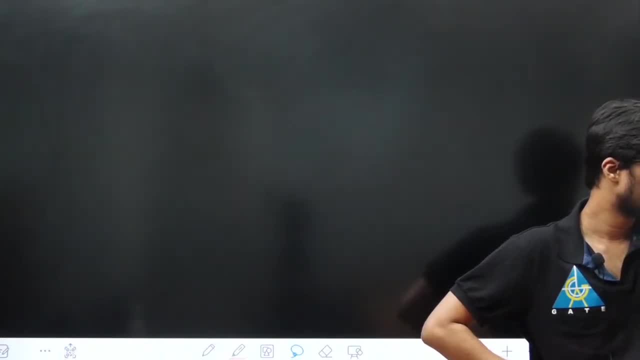 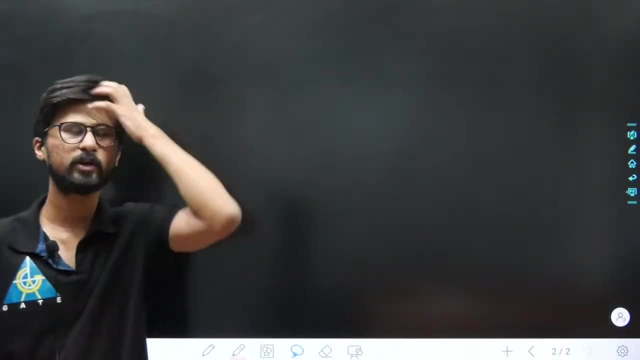 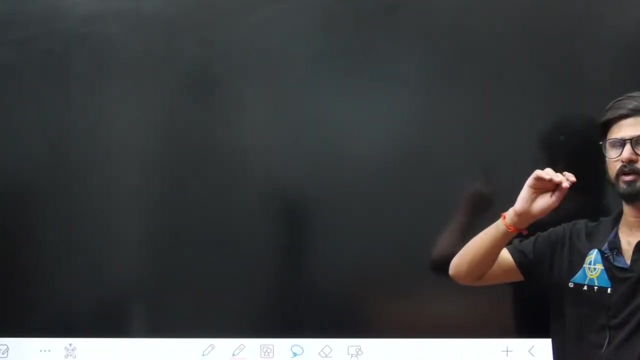 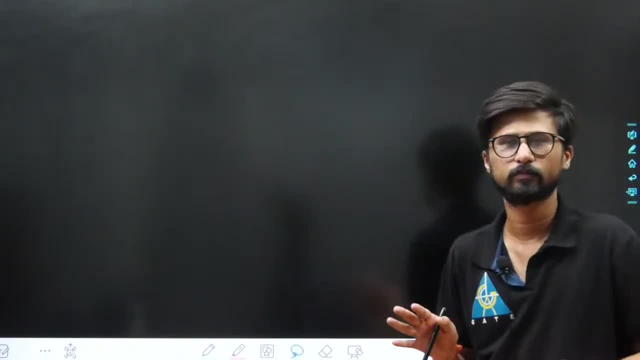 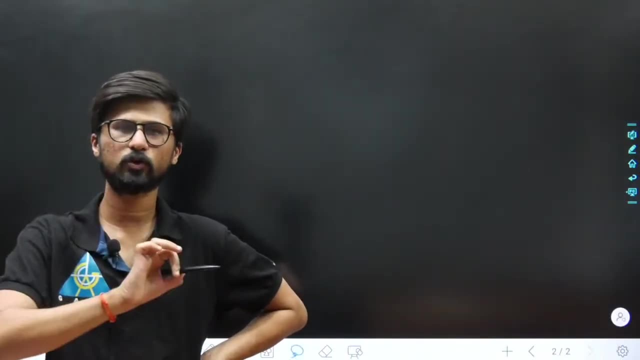 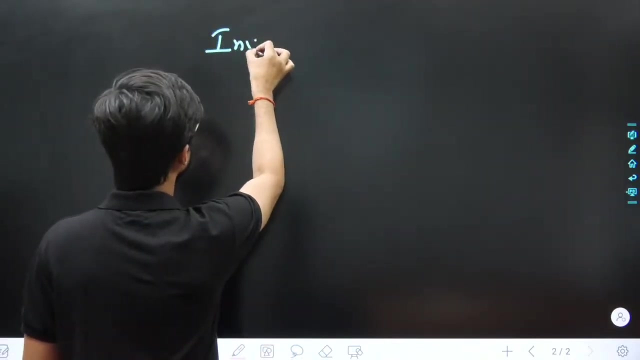 Air to close is direct acting. That is it Now? inverse response. We were talking about inverse response: Right half plane 0.. Right half plane 0.. Inverse response. Inverse response: Right half plane 0.. Inverse response. 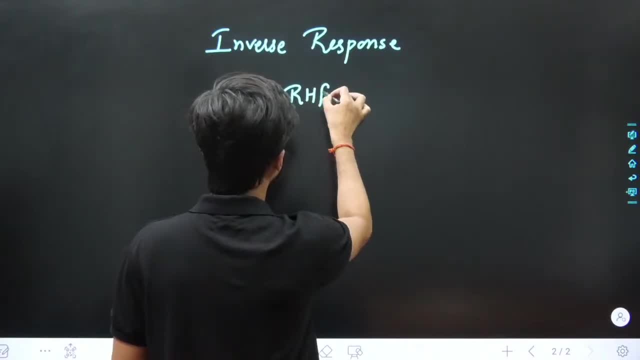 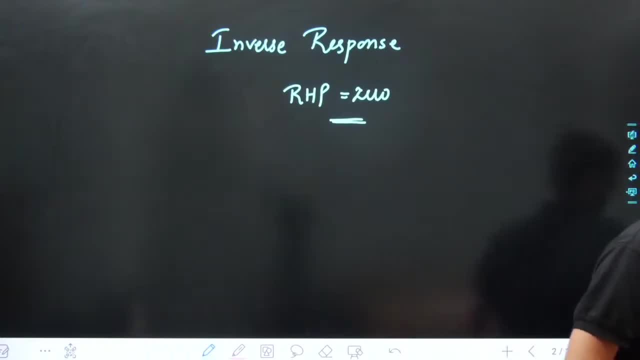 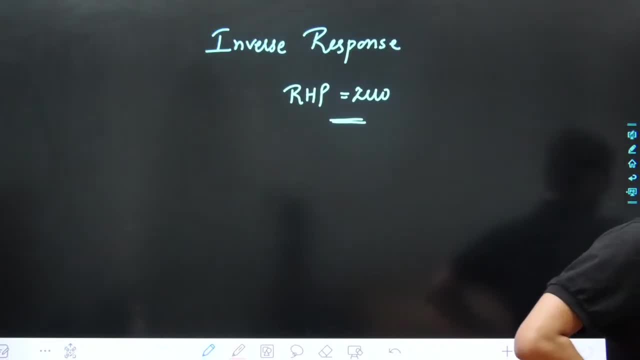 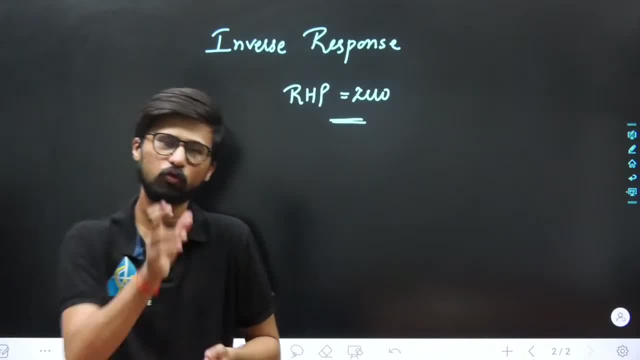 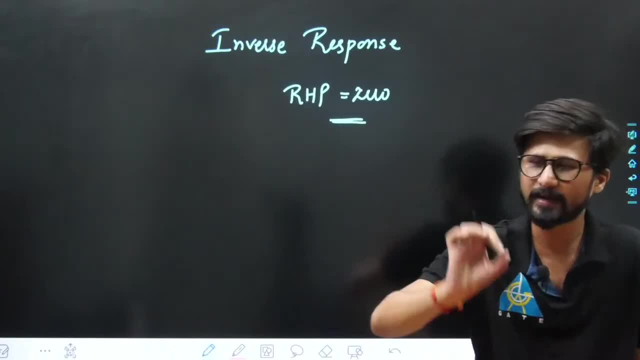 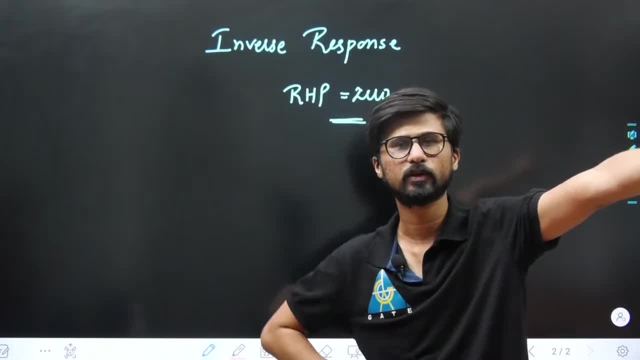 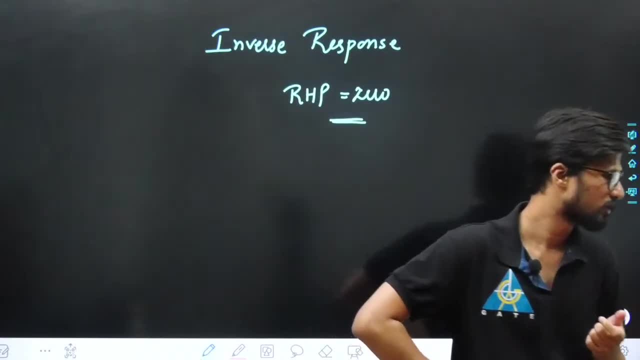 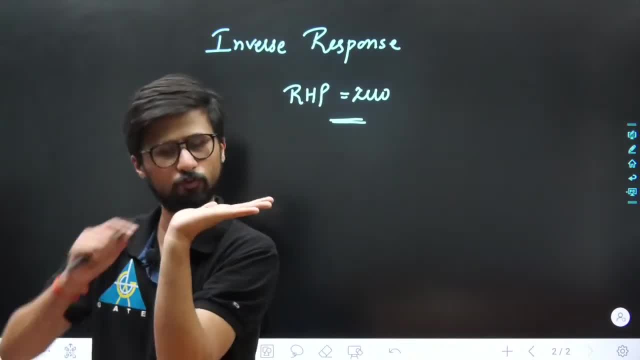 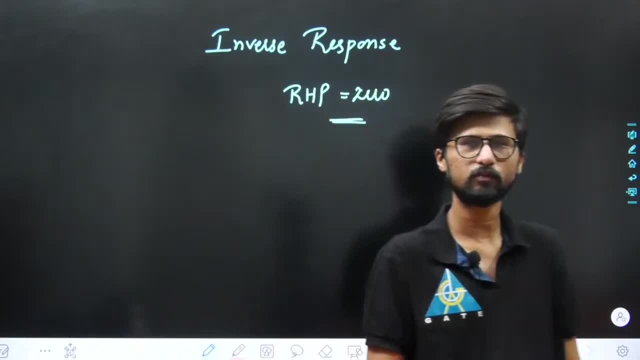 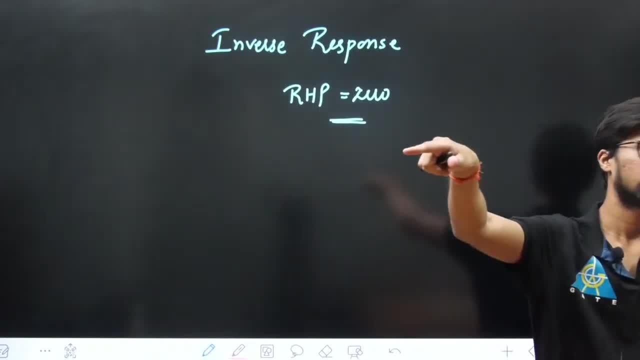 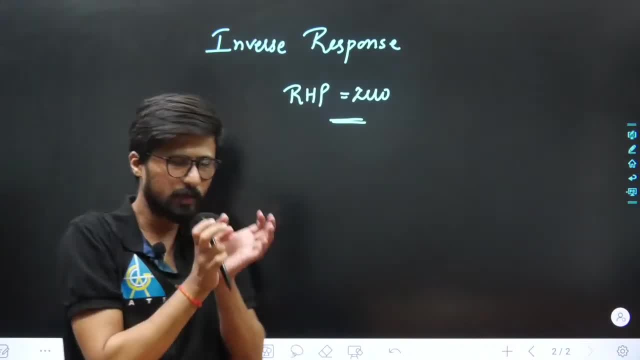 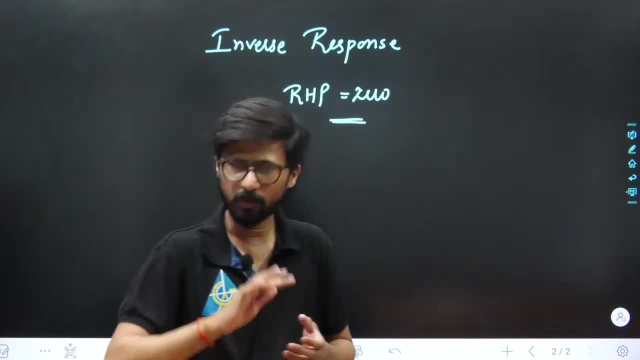 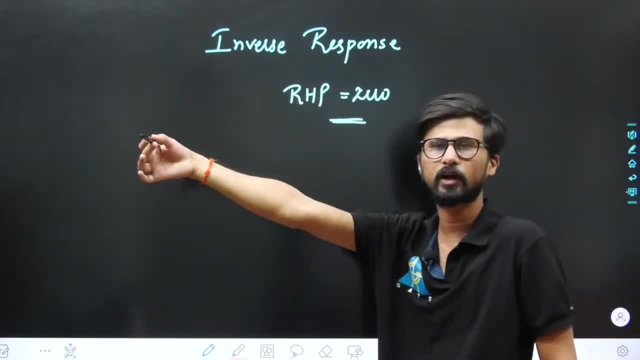 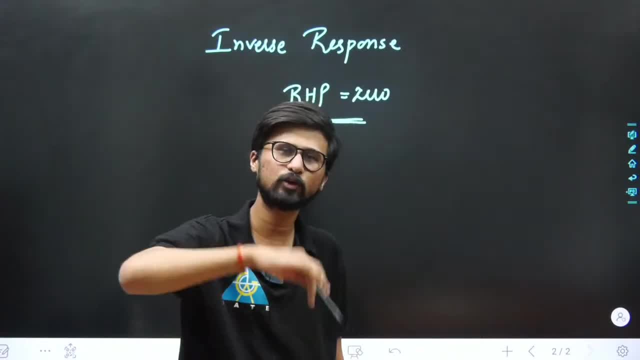 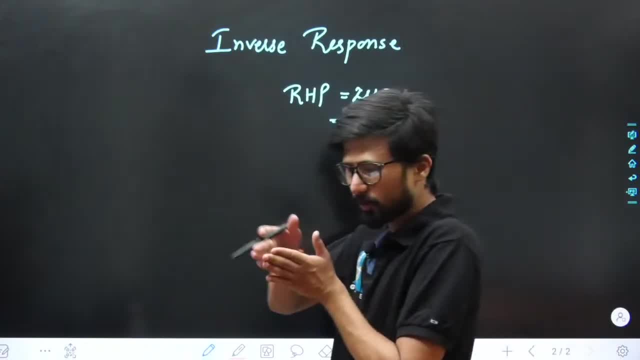 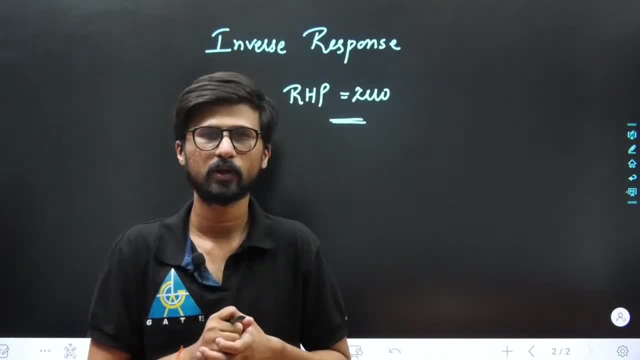 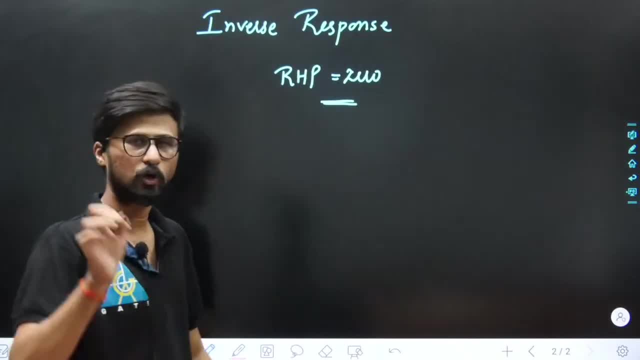 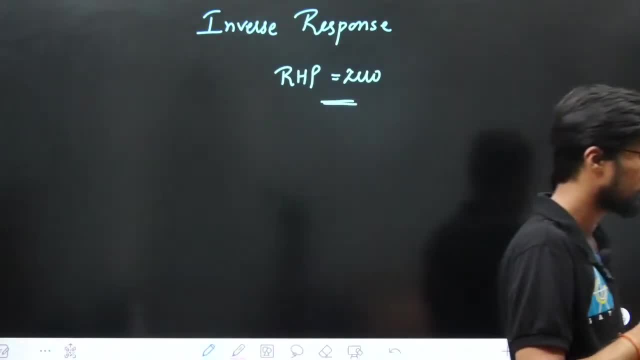 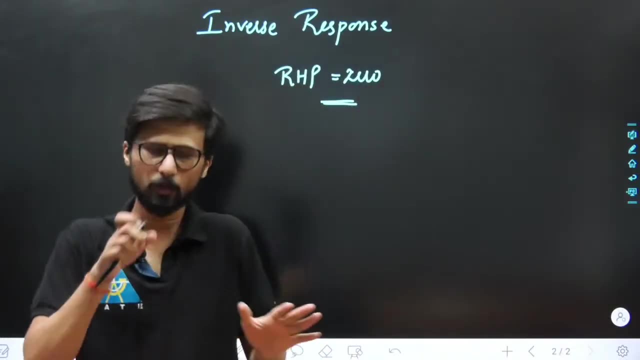 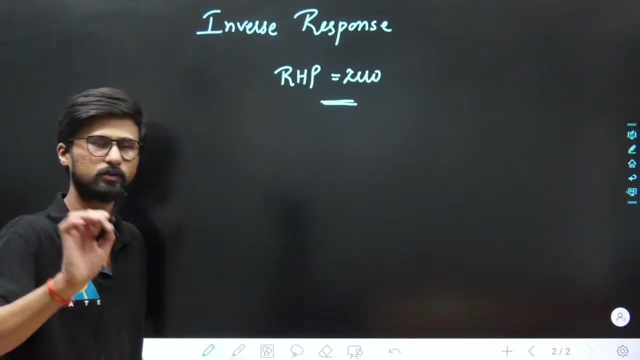 Both have different meanings. It is not necessary that air to close, So controller will also be direct acting. There is no such relation. You will have to judge that by looking at the process. Good afternoon. So let us see a problem on inverse response. 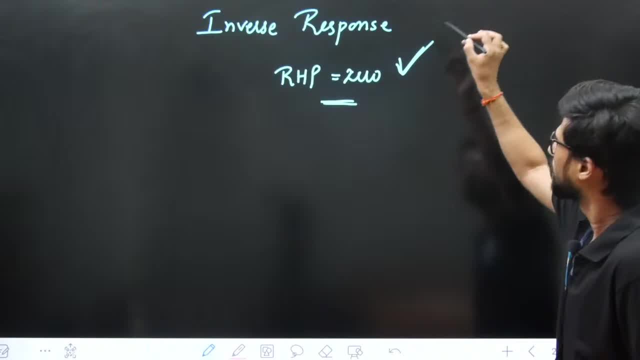 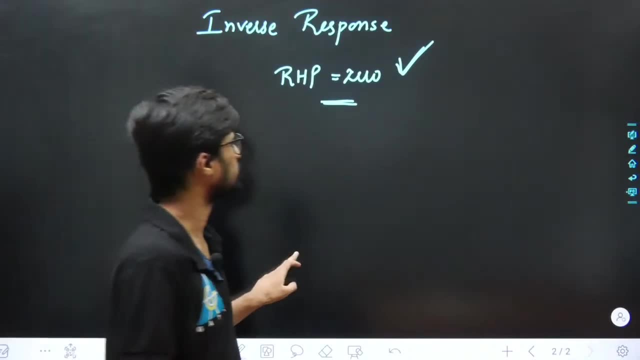 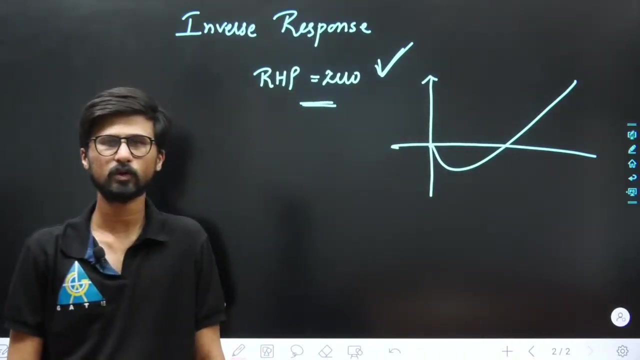 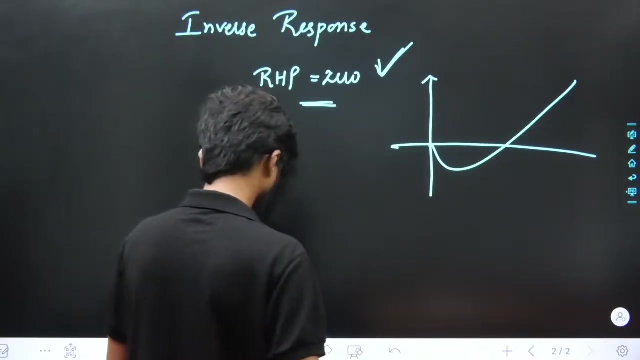 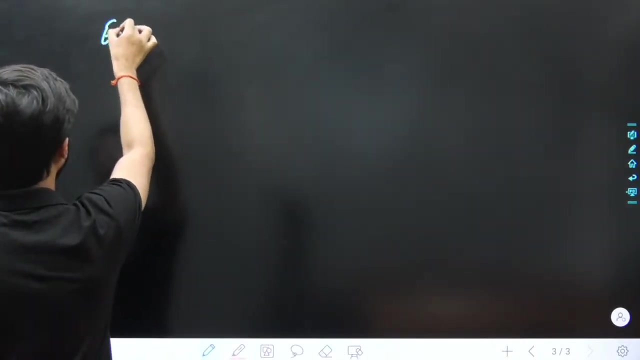 You just have to pay attention that right half plane is zero. It means inverse response And the main thing to remember in inverse response is graph. The graph is always like this: Let us see the question. Look at the question. We are taking an example of inverse response. 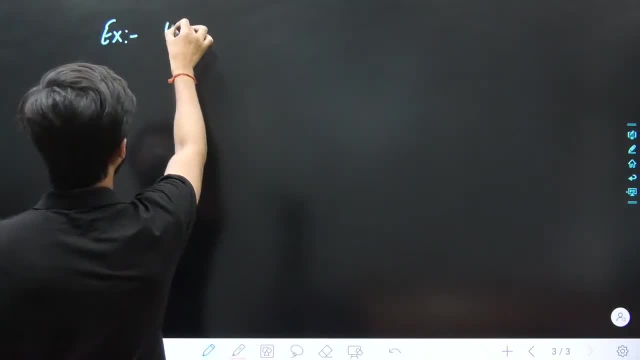 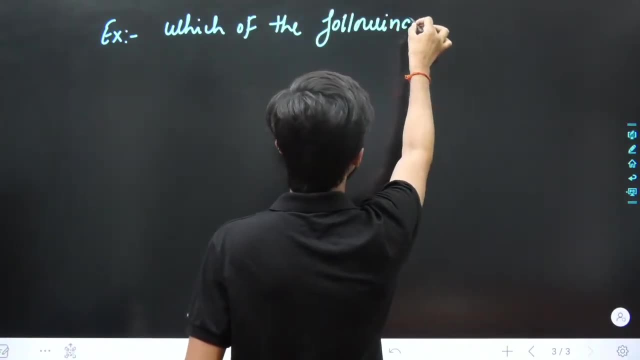 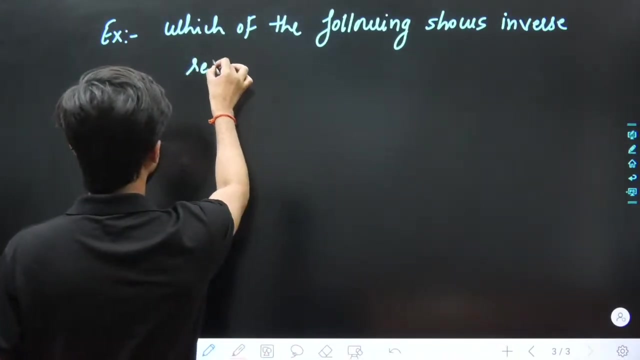 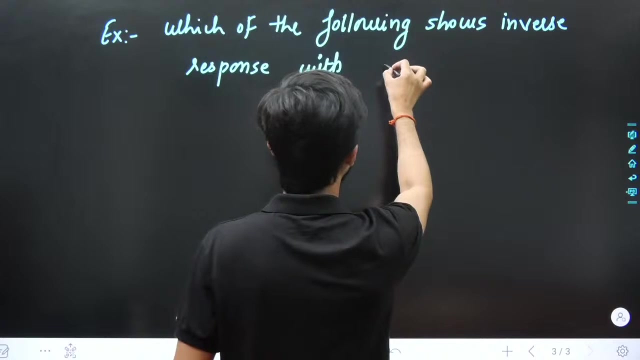 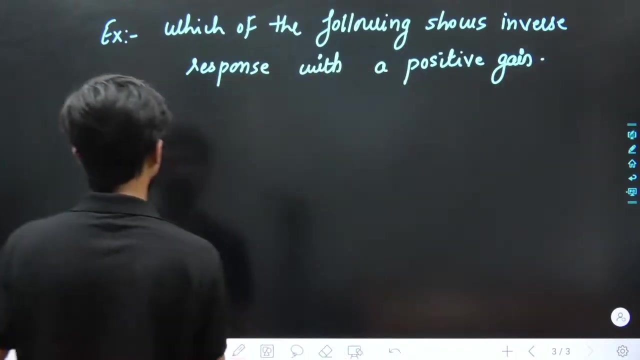 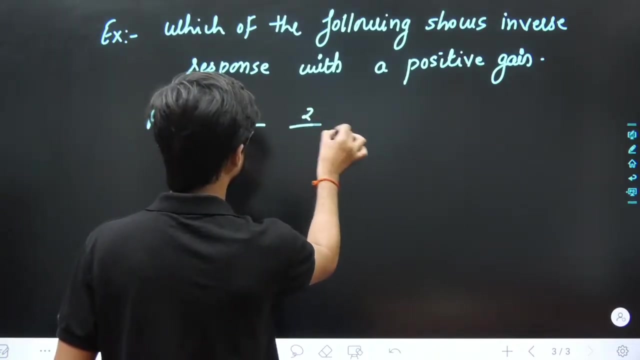 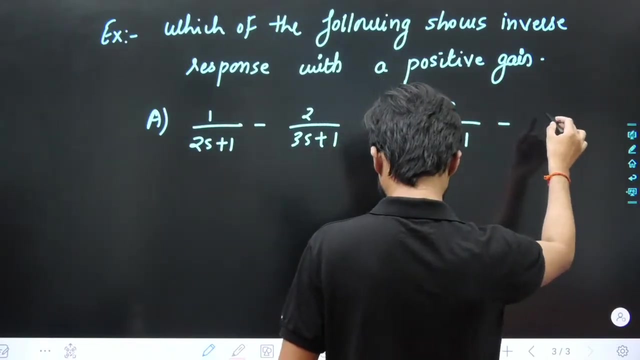 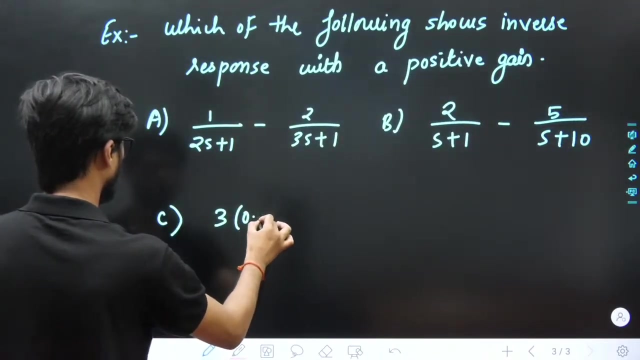 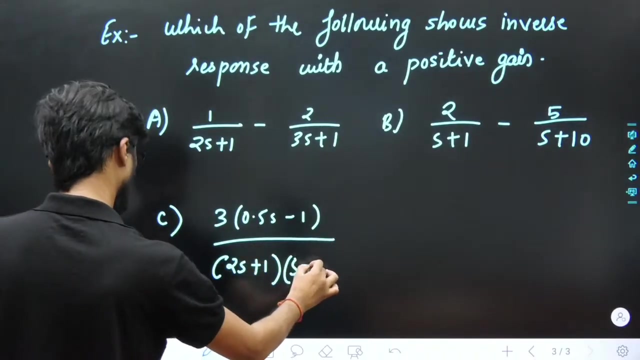 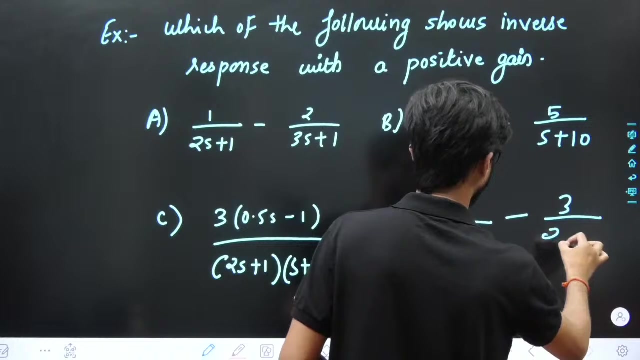 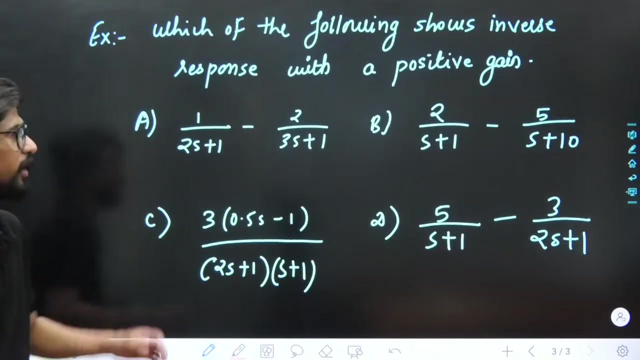 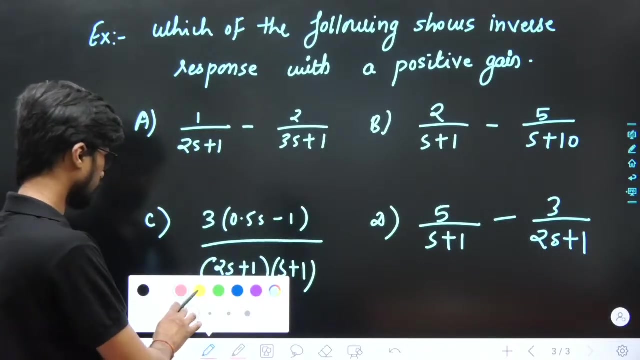 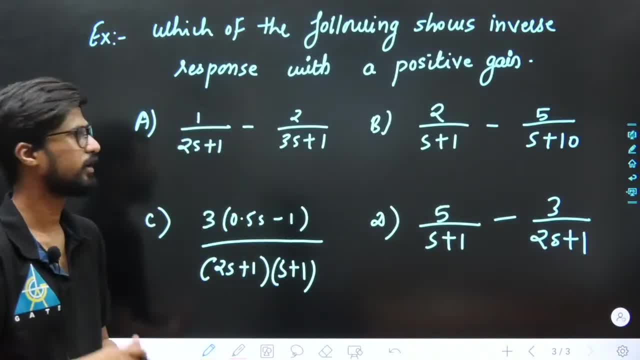 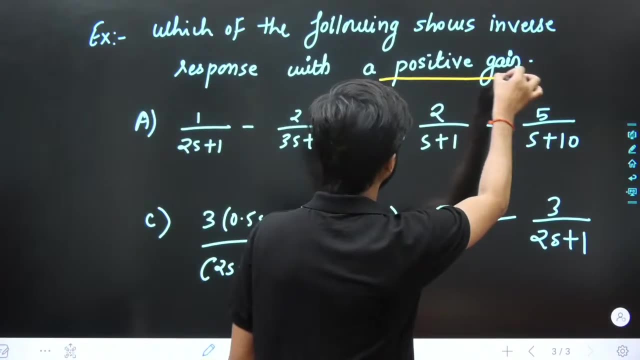 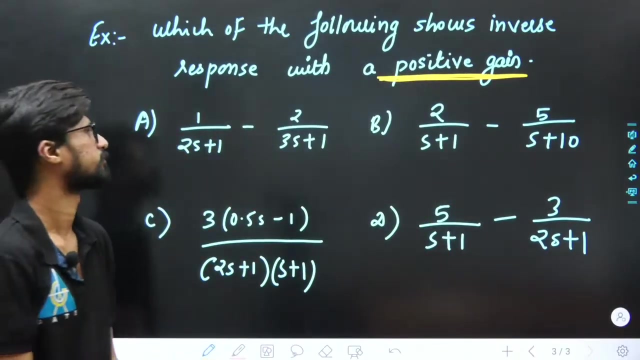 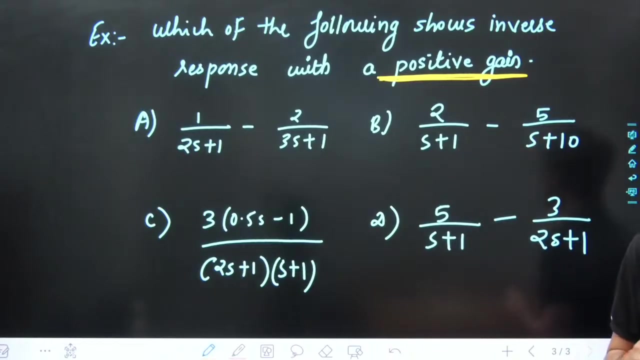 You have given a transfer function, You have asked which transfer function will show inverse response. And the second thing: Gain, positive. Gain should be positive. The importance of every thing. Gain should also be positive. So the first thing: What do we need for inverse response? 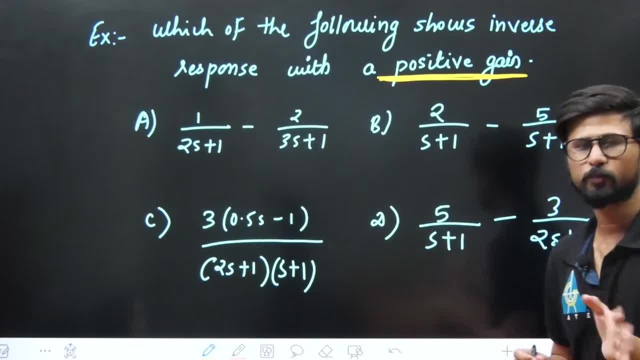 Right half plane 0.. In whichever transfer function Right half plane 0 comes, That will be the inverse response. Okay, First check this condition. Second Gain: Positive gain is said. Positive gain means How will you get the gain? 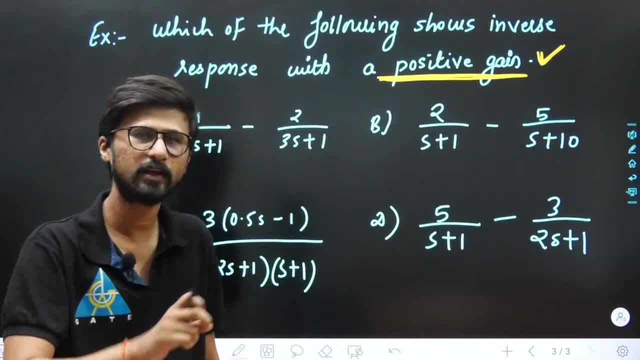 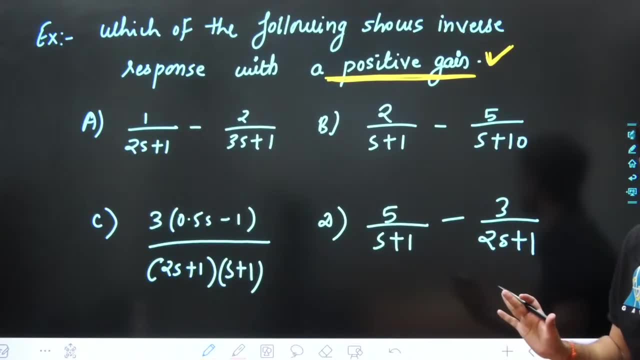 What is the method to get the gain? The method to get the gain is: S is equal to 0. Okay, S is equal to 0. You will substitute at every place: Okay, And Gain Positive or negative. You will get the value of the gain. 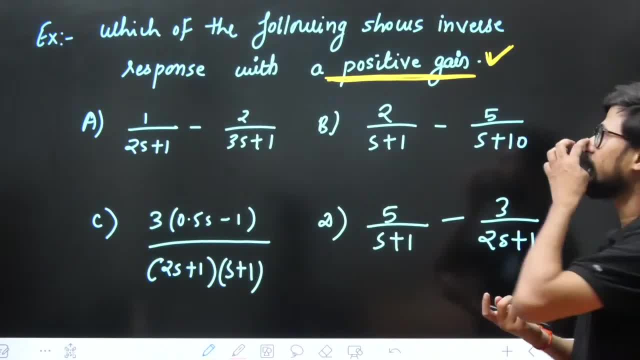 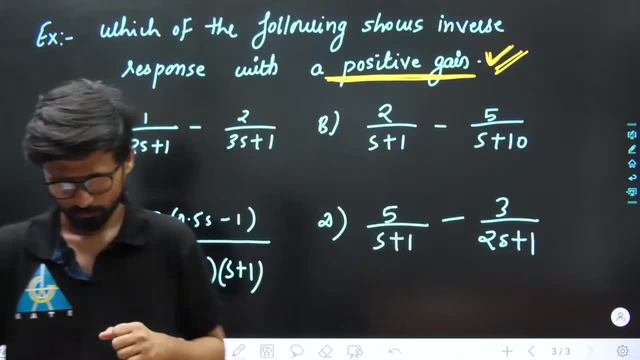 You will get the value of the gain. Okay, So first let's do the gain part. First let's do the gain part. Okay, See, D Rishabh is saying D. Okay, Come on, Let's see. 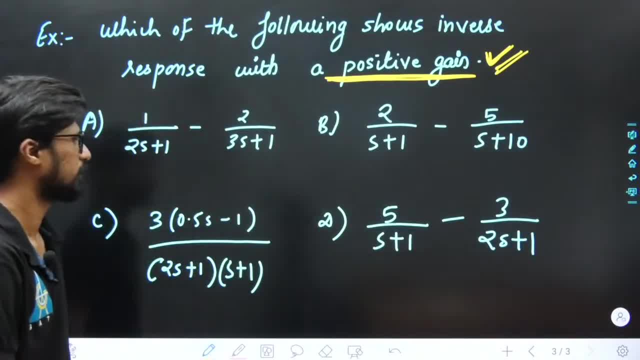 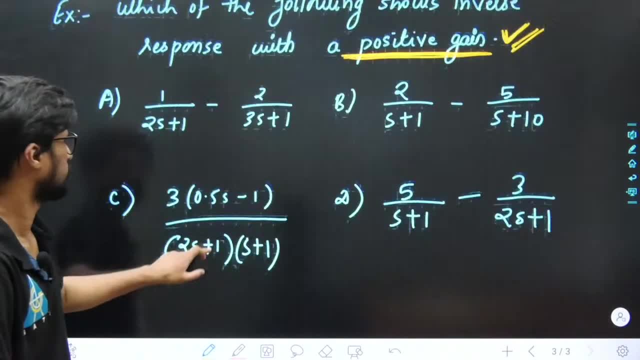 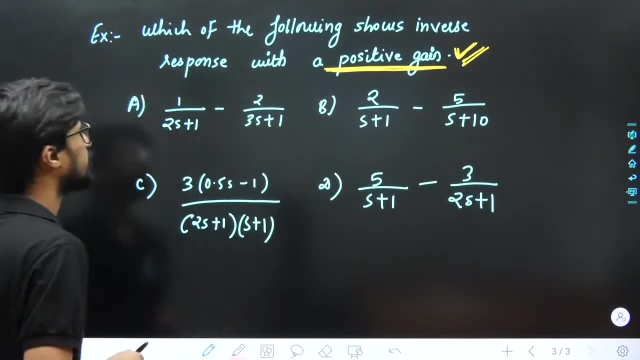 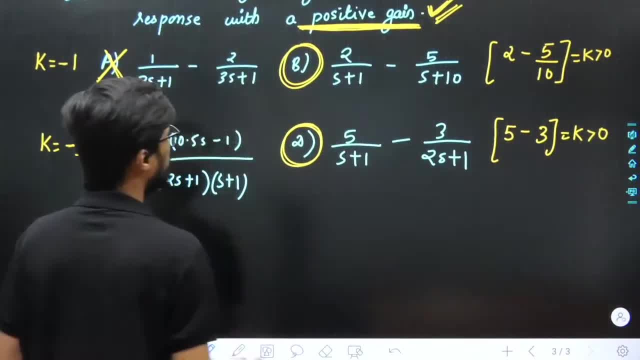 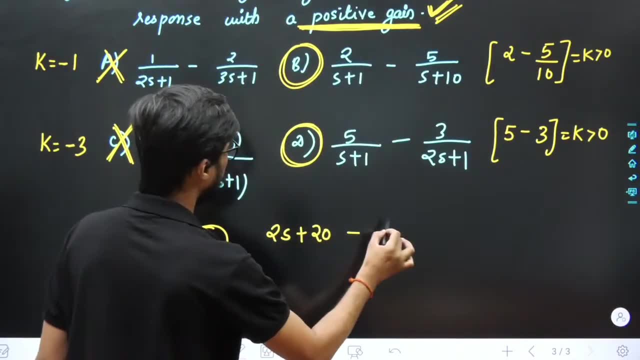 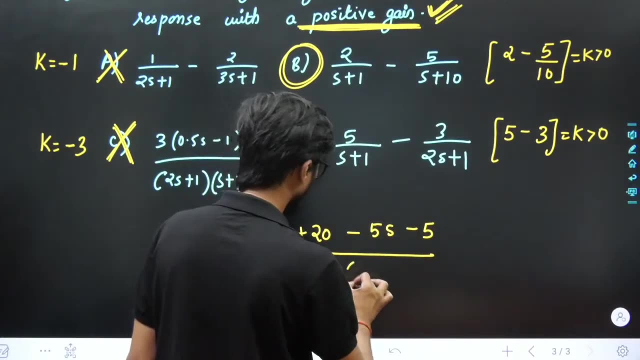 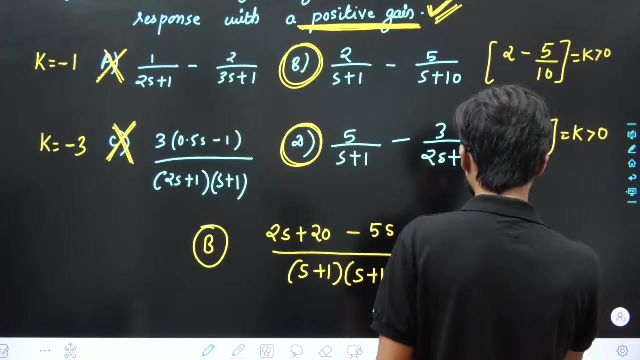 Negative, Negative, Negative, Negative, Negative, Negative, Negative. So 2s plus 20 minus 5s minus 5, divided by s plus 1 into s plus 10, this will be equal to 2s minus 5s minus 3s plus minus 5, sorry, minus 3s plus 15, divided by s plus 1 into s. 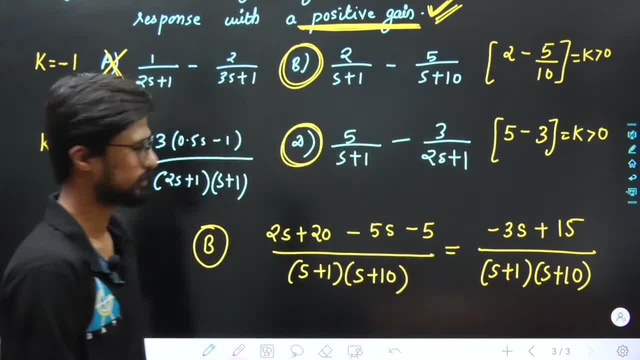 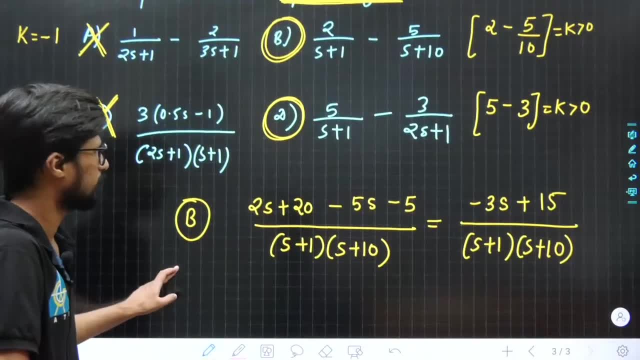 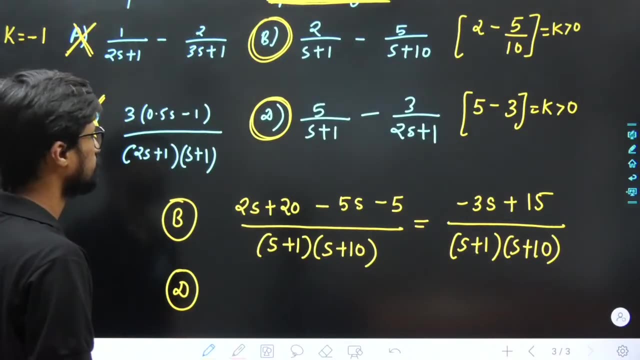 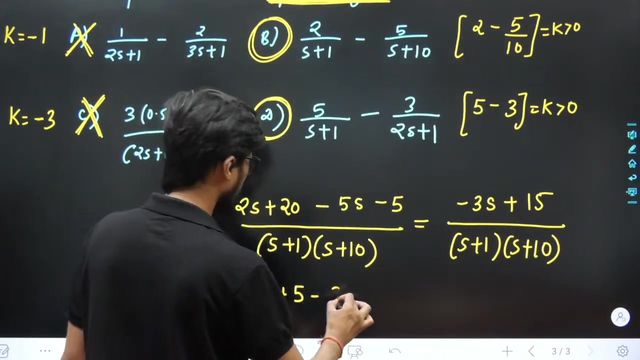 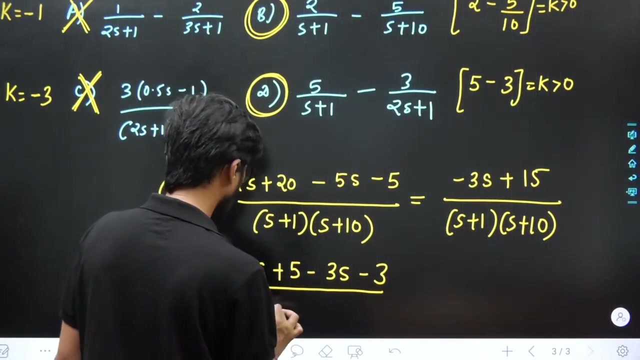 plus 10, this is the condition, right. If I solve the d option, solve the d part, then I will get 10s plus 5 minus 3s minus 3, divided by s plus 1 into 2s plus 1.. 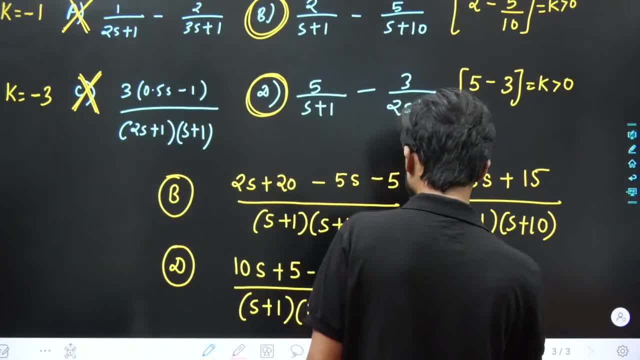 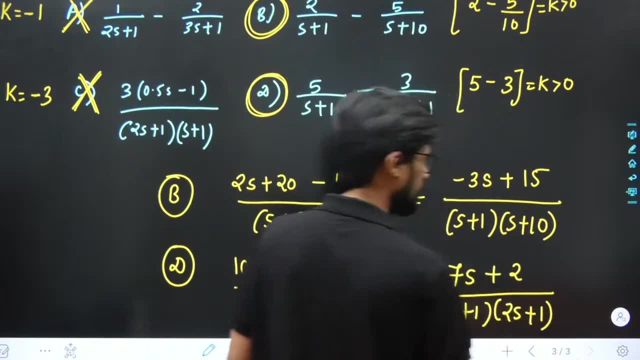 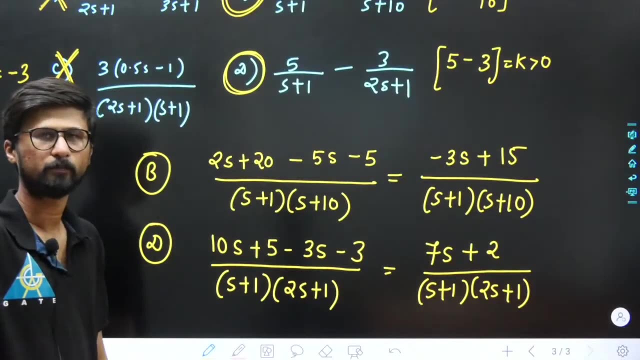 This will be equal to 2s plus 1.. This will be equal to 7s plus 2 upon s plus 1 into 2s plus 1, I have solved both of these. I have solved both of these things. 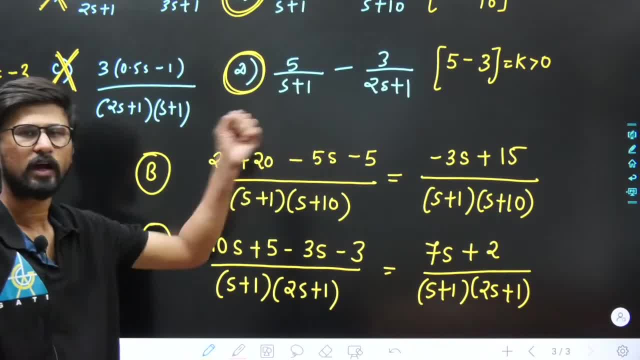 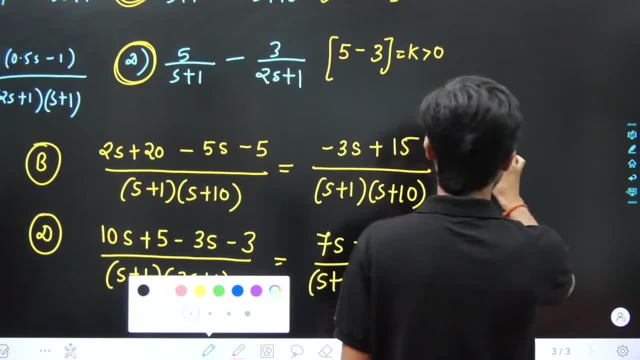 Now what you have to do is to get zeros. How do you get zeros? Numerator is equal to zero. So if you do the numerator zero, then how much will be its s? 5. Its s will be minus 2 by 7.. 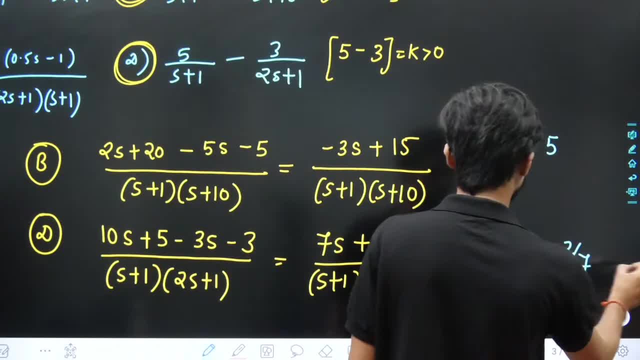 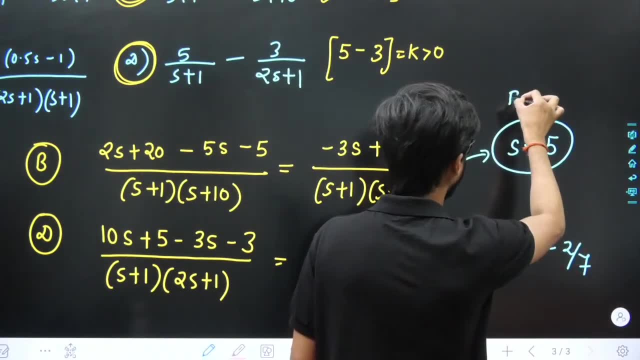 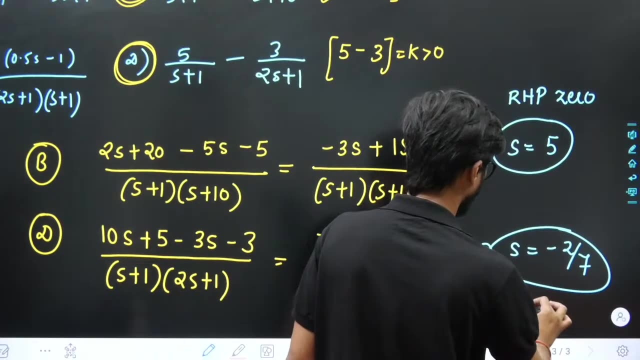 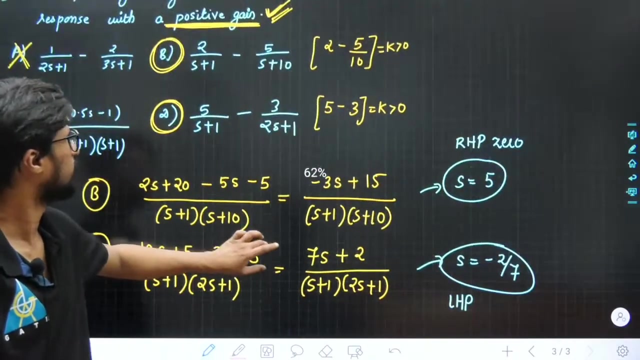 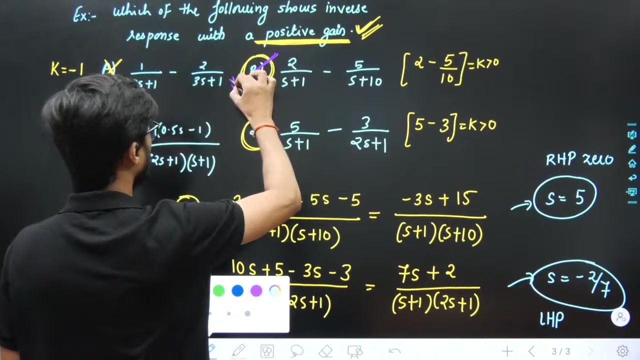 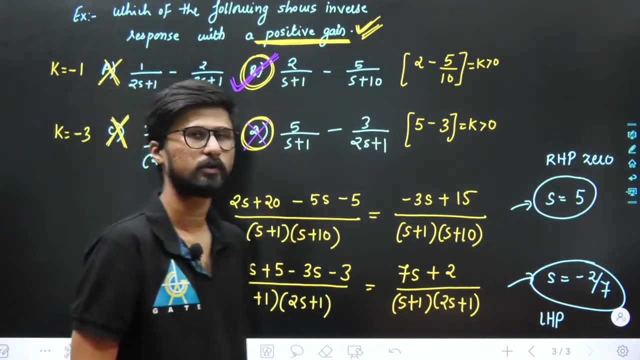 So you are seeing: its zero is right half plane, zero its left half plane. Its right half plane is its left half plane. So what will be the answer? 2s B is the correct option. B is correct. This is wrong. Is it clear? Note it down, So correct. 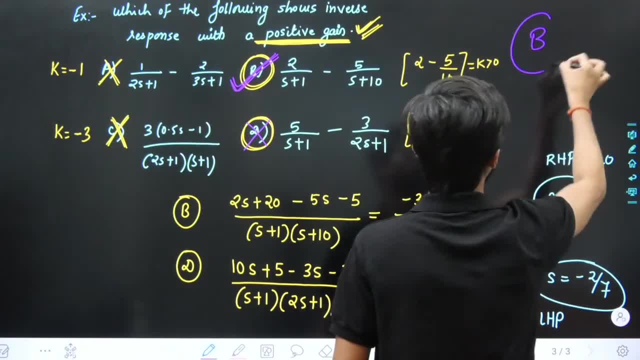 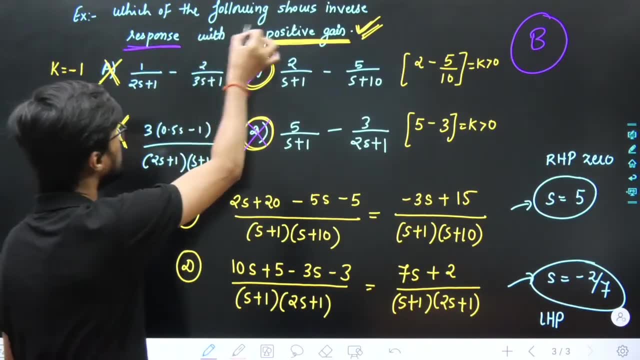 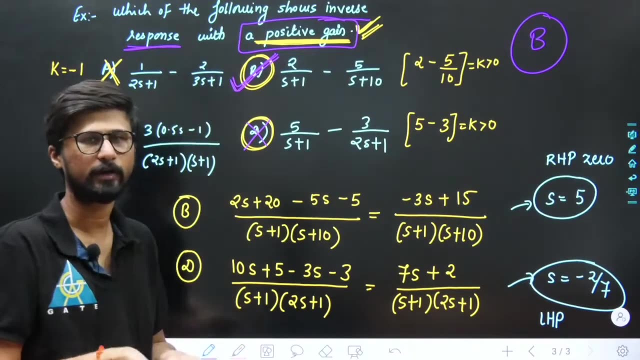 answer is B. B option is correct, B option. So read the question properly. Inverse response is asked, Inverse response is there. Talk about positive gain also. So how will you do this question? By eliminating the option Obvious thing. Which of the following is asked: 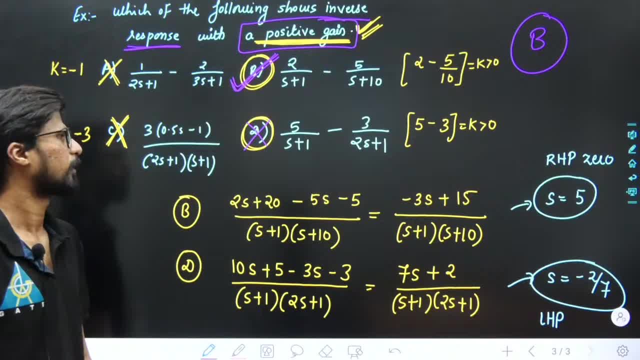 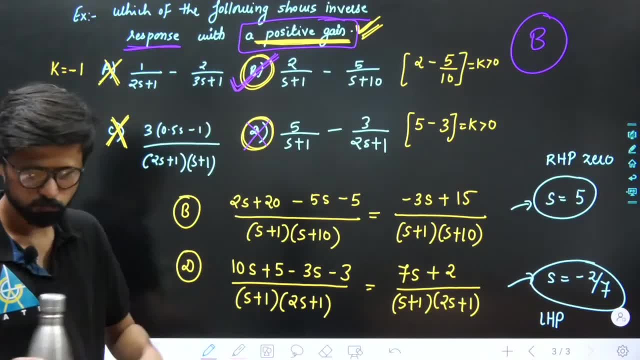 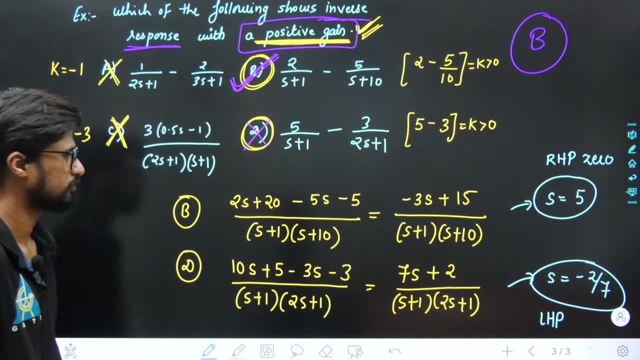 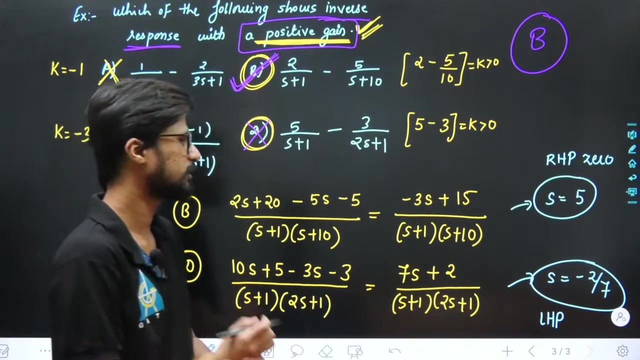 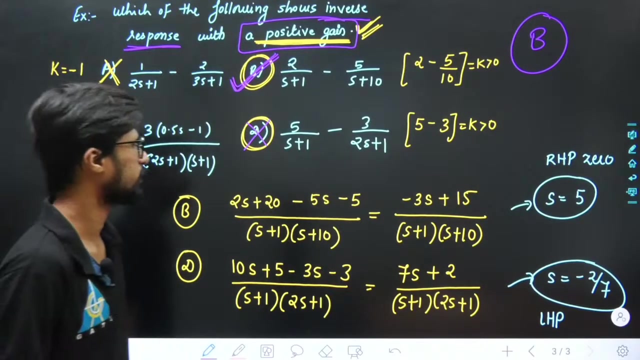 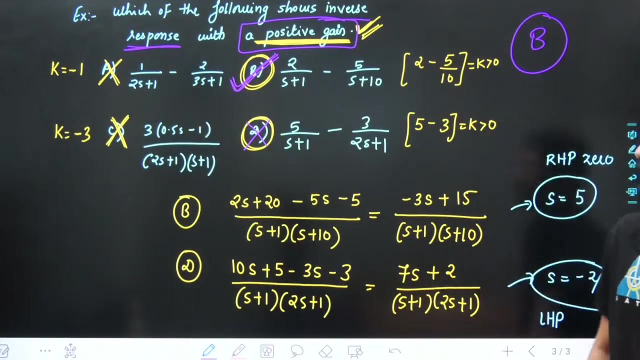 so one of these will be one: Note its solution. Is it clear? If there is any doubt, then ask: Is it correct? Is it clear? Come on, let us do next question. Let us do some question, then we will start feed forward control. Come on, look at the next question. 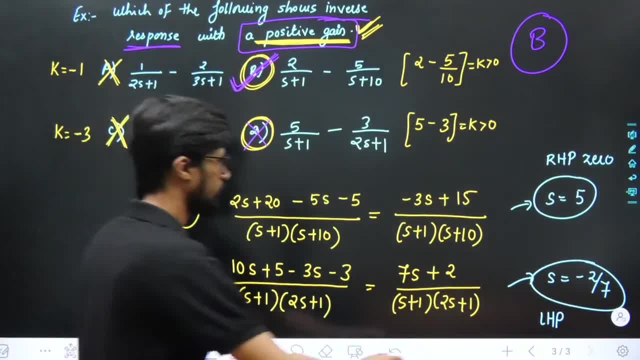 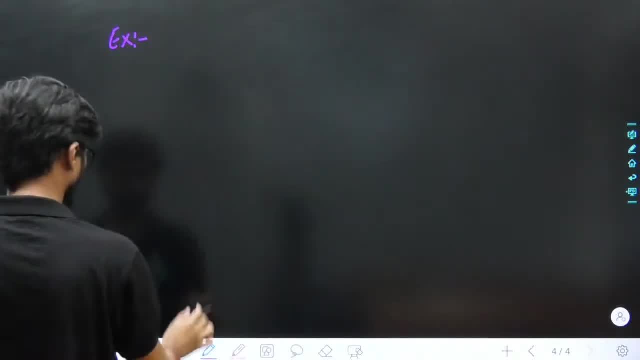 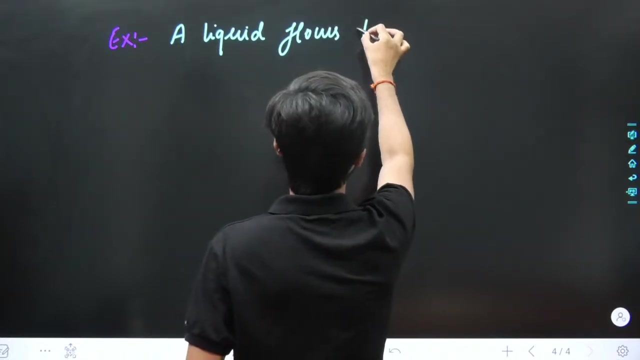 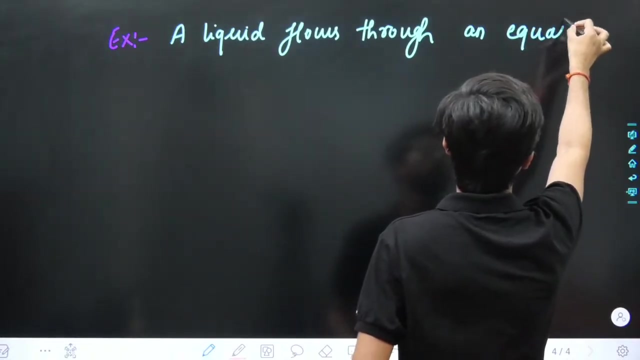 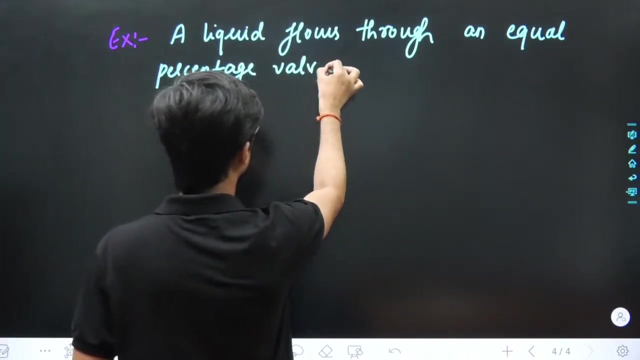 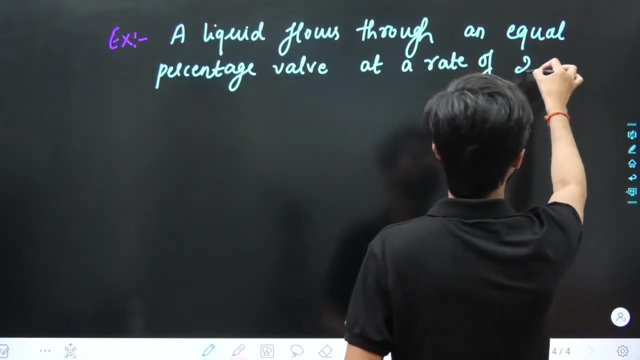 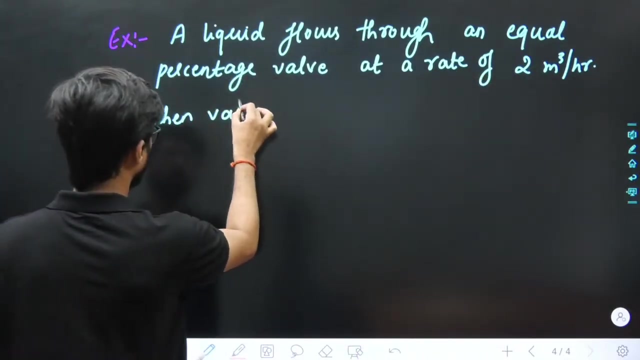 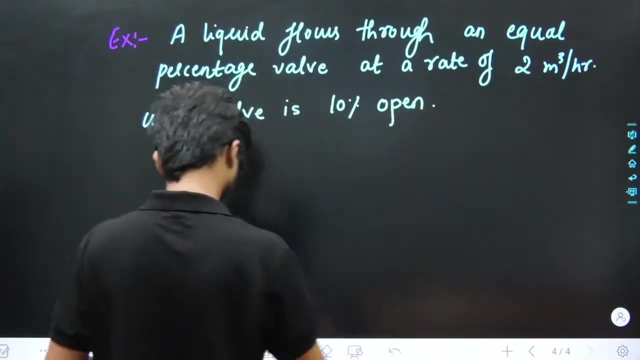 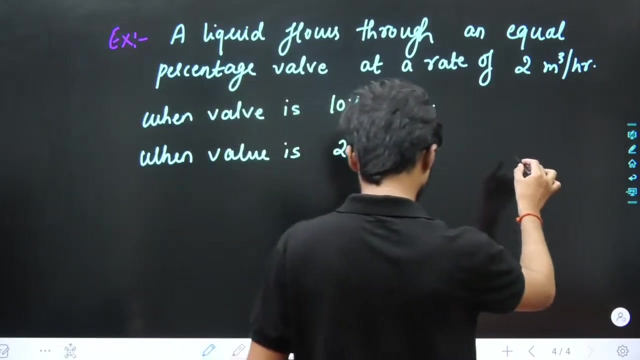 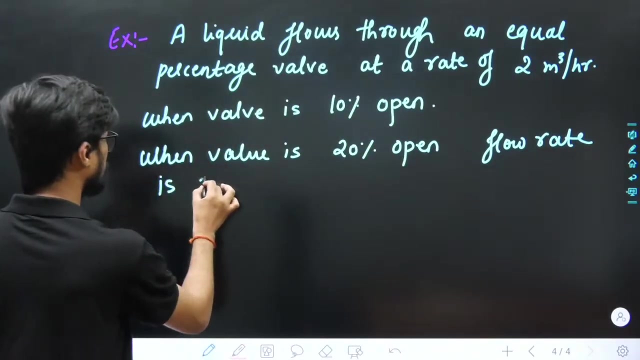 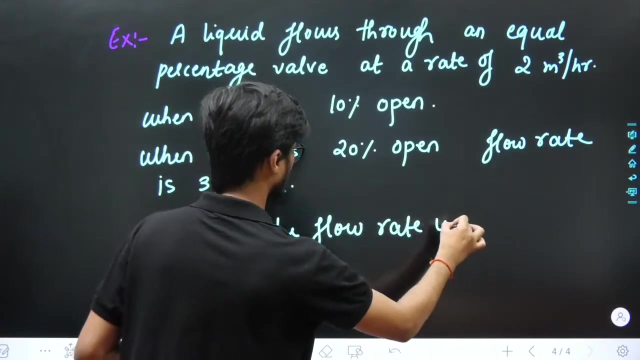 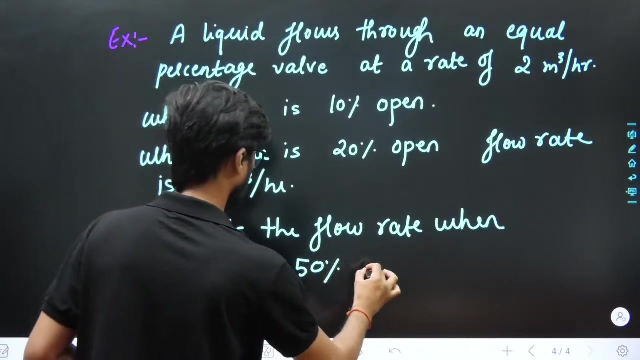 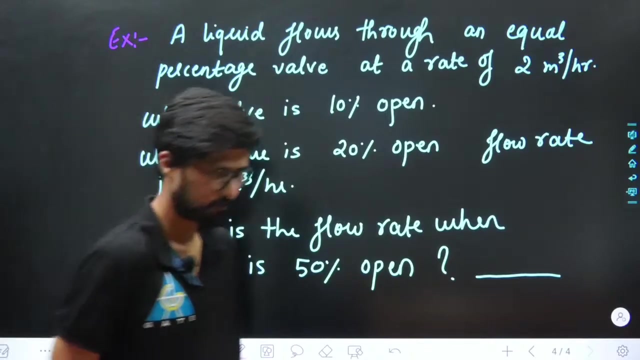 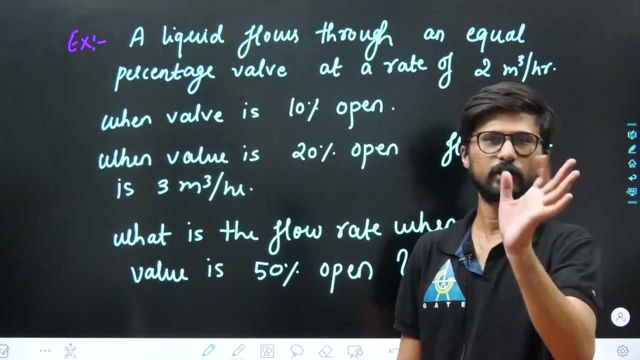 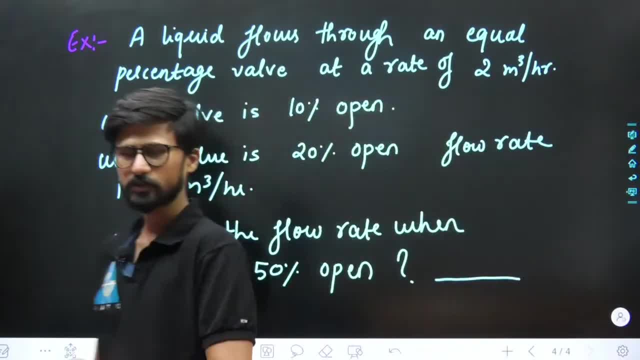 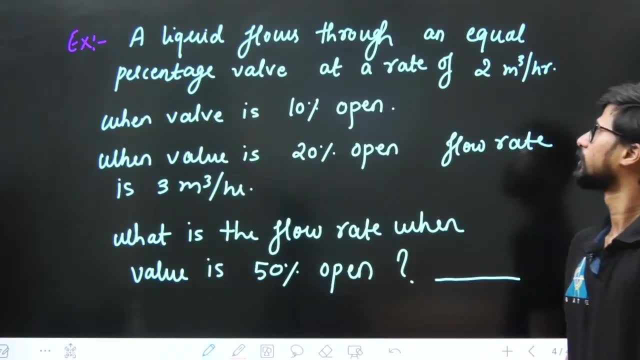 Zeros ka stability mein kol kaam nahi. Stability humesha aap pole se check karenge. Zeros does not interfere in stability. Chal ye next question. kariye jara Yeh wala question bana ye. 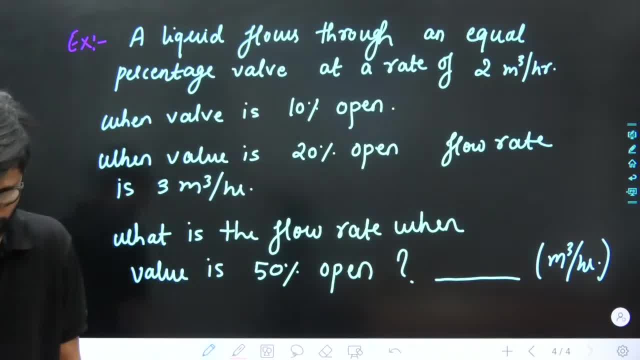 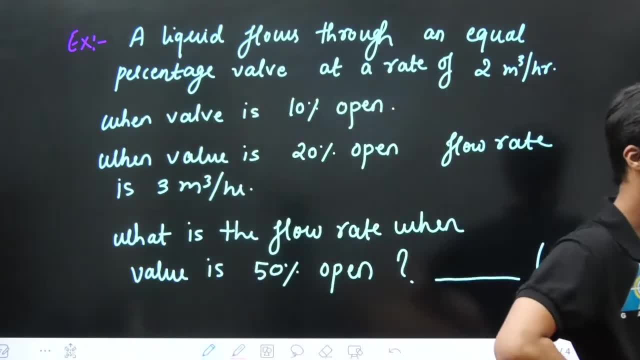 Next question: kariye jara: Zero negative aaya matlab. zero negative aaya matlab, wo left half plane ka zero hai Thik Zero sirf. yahi batata hai ki inverse response hai ki nahi, That's it, Thik. 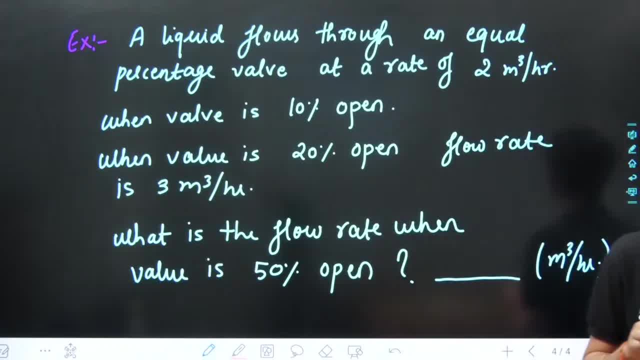 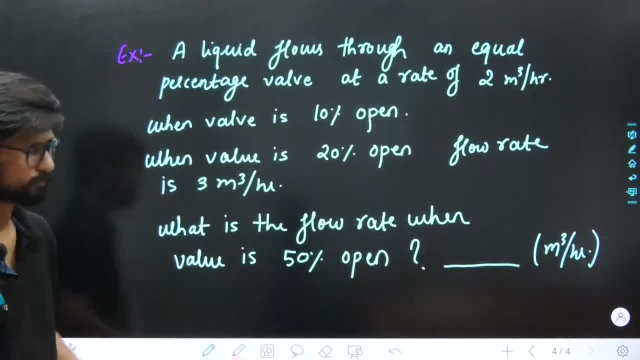 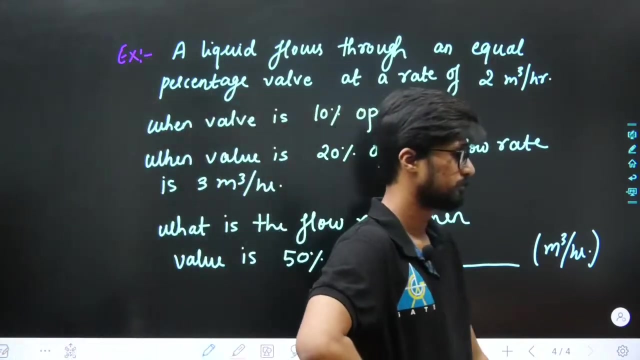 Aur humko uske baare mein aur kuch nahi jaa Thik Question kariye next jara Yeh wala Answer bataiyega. Answer bataiyega. Answer bataiyega. Solve kariye jara Answer bataiyega. 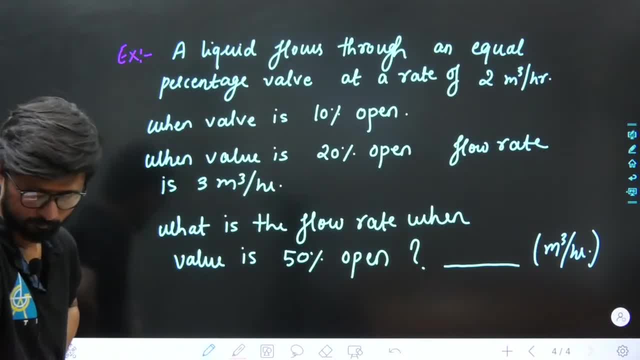 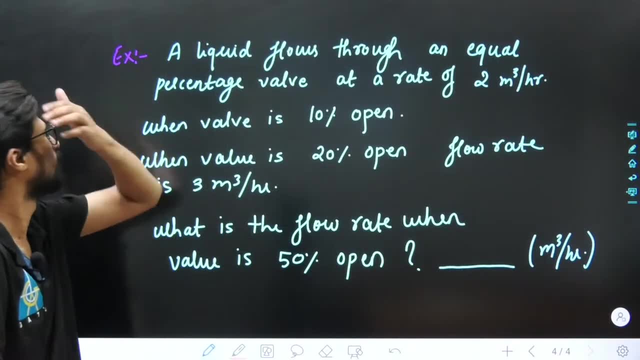 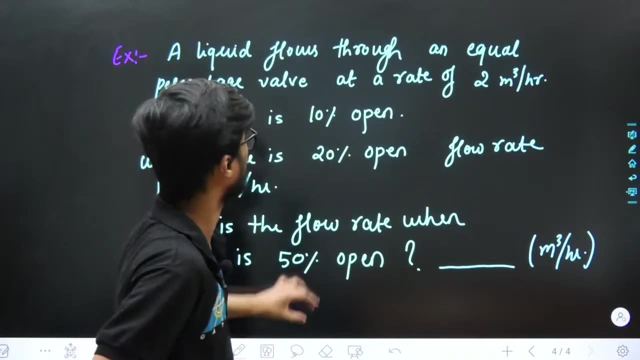 Solve kariye jara Answer bataiyega: Dekhe kya bol raha hai. Dekhe kya bol raha hai, Dekhe, Dekhe A liquid flows through an equal percentage wall at a rate of 2 meter cube per hour. 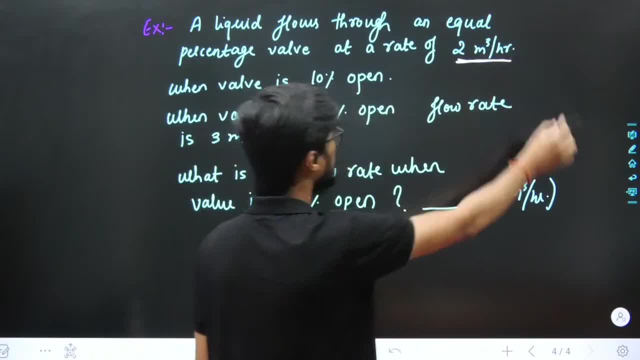 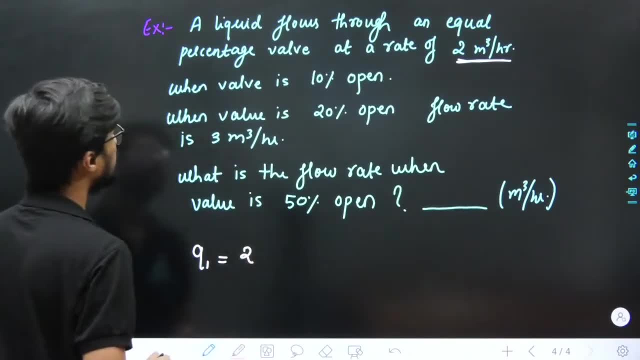 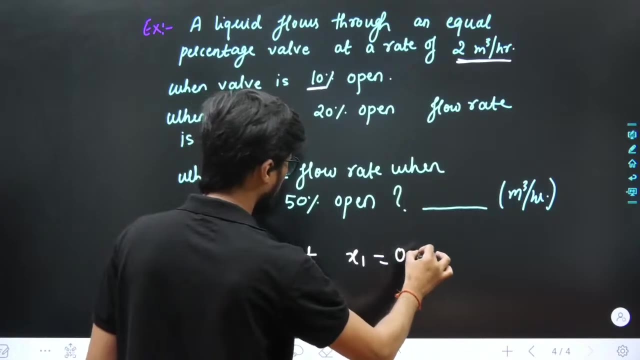 Remember kya diya hua hai, Flow rate, Kya diya hai Jo jo diya hai pehle, wo dekha kariye, Q1 is 2 at x1 is equals to 10 percent open Matlab: 0.1.. 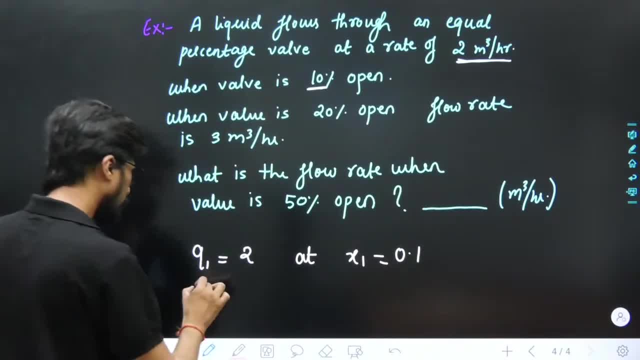 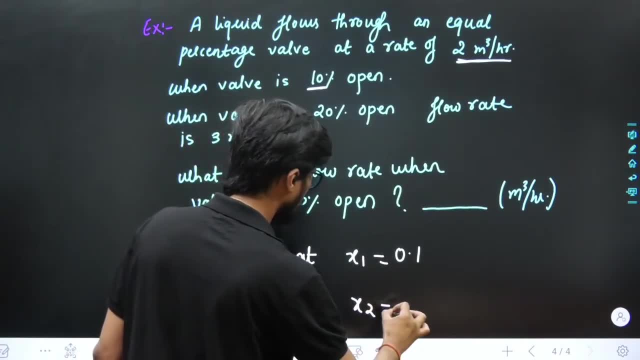 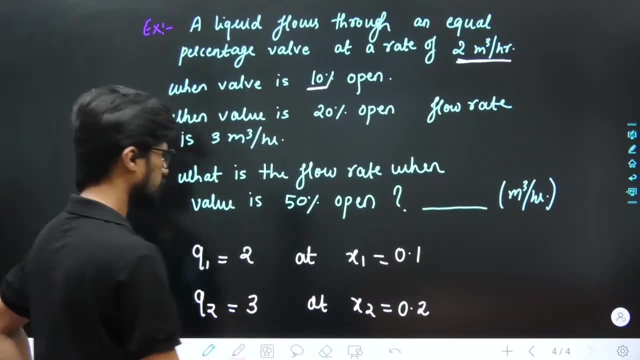 Fraction diya hai. Dekhe Q2 kitna diya hai. When wall is 20 percent open, Matlab x2 is 0.2.. Thik Flow rate is 3 meter cube per hour. Yeh condition diya hai. 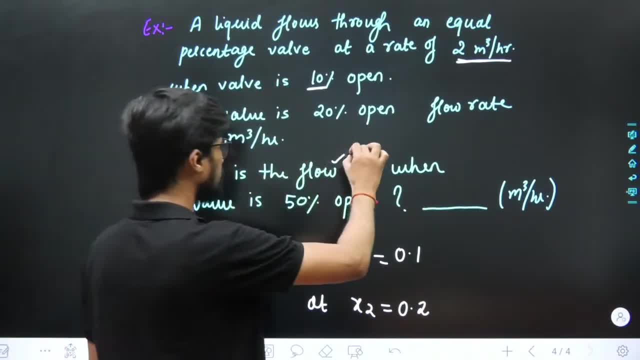 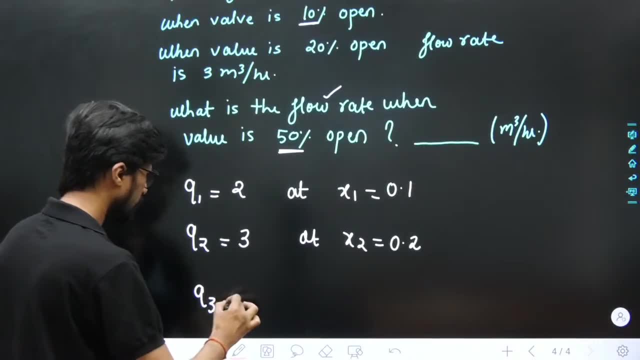 Aap se pooch raha hai ki flow rate kya hoga jab x will be 0.5.. Poocha kya hai Q3. pooch hain At x3 is equals to 0.2. Point. 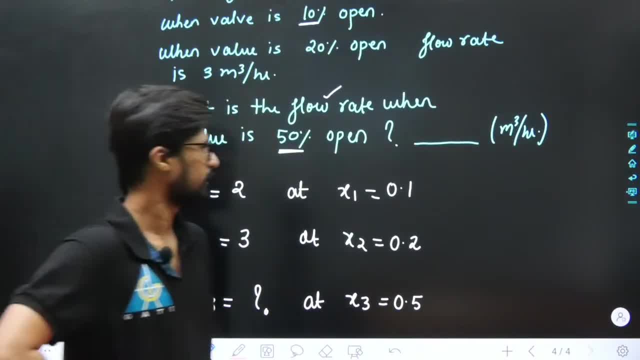 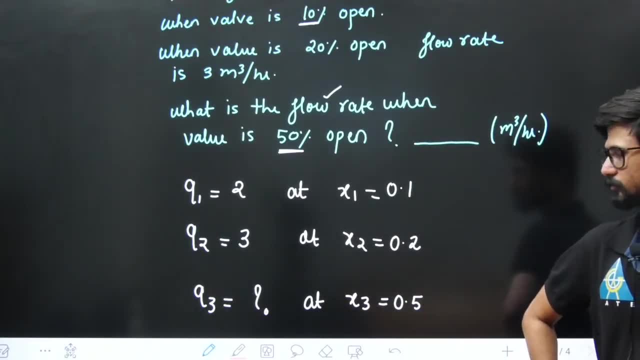 Yeh pooch raha hai. Thik hai. Karo zara isko. Equal percentage wall hai Formula already aapke paas hai. Equal percentage wall ka already formula hai ki nahi. Karo zara isko. 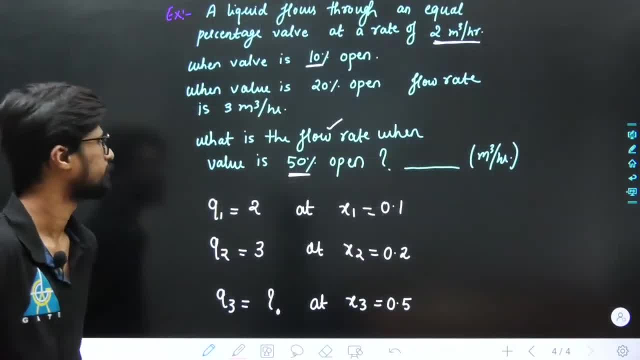 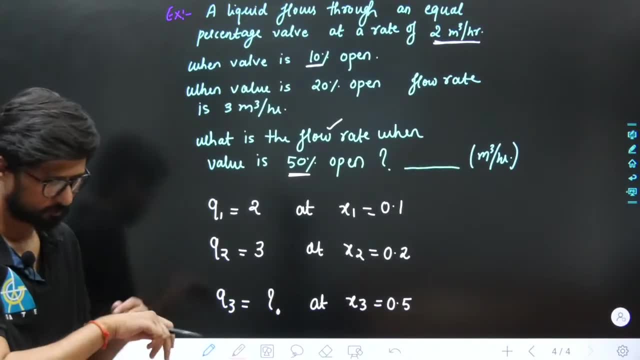 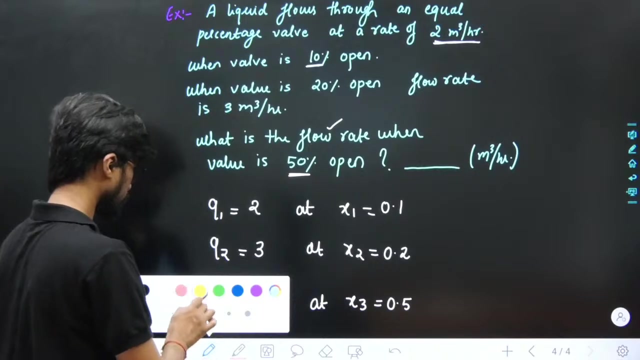 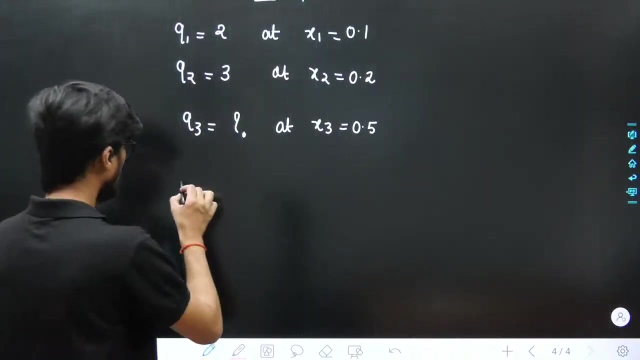 Kariye zara isi cheez ko, Karo zara, isi cheez ko Karo zara, isi cheez ko. Dekho, Dekho, Kya formula equal percentage wall ka, Kya formula equal percentage wall ka. Fx is equals to alpha x minus 1.. 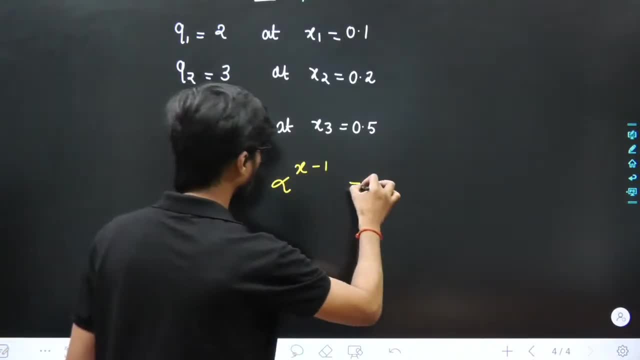 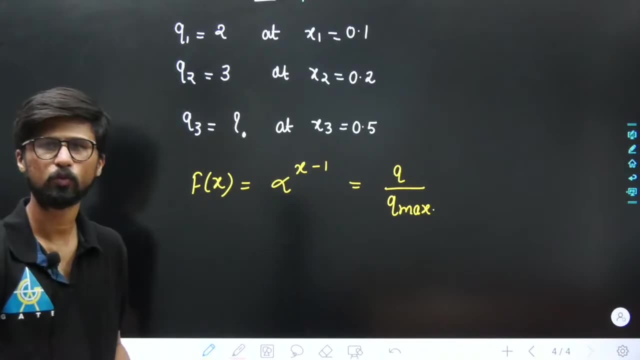 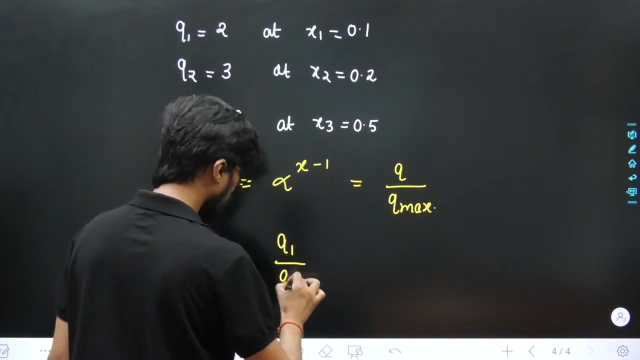 Yehi hai Fx. kya hota hai Q by Qmax. This is Q by Qmax. Aap dekhega, Agar mai Q1 by Q2 ka ratio loo. This means Alpha x1 minus 1.. 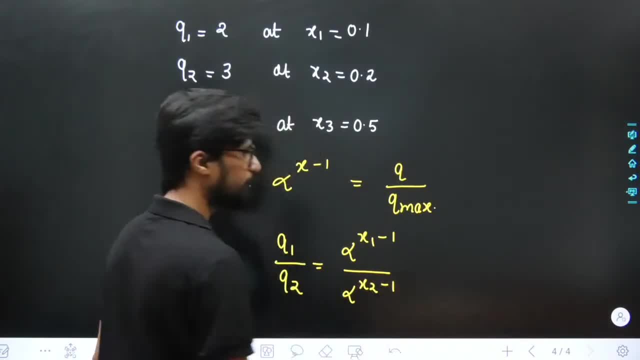 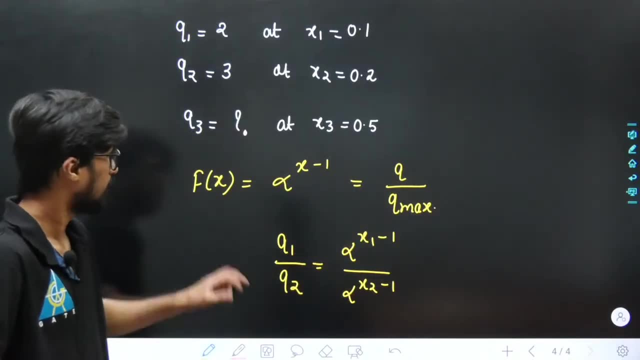 Upon alpha x1 minus 1.. Upon alpha x2 minus 1.. Ratio: lia maine Q1 by Q2.. Thik hai Q1, pata hai Q2, pata hai X1, pata hai X2 pata hai. 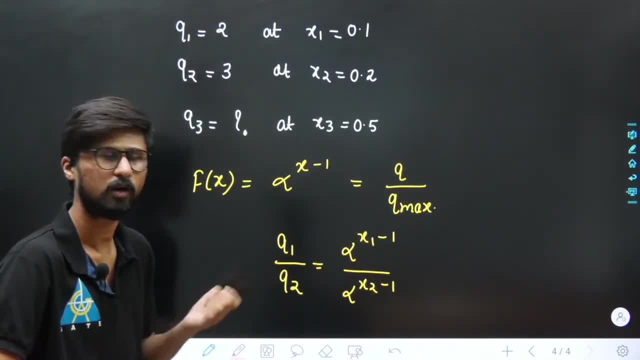 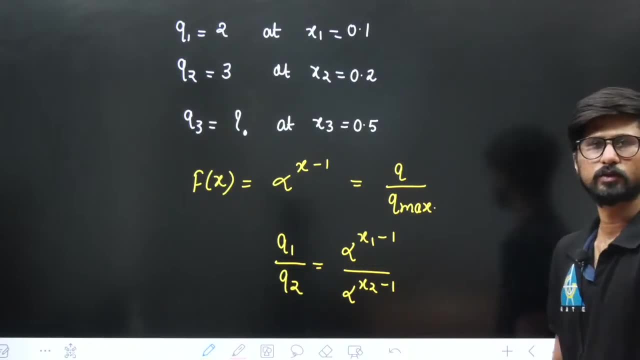 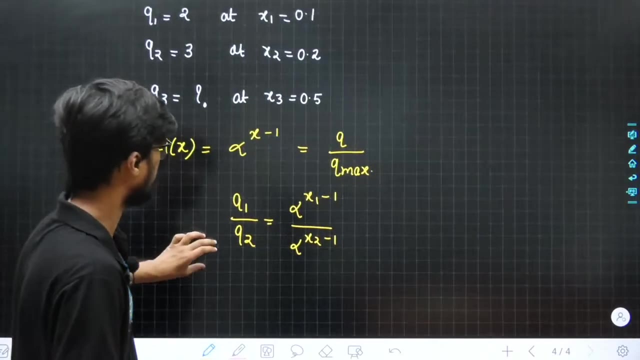 Alpha nikal jayega, aapka Alpha, nikal jayega, ki nahi Thik. Alpha nikal jayega, Nikalu, zara Alpha nikalu Nikalu. Alpha 2 dataya sakte aap? 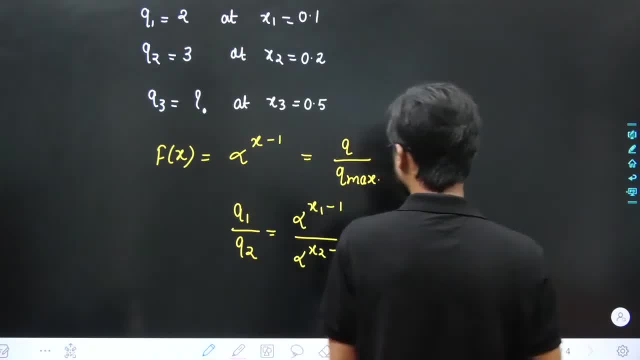 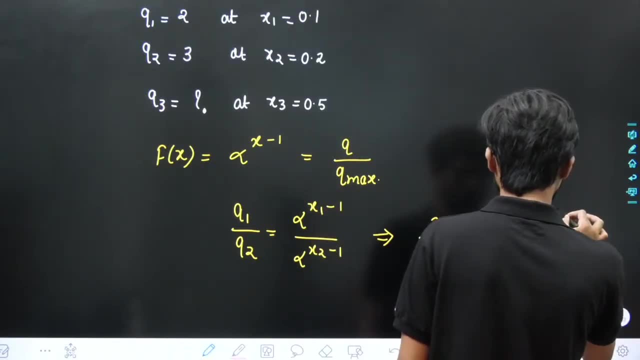 Hasi idea. This Ph relegao to kya tahe Jaahe hai. Khi aap ka Alpha, kayo pa Kh whale nikal, nikal nila Alpha. kya nikal nila Nikal, yaba hai nikal. 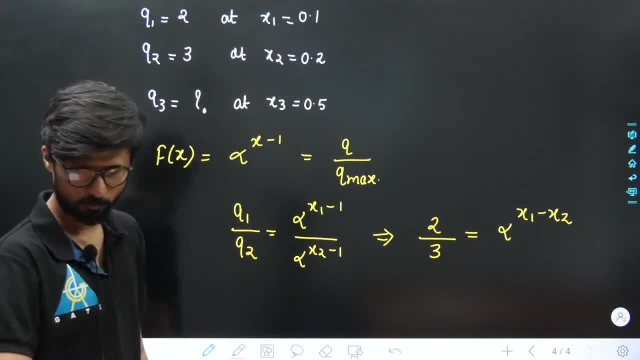 Alpha 1: kalana nayai Nikal ul Bali yaya na Started ahle hap disa pe Khi hla pahar ki tam Jaahe hai Hla apan Nike dhuga missing aa2itiya. 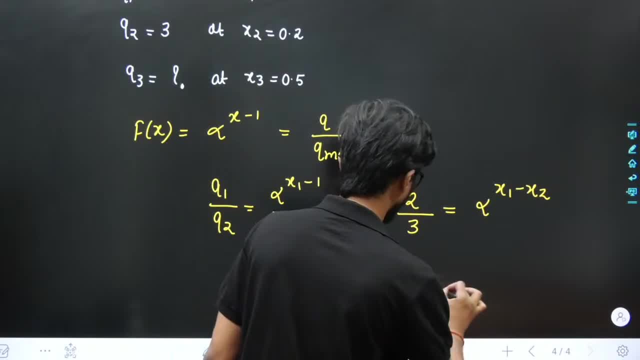 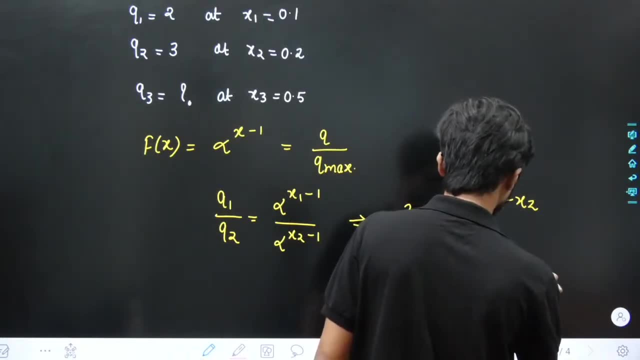 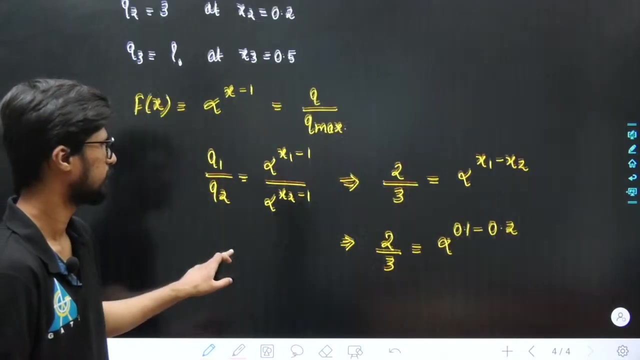 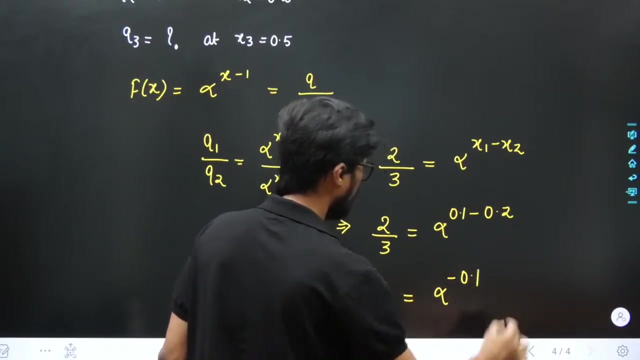 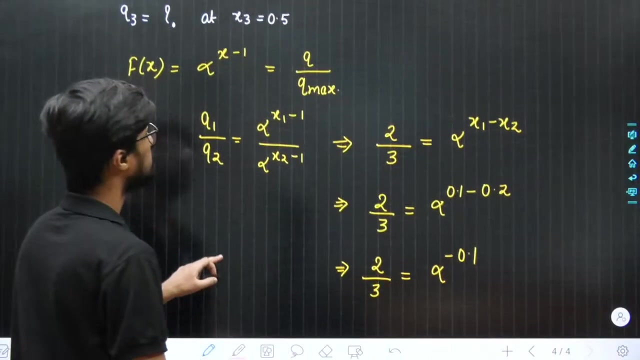 This is equals to 2 by 3. alpha x 1 is 0.1 minus x 2 is 0.2.. This implies 2 by 3 is equals to alpha, to the power minus 0.1.. Alpha is 57.67.. So alpha is 57.67.. This is the value. 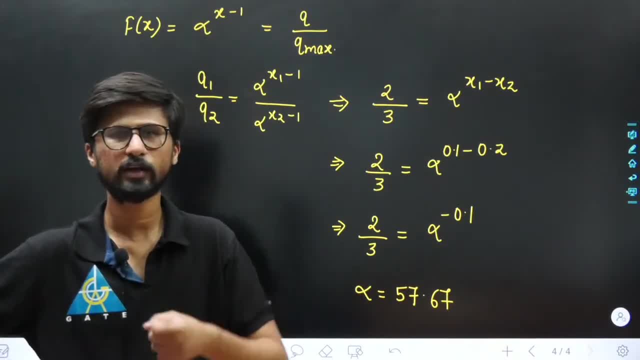 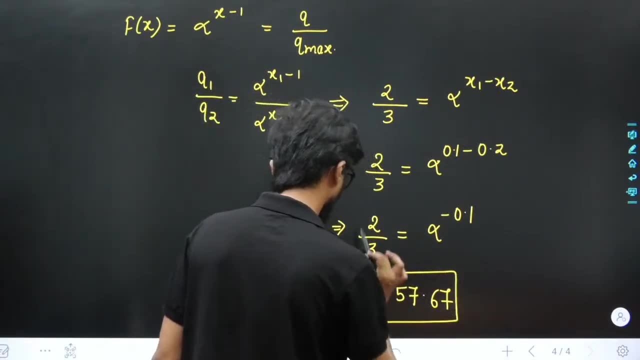 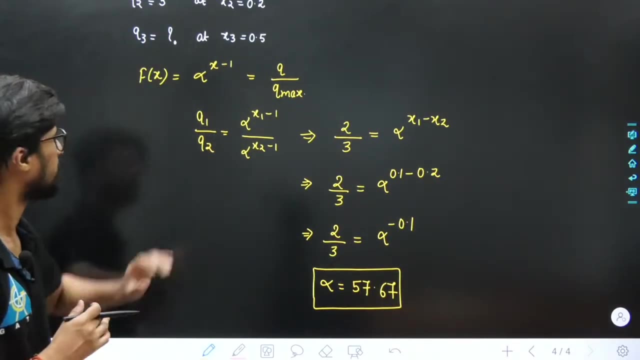 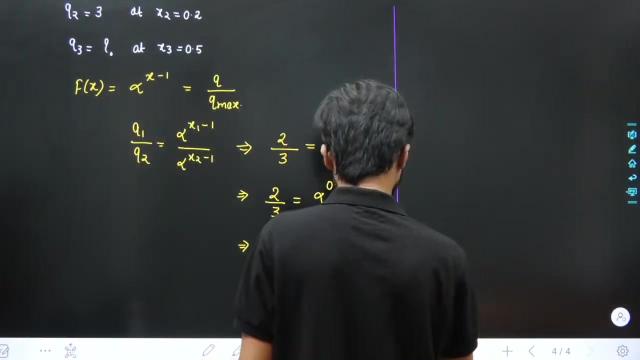 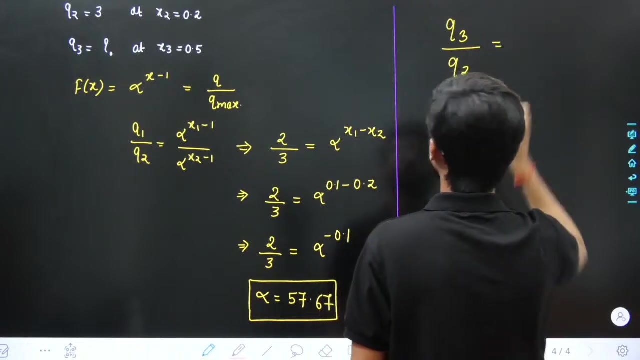 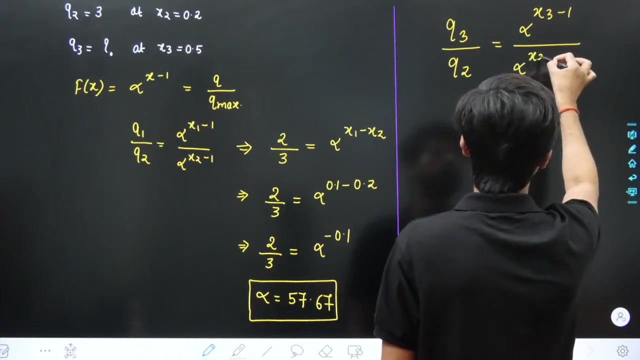 of turnover ratio or rangeability. So this is alpha. What do you have to do? You have to take out q 3.. So when alpha comes, then see what we will do. Now see what I am doing: Q 3 divided by q 2. This will be alpha x 3 minus 1 upon alpha x 2 minus 1.. Let us do. 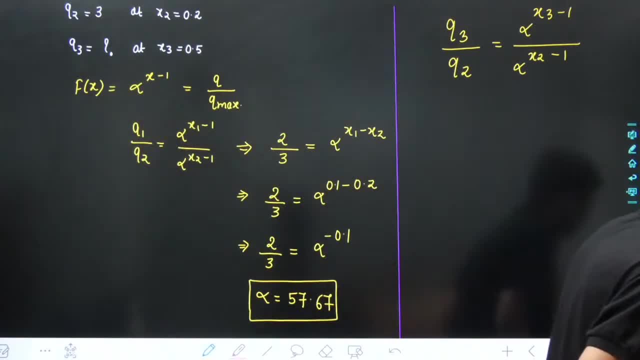 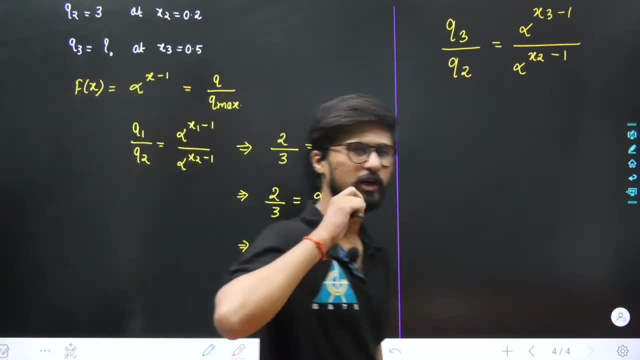 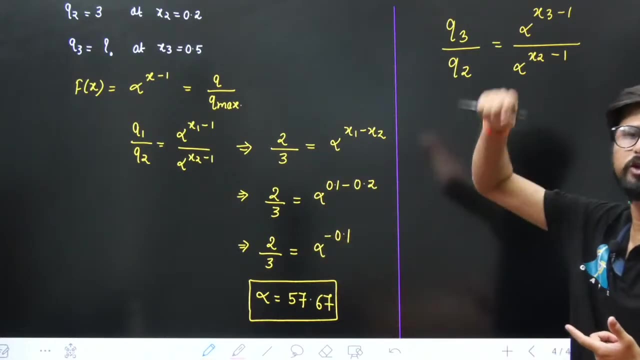 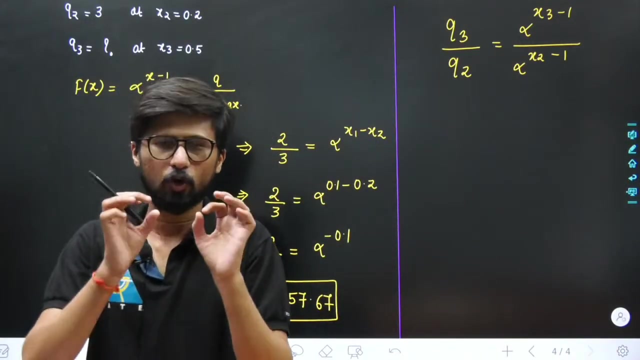 this. Okay, Rishabh, Will it work? Whenever you do this calculation, always do it up to 3 decimals. Whenever you do this log or to the power calculation, always do it up to 3 decimals. A little accuracy comes in the answer and range is given in the gate. Your answer will never go out of range. 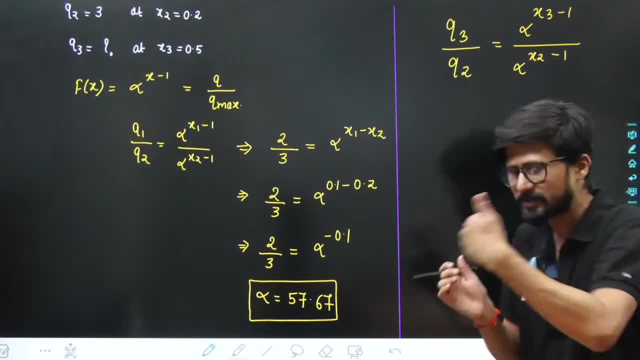 Otherwise, if you keep doing round off in the beginning itself, then the answer will never go out of range. Otherwise, if you keep doing round off in the beginning itself, then the answer will never go out of range. Okay, Chances are there that it happens with a lot of students. that answer use in the right. 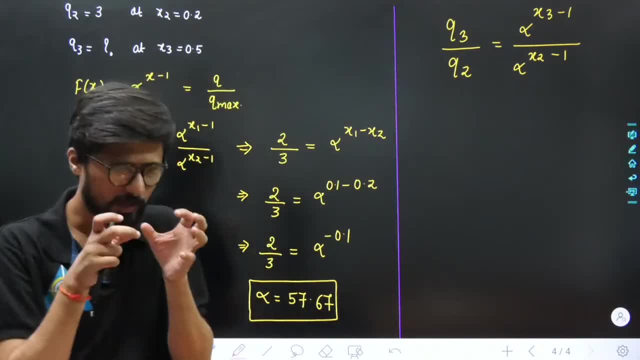 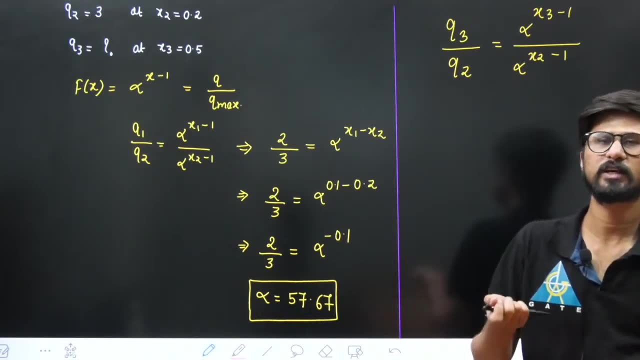 range of response. Nice, Nowadays in the range search tousles is very low. Earlier what used to happen is: first 57.6 answer came, So the range was given very long. Ok, give 57 to 58. Now give completely closed range. Whenever you do the calculation, do. 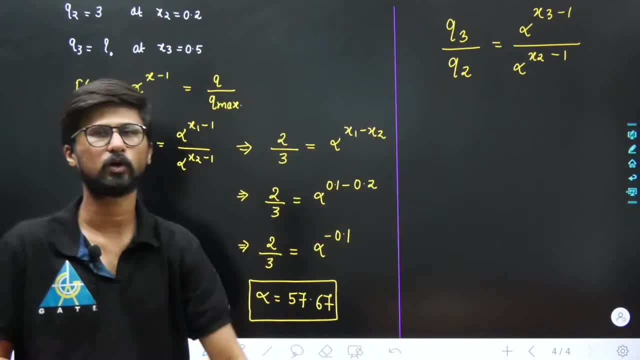 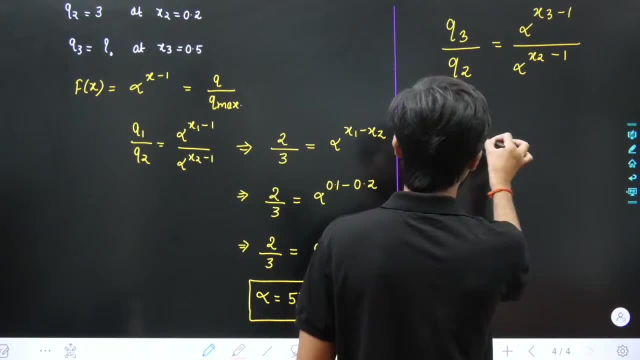 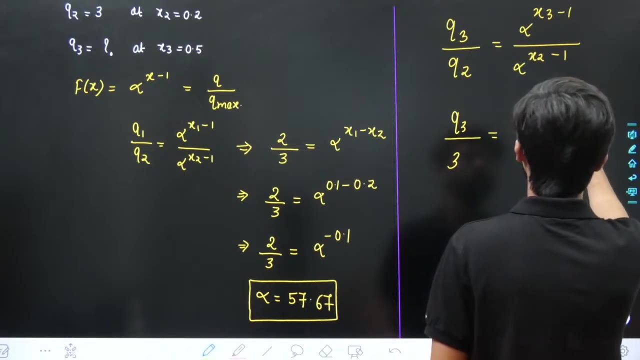 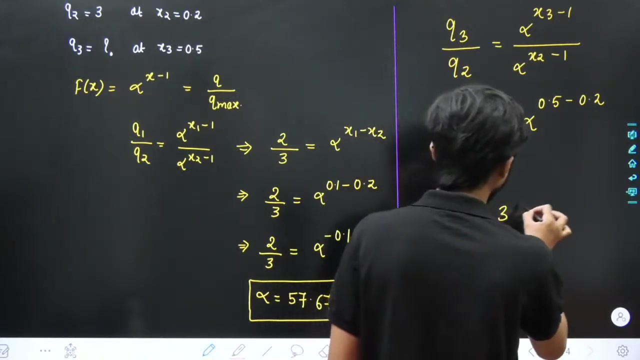 it up to three decimals, Okay, Okay, Now take the ratio of this. So I have to take out q 3.. Q2 is 3, alpha x3 is 0.5, minus x2 is 0.2 and alpha's value I know. So Q3 will be 3 times. 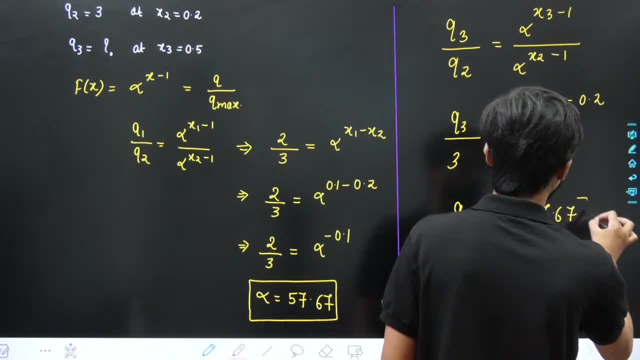 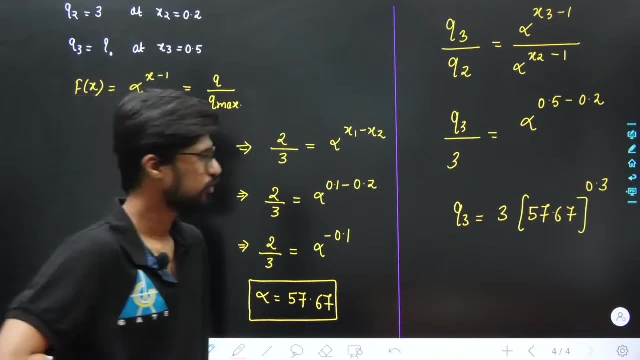 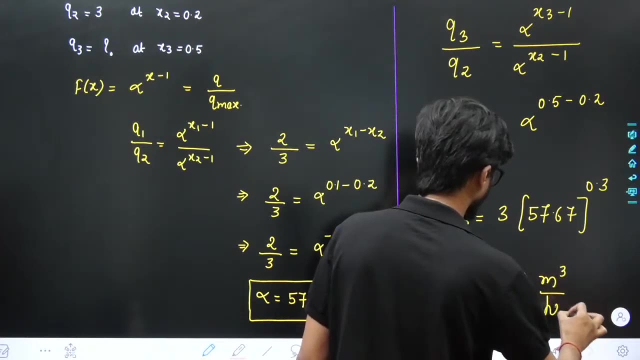 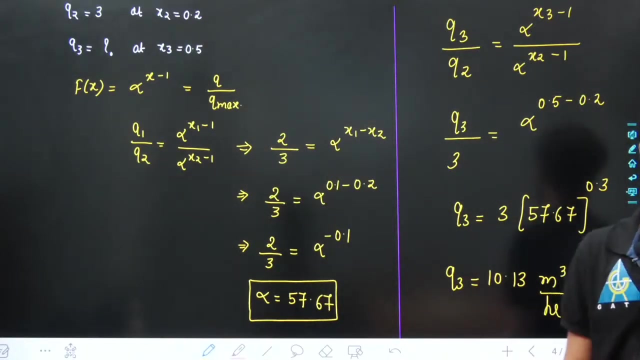 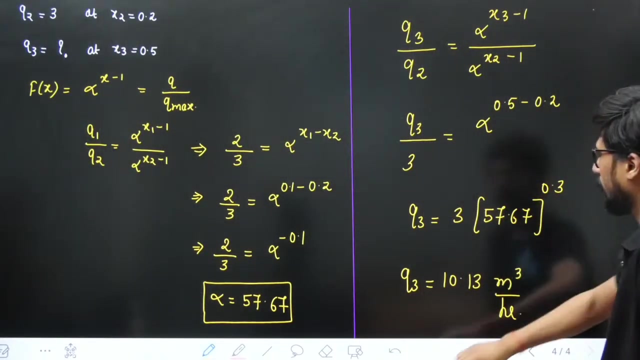 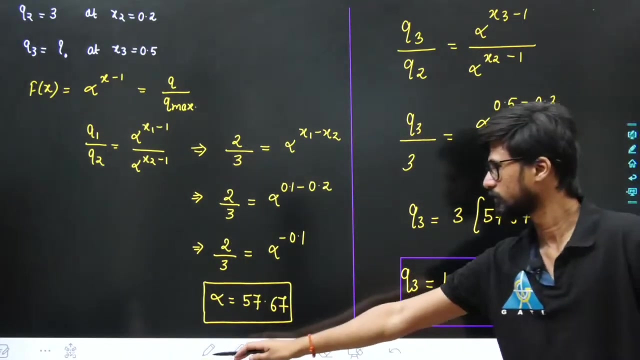 57.67 into 0.3 to the power 0.3.. So answer will be 10.13.. So this is your complete solution. Is it clear? This is your solution. Note this. Let's move to the next question. Is it 11.43?? 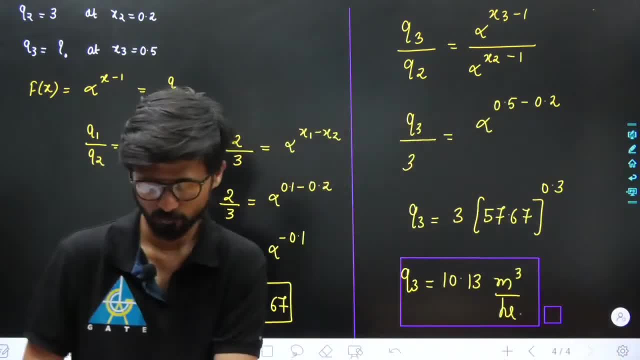 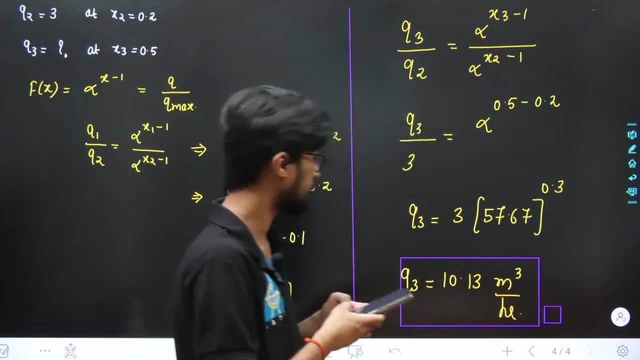 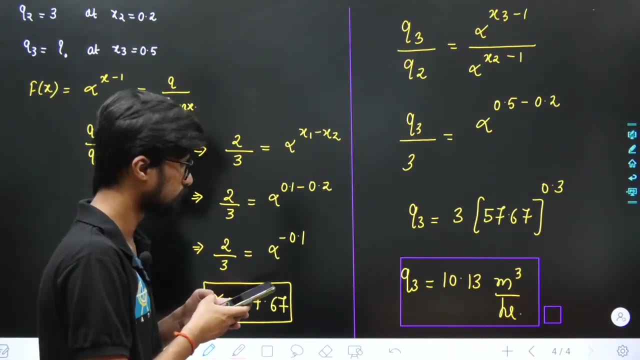 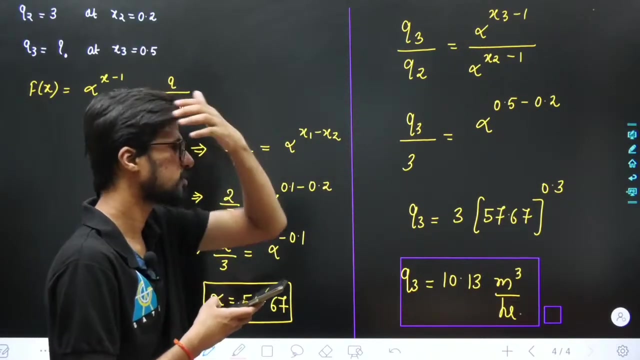 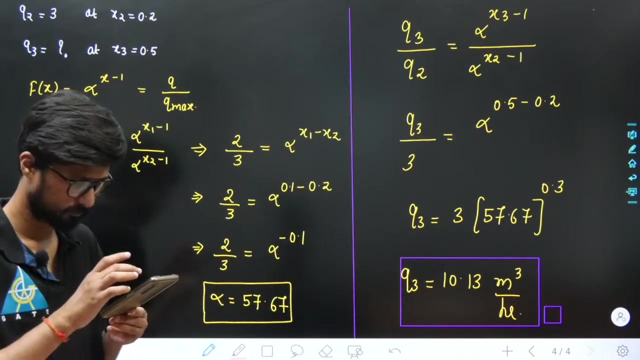 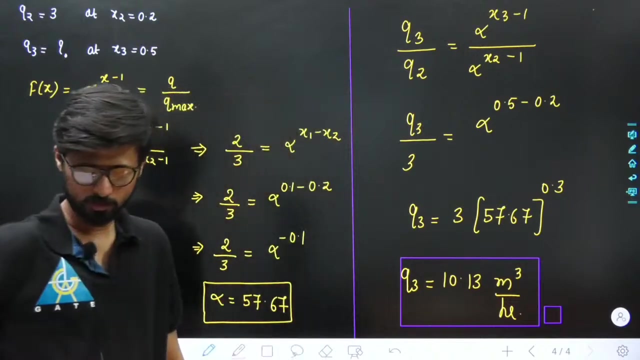 You have to do the calculation. Let's see. Let's do the calculation and see Approx of 10.13 is coming 10.13.. 10.13 is correct. Check it once, Navin. you must have made a mistake in the calculation. Check it. 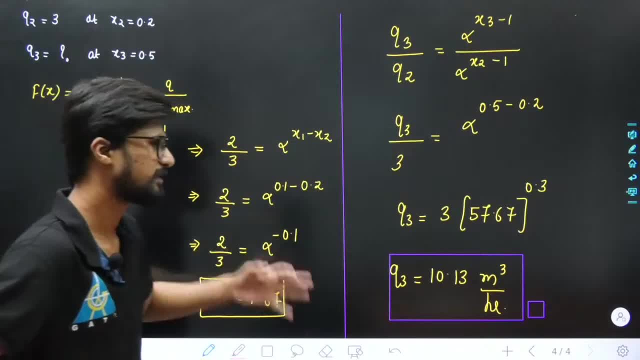 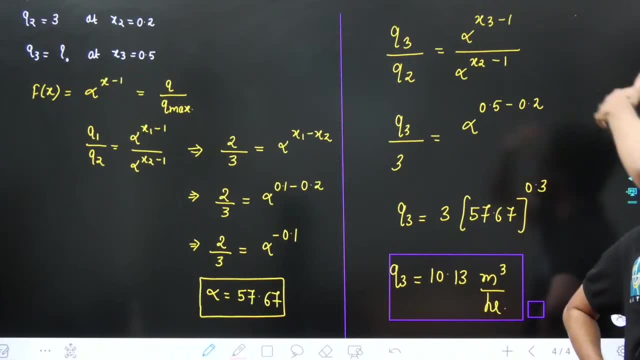 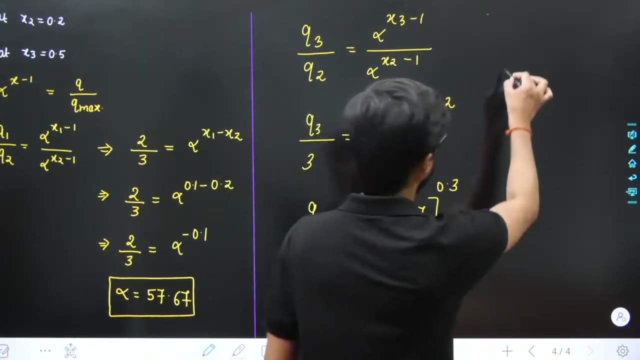 Okay, So we will make a simple question from the wall. Okay, No problem, Sorry that there is no problem. Okay, You are making a mistake now. So if you have made a mistake, then write it somewhere. Write it here in front of this question. 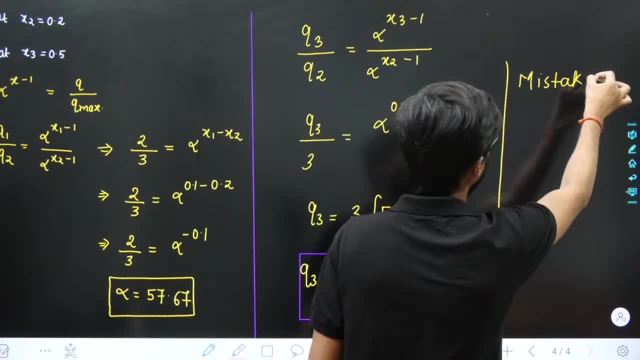 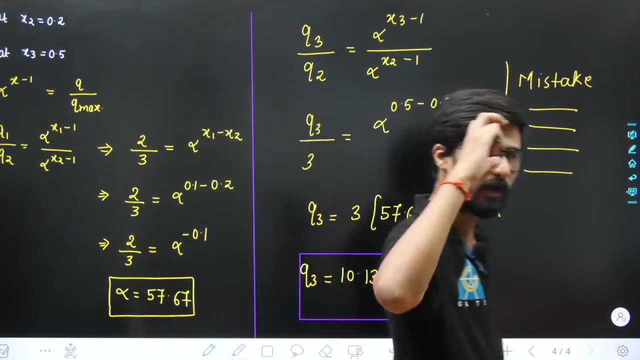 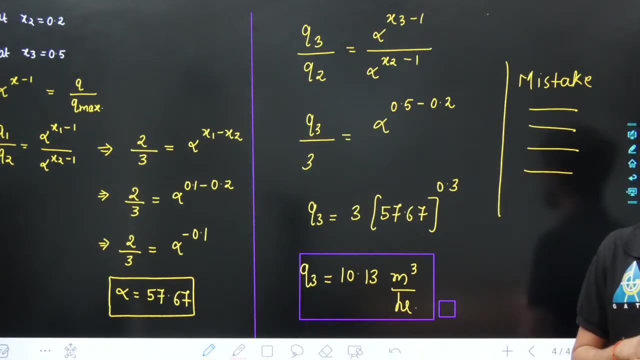 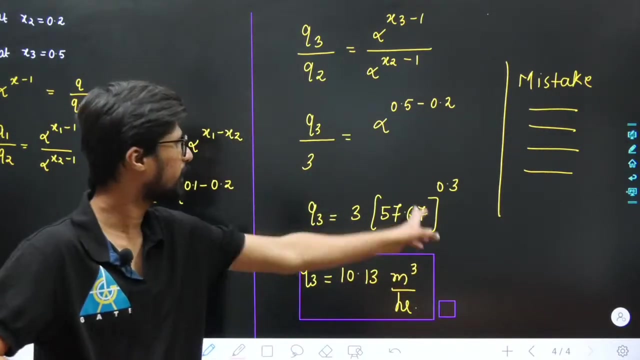 That I did this mistake, That I did this mistake. If you keep writing, then that thing will keep coming in your mind Again and again. Okay, You will feel that you made a mistake here. So when you are doing a similar type of calculation, then this thing will come in your mind: that I have to do this thing carefully because I made a mistake here once. 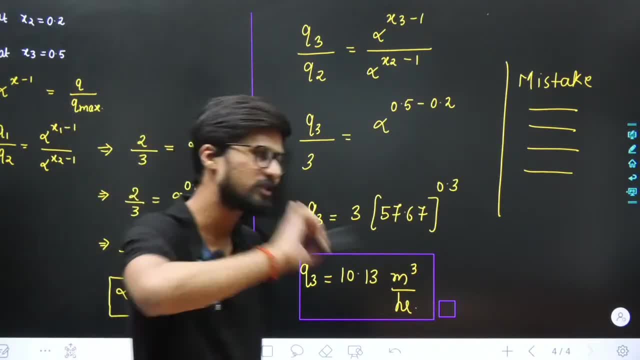 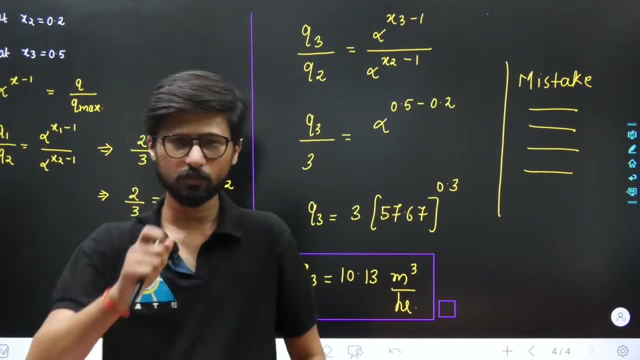 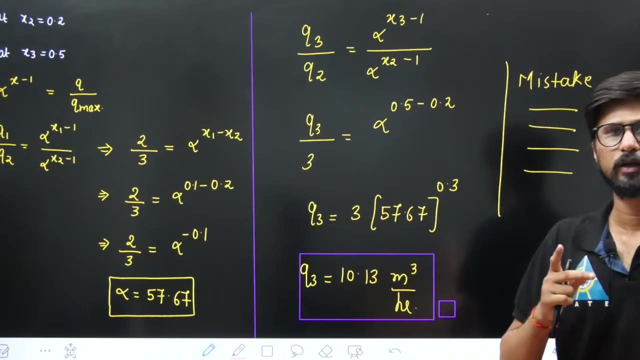 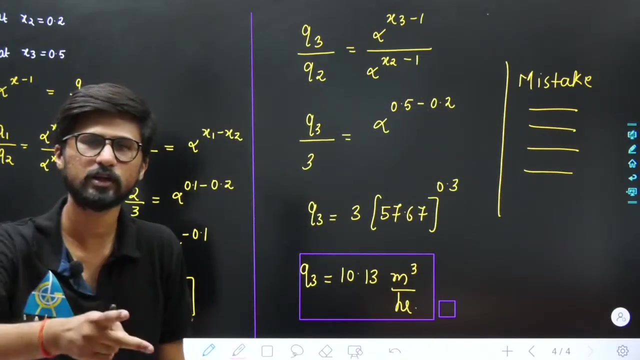 Okay, And due to that, your silly mistake will go away slowly. Okay, Write the mistake. now You will write the mistake. Do this for two months. Do this for two months. Okay, Do this for two months. Okay, If you don't feel any change, then don't do it. Okay, If you don't feel that your silly mistake is going away slowly, then don't do it. 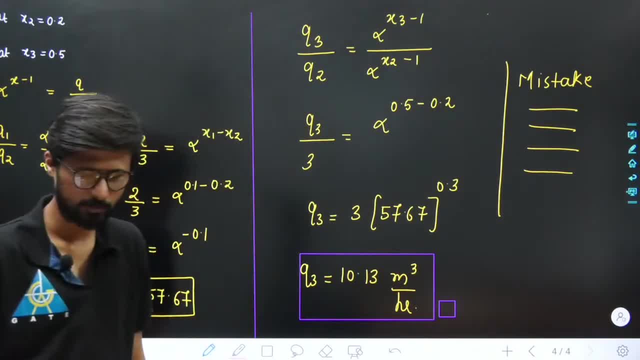 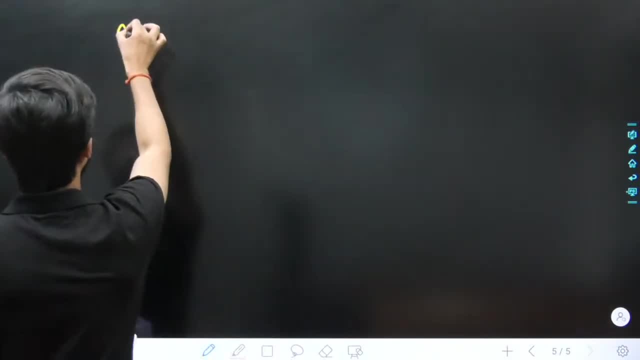 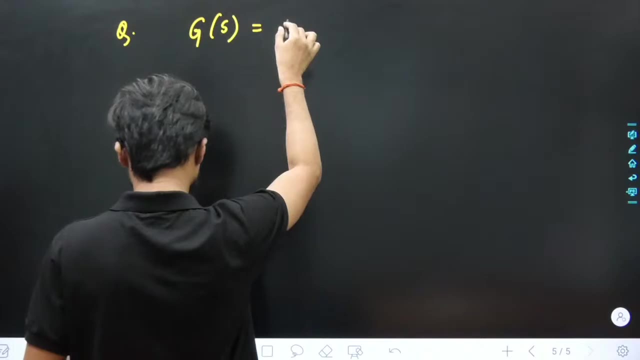 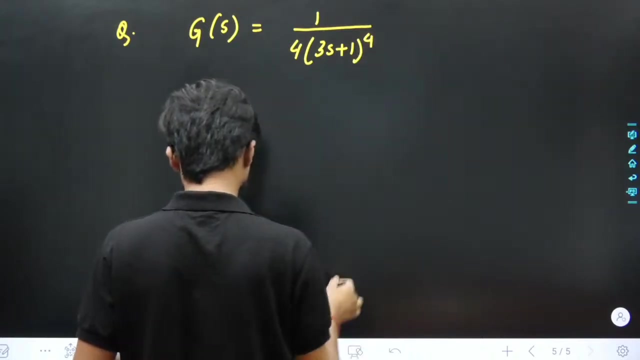 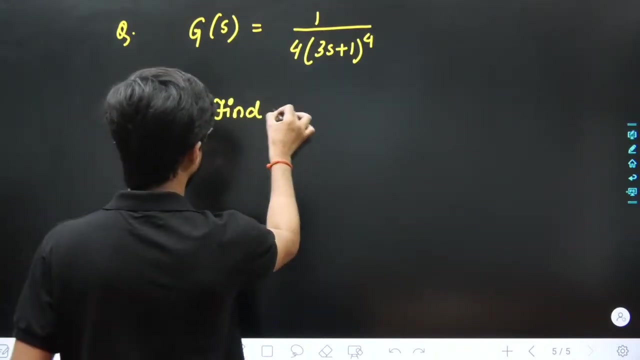 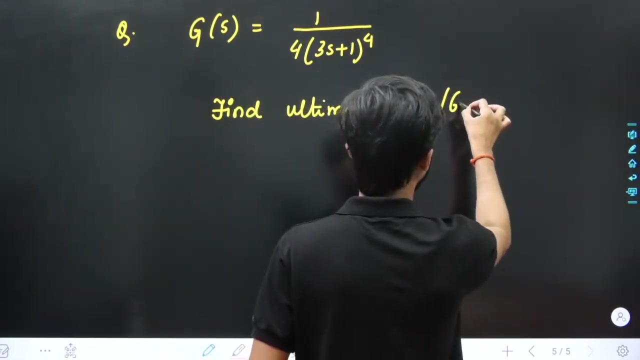 Do this for two months and see that it will go away slowly. Okay, Okay, Next question. Let's take the next question. Okay, Open loop transfer function is given. Okay, Okay, Open loop transfer function is given. You have to find. 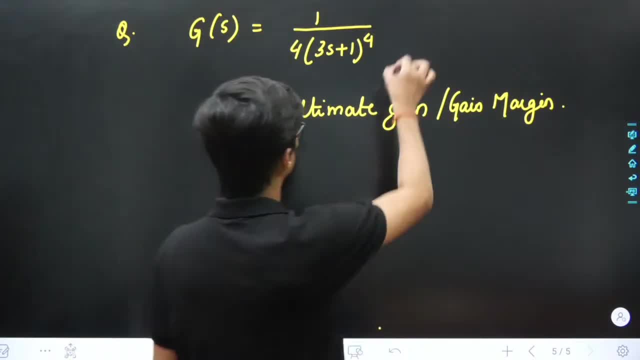 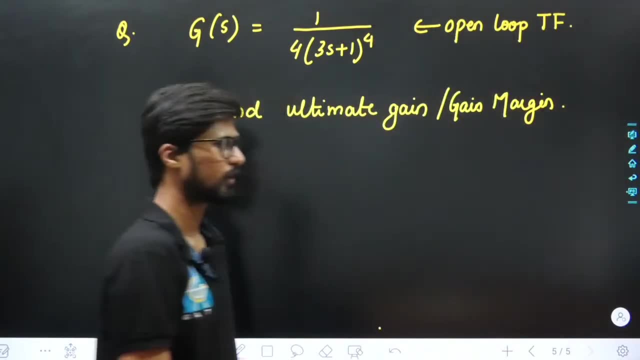 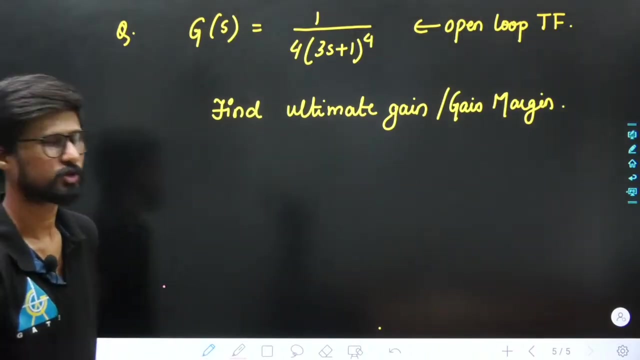 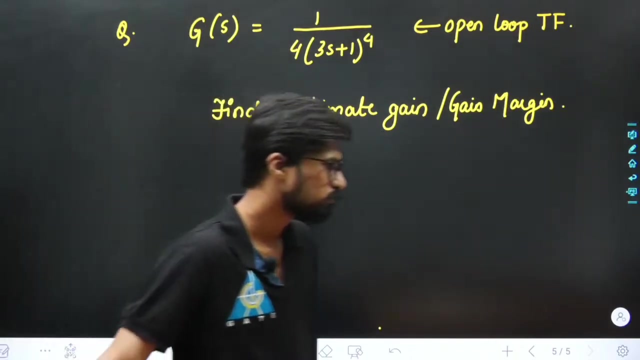 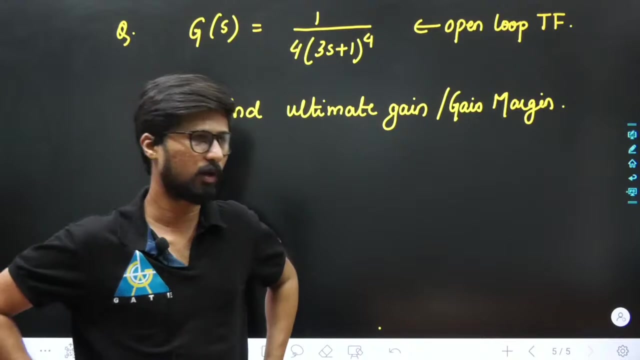 Okay, Okay. So we have to find the ultimate gain or gain margin. Let's try to find it Okay. Let's try to find it Okay. Yes, Yes, Yes, Yes, Yes. I have already told you about mass transfer. let me tell you again now: ma'am's mass transfer. 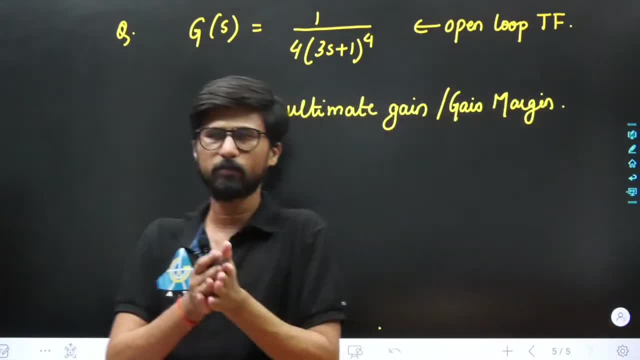 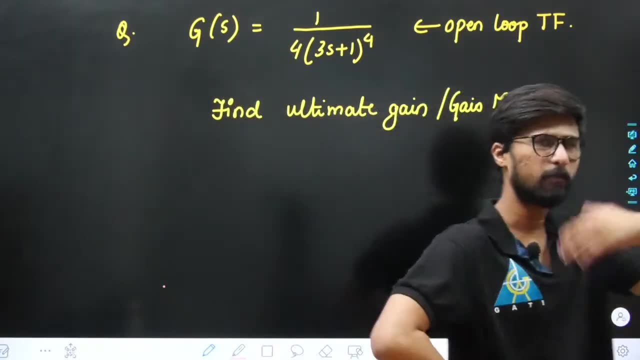 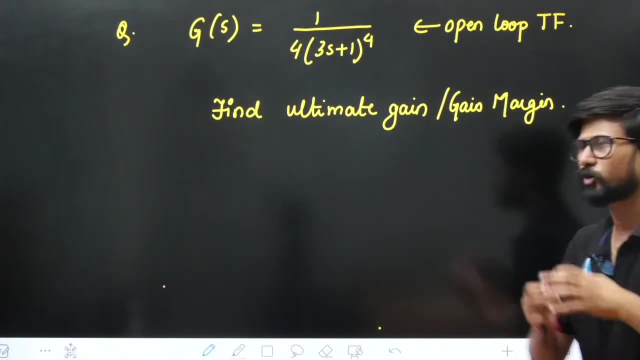 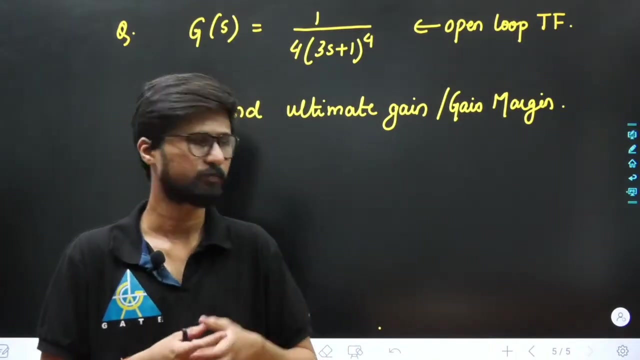 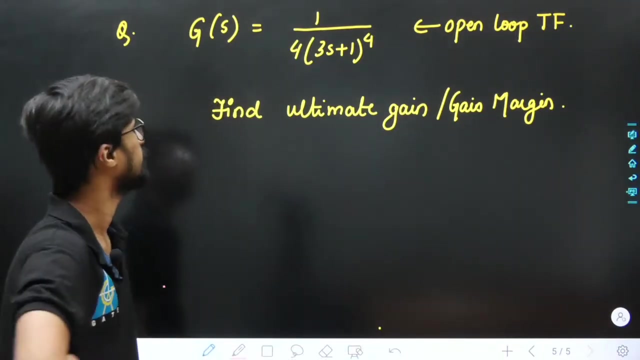 class is going on, so ma'am will complete the mass transfer once. when ma'am will be complete, after that I will start and after that I will take the classes, Because now ma'am is teaching it and I will teach it. I don't mind teaching one thing in two places. 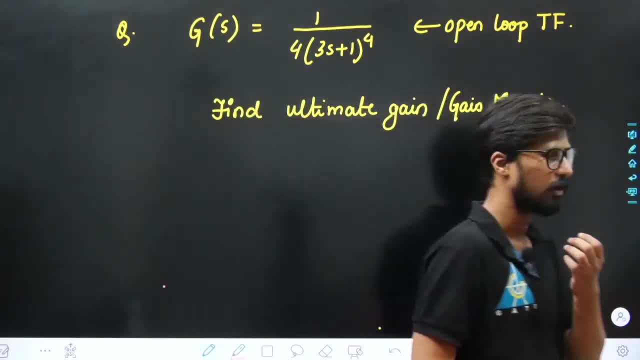 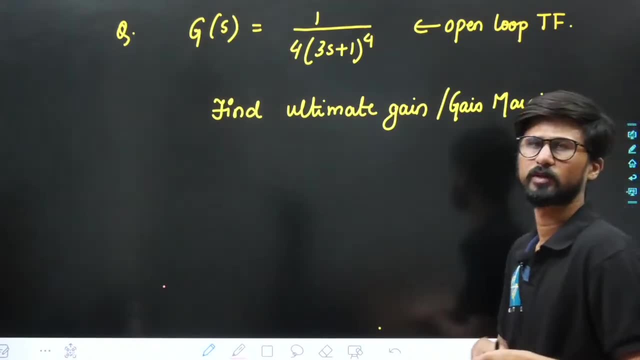 Let's do it. control equation is easy In control, So you should know what to do, which formula to apply at which place, and that's it. You don't have to think much about the brain type, you have to think about the thermo. 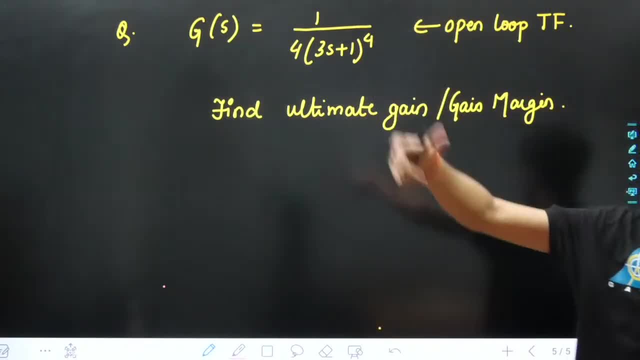 That is, if the idea is a bathe process, then what will have to be thought separately for it? The graph has been given. You have to think about CRE. You have to think about the concept in the mass transfer. There is nothing in this. 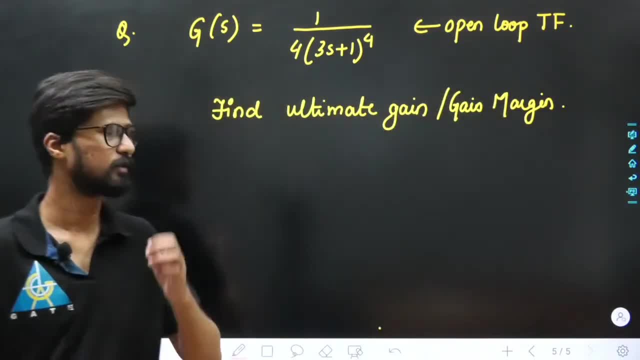 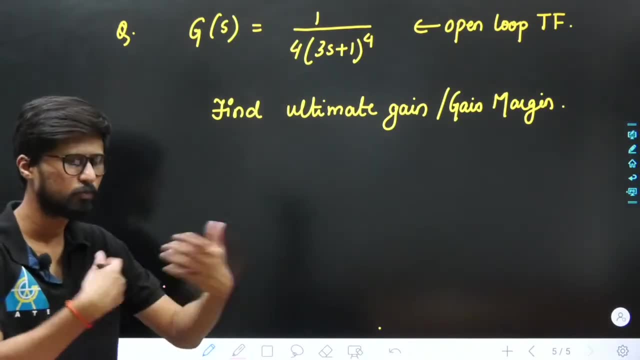 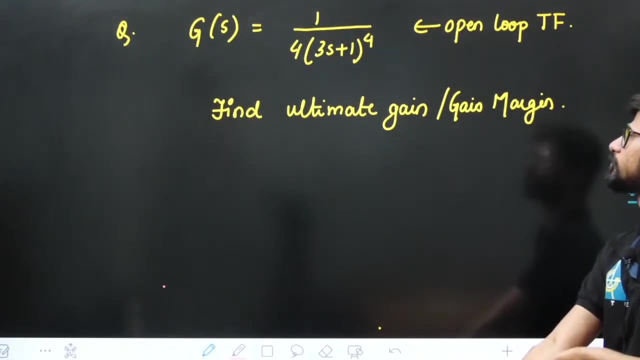 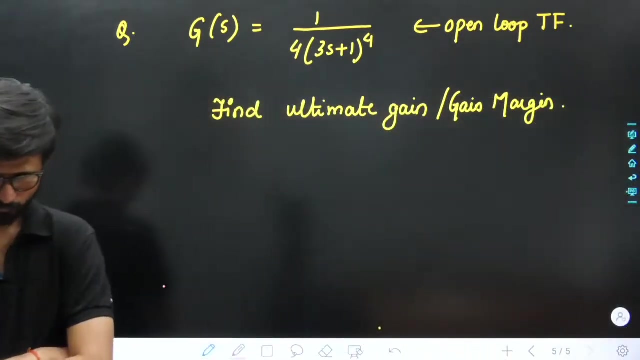 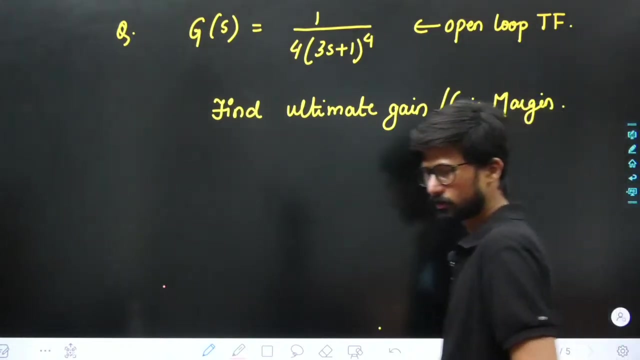 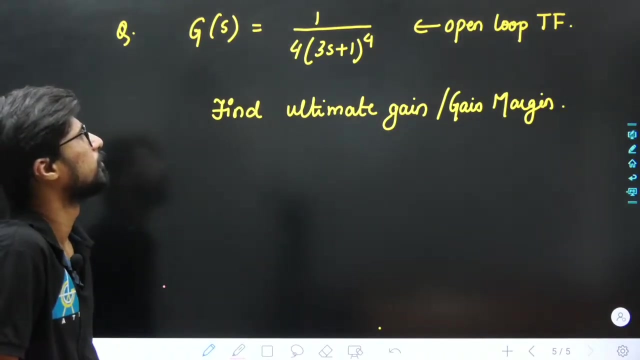 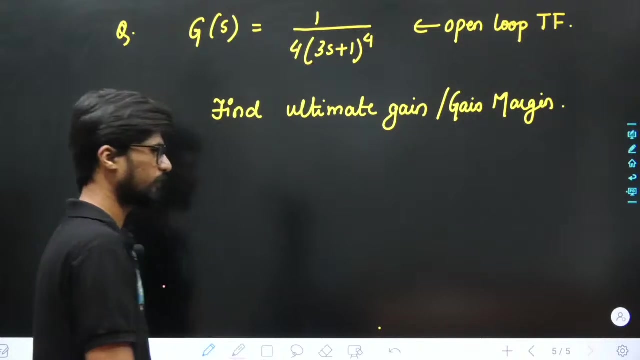 There are two or four things, apply directly and answer, Okay, Two or four things. he will ask the same thing again and again. Come on, tell me the answer. I have done it Correct. It is taking so much time. 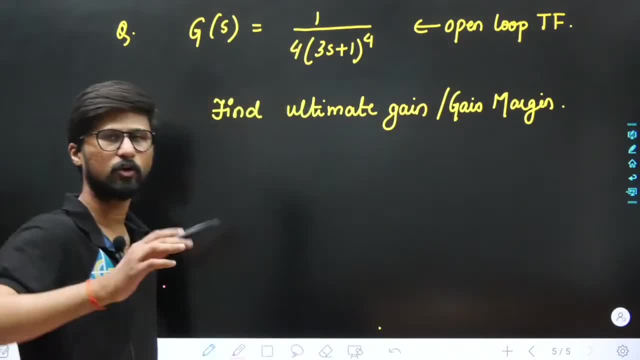 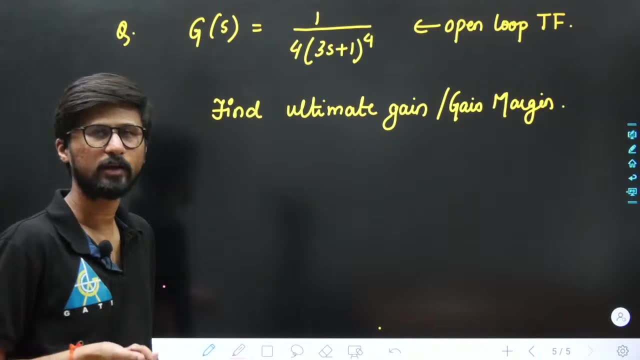 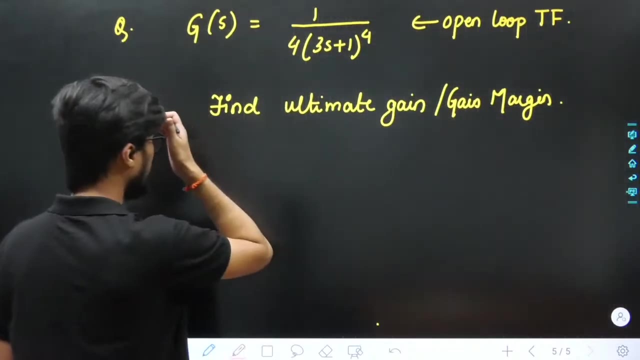 What did you ask? Ultimate gain gain margin. What is the gain margin? AR, Correct, Sorry, 1 by AR at omega CO, Correct? So let's remove omega CO first. Okay, It is first order. You can write it by breaking it in three first order systems. 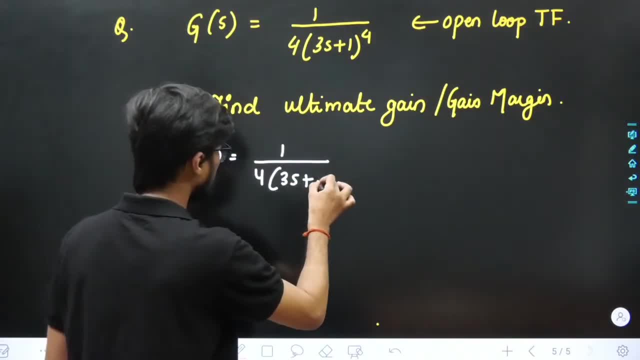 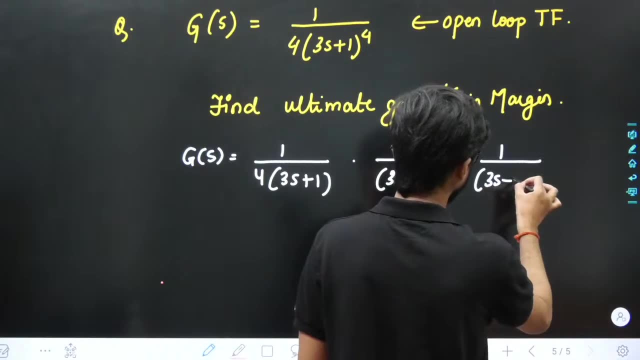 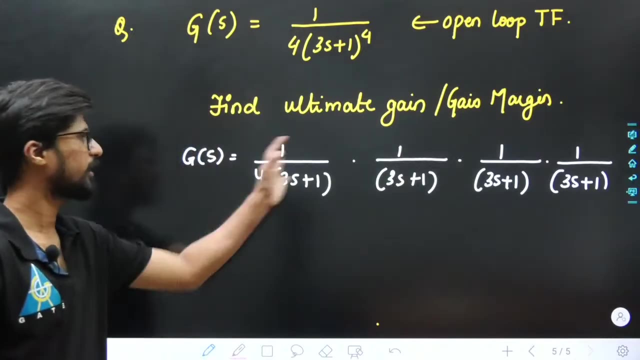 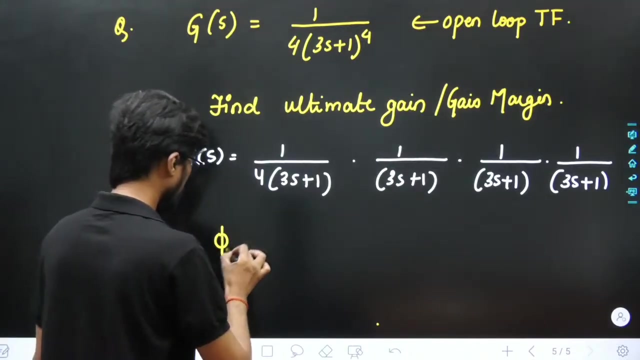 You write it by breaking it. Four first order systems- sorry, It is to the power 4,, isn't it? You have taken 4 first order systems. will write it in four, All writing 4, then 109 times. 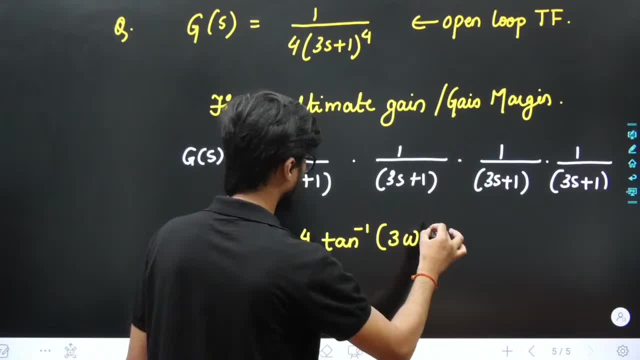 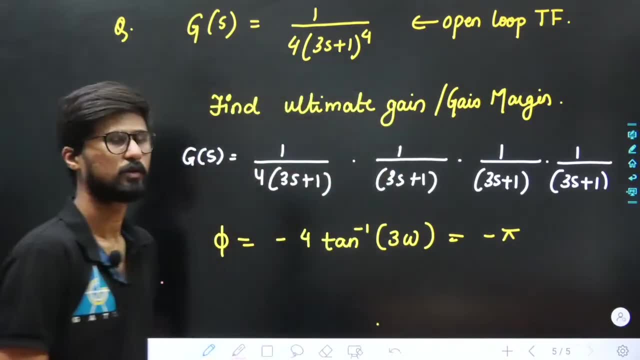 At that window you will come to the cube. you will write 5.. Then you write 5.. 5 is minus 4 times tan inverse omega, And to this you have to equate it by minus 5.. So if you equate it by minus 5,. 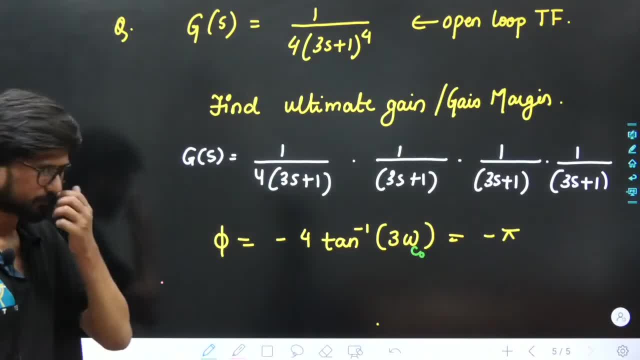 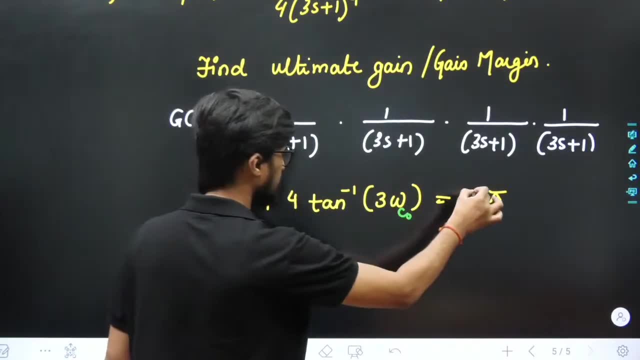 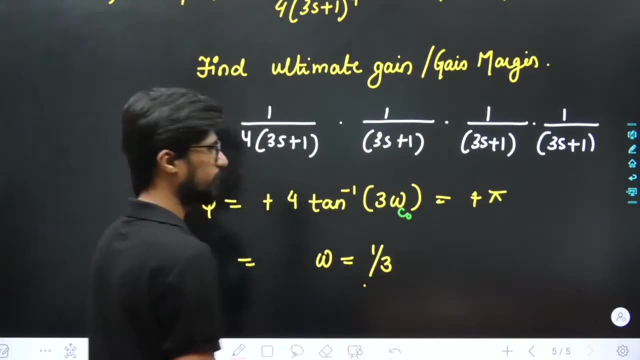 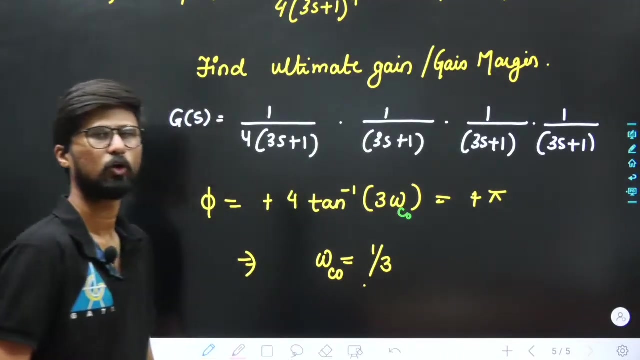 it will be omega CO. ok, Yes, the figure Is of 2 degrees, Absolutely. So this is acave. So this will be minus A, minus cancel. omega will be 1 by 3, omega is 1 by 3, omega CO. 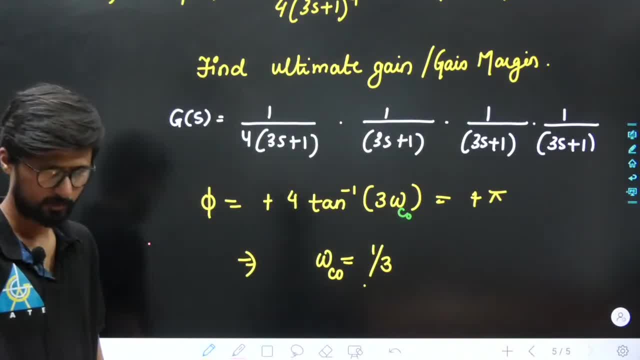 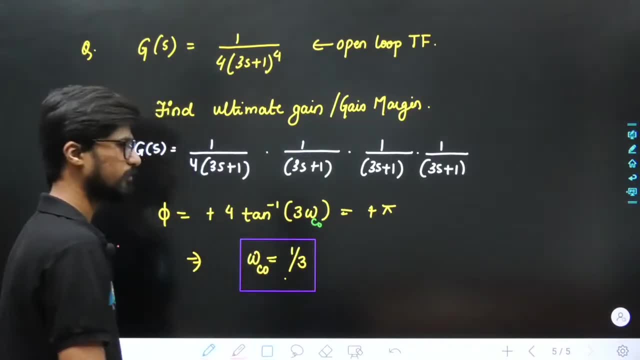 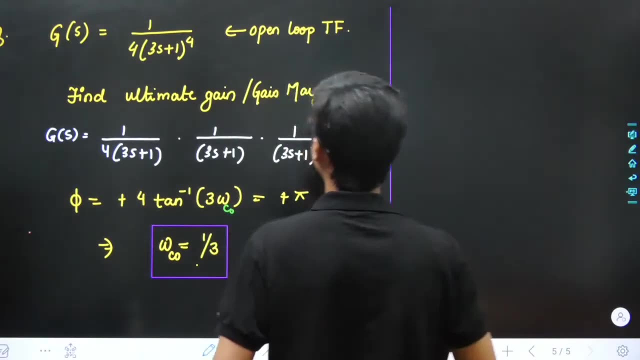 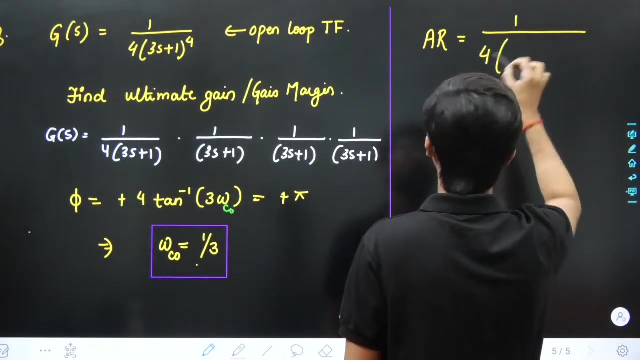 omega CO is 1 by 3,. this is your omega CO. Now, when omega has come, omega has come, what will be AR? AR is 1 by 4, what happens? Omega square, tau square, so 9 omega square. 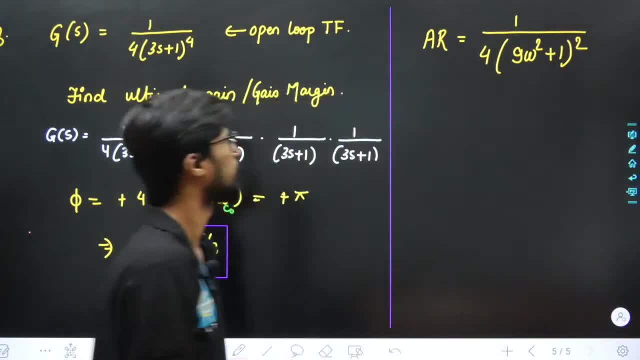 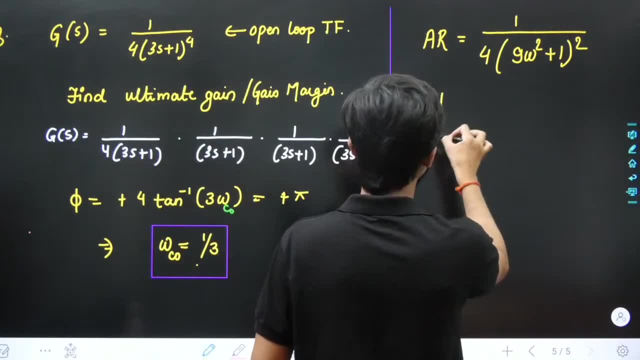 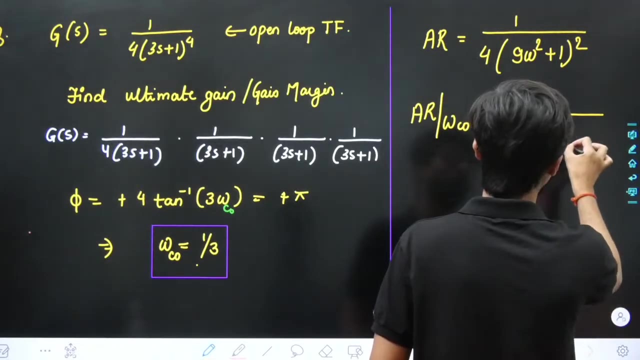 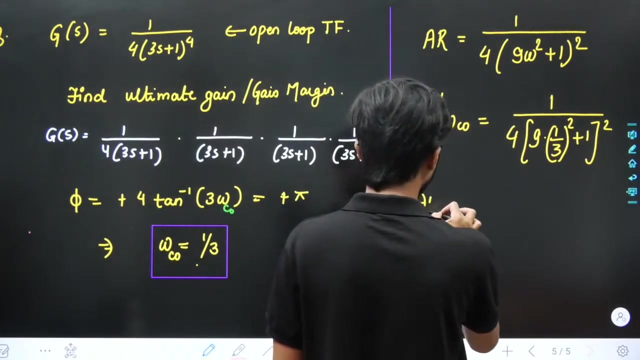 plus 1 square. now I am doing directly. now I have told you to remove AR, AR at omega CO. this will be 1 by 4, 9 into 1 by 3 square plus 1 square. So AR at omega CO will be how much? 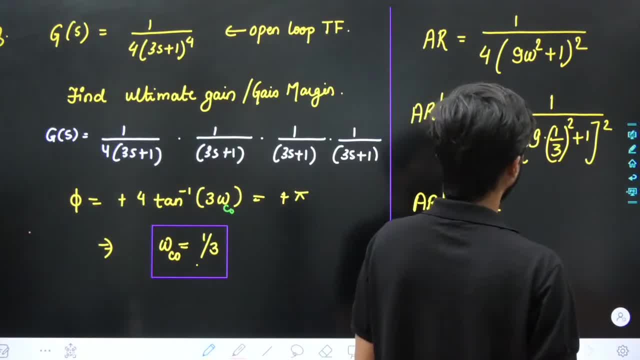 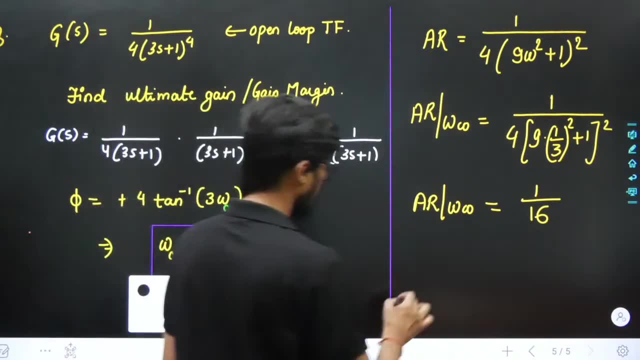 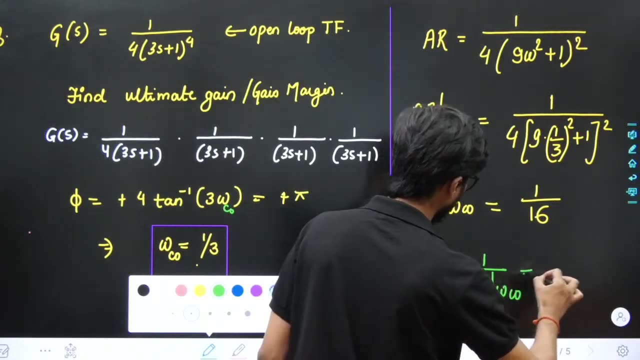 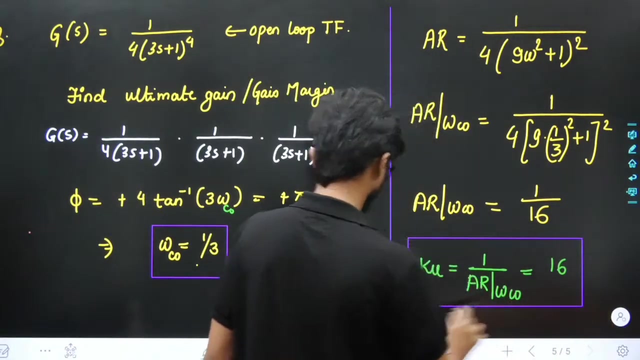 1 by 4.. 1 by 4.. 1 by 4,, 1 by 16, which means your Ku will be 1 by AR at omega CO. this will be 16.. This is your final answer. This is your final answer. 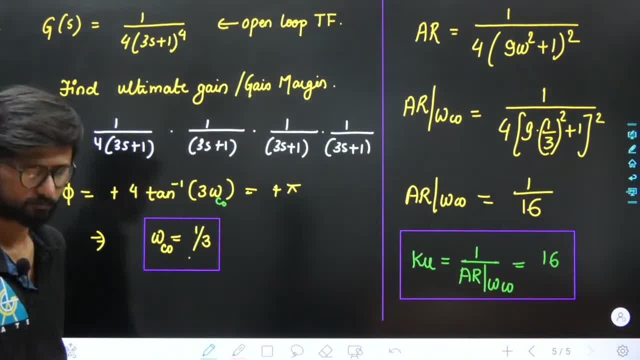 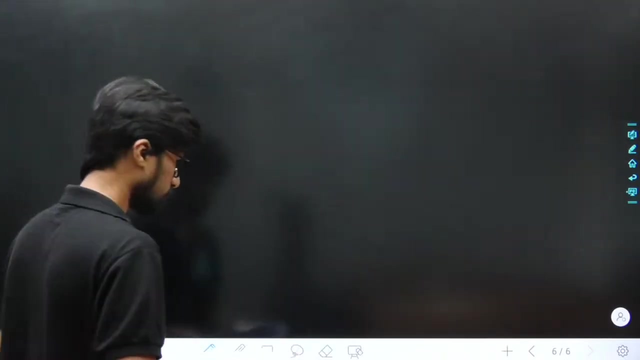 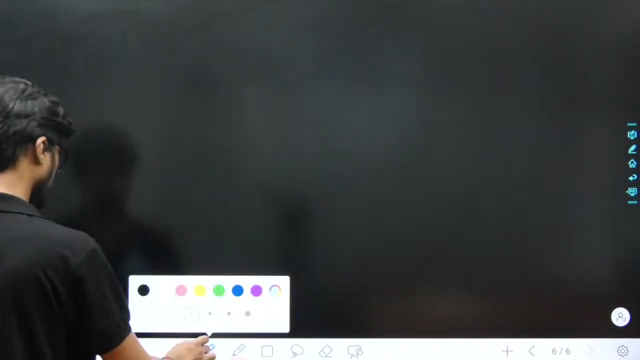 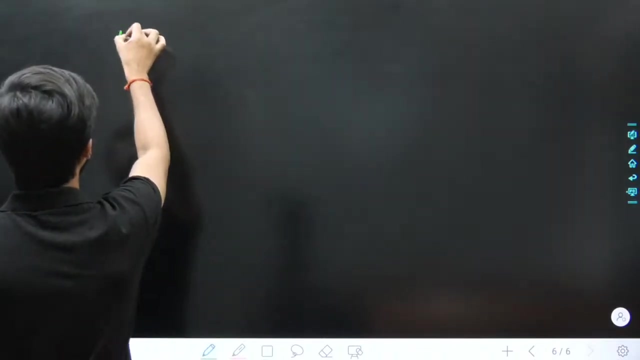 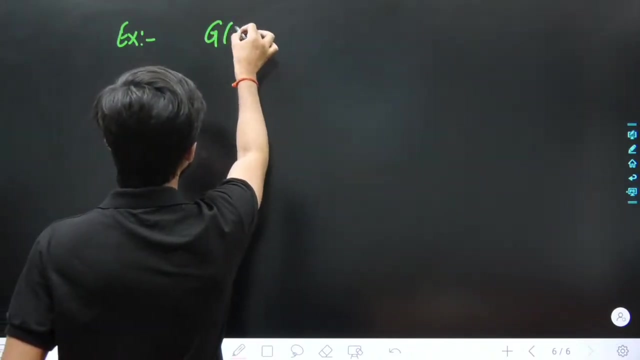 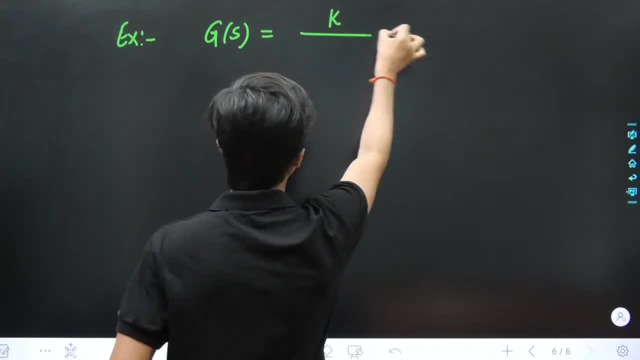 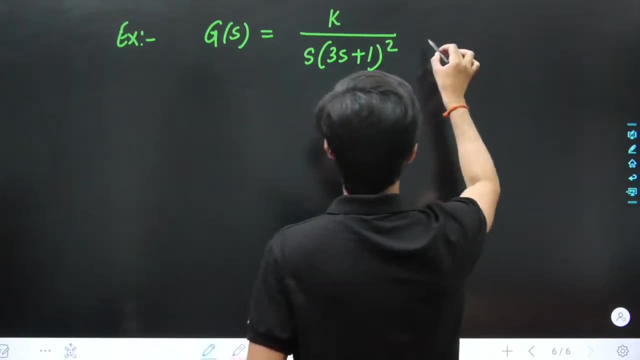 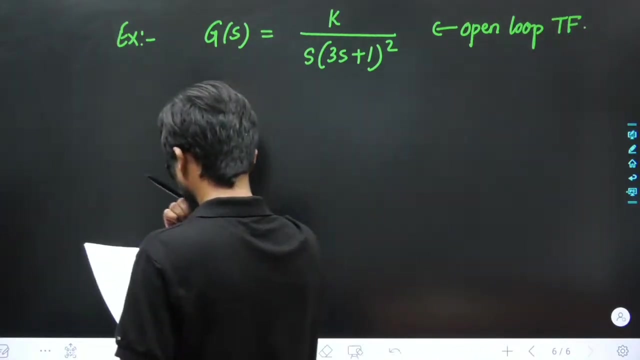 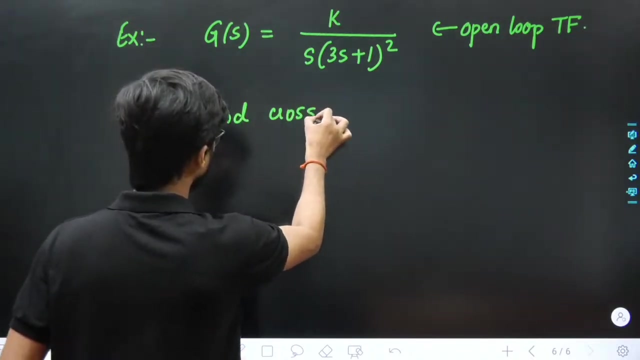 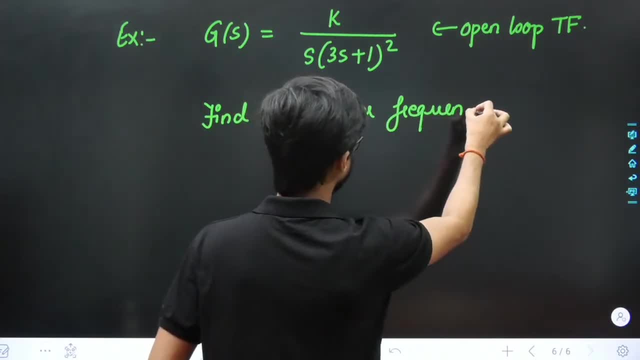 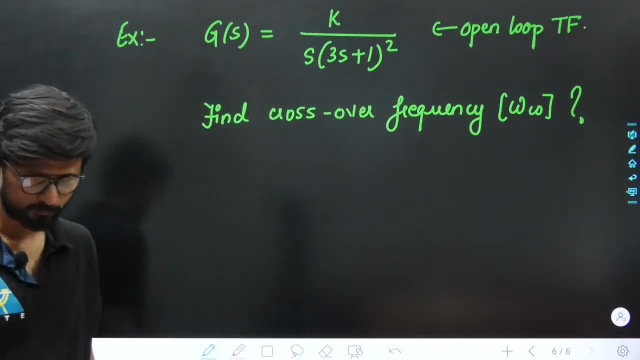 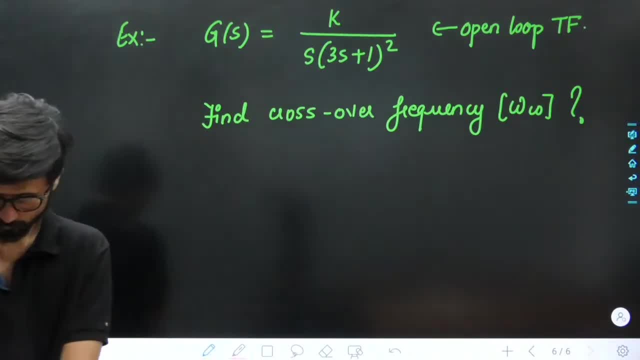 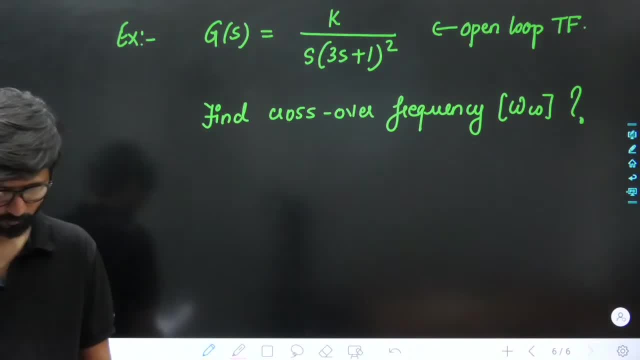 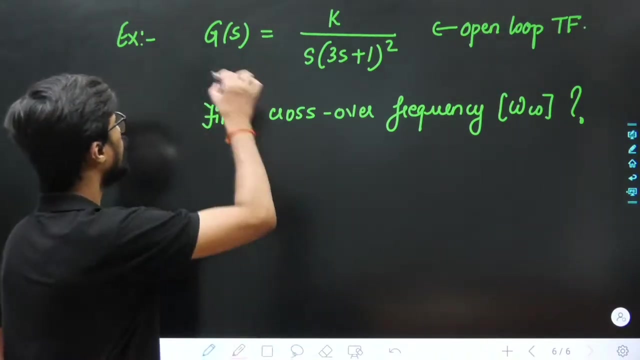 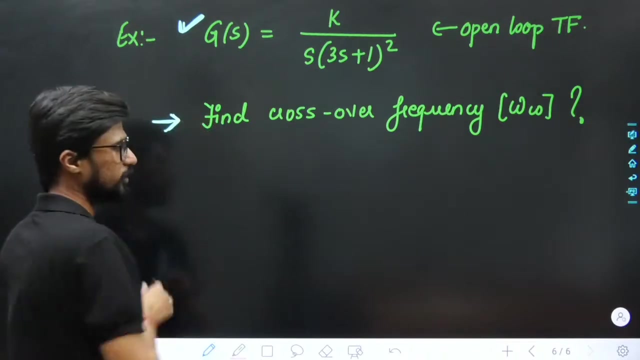 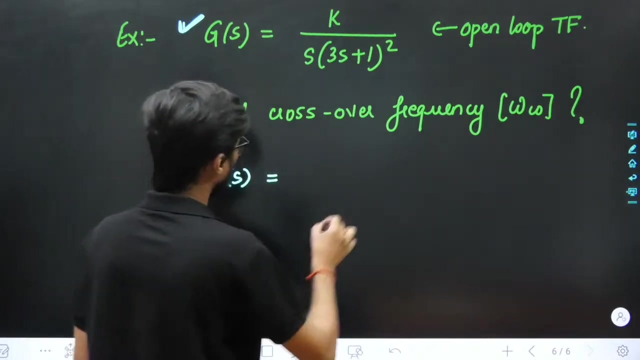 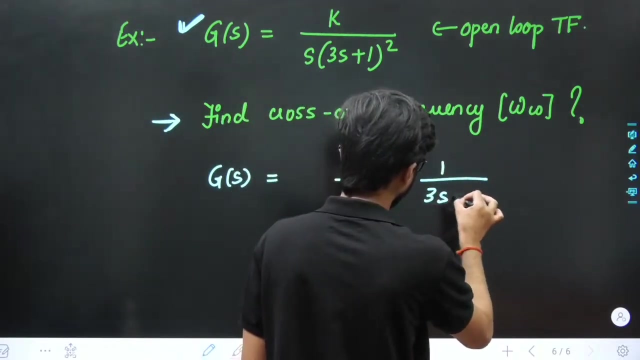 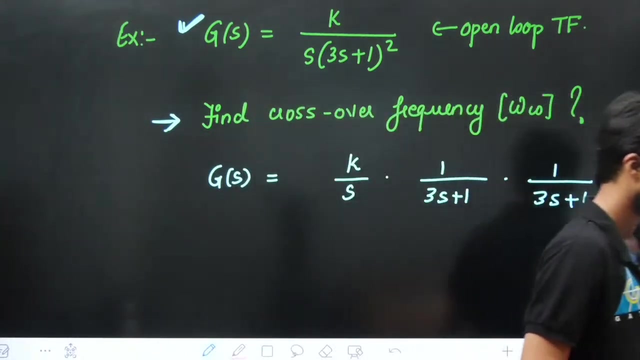 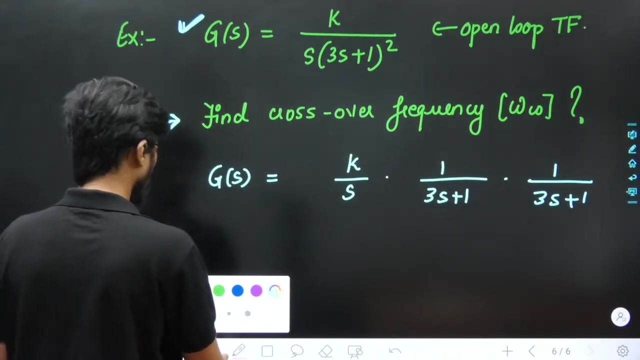 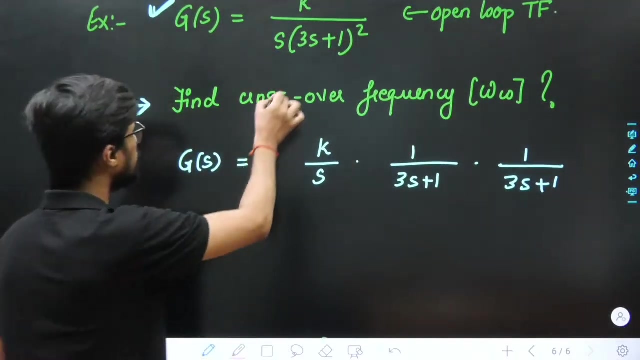 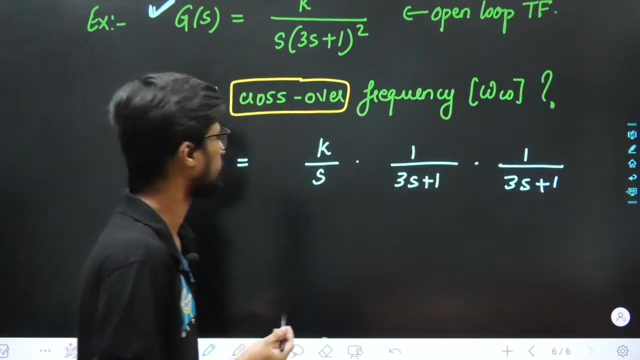 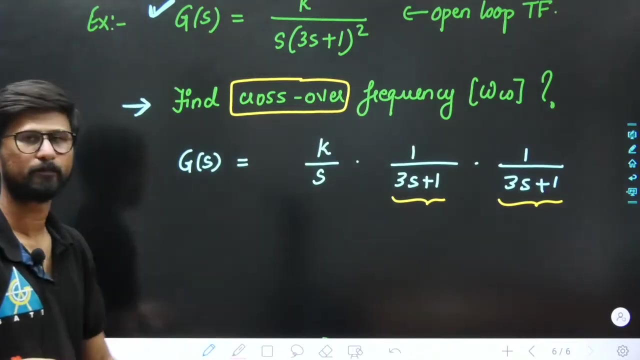 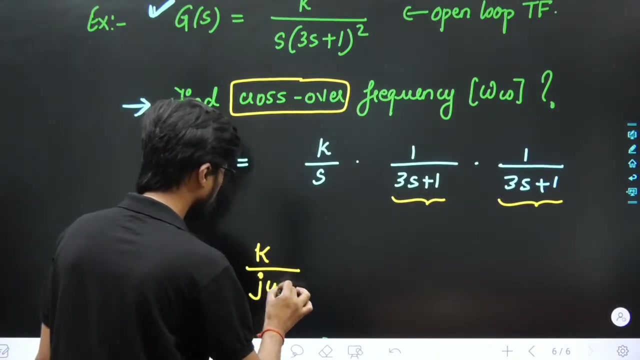 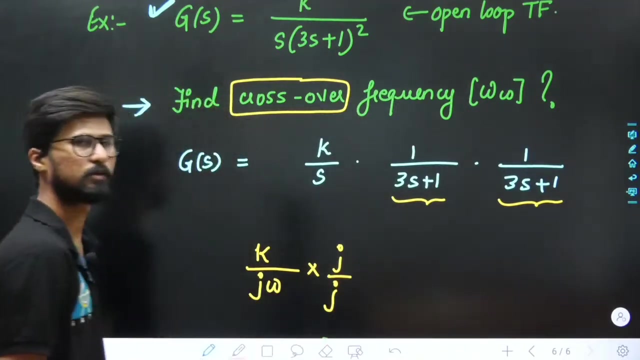 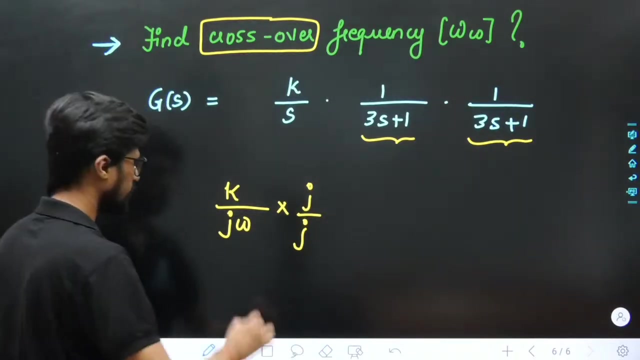 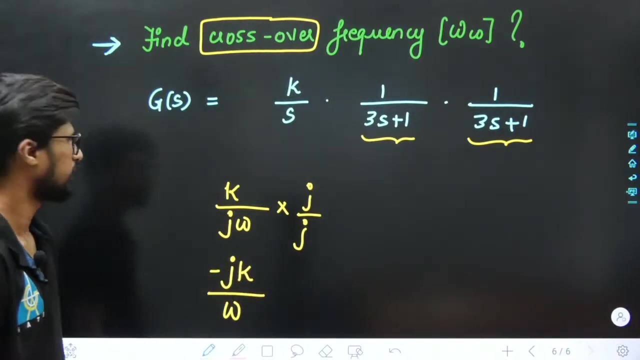 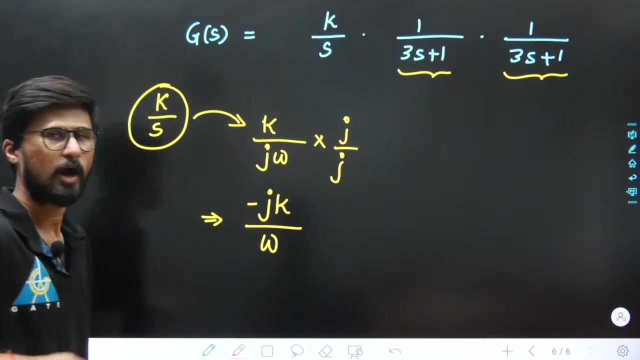 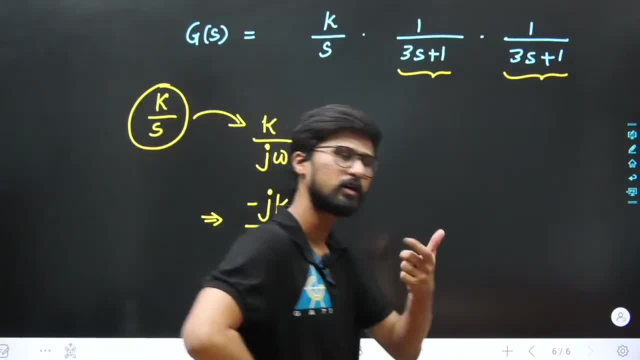 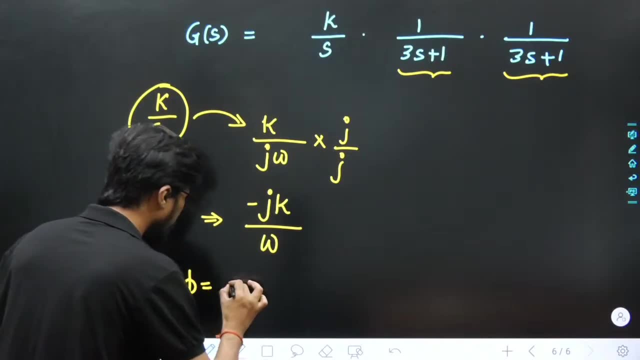 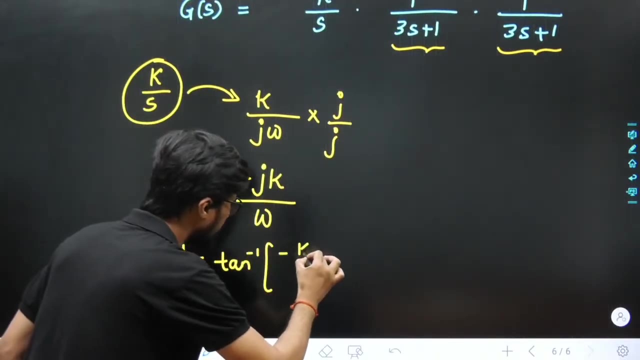 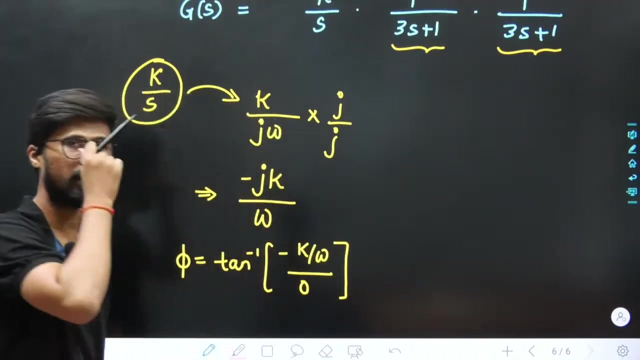 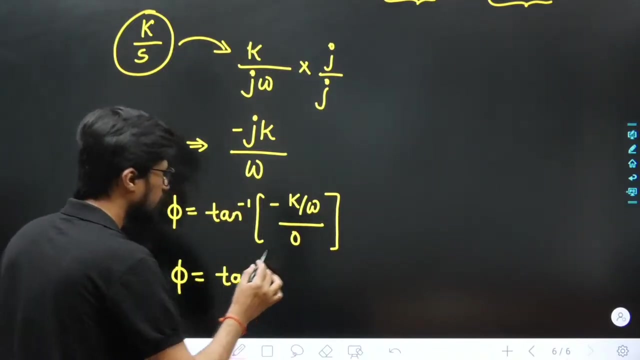 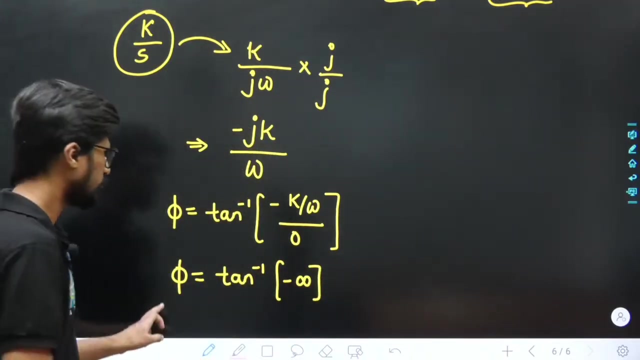 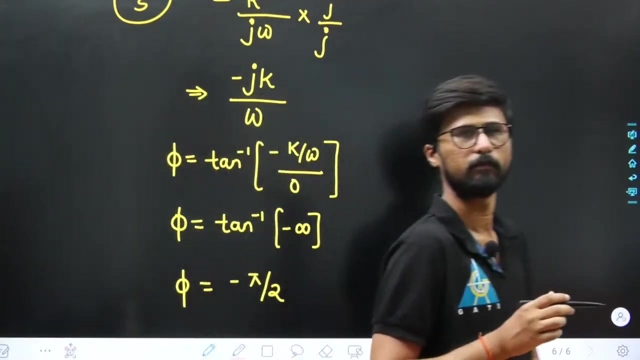 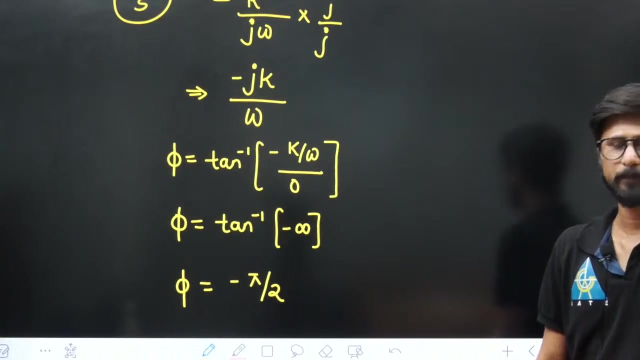 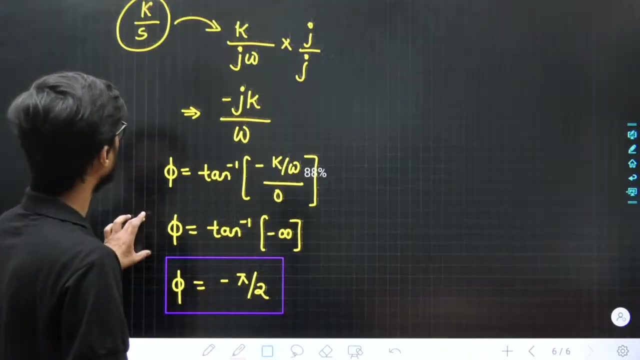 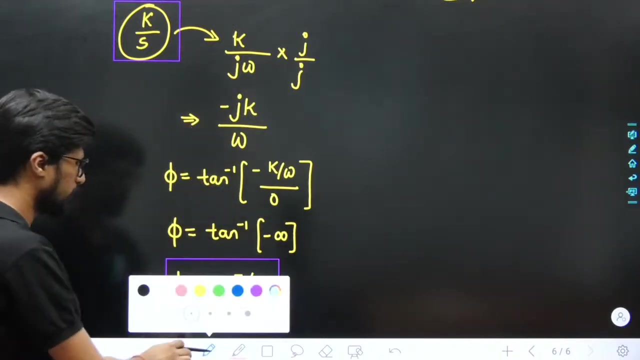 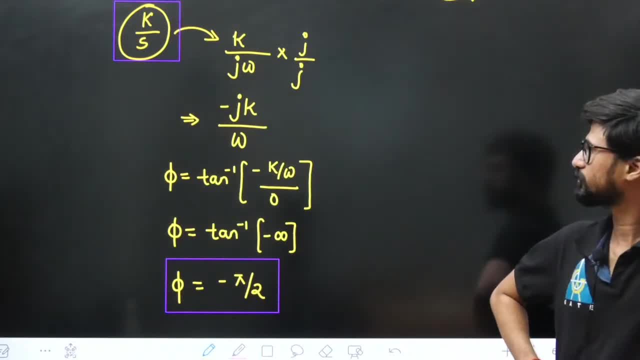 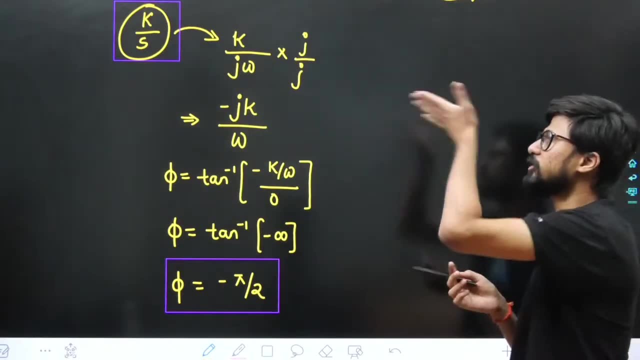 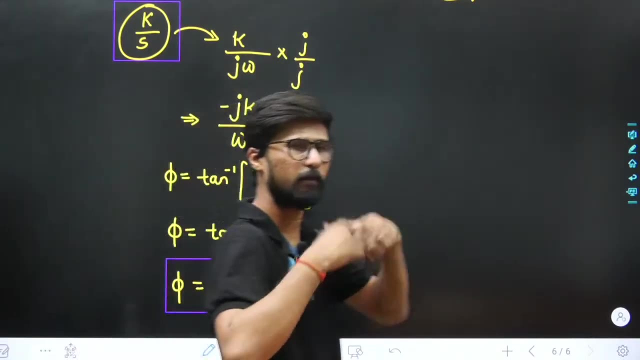 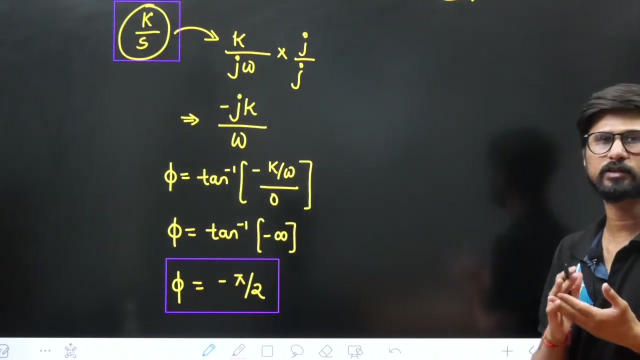 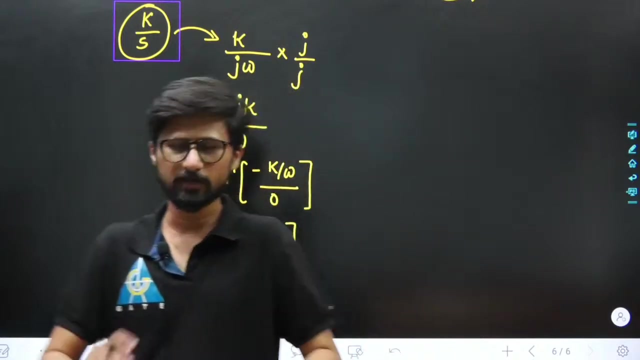 If you want to keep, s is equal to j omega. you have to follow your steps now. don't be hasty. hasty means you are calculating in your mind that here is k by s. then how to get it out? what to do? infinity will come. no think about it. s is equal to j omega. you know the method. follow your method. don't go away from the method. 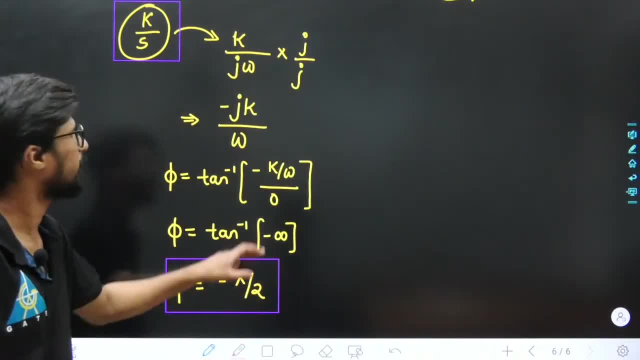 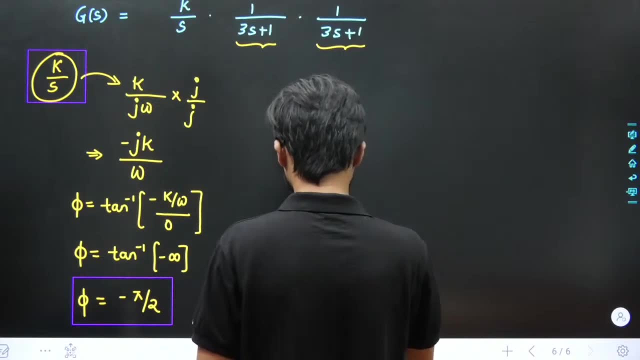 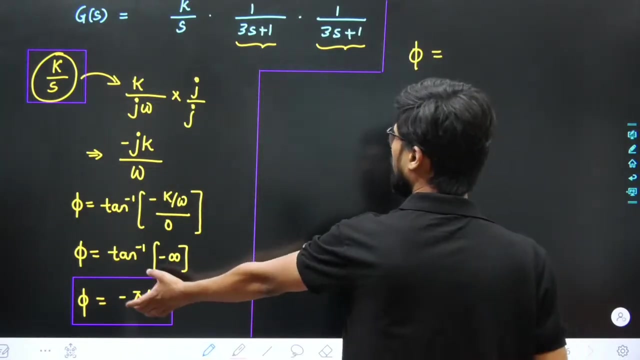 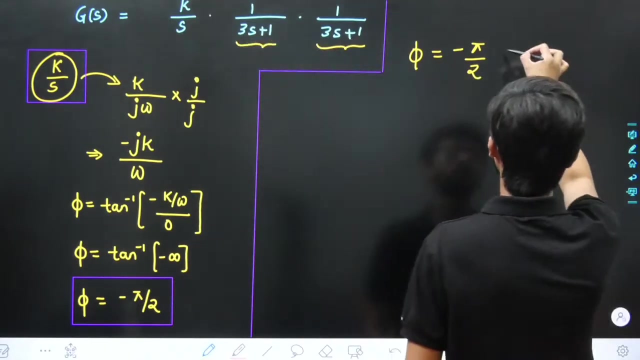 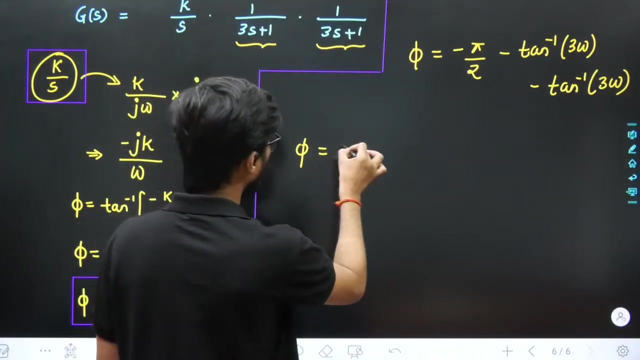 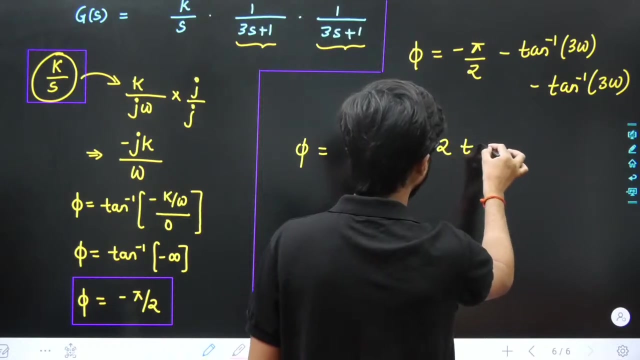 Okay, so its phi is minus pi by 2, so what was our problem? our problem was this: so if I talk about phi overall, then how will I write phi overall? phi of this function is minus pi by 2, both are first order system. what they have- tan inverse omega, tau, tau is 3, its also minus tan inverse 3 omega. okay, if I solve it further, then phi will be minus pi by 2, minus 2 tan inverse 3 omega. okay. 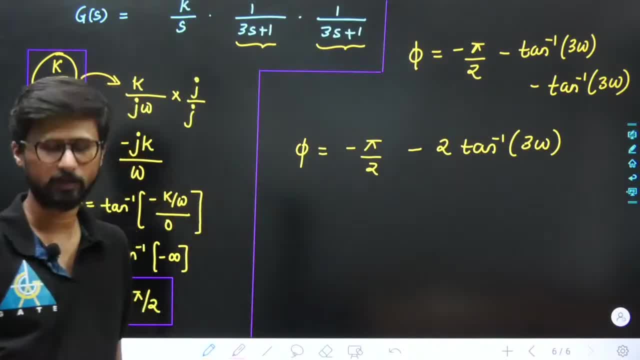 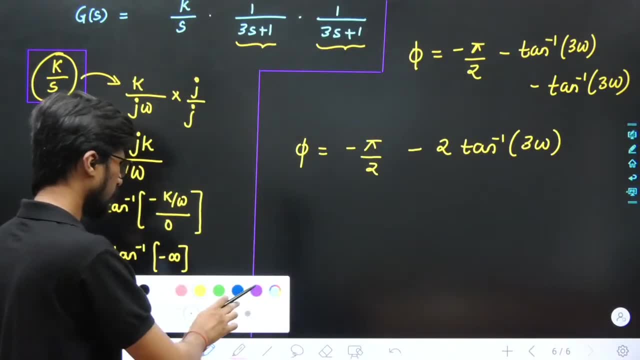 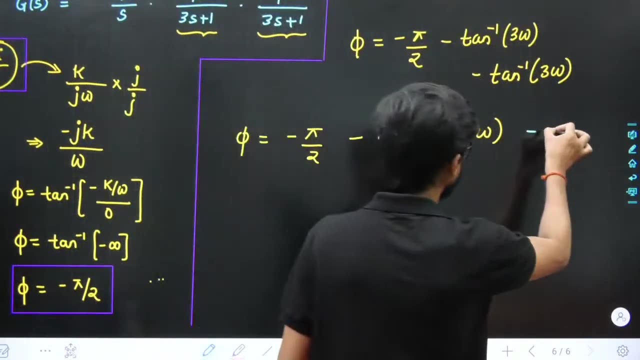 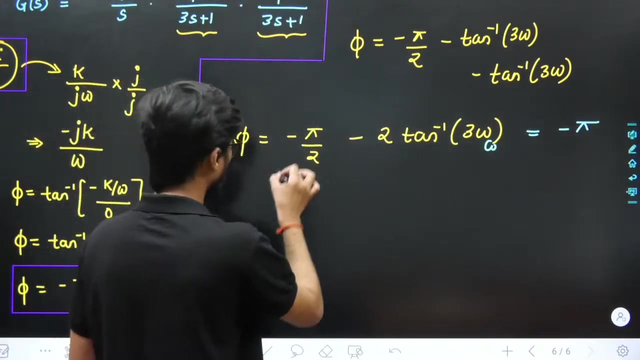 okay, Okay. So this is my final expression. this is my final expression. okay, is it clear now what to get out? crossover frequency, for which I will substitute this: if it is minus pi, then this will be my omega c. okay, let us solve it. so minus is cancelled from all the places. pi minus pi by 2 is 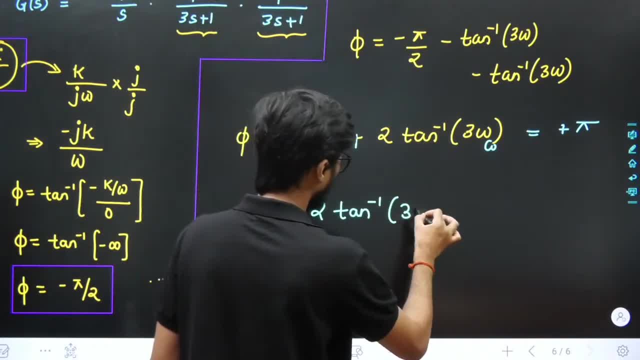 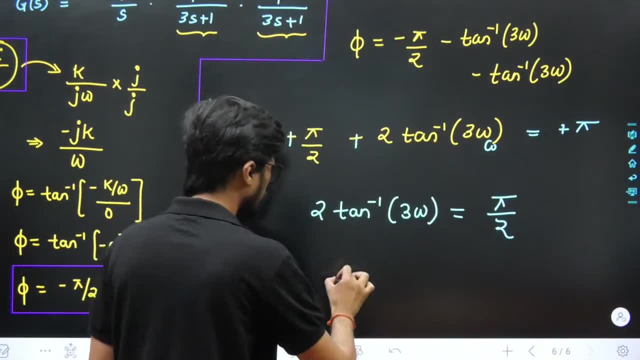 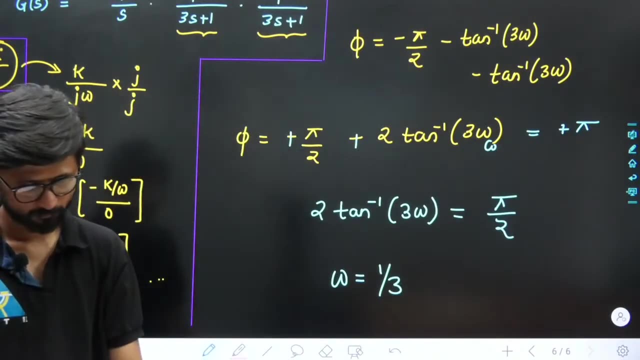 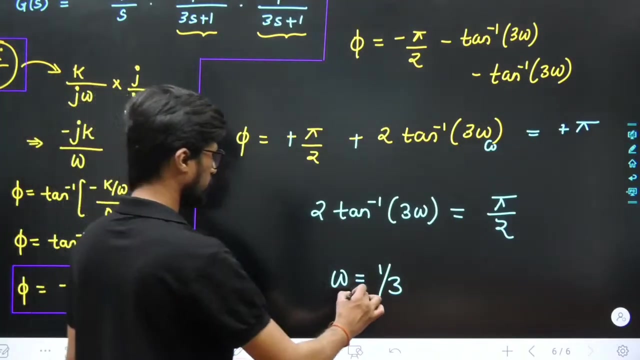 okay, Pi minus pi by 2 is pi by 2, solve it. so omega will be 1 by 3,. omega will be 1 by 3, okay, omega c o this will be 1 by 3.. 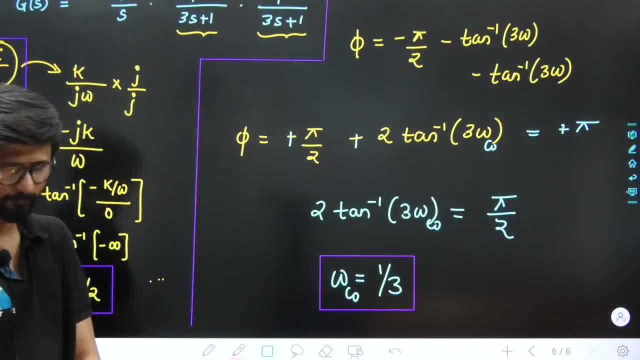 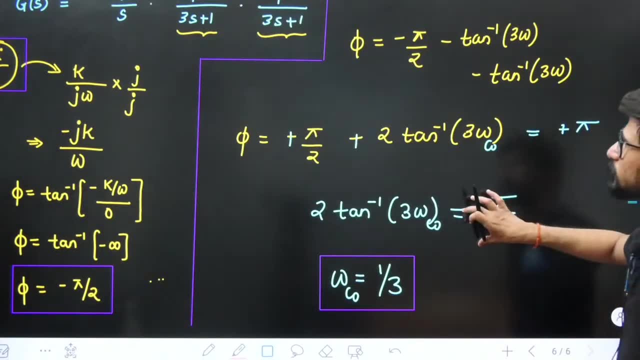 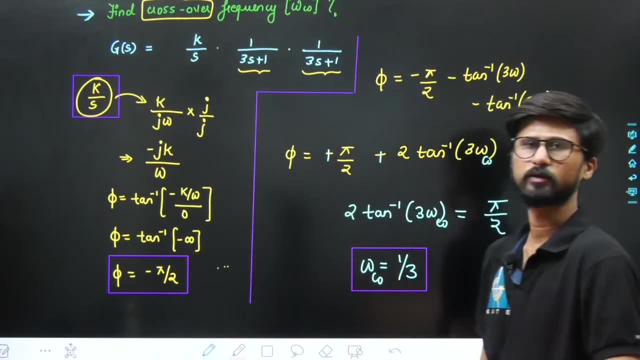 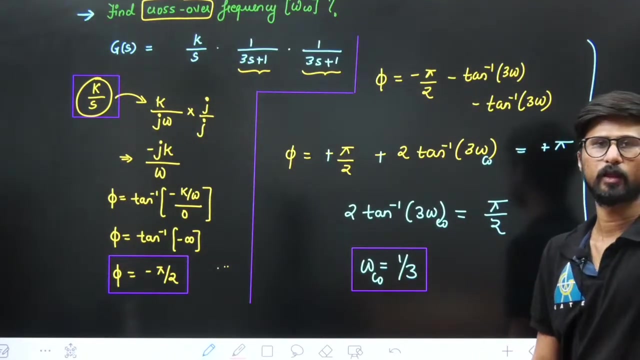 Okay, Yes, 1 by 3 is correct. Rishabh, 1 by 3 is correct. just follow the method. whatever you tell, you don't have to deflect at all. you don't have to go far. just look at the method. look at the method and solve it. there is nothing else in it. the calculation is on you. 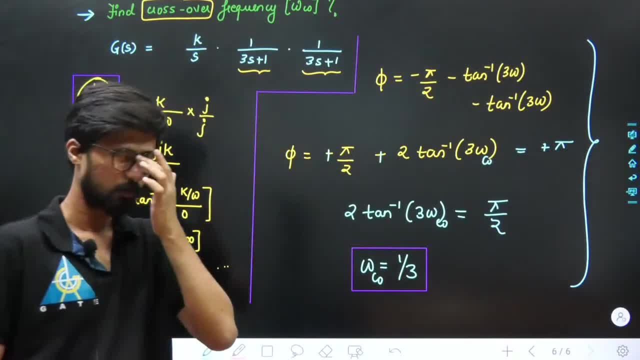 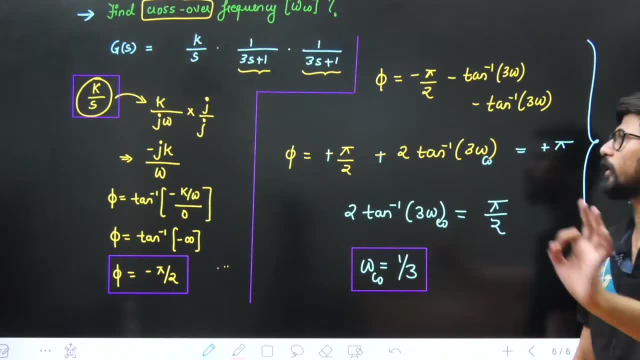 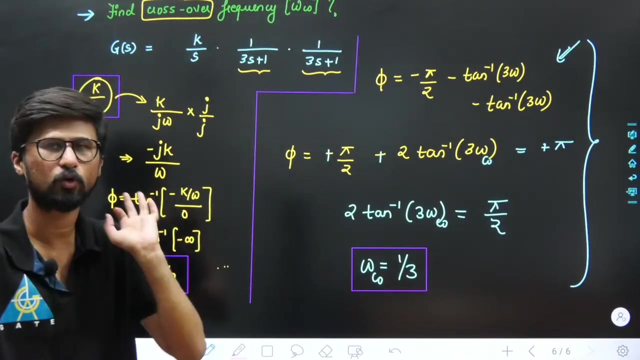 Calculation is on you. yes, calculation is on you. take care of yourself calculation mistakes. if there will be calculation mistakes, there is no chance of a mistake in the concept. there is no chance of a mistake in the concept in this part, in the control, in the process control. you just have to take care of the calculation a little bit. 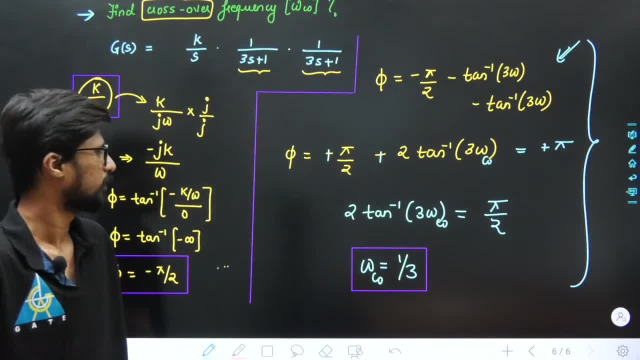 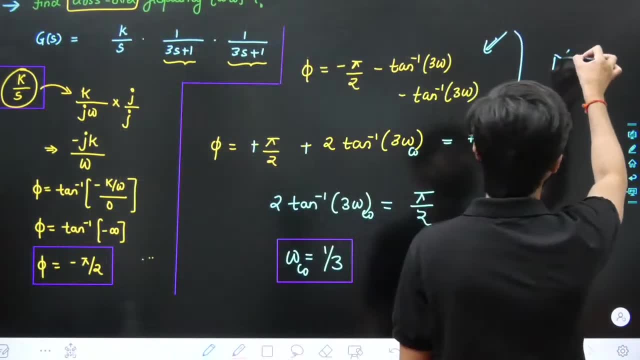 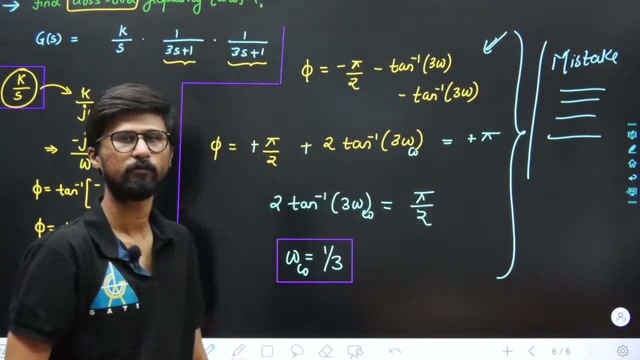 Ok, Is this thing clear? Ok, So, whatever mistake you make, write it down here what mistake I have made, mistake that I have done. that's it. it will never happen. after doing it for 2 months, it will stop. 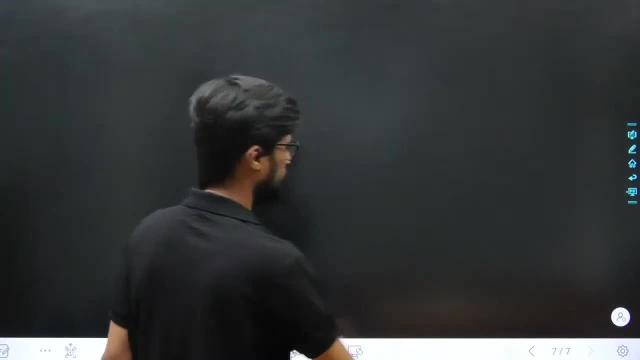 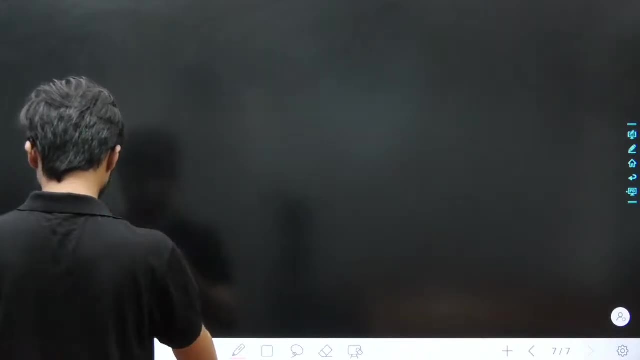 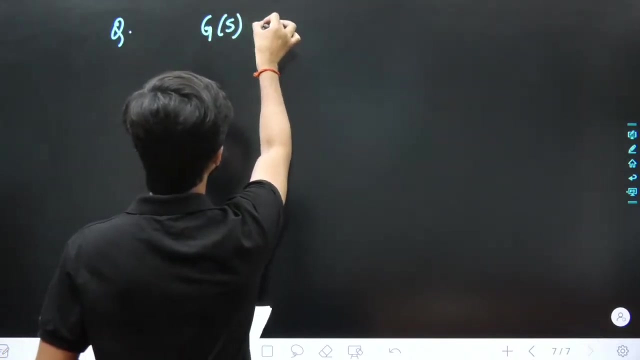 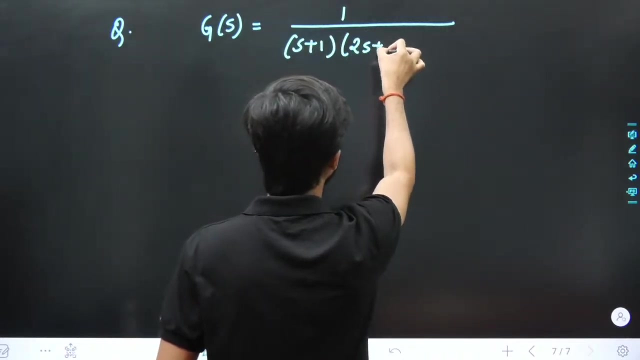 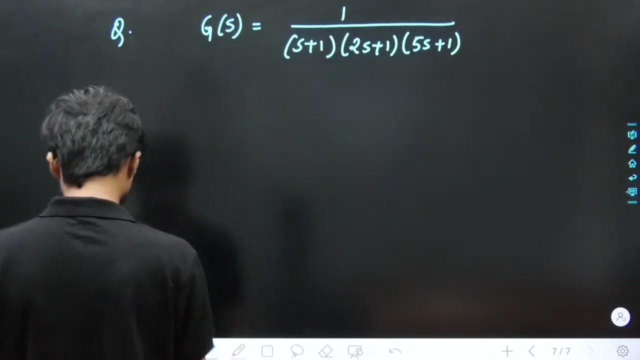 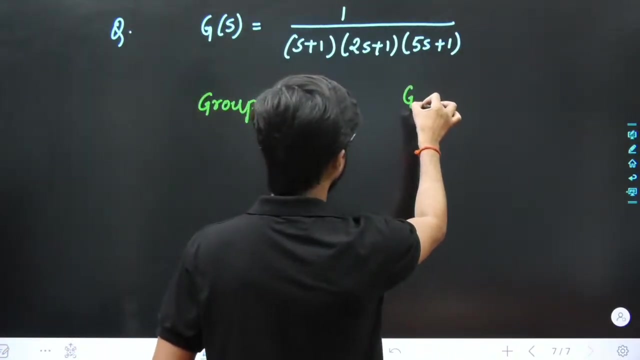 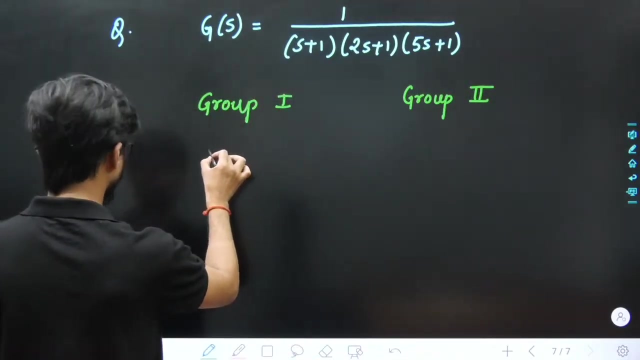 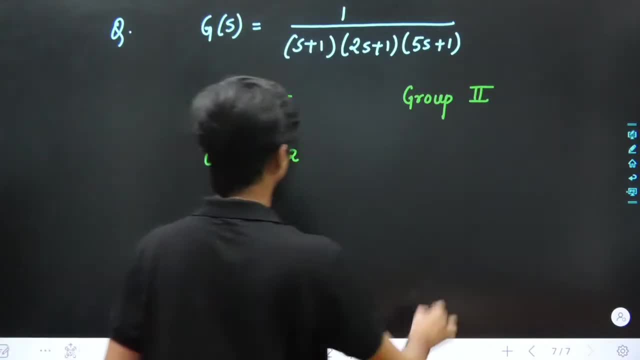 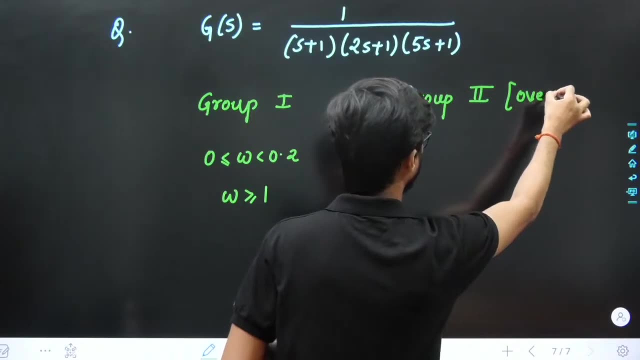 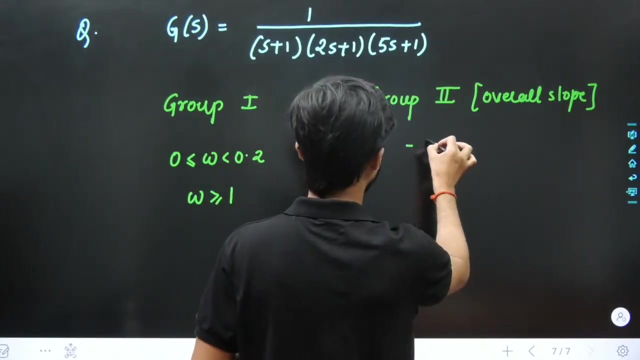 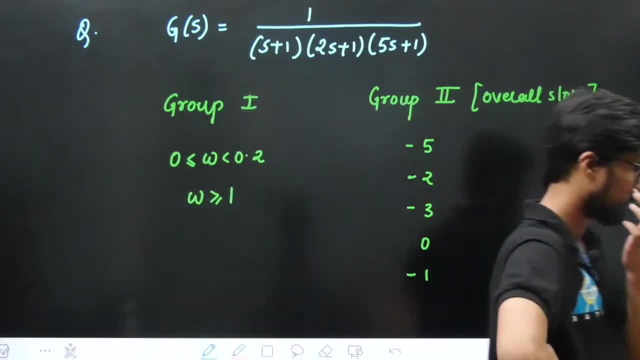 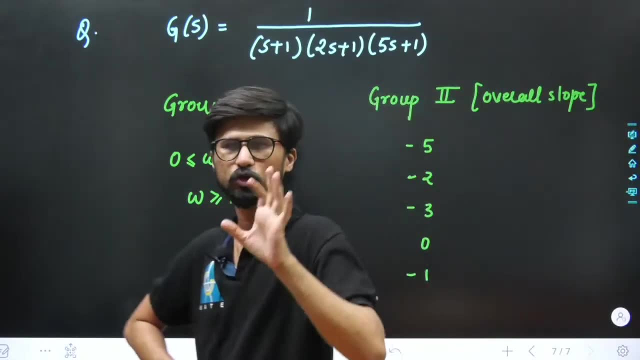 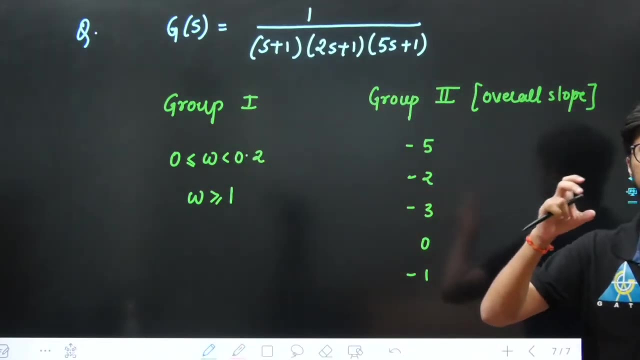 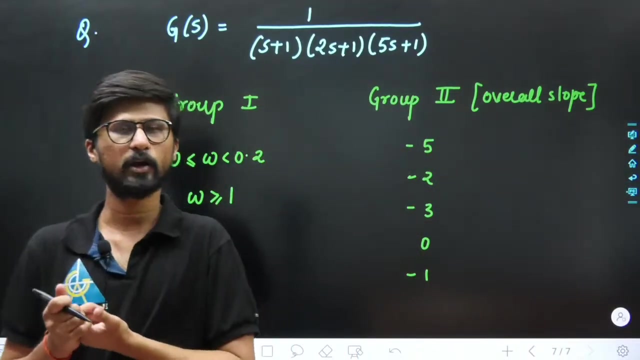 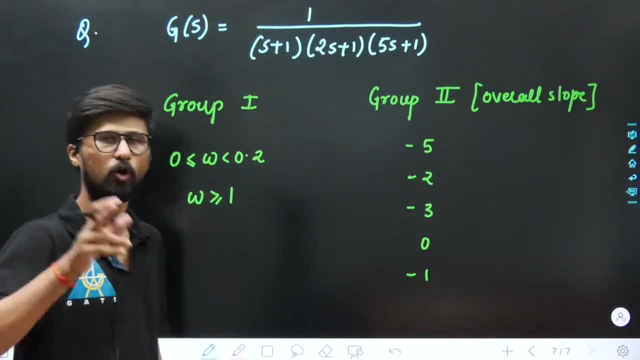 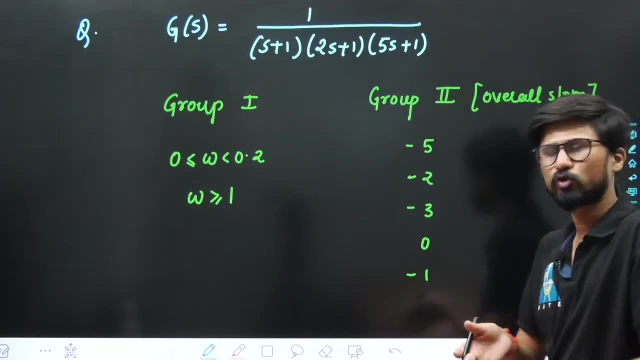 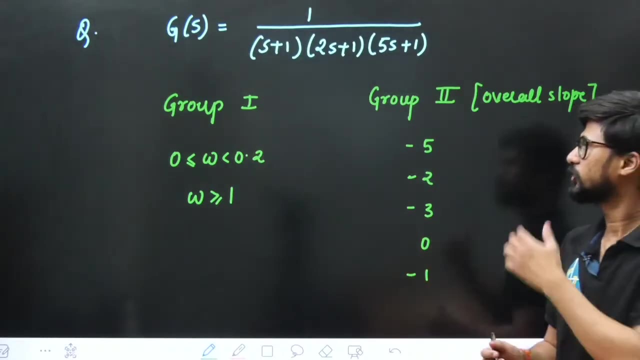 in the class. and second thing, the list, like temperature. what instrument is used? what is the concentration will be given in the list, what will be done? that is something to remember. ok, you have to match. this is the range of omega. ok, and here the overall slope is given. 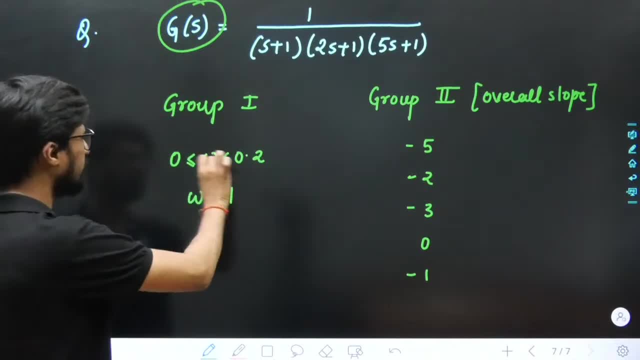 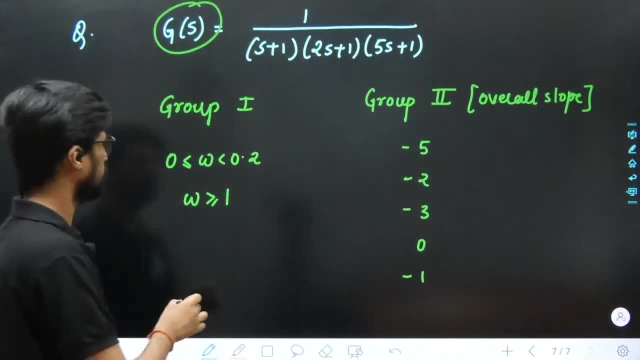 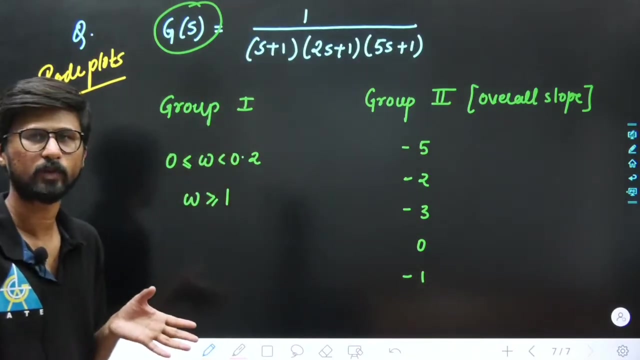 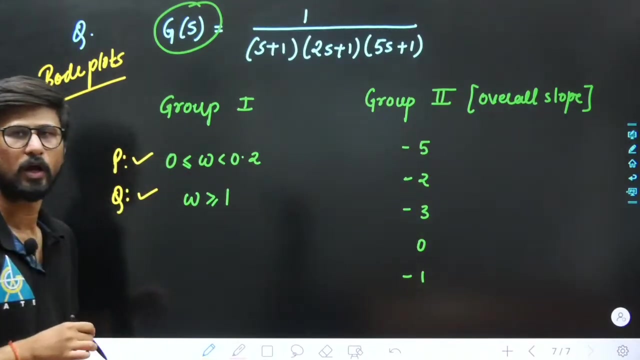 in this transfer function, so you have to match in which range. ok, ok, do this question. question related to bode plot. do this question, do this question. you are given a transfer function, ok, and range is given. this is p, this is q. you have to tell that overall slope. 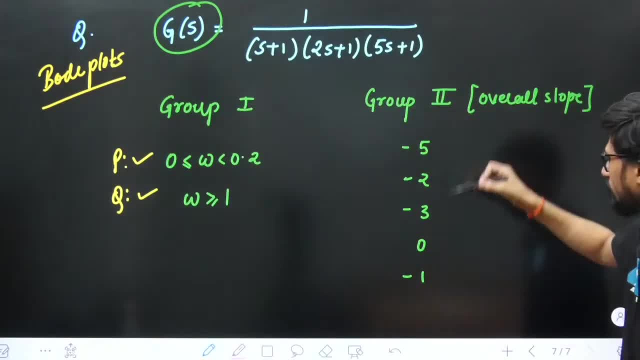 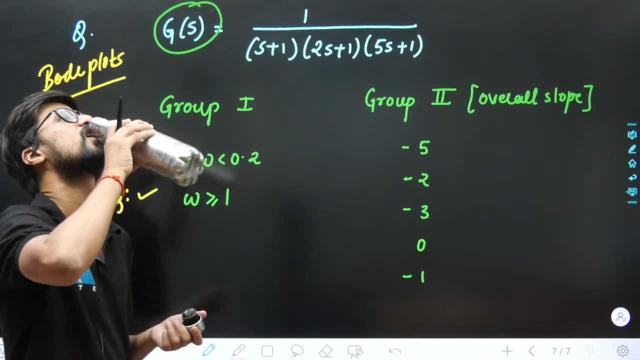 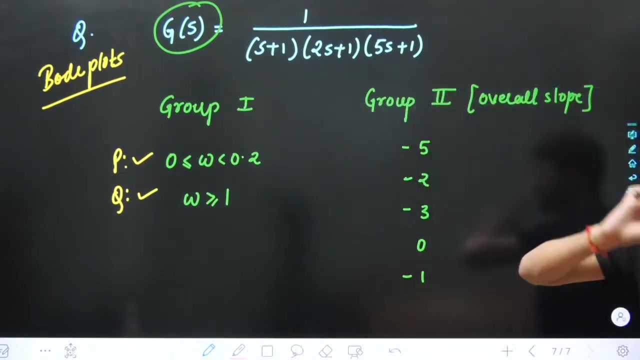 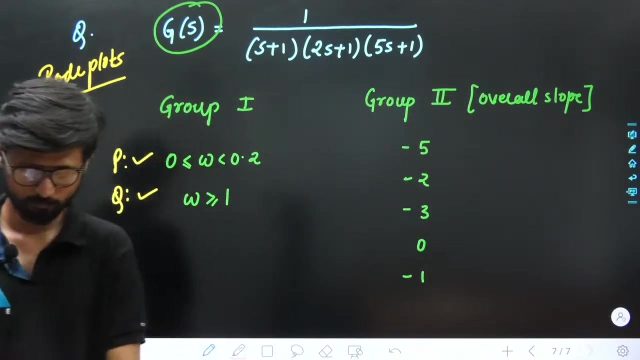 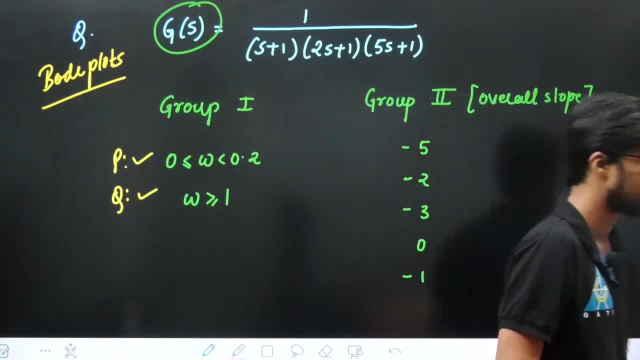 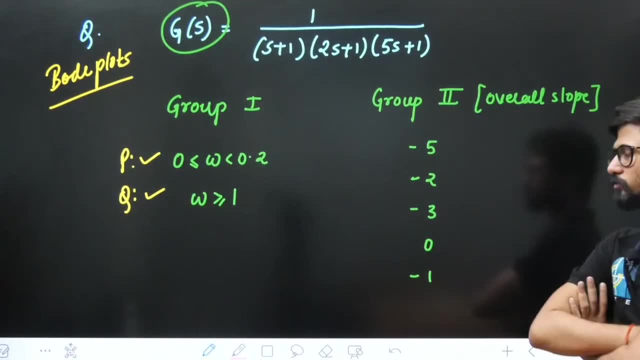 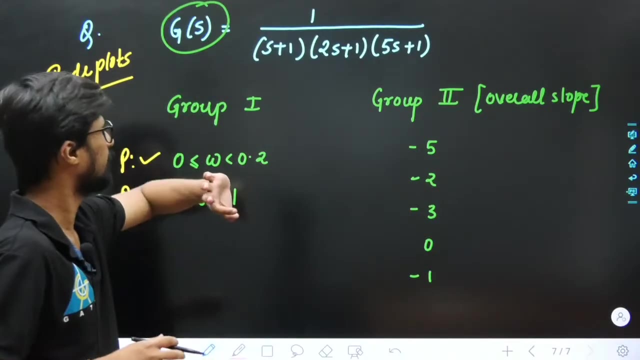 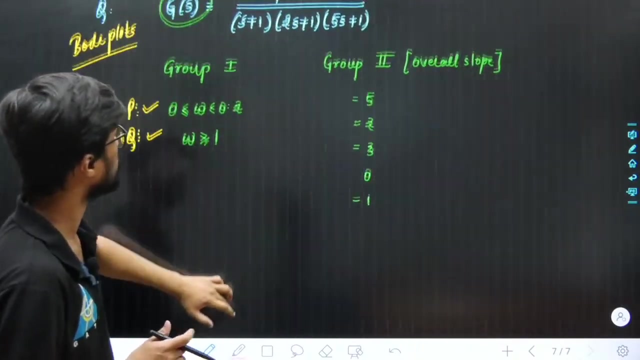 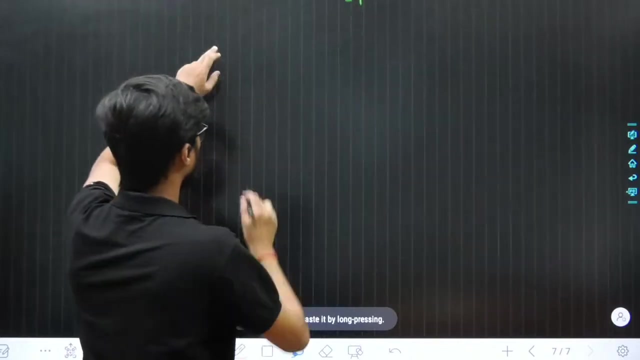 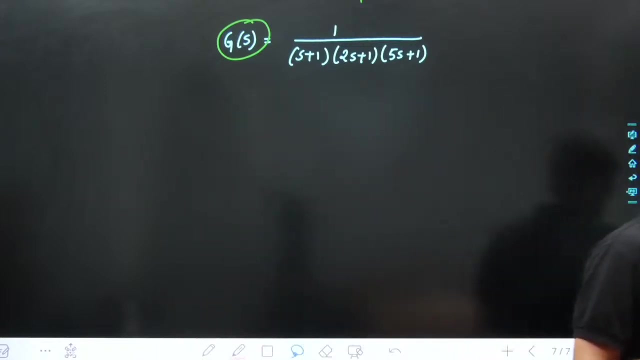 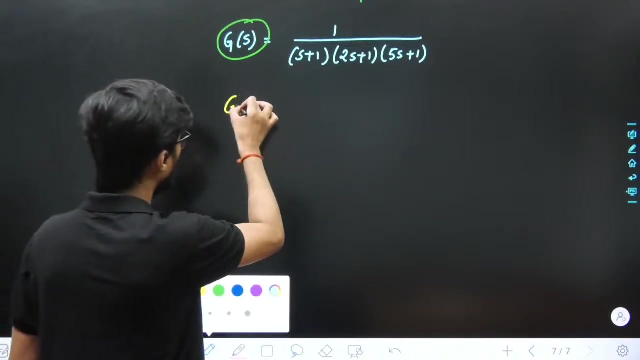 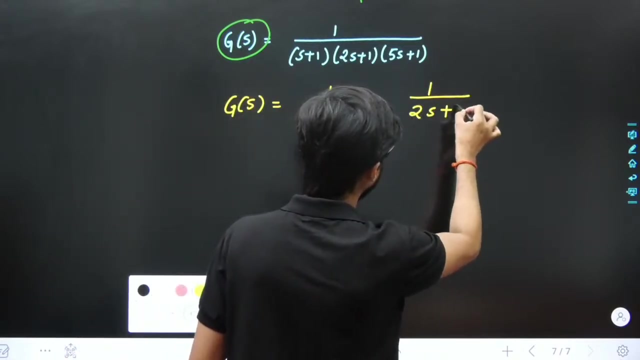 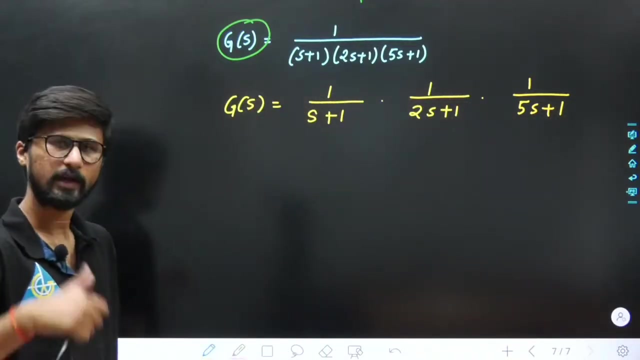 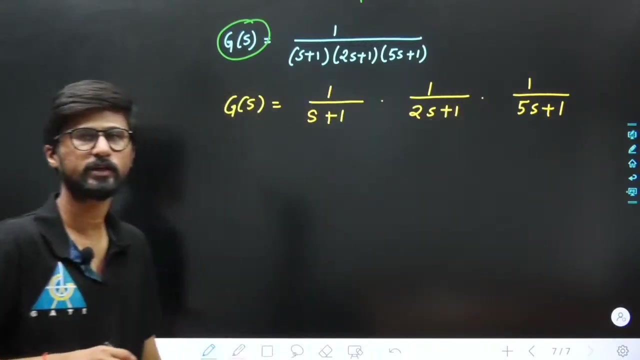 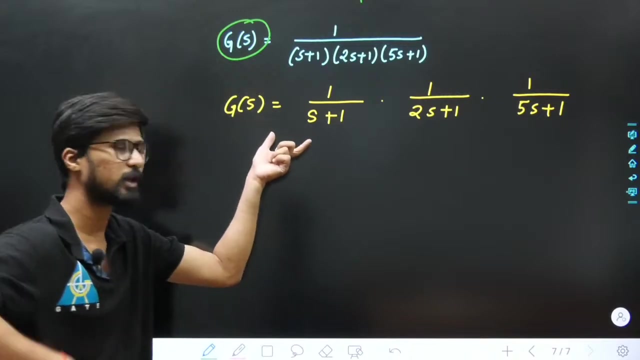 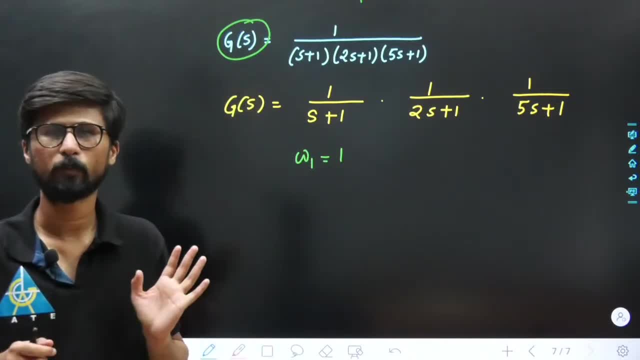 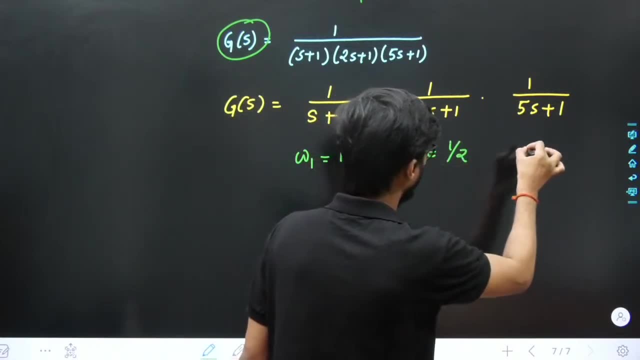 its 1, what is the corner frequency? 1 by tau, 1 by tau is the corner frequency. omega 2, this will be 1 by 2, omega 3, this will be 1 by 5.. So we have written all the corner frequency. 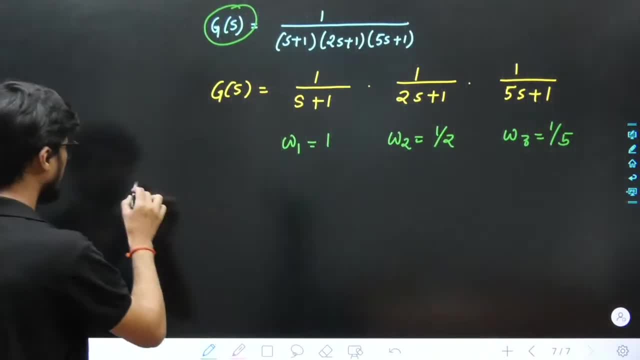 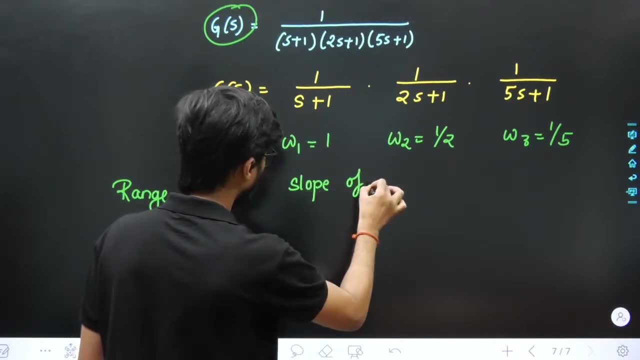 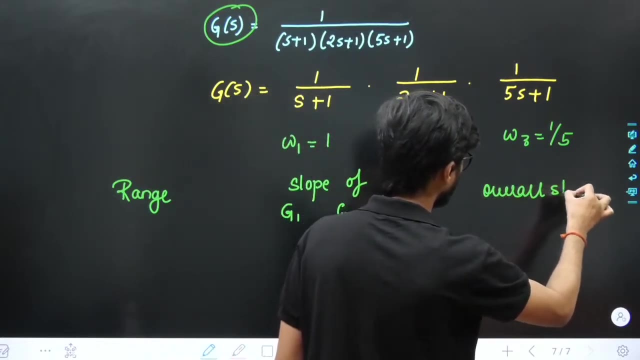 After that, what we do? we divide the range. here we write the range. here we write the slope of G 1,, G 2,, G 3, here we write the overall slope. here we write the overall slope, how to divide the range. 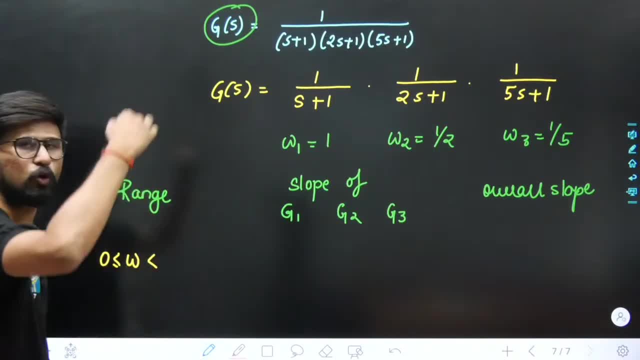 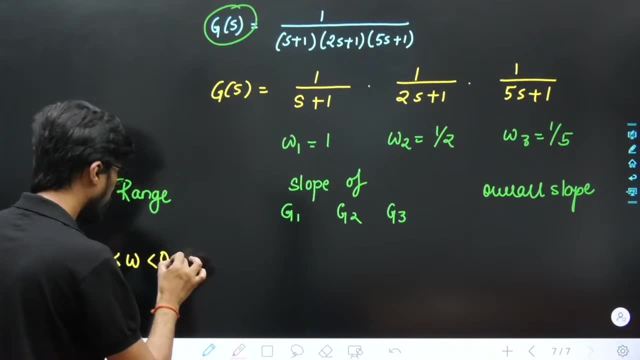 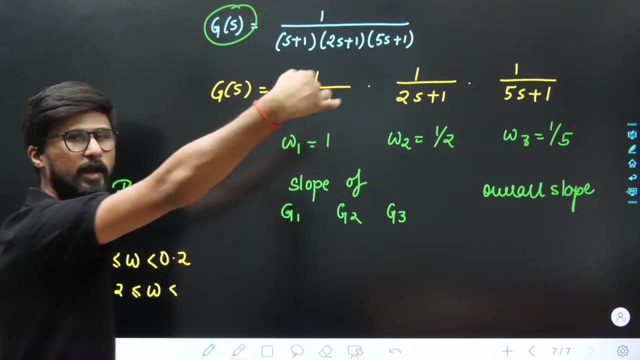 Start from 0, 0 to the lowest corner frequency now, which is the lowest: 1 by 5,. 1 by 5 is 0.2, then how will you divide from 0.2 to next higher? next higher is 1 by 2, which is: 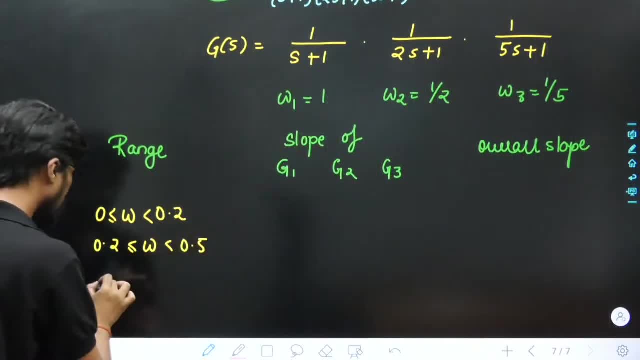 0.5,. what will be the next division? from 0.5 to next higher, next higher is 1 and then omega greater than equal to 1, this is how you divide the range 0 to the smallest corner frequency, then next higher from the smallest. then again, keep repeating like this. 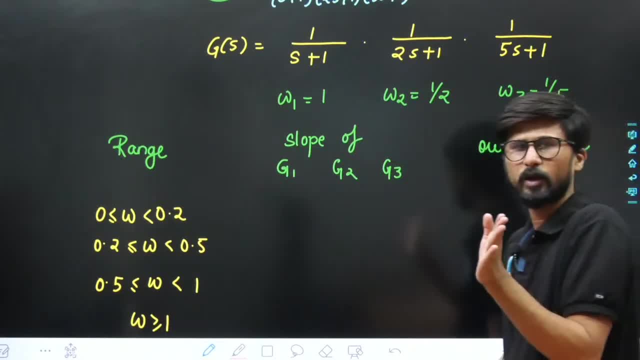 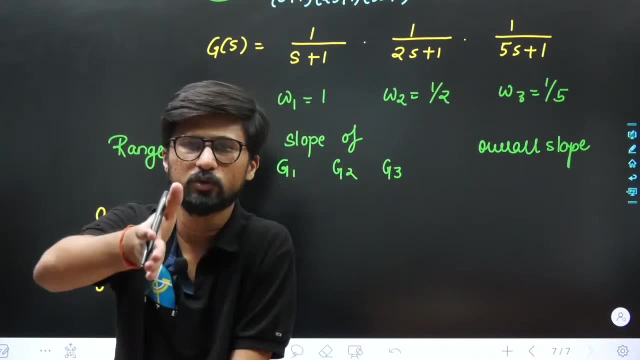 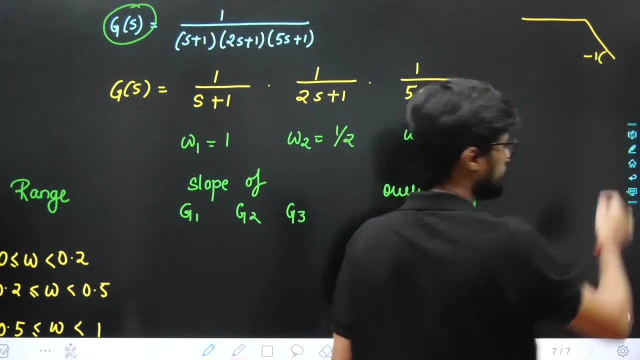 What happens in the bode plot of the first order system. till the time the corner frequency does not come, till then the slope is 0, once the corner frequency comes, the slope is minus 1.. Ok, Then what is the order of the transfer function? 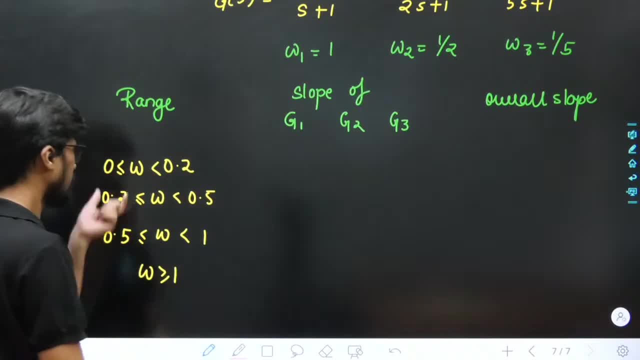 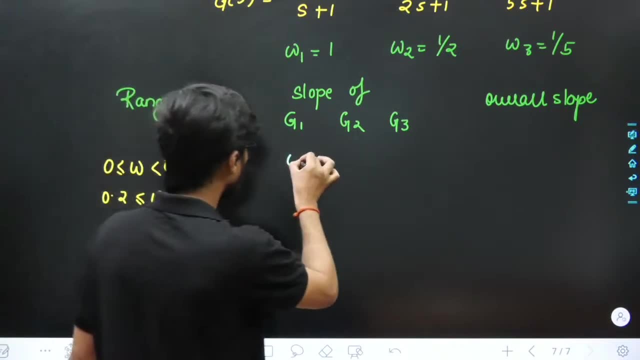 This is the graph. We will use it. So see, the 0 is omega .2,. in this range, no corner frequency has come yet. the slope of all is 0,. in this range, see from 0.2 to 0.5, whose corner frequency has crossed G 3,. 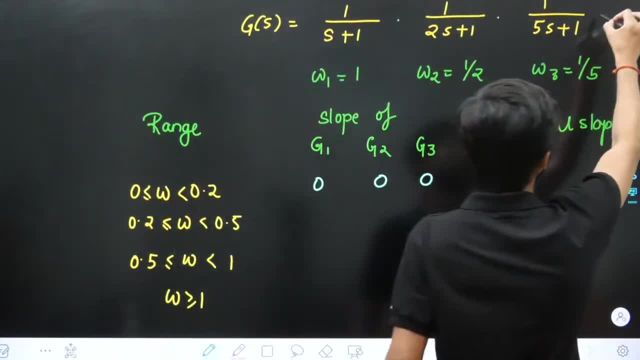 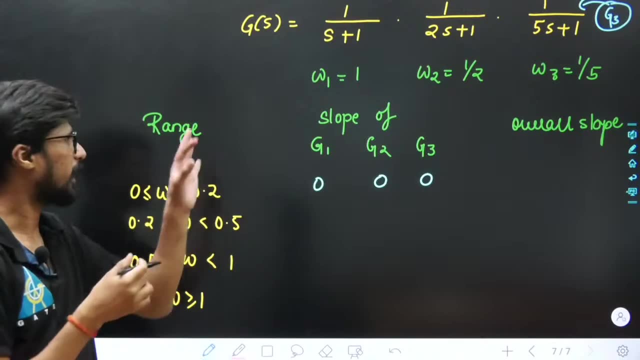 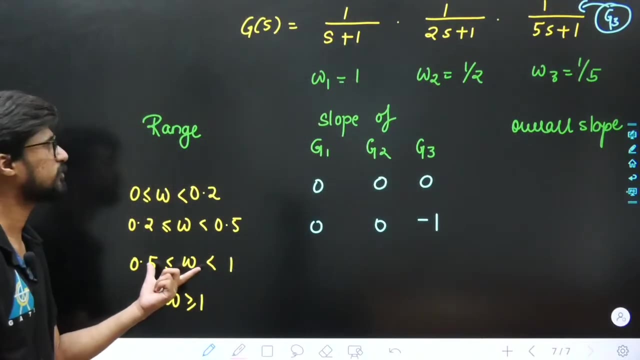 G 3 is the transfer function. So see the G 3, is 0.5.. transfer function: Its corner frequency has crossed. Its slope is minus 1.. Have other people crossed? No Other people have 0. In this range: 0.5 to 1.. Now this has also crossed. 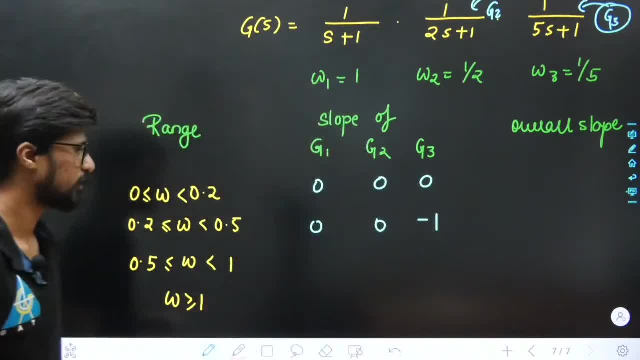 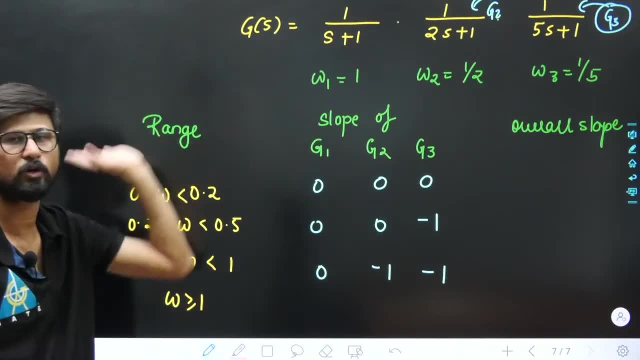 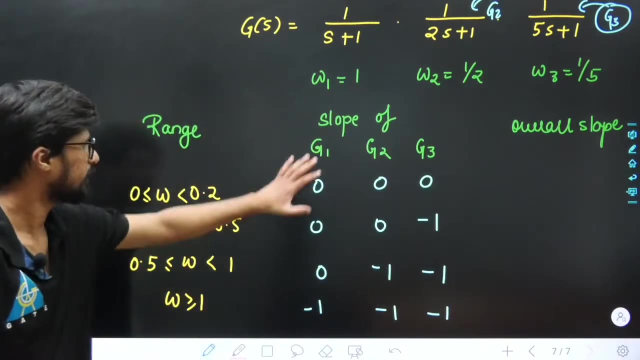 G2 has also crossed the corner frequency 1 by 2.. So its slope is also minus 1.. And omega greater than equal to 1, the corner frequency of all three has crossed, So the slope of all three is minus 1.. How do we get the overall slope? We sum individual slopes. If you sum. 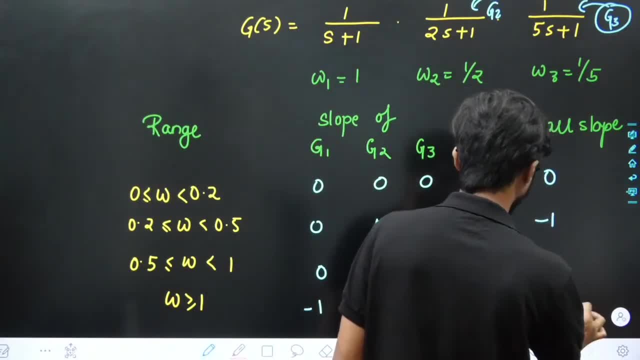 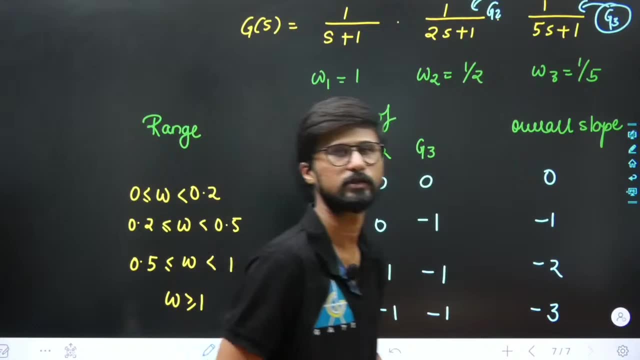 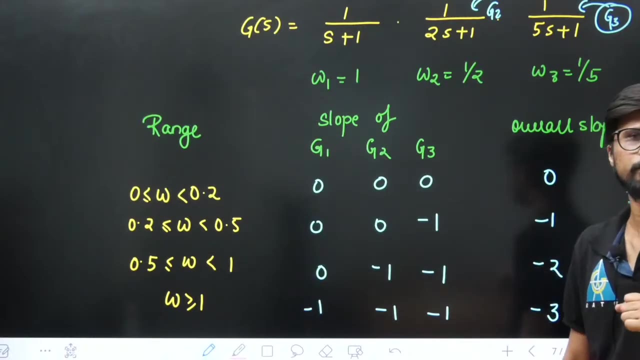 then here is 0,, here is minus 1, minus 2, minus 1.. This is how you plot the Bode plot for a system in series. Bode plot of system in series is very easy. There is no problem in it. Is this thing clear? 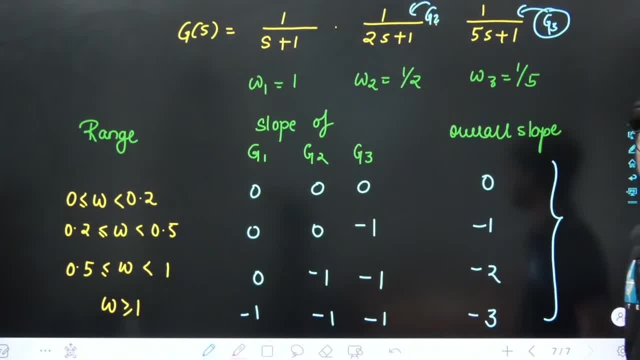 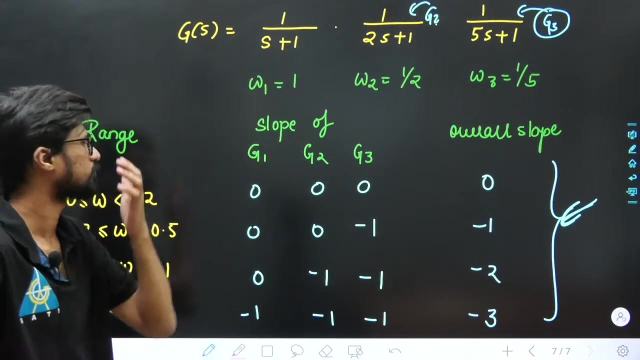 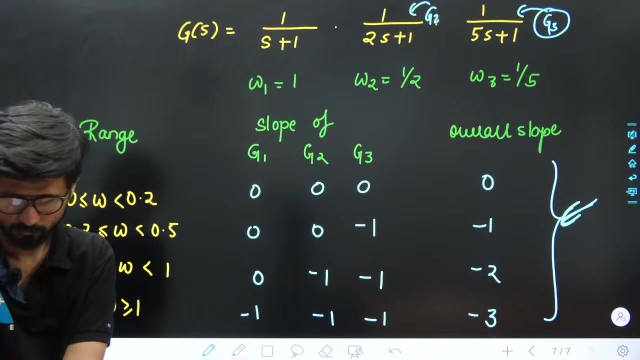 So now you can make options Match. Maybe these two things are given. This is your P, this is your Q, So P is 0, Q is minus 3.. Okay, Is it right? If X gives the number, then everything will be repeatable. This is your you classical. 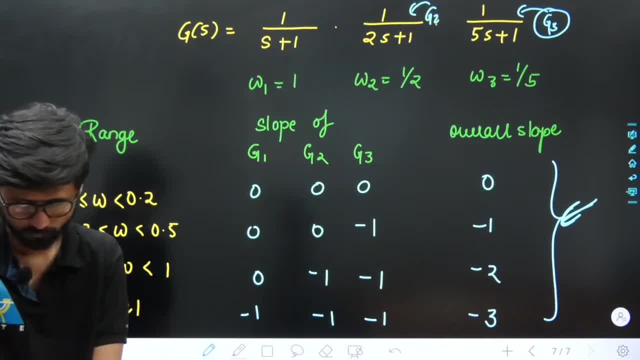 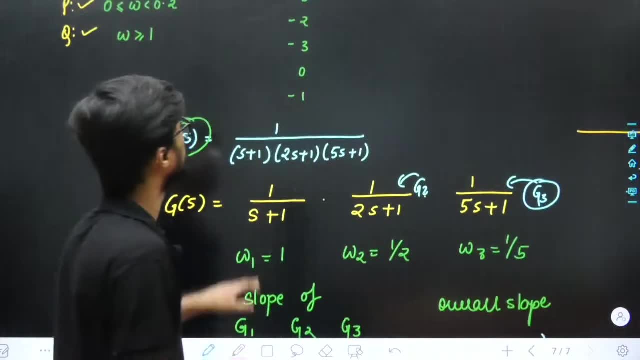 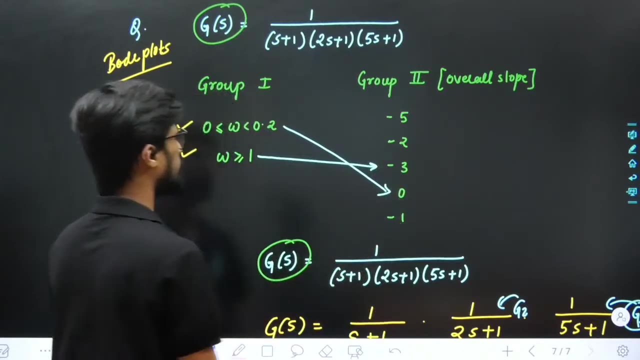 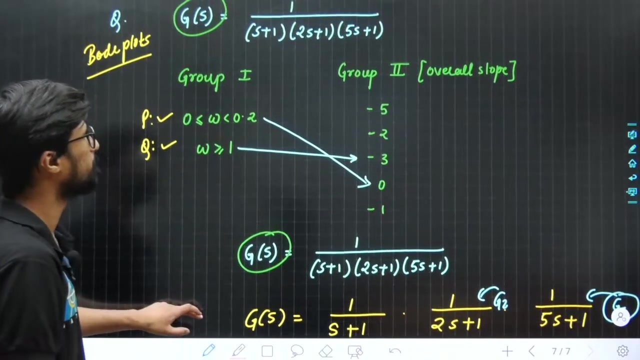 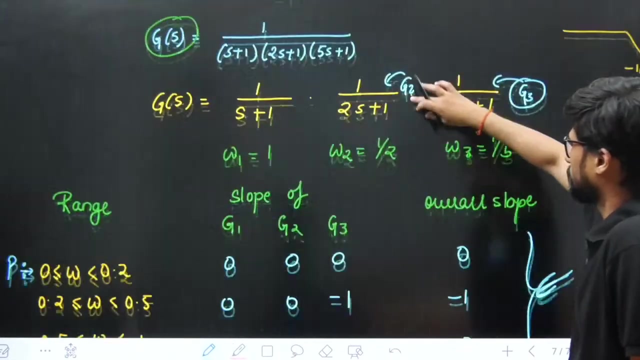 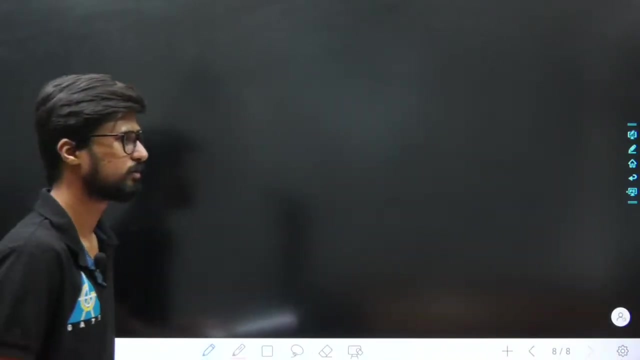 A's Okay, Sorry. So what we got, p is 0,, q is minus. Ok, take next question. note it down. Ok, next question. Next last problem. let us take then feedback, feed forward control. Let us take root array. problem. 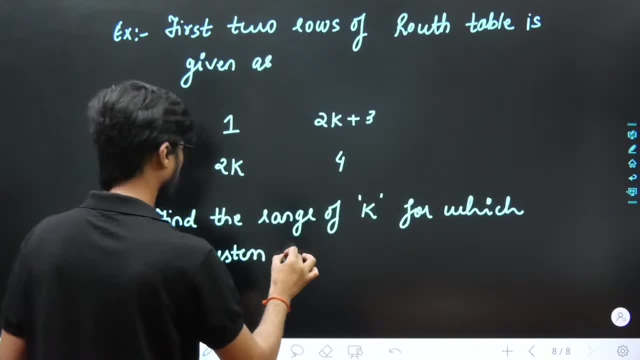 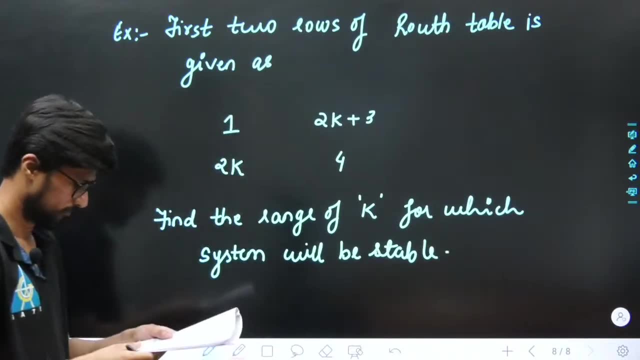 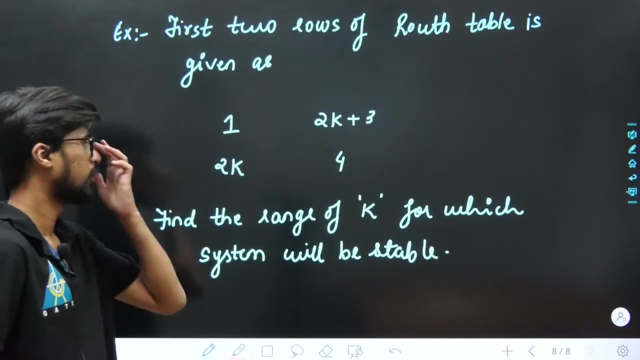 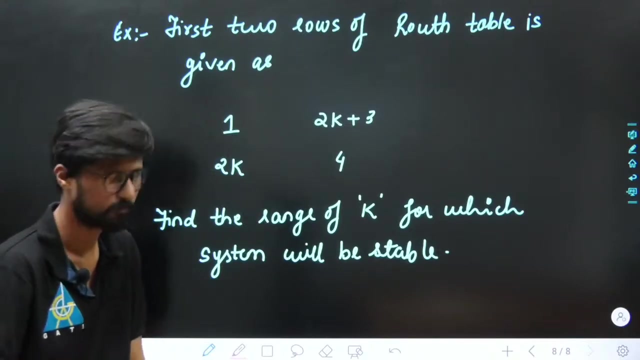 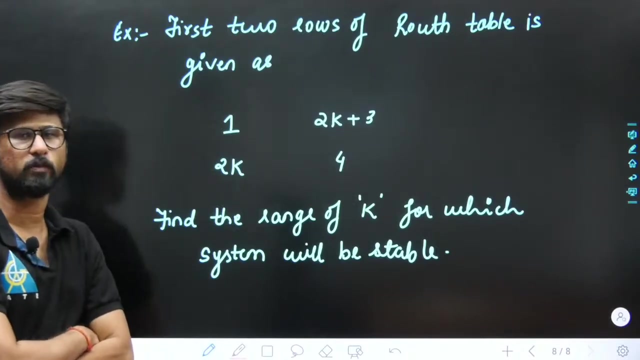 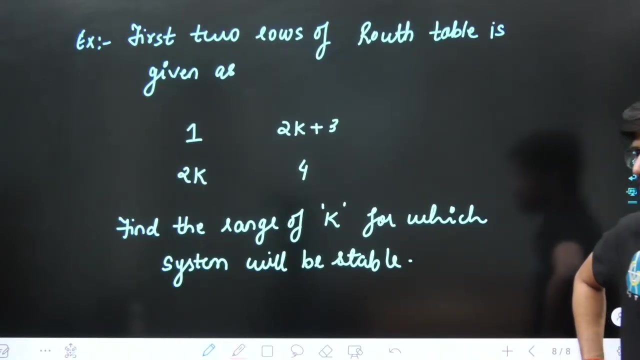 Let's do this question. Aapko batani hai range of k, for which the system will be stable. ok, Banayee jara is problem, Ok. So what is the risk factor? D Doc. Aapko batani hai gain of k, so your number is in the range of k. so your number is in the range of k a, and so your number is in the range of k b. 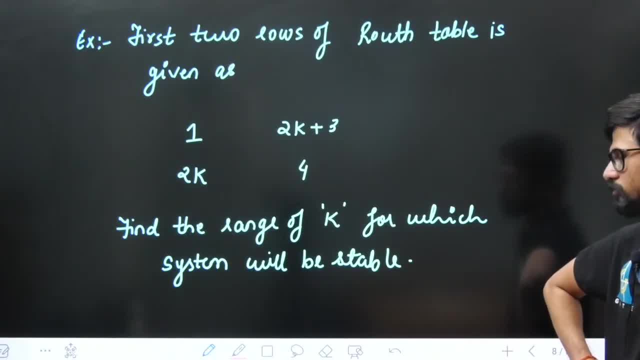 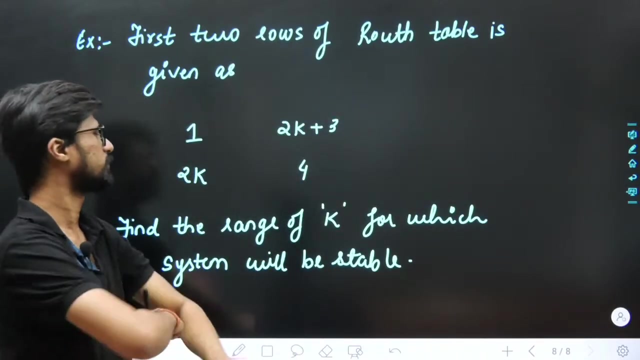 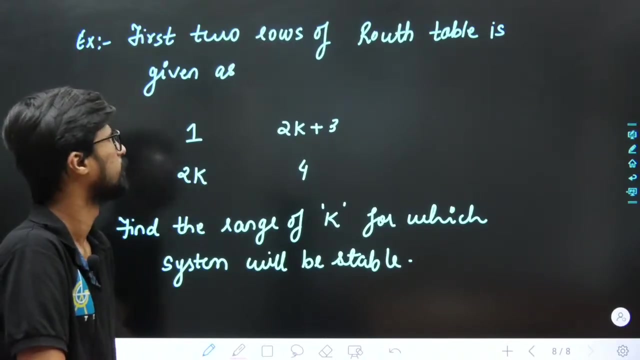 Alright, so you're not going to have an answer if your number isn't stable. Ok, So in the range of k, the highest possible risk factor would be: a number is better than a. Ok, so what's your number? Tell me the range, solve it. 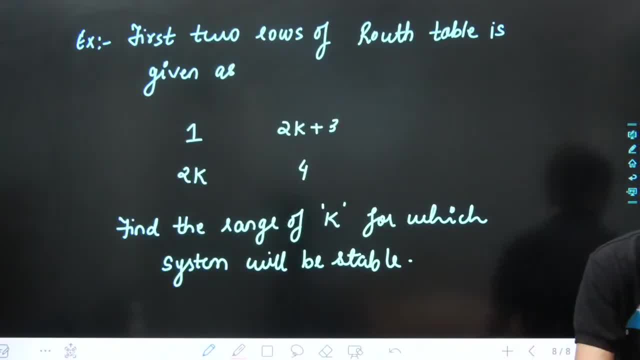 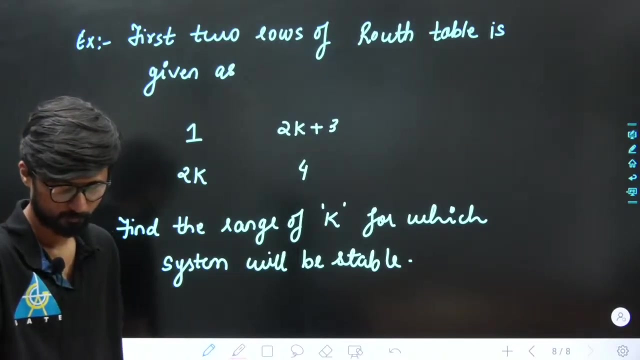 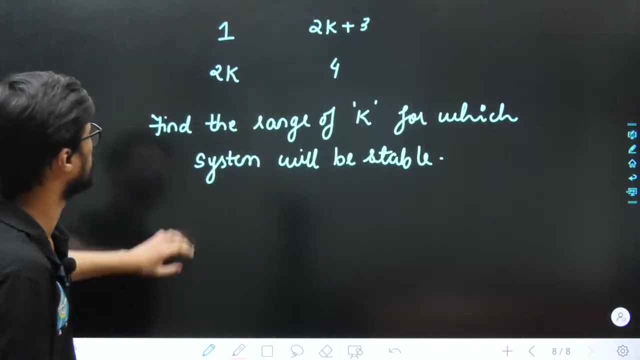 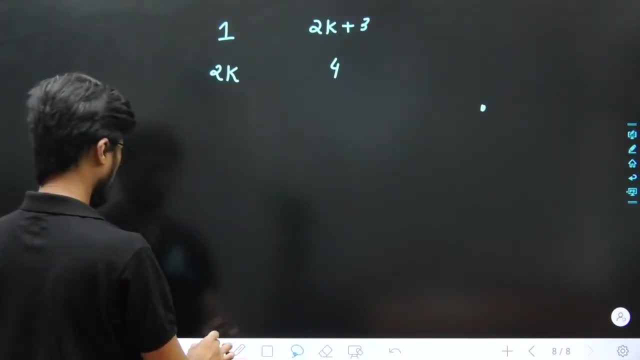 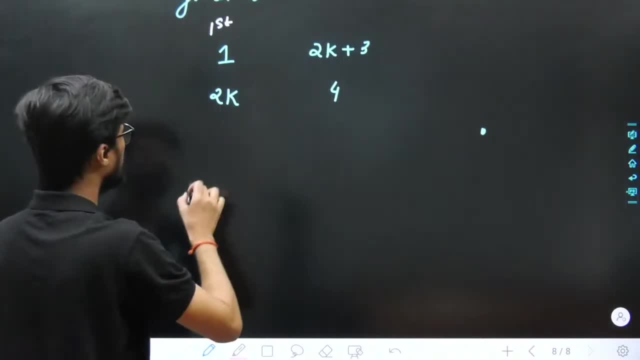 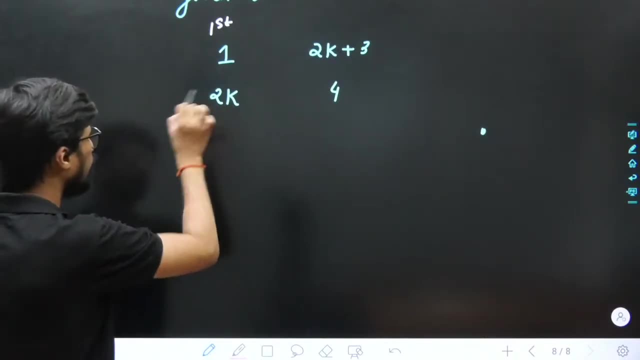 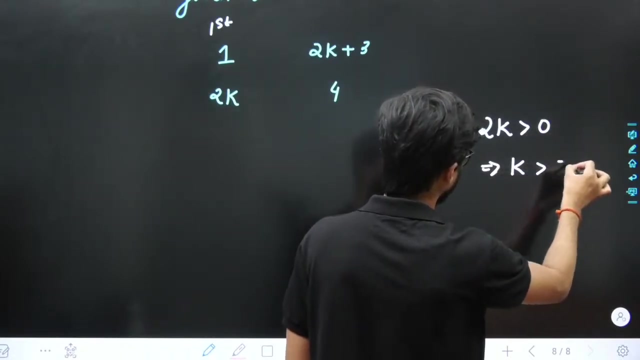 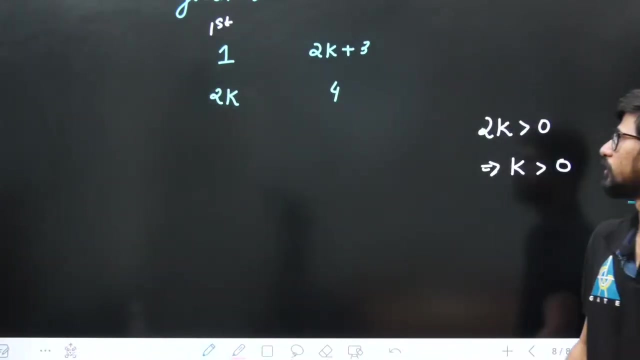 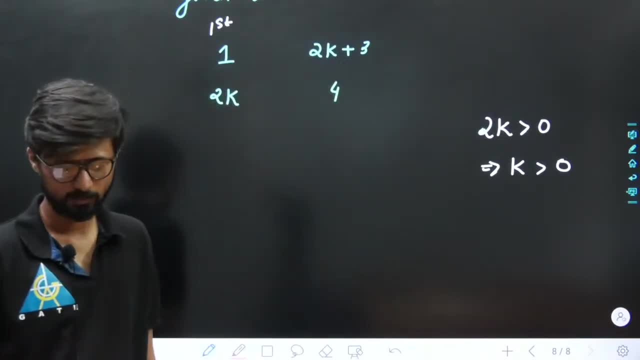 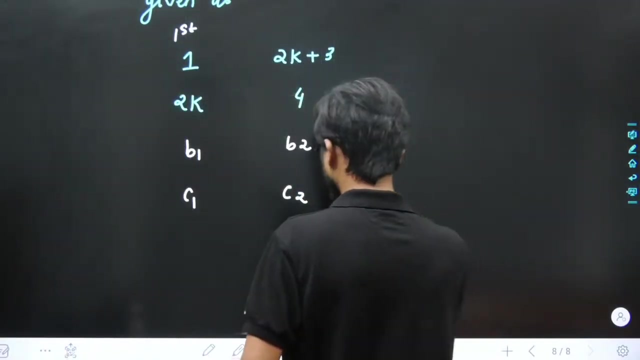 So the first thing is that k should be greater than 0. Now we have to find more elements: b 1, b 2, c 1, c 2.. How will I write b 1?? b 1 is k should be greater than 0. So k should. 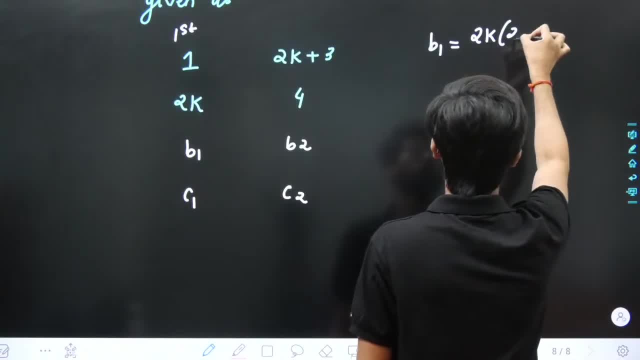 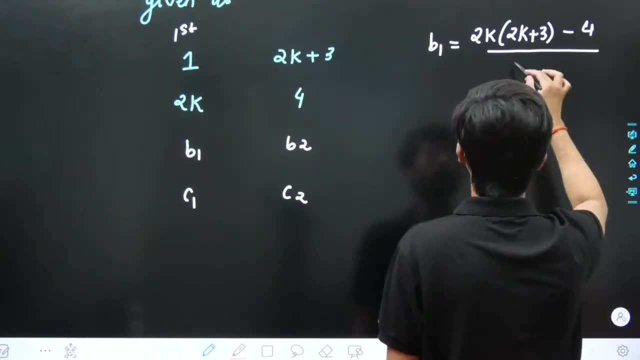 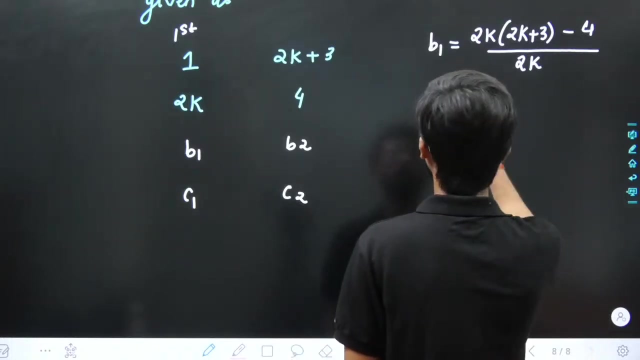 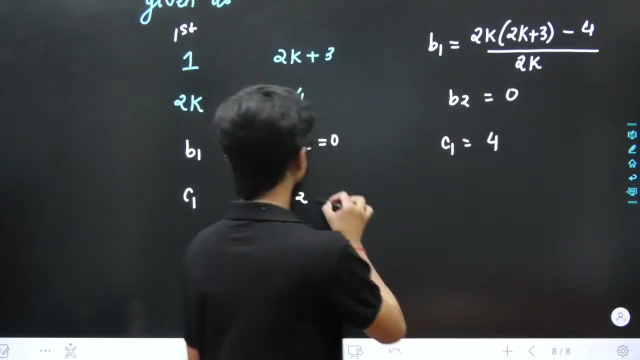 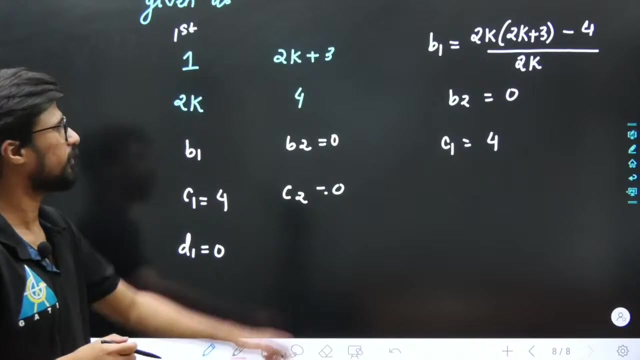 be greater than 0.. 2 k into 2 k plus 3 minus 4, divided by 2 k, This is your b 1.. b 2 will be 0.. c 1, c 2, 0.. d 1 will be 0.. This is your root array where b 1 is given. Now see. 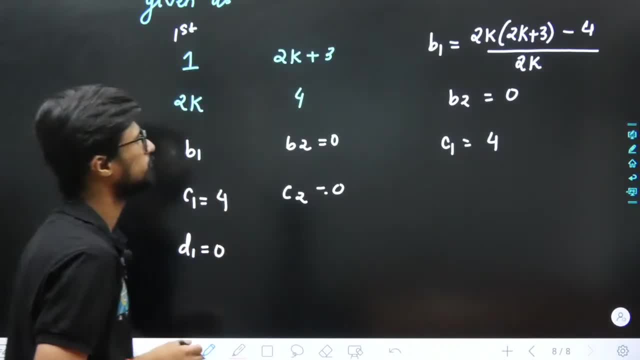 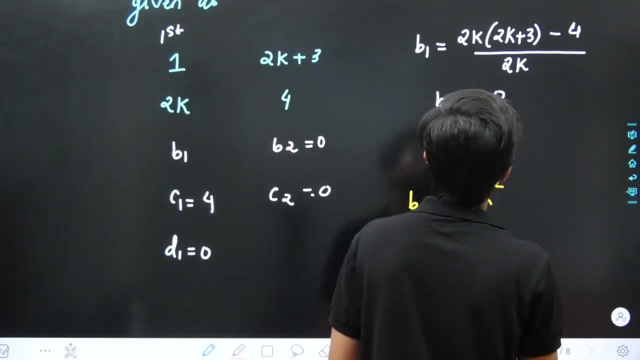 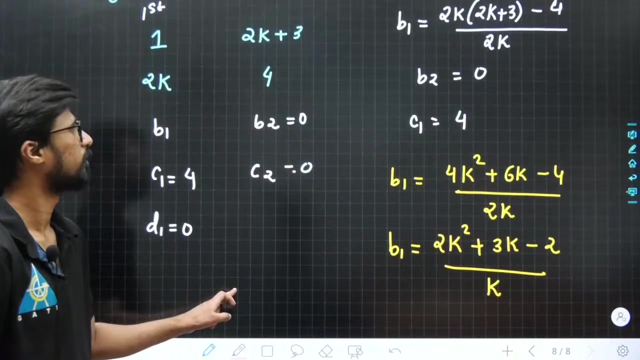 Now let us solve b 1 a little bit. 4 k square plus 6 k minus 4, divided by 2 k, 2 k is greater than 0.. 2 k square plus 3 k minus 2 by k. So one condition is that 2 k should be greater than. 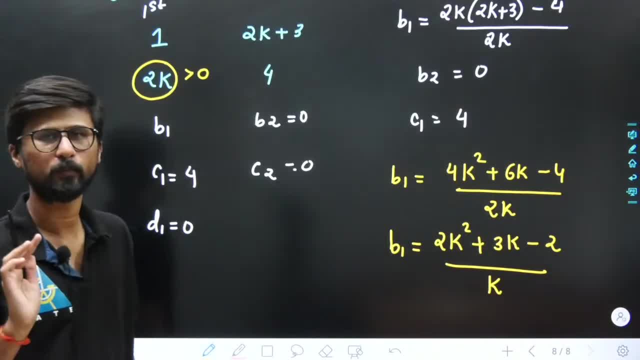 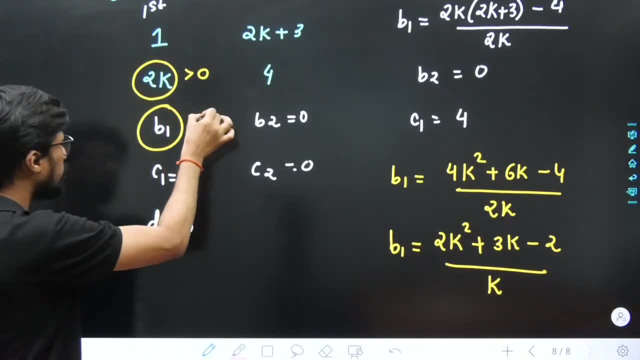 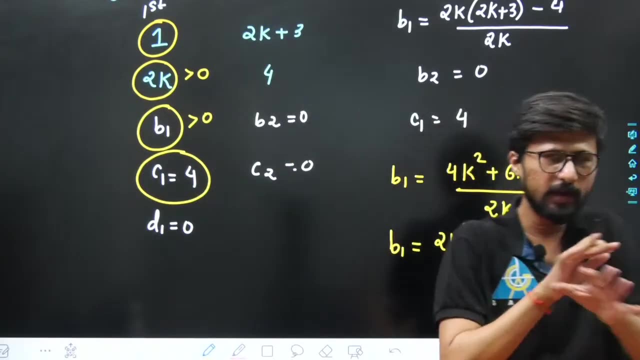 0, which means k should be greater than 0. This is the condition: k should be greater than 0.. Second thing is: b1 should be greater than 0, because 1 is greater than 0, 4 is greater than 0. So how will all the elements of the table be? Sorry? how will the elements of 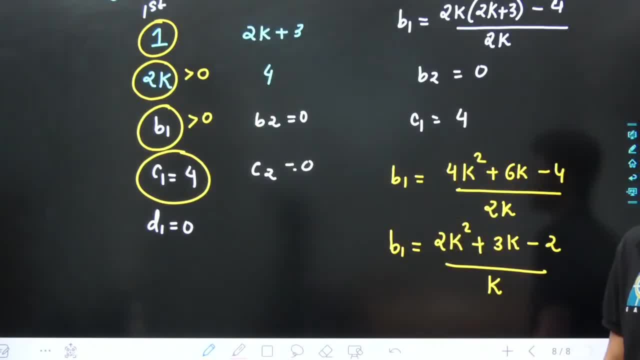 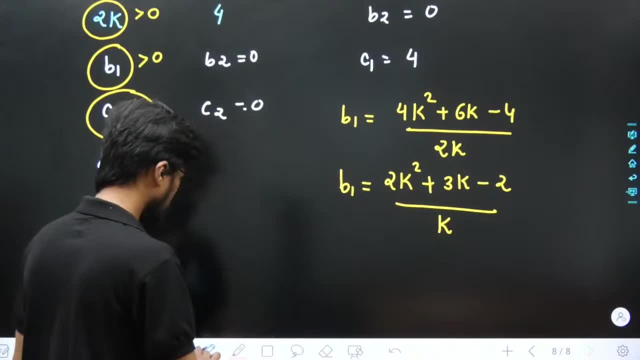 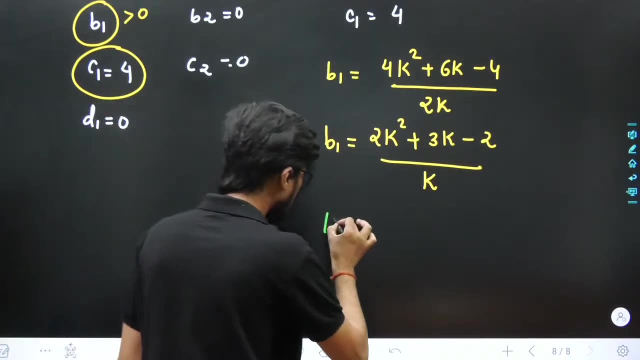 the first column be: They will be positive. Let us see what condition is there to make b1 positive. We have to make b1 positive. So see: k is greater than 0. This condition is there that k is greater than 0. k cannot be negative, So k is greater than 0. So 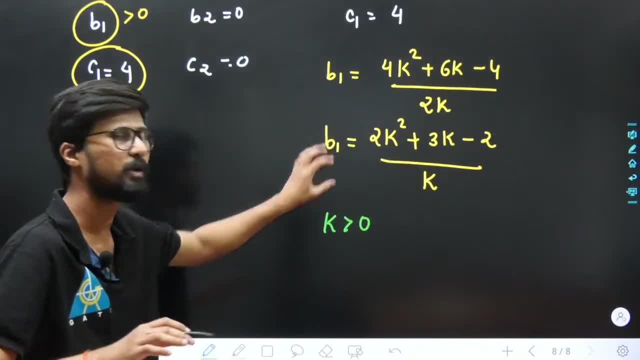 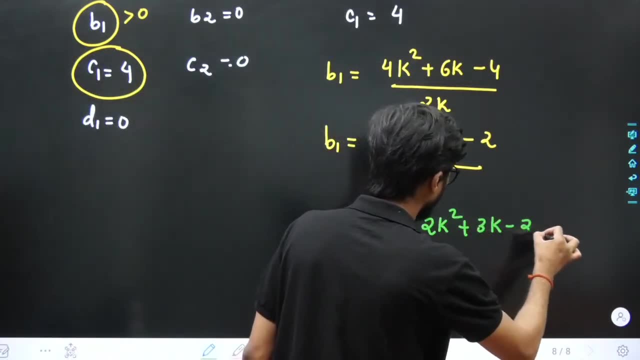 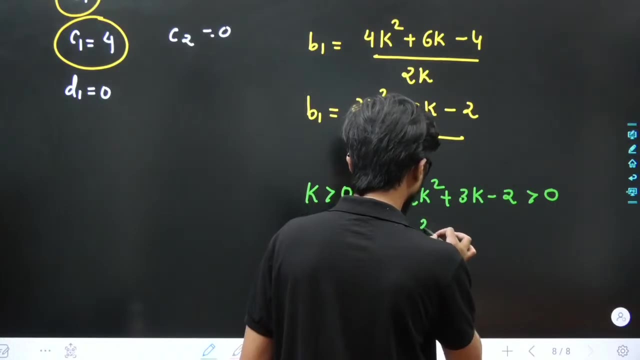 how should the above term be Greater than 0. Then only b1 will be positive. So 2 k square plus 3 k minus 2, this should be greater than 0.. We will solve it: 2 k square plus 4 k minus. 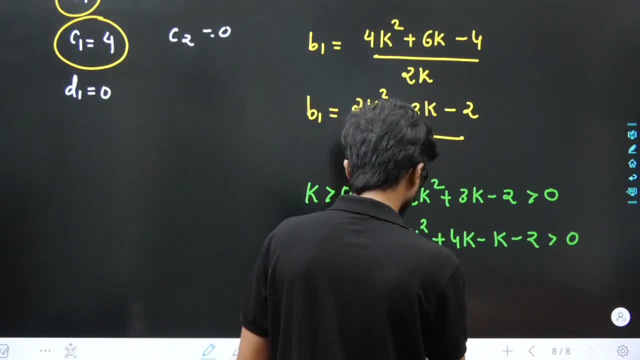 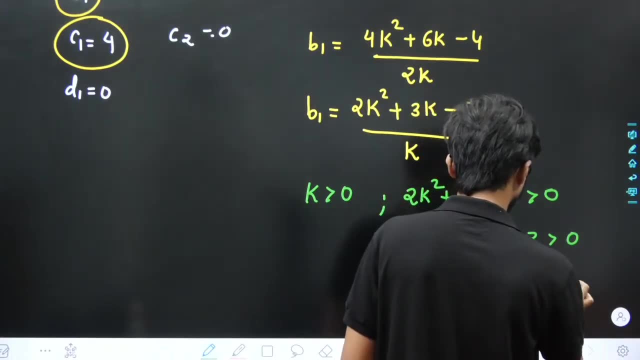 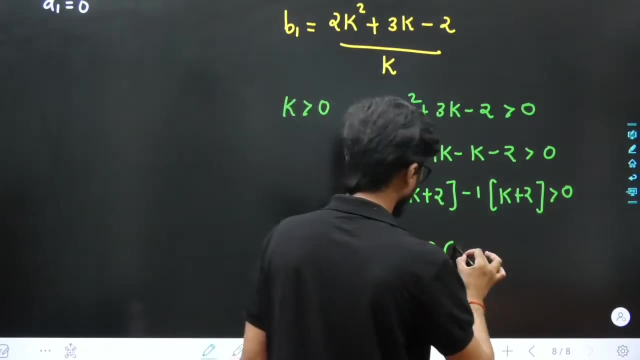 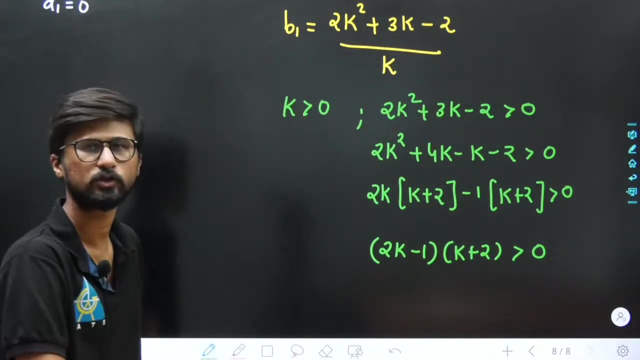 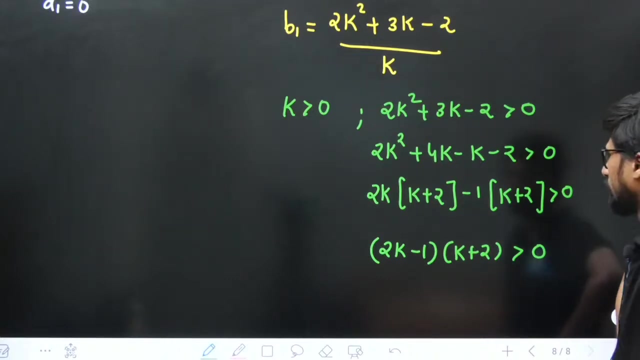 k minus 2 should be greater than 0.. 2 k k plus 2, 2 k minus 1 into k plus 2, this should be greater than 0.. This should be greater than 0.. And for this, CIAE equals to kleine chips plus minus 1, to do this, let us follow one. 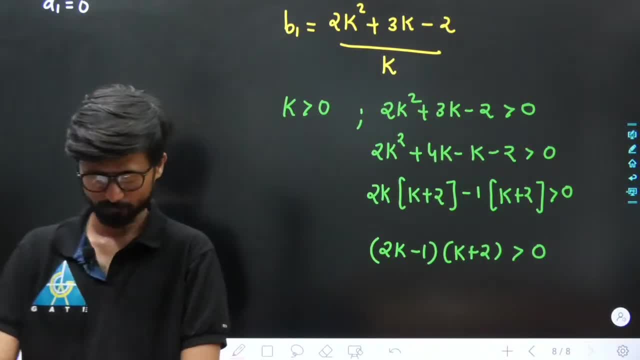 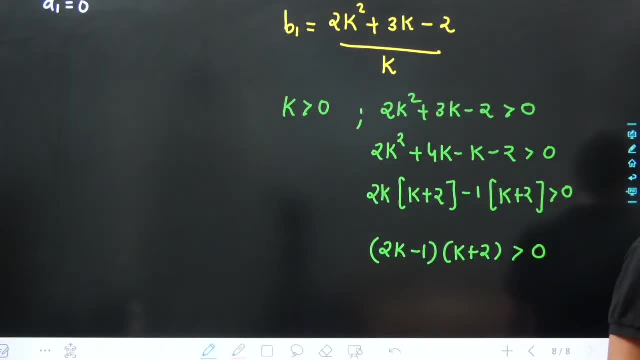 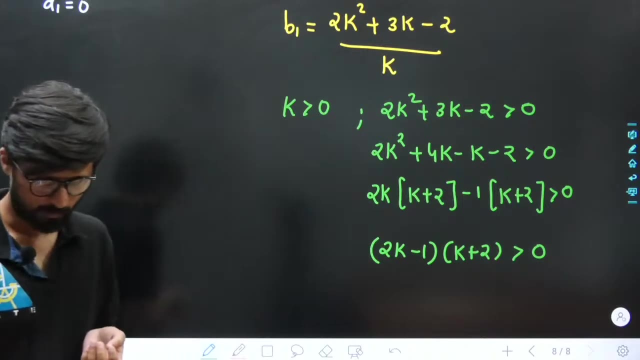 more experiment here, For x is greater than 0.. Think about it. Let us assume that it is greater than 0.. Tell me Minus 2 to consider: he nahi kar sakte. Minus to hoi nahi sakta. Minus to hoi nahi sakta. 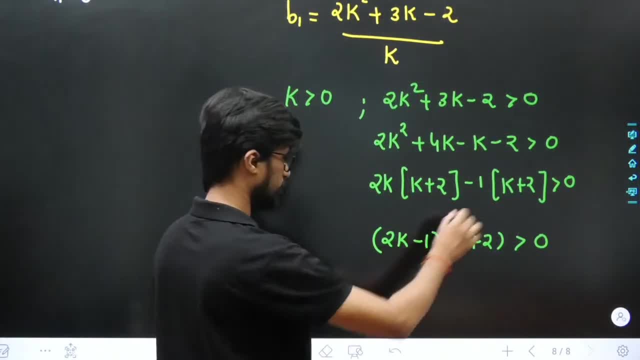 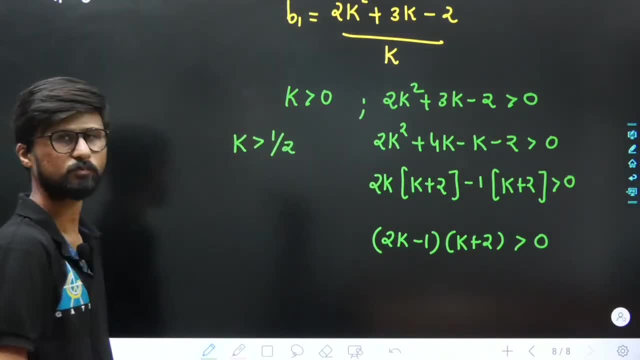 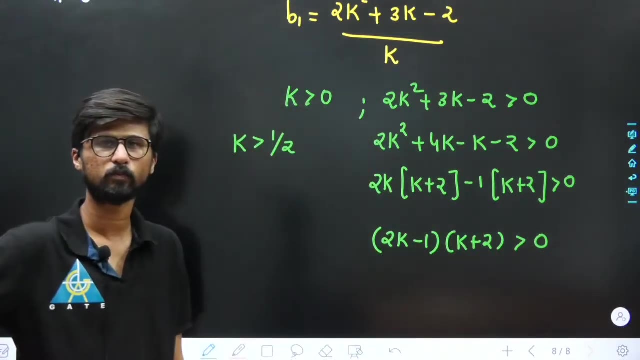 Aur aur. tum dekho ki k should be greater than 1 by 2.. K should be greater than 1 by 2, tabhi ye positive aayega. Dekho na K ki value, agar 1 by 2 se kam rakhoge, maanlo k. 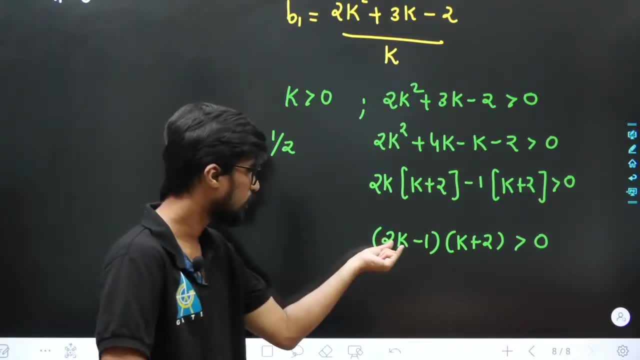 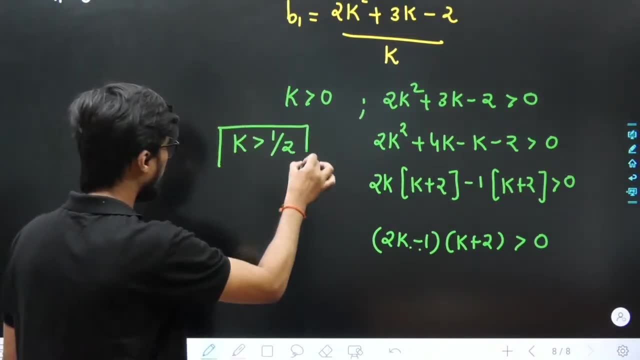 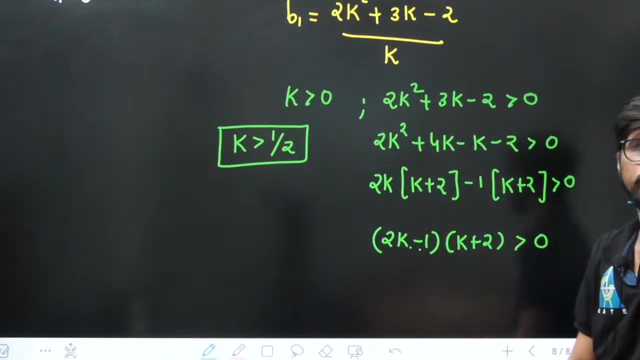 ki value apne 0 ragdi. K ki value apne 0 ragdi to ye to minus 1. ho gaya Minus 1 into 2.. Dekho To k should be greater than 1 by 2.. Dekho K should be greater than 1 by 2.. Dekho. 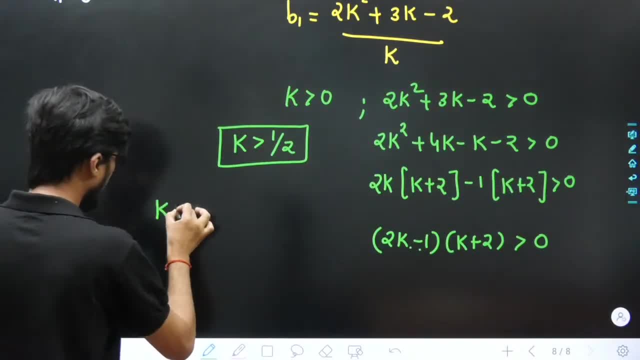 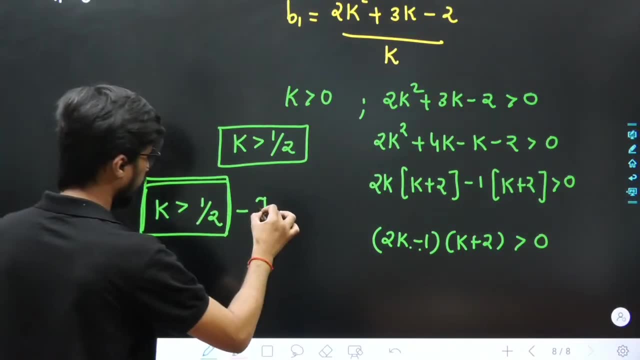 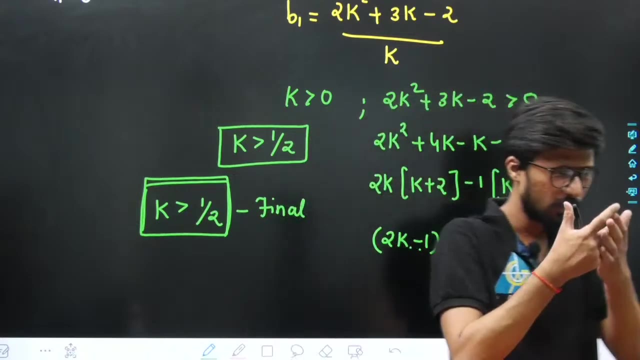 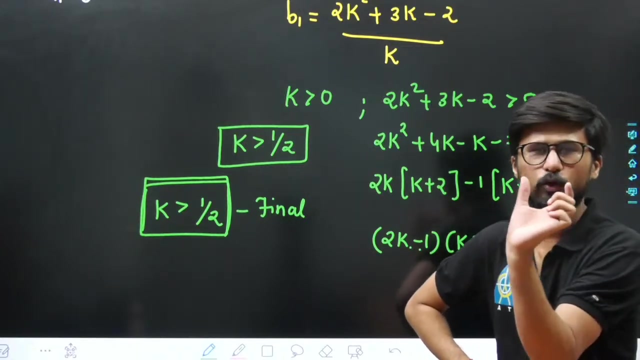 This is the condition K greater than 1 by 2.. Final condition, Final Dekho Kyuki k: ek jaga se aaya greater than 0.. Ek jaga se aaya greater than 1 by 2.. To aap 0 se 1 by 2 ke. 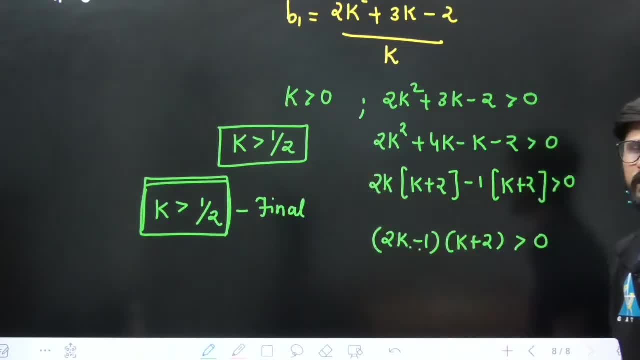 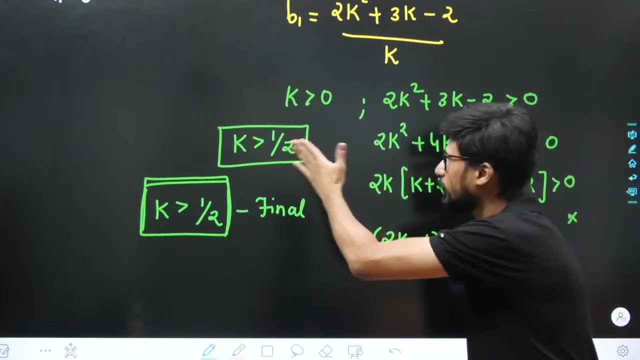 beech me bhi nahi rakh sakte, 0 se 1 by 2 ke agar me beech me rakh doge, to ye wali condition satisfy nahi ho paayi, Humko dono condition satisfy karne To. k should be greater than. 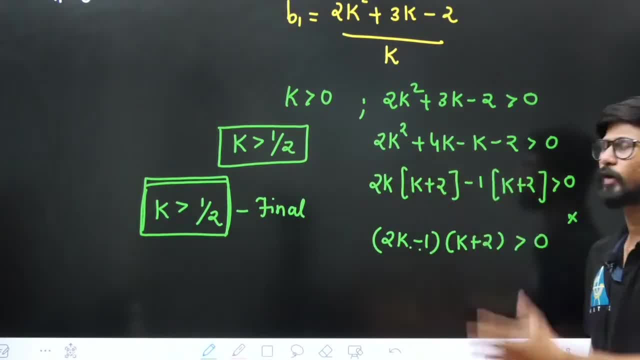 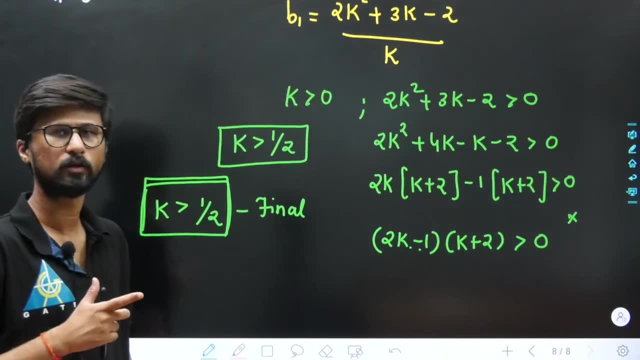 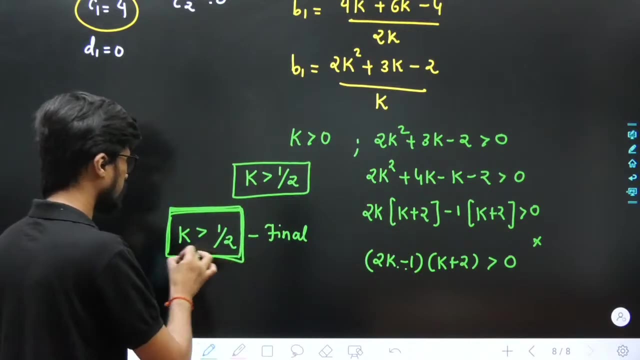 1 by 2.. This is your final answer, Kike Clear hai. So dhyan rakhenge. mistakes ho jatey Dekho, Mistakes ho jatey. K should be greater than 1 by 2 is the final answer. Final range. 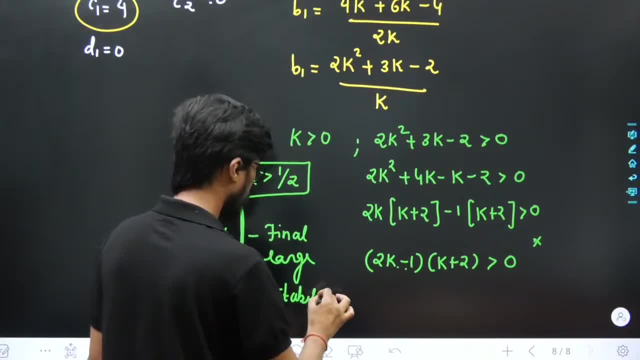 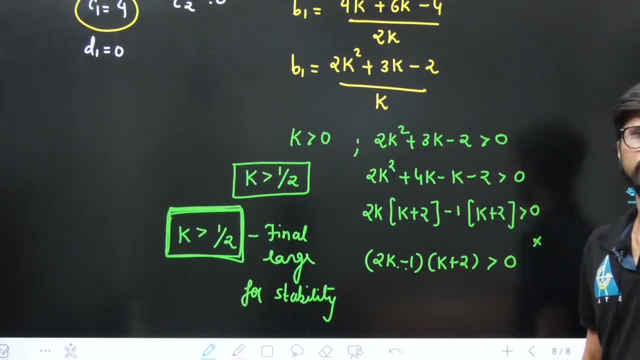 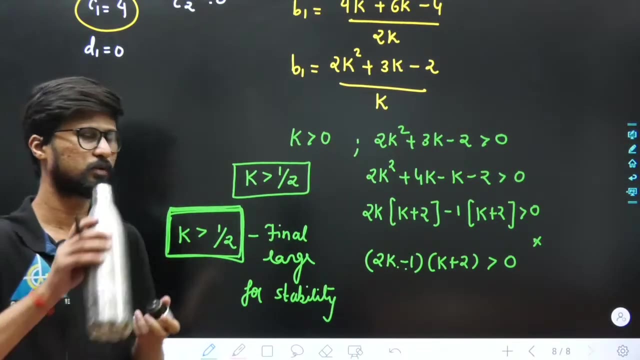 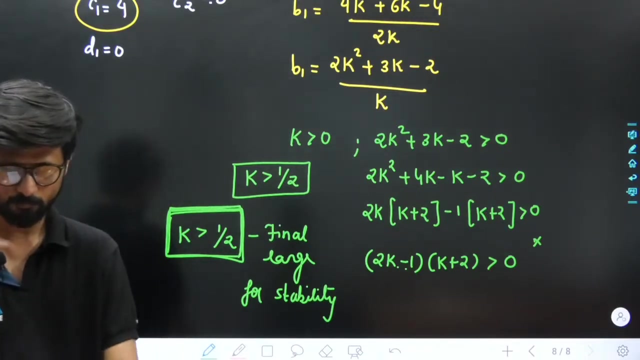 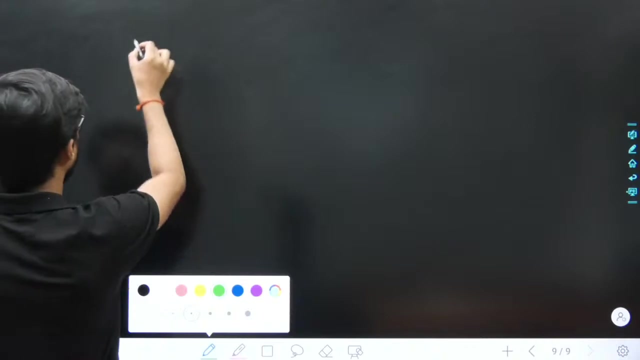 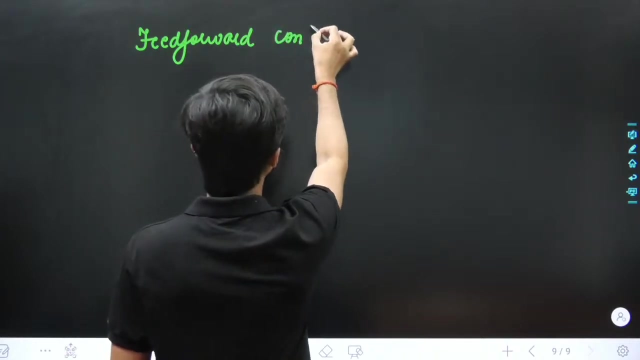 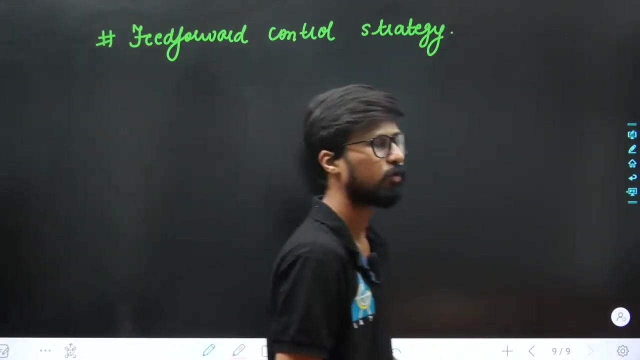 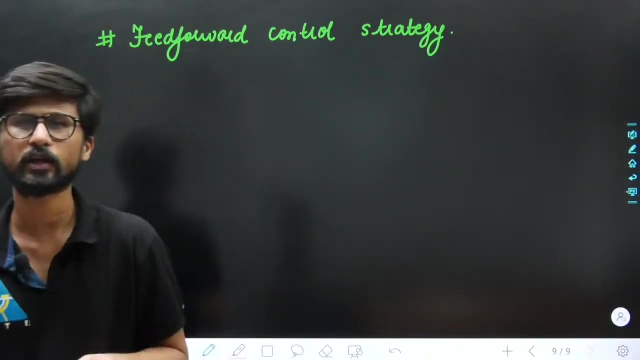 For stability. Dek baat hai Mistake likhna. agar mistake ke ho. Dek Clear hai: 0.. Let's start feed forward control. so feed forward control strategy. Feed forward control strategy. so problems practice karte rahi hai ye mistakes kar raha. 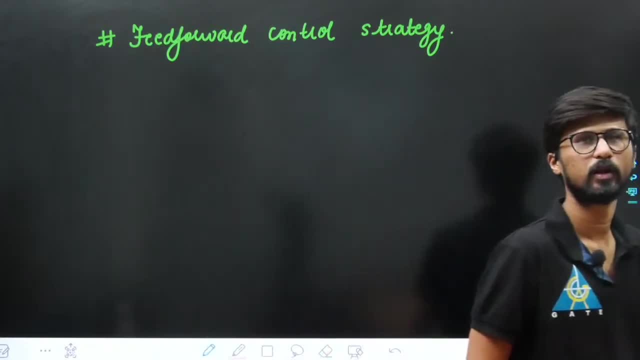 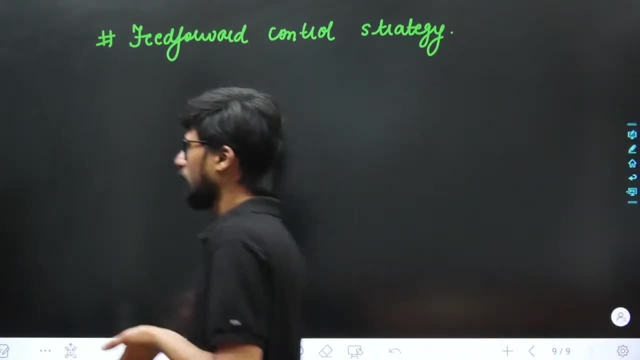 hai choti, choti mistakes ho rahi hai. ye practice se chali jayi practice karte rahi hai mistakes kam ho jayi feed forward control strategy. ab dekhi ye kya hai feedback me. 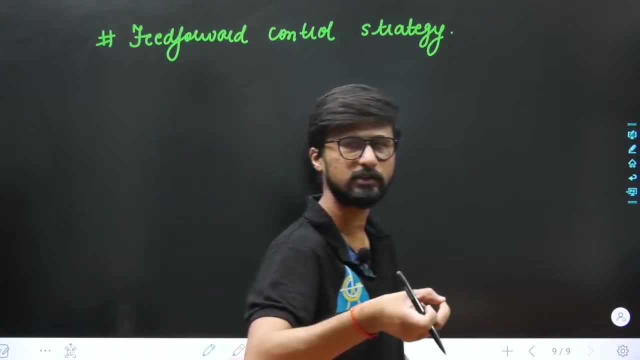 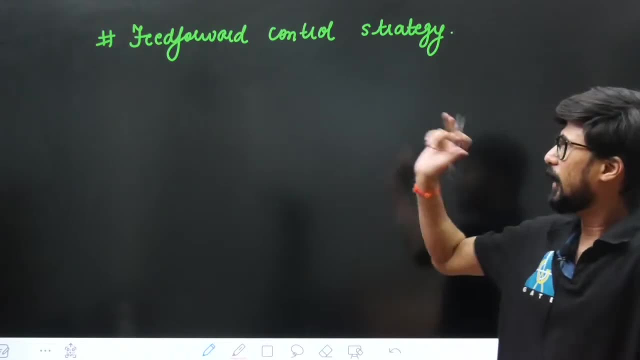 hum log kya kar raha hai feedback me. hum log output ko sense karte the jo control variable hai usko measure kar ke, then hum integrate it, then we will be able to do: change the output ko change karte the the yaha pe hum kya karenge hum disturbance ko. 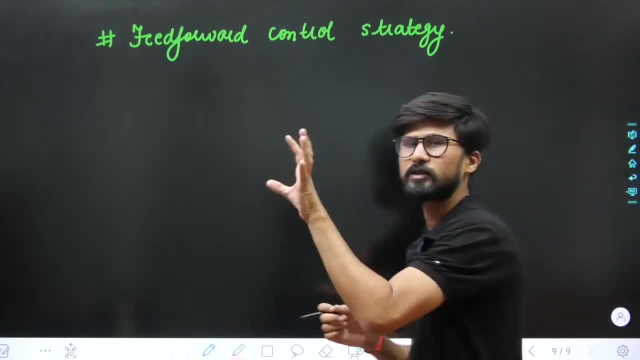 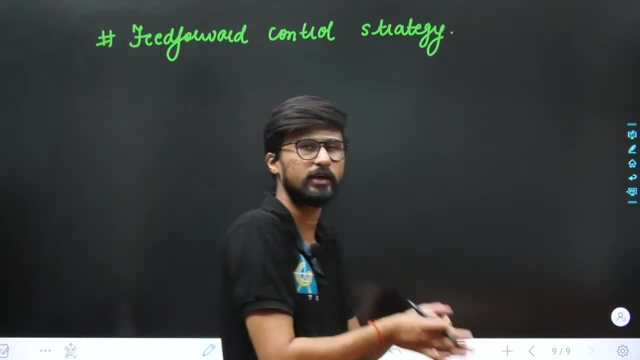 sense karenge the aur jo disturbance hai, uske effect ko hum output pe nahi aane. dekhe the disturbance ko sense karke, then hum apna output adjust karenge. the dekho jara. 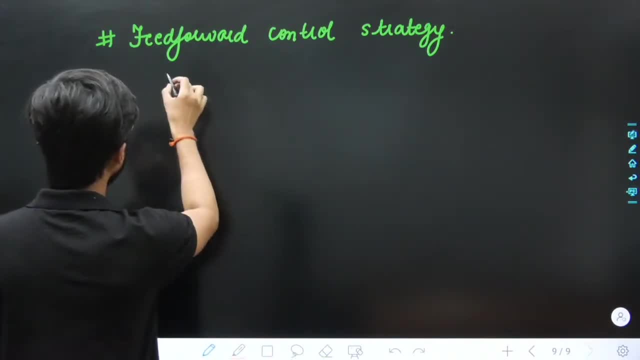 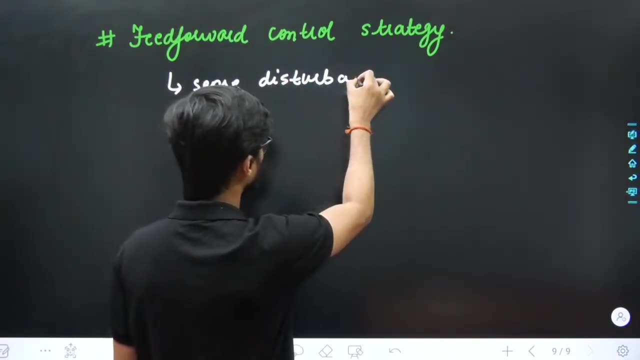 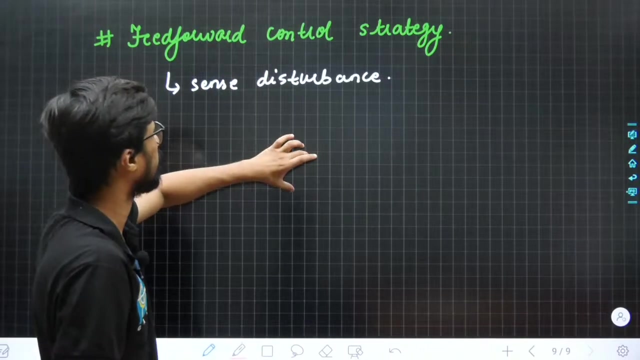 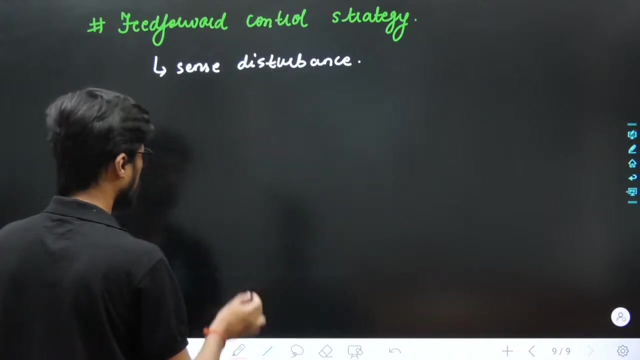 ki in feed forward control we sense Disturbance, disturbance. ko sense karte the Ab dekhi, kyaise iska maa kar block diagram banao aapko to dekhi, dekhiye ga iska block. 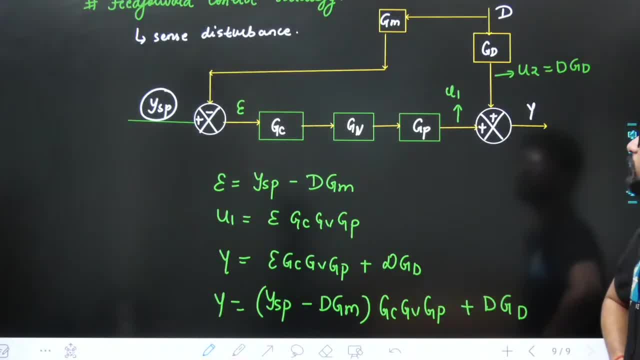 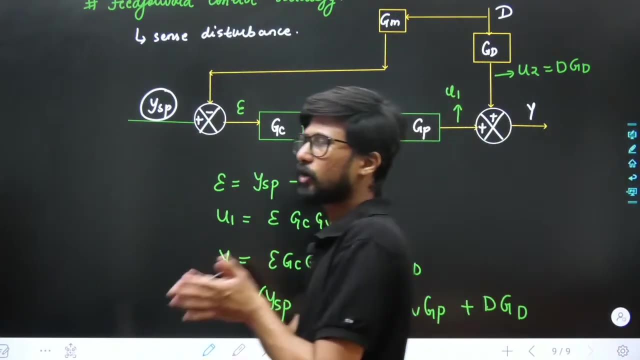 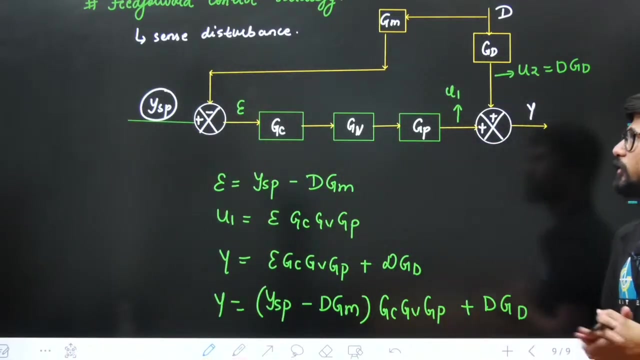 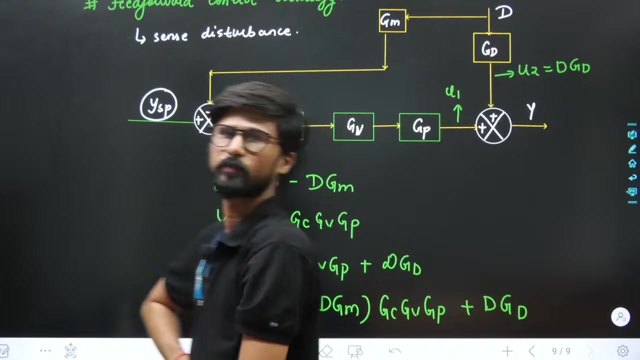 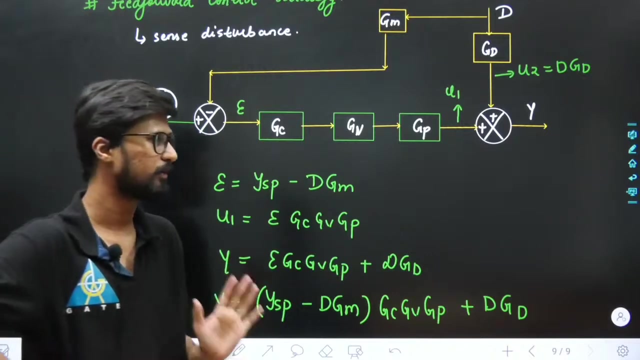 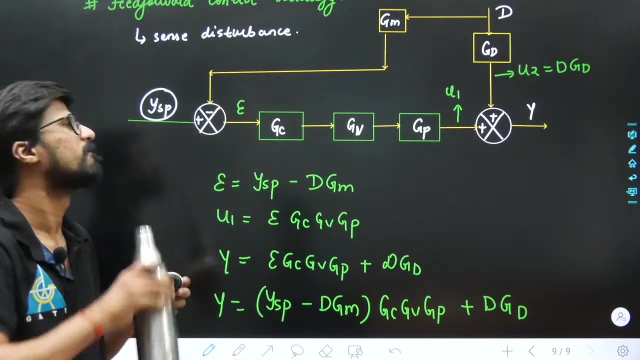 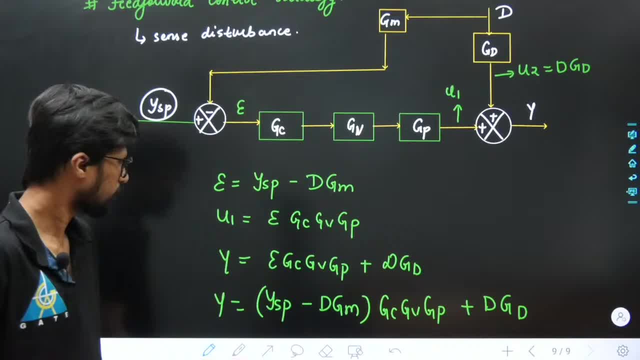 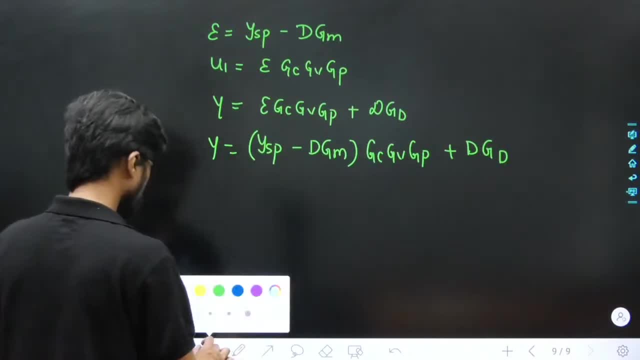 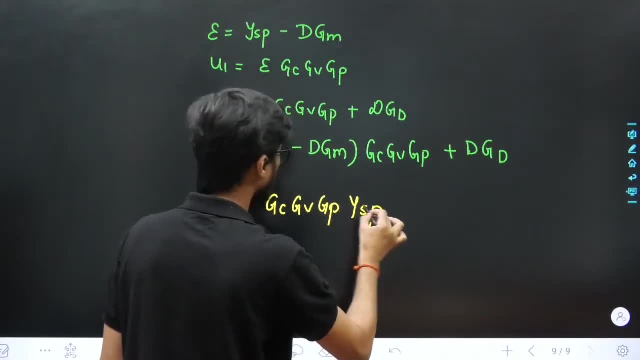 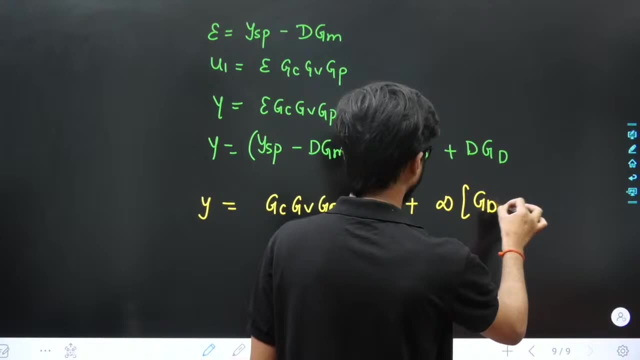 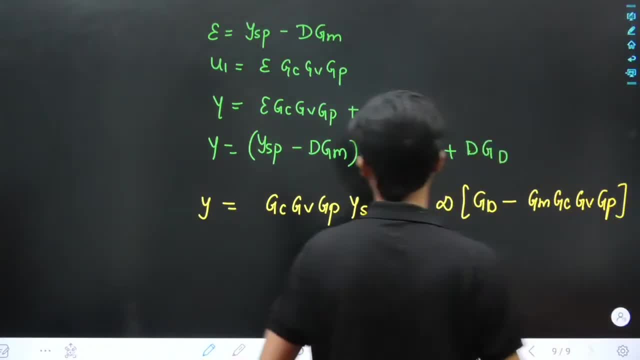 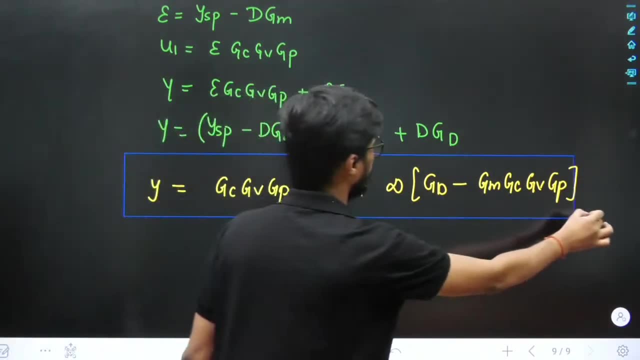 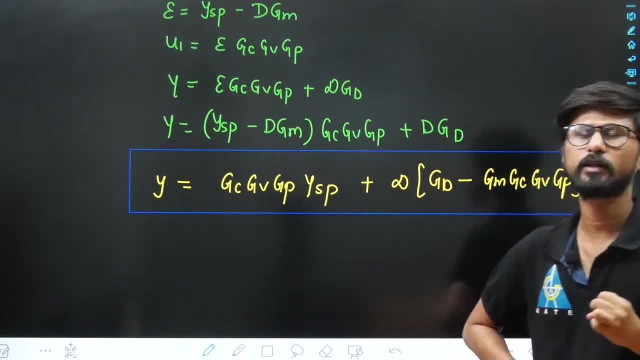 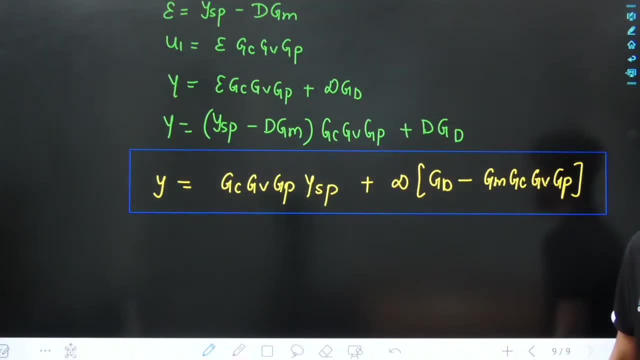 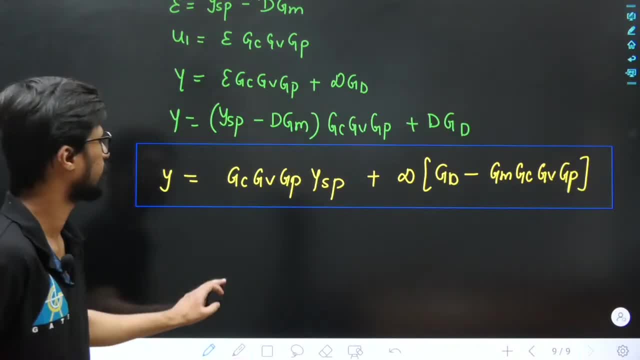 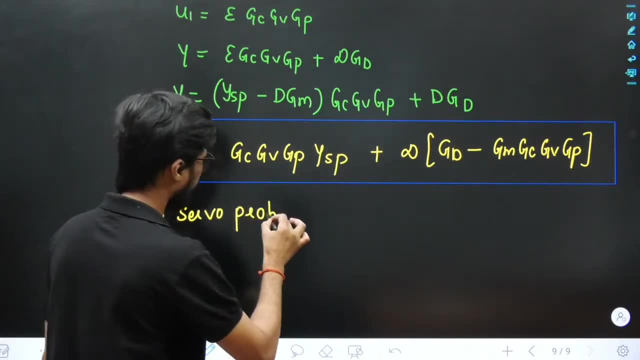 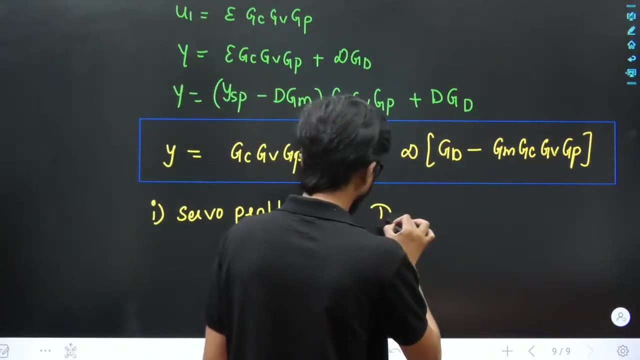 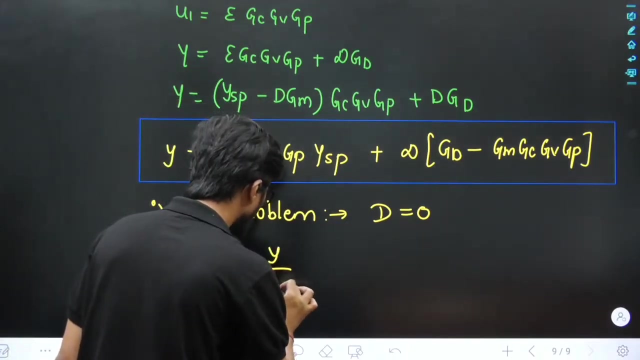 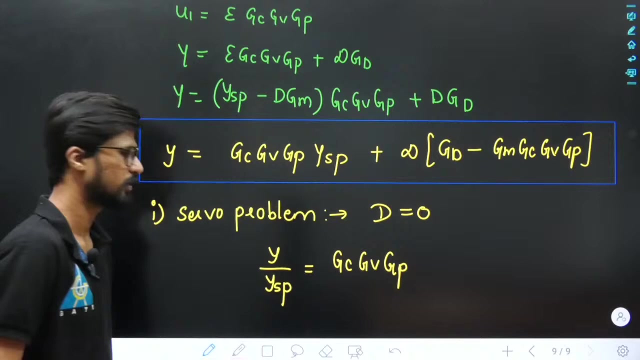 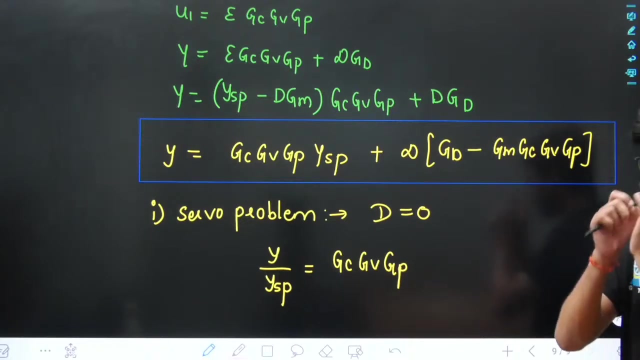 Thank you, Thank you, Thank you. What do you do in servo problem? In servo problem, you keep disturbance as 0, ok, This is done and write value of y by ysp. ok, Now, servo problem means what you have to do. 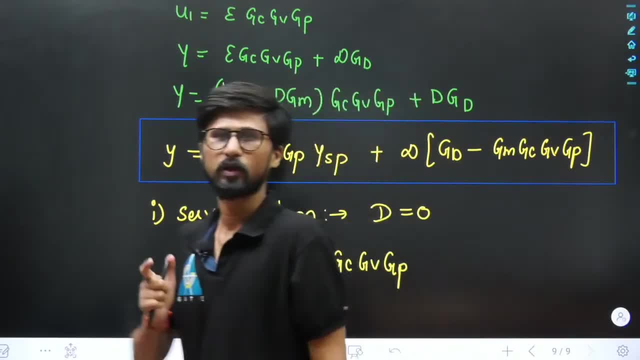 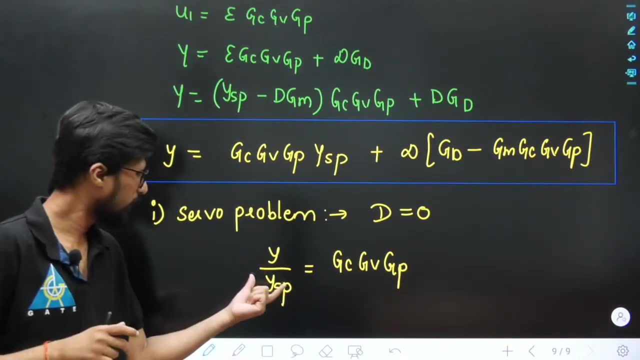 If I give any output in set point, then my output should go same. Any input I give in set point, no matter how much input I give in set point. any input I give in set point, no matter how much input I give in set point. no matter how much input I give in set point. 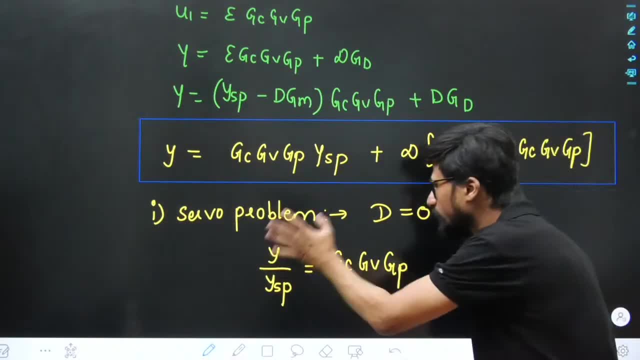 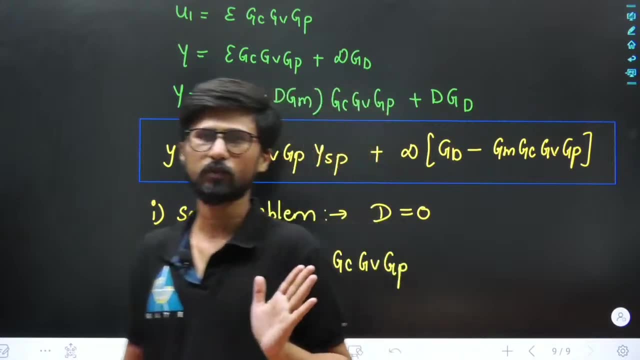 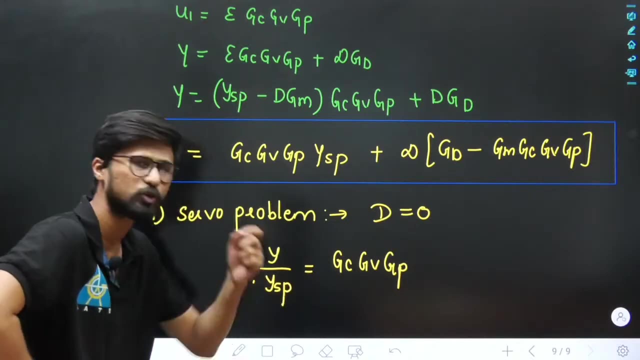 any change I give in set point, same change I should see in y. This is perfect feed forward control. ok, What is perfect feed forward control? What is perfection? We were looking at the change I am doing in ysp. if same change comes in y, then the thing is perfect, right. 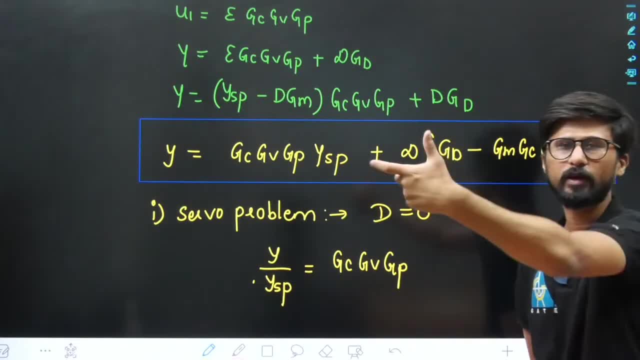 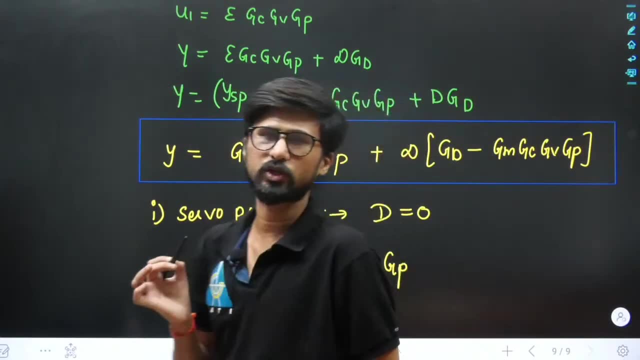 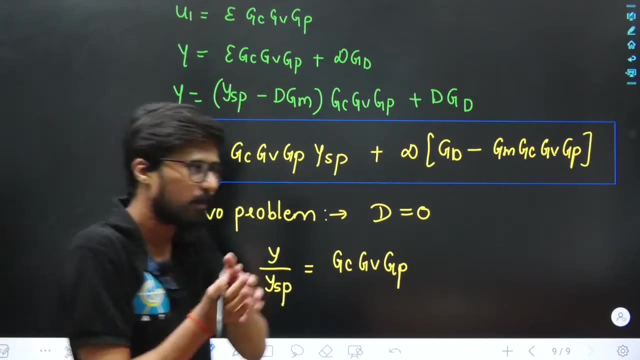 If offset is coming, then the thing is not perfect. ok, So the change I will give in set point, same change should come in y, then only the thing is perfect, Then only you will be able to test that there is one set point. If I give change of 1 meter in set point, then my 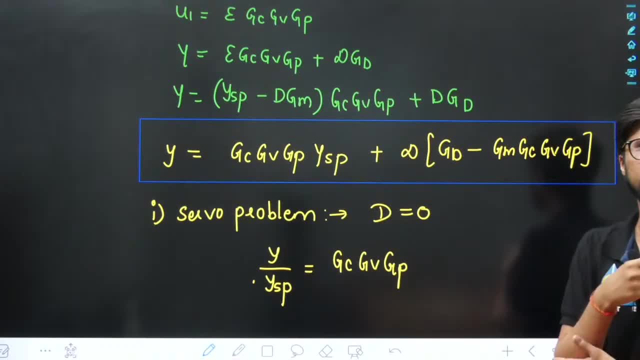 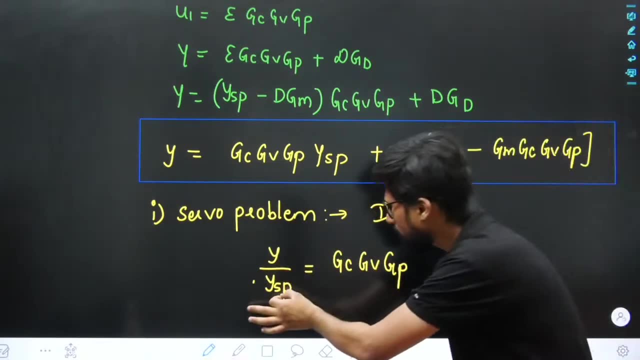 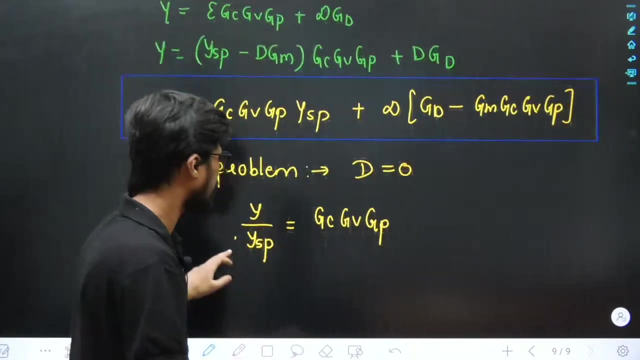 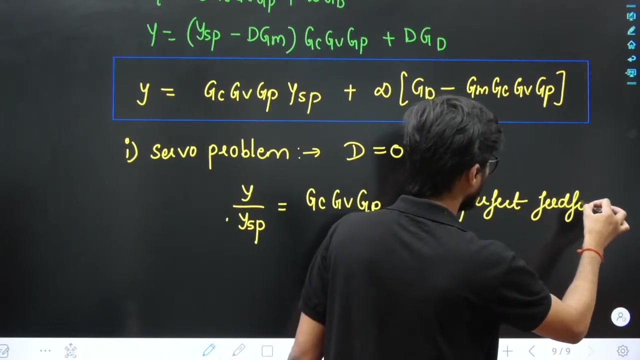 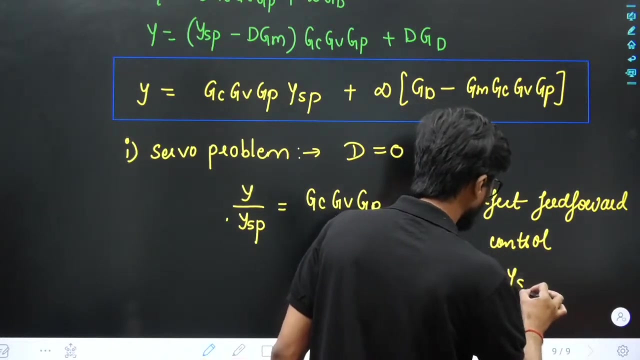 output should also go 1 meter. ok, But generally this does not happen. Value is a little less, But if change in set point comes in y, that is perfect condition. ok, I will call this as perfect feed forward control. given y is equals to ysp, The change I give in output. 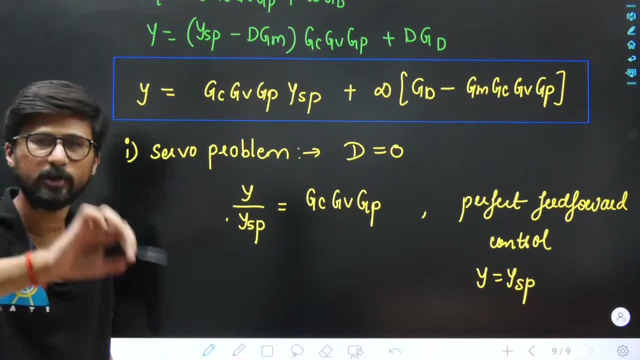 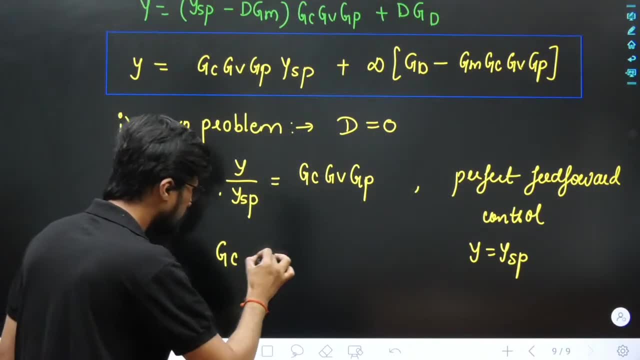 sorry, the change I give in input the same change I reflect in output. So if I substitute this as 1, then from here I will get gc. that will be 1 upon gc. So if I substitute this as a zero, it will be 1 upon gv. gp. 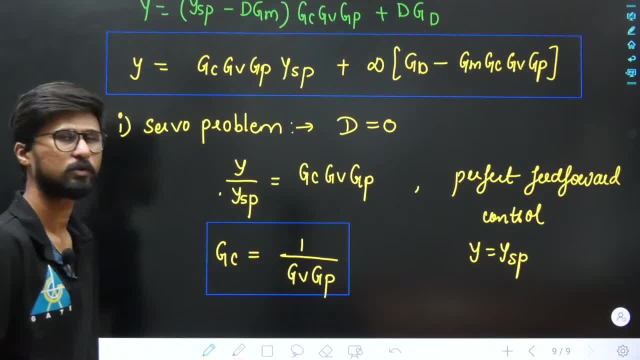 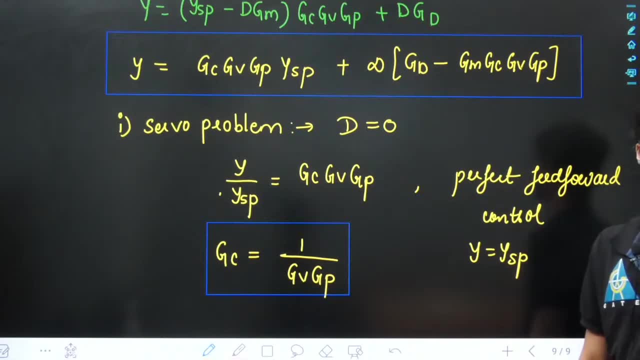 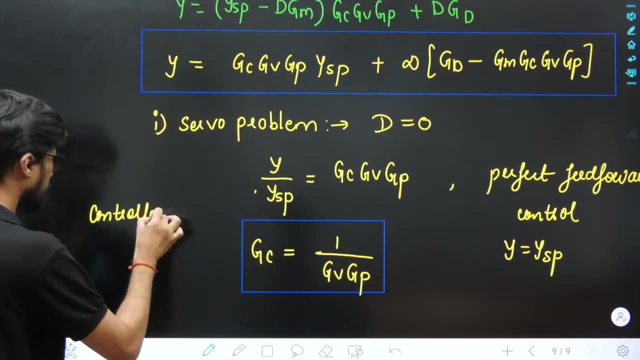 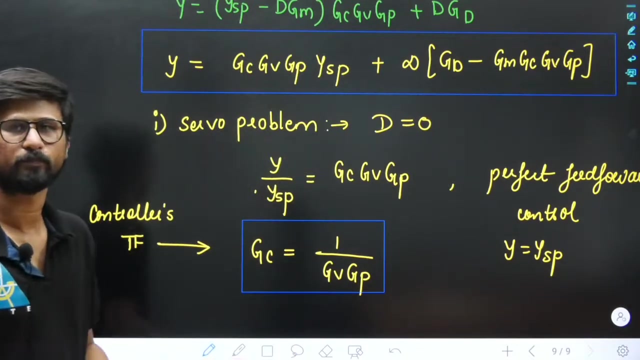 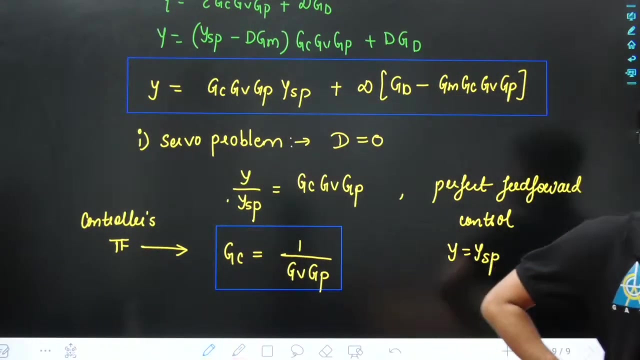 So this is the transfer function for the controller That is to solve the servo problem. this is the transfer function of the spot-forward controller. So this is controller's transfer function. Ok, 2nd thing we learnt was regulatory problem. Regulatory problem: set point may change 0,. 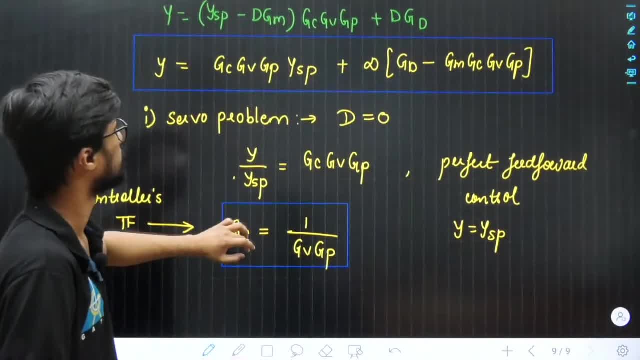 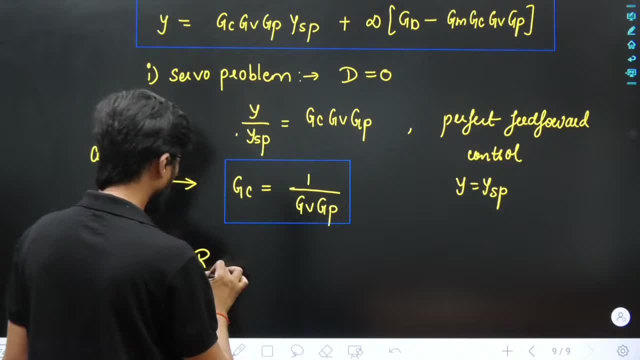 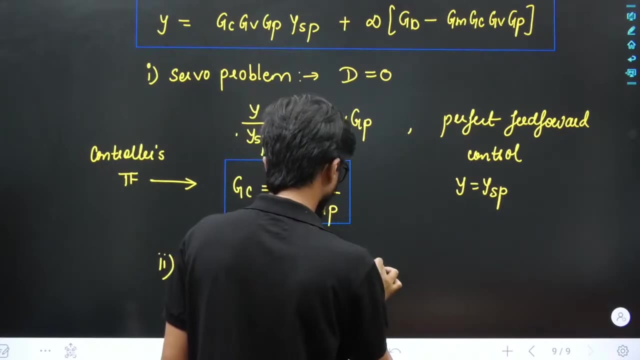 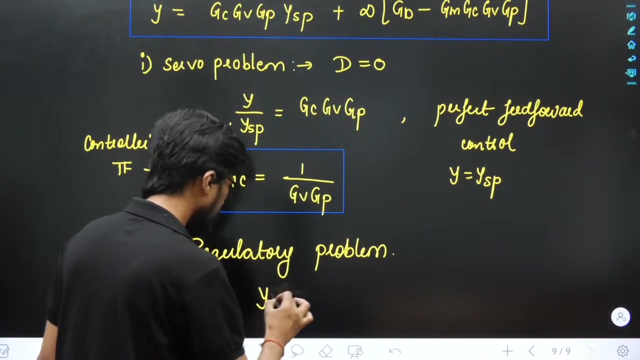 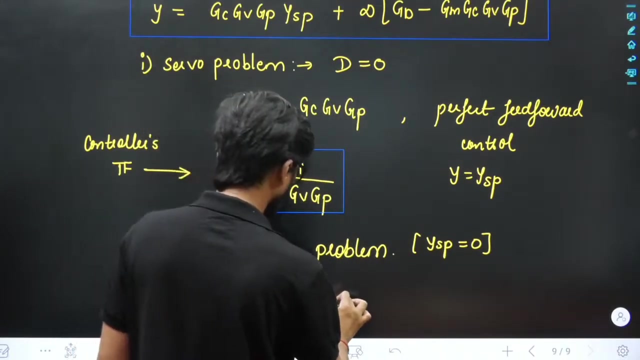 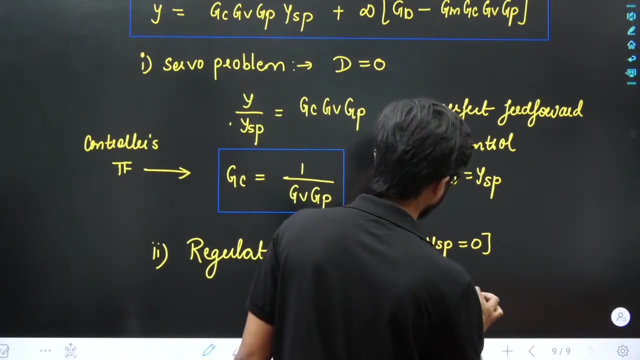 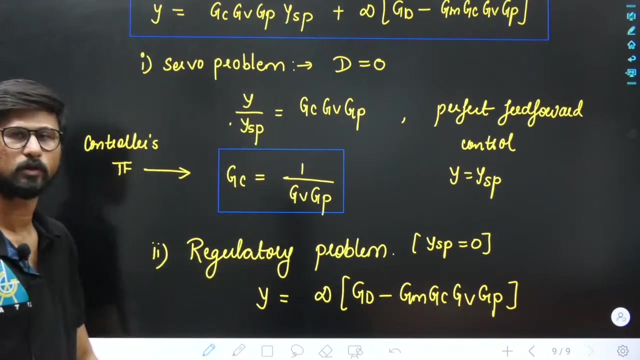 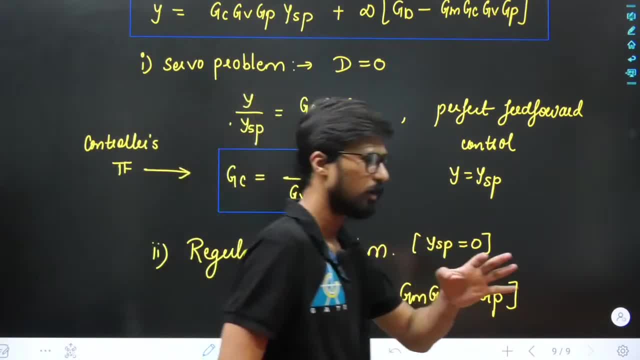 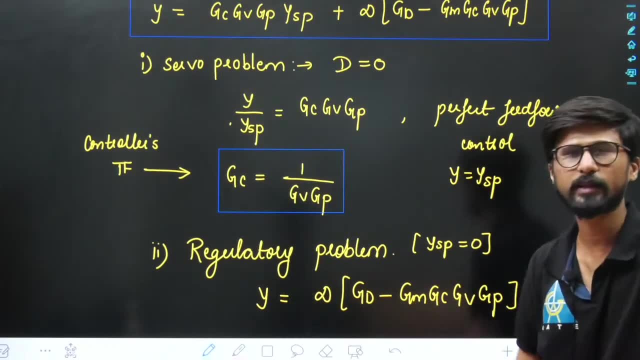 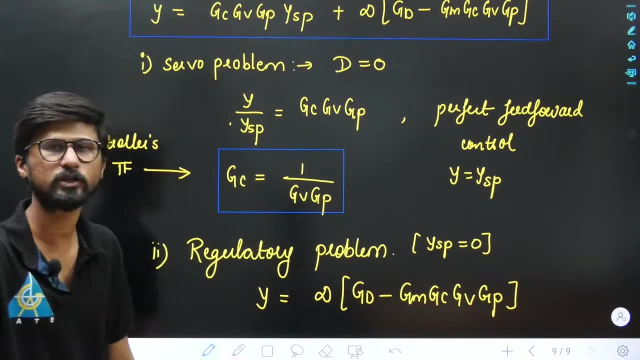 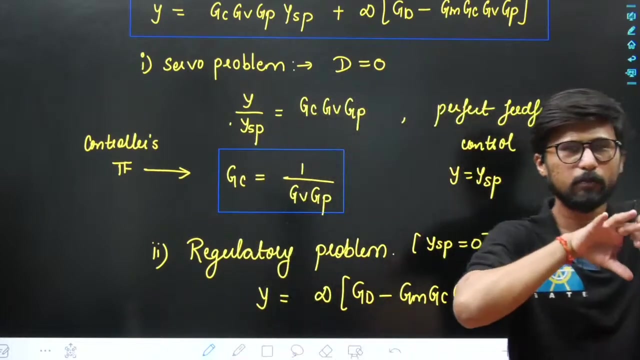 function of controller. So tell me one thing: if I give any change in disturbance, then do you want that change in y also? Tell me, if I give any change in disturbance, do you want that change in y also? No, we want our process to reject the disturbance completely. It should. 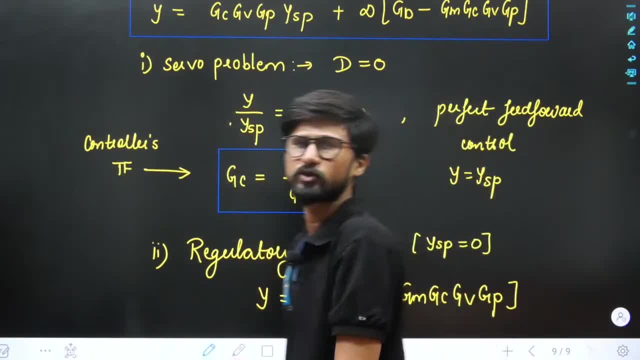 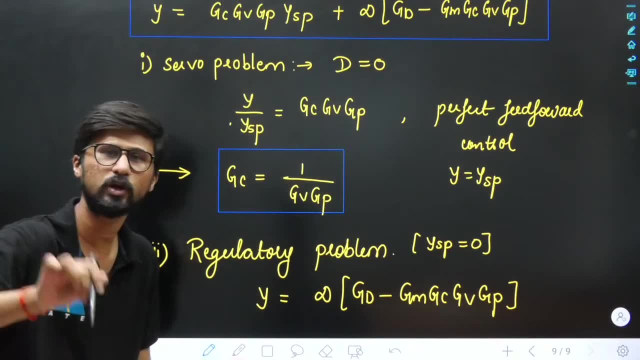 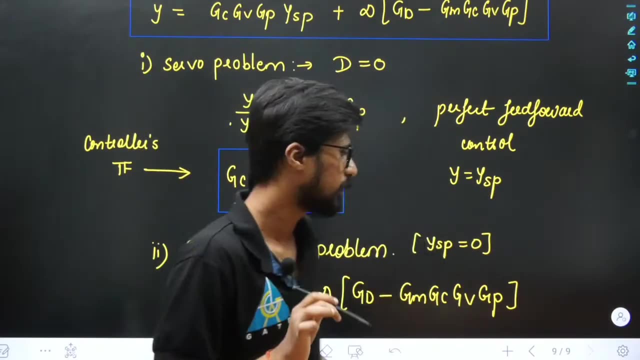 reject the disturbance completely, no matter how much I change in disturbance. What does reject mean? If I give any change in disturbance, it means the change in my output will be zero, And this condition is known as perfect disturbance rejection. What is the condition of perfect? 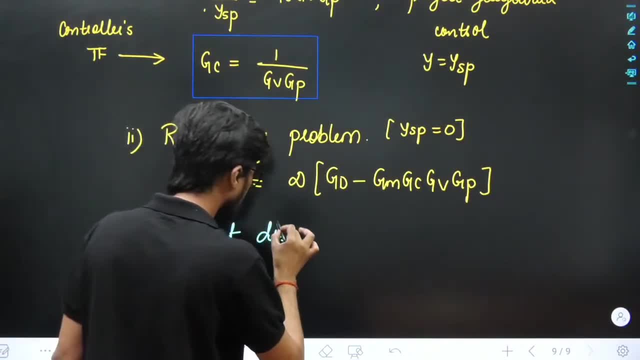 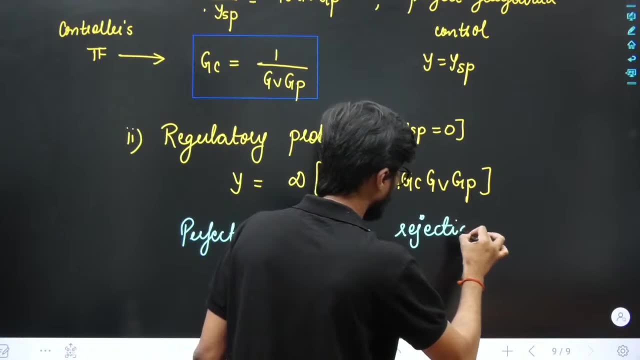 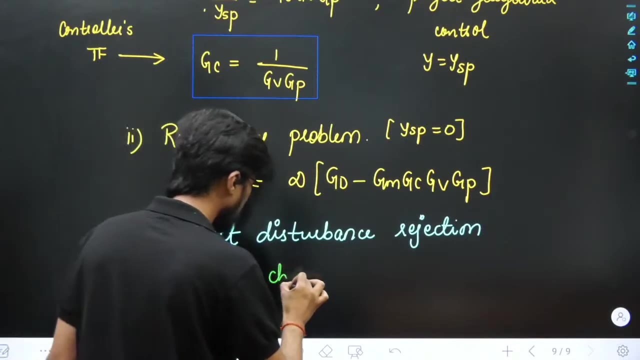 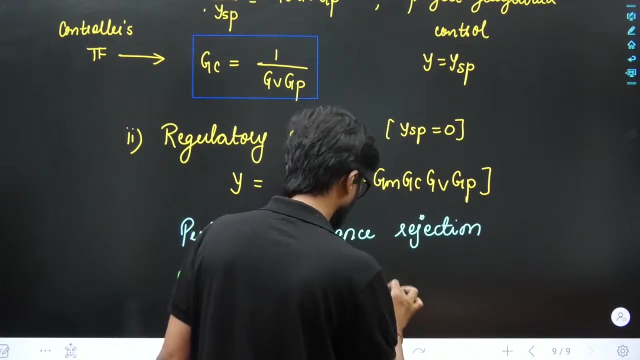 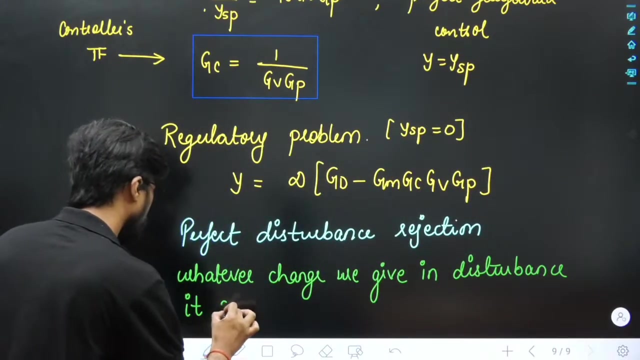 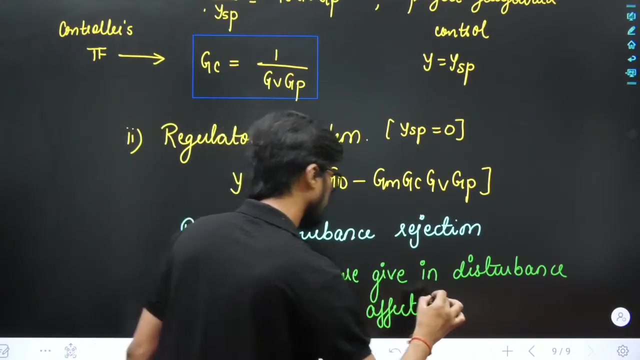 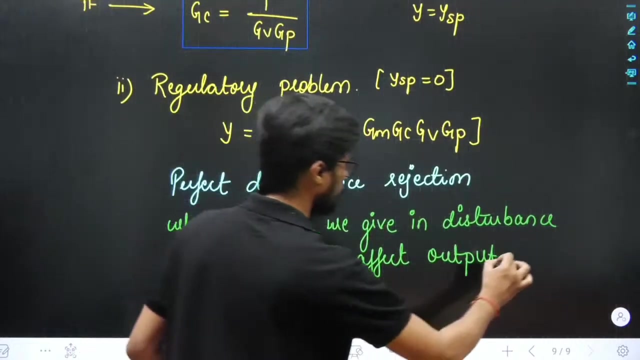 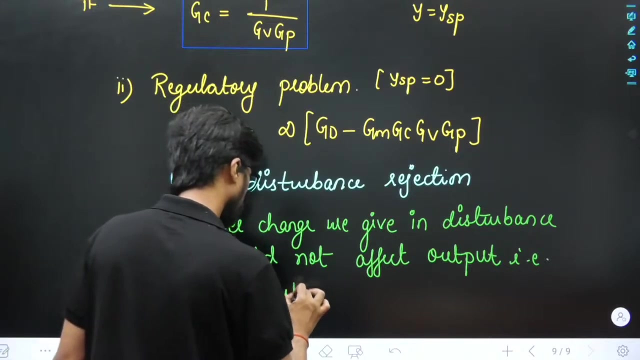 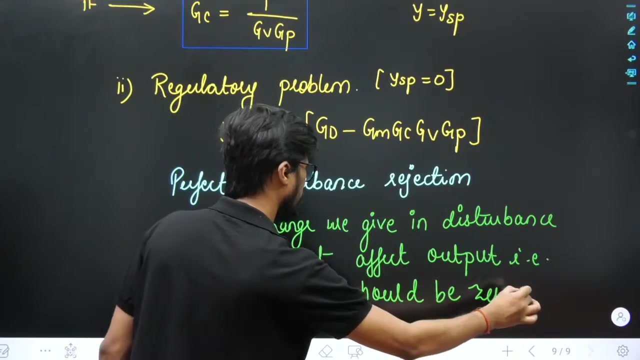 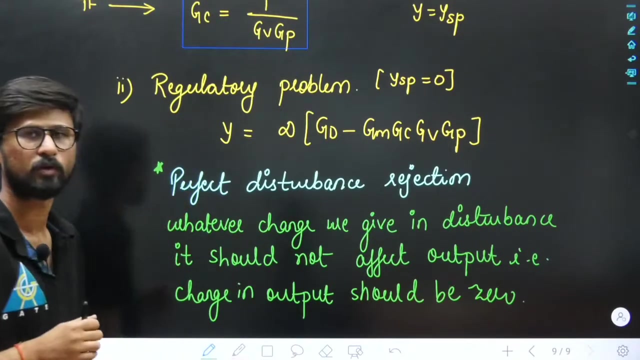 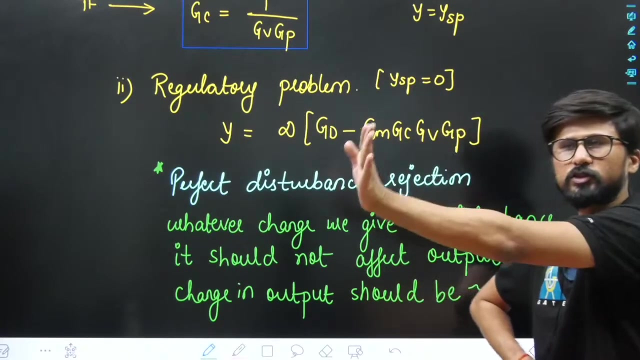 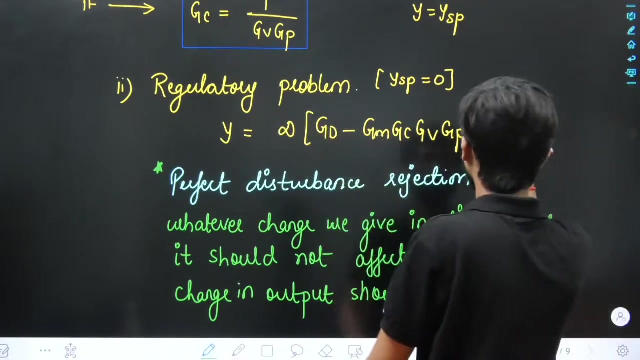 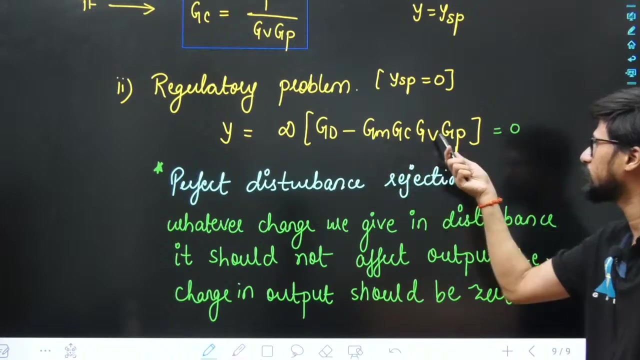 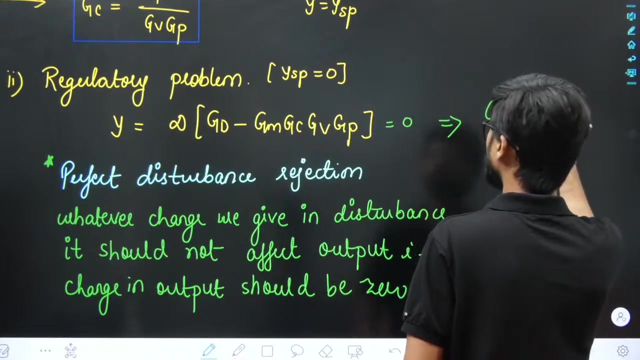 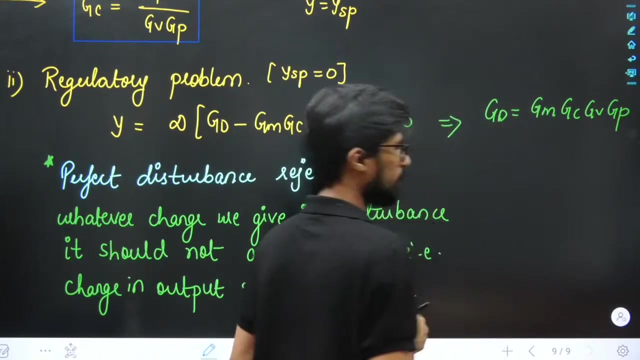 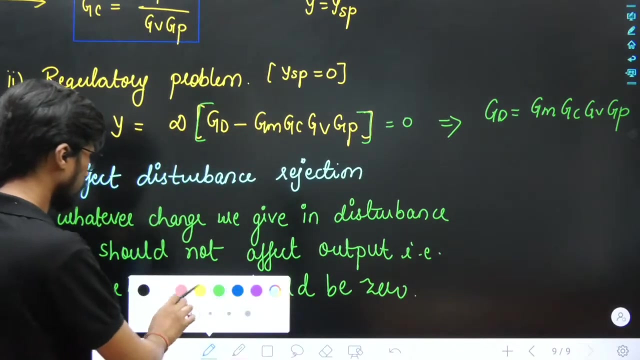 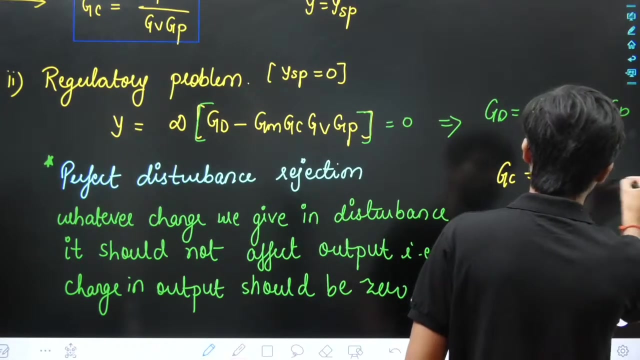 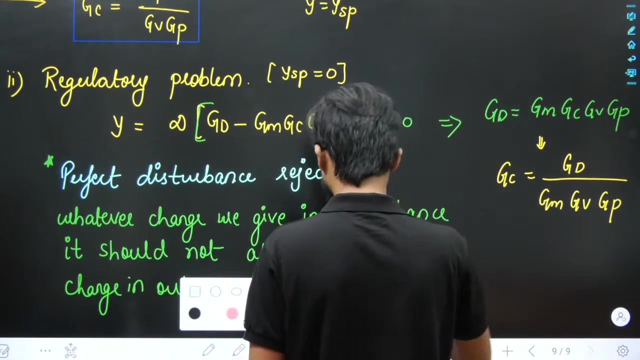 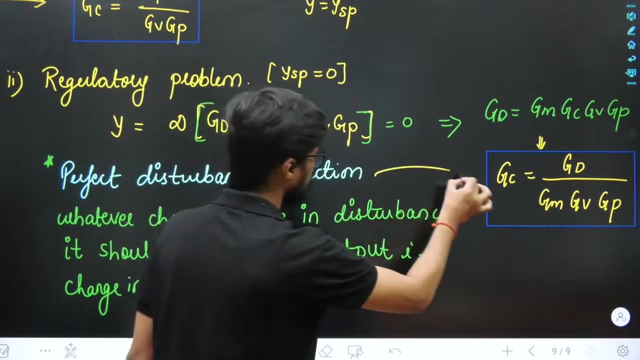 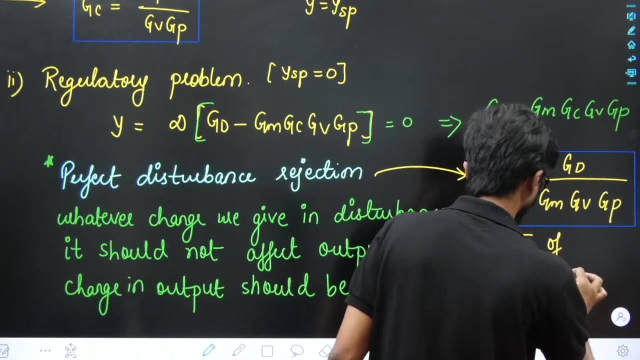 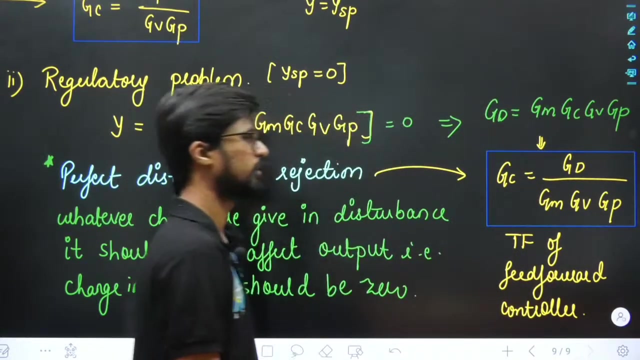 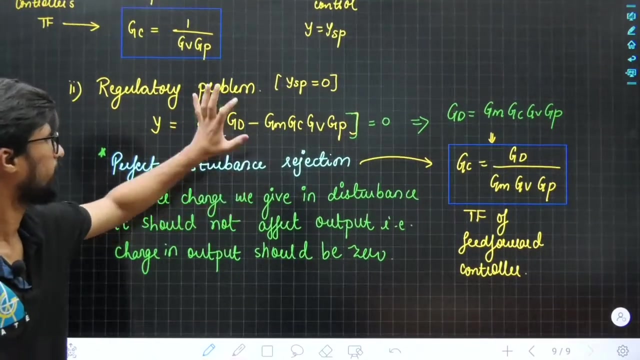 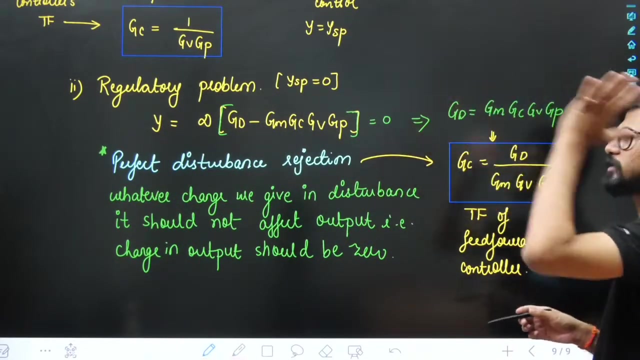 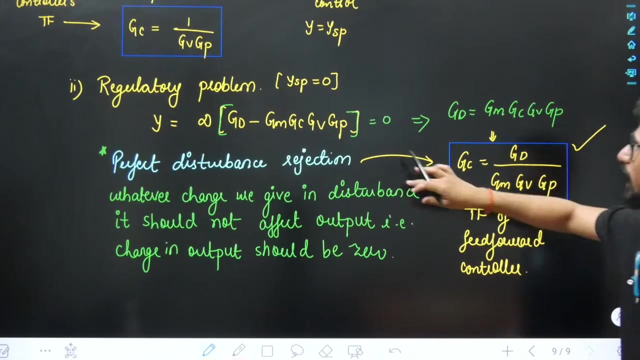 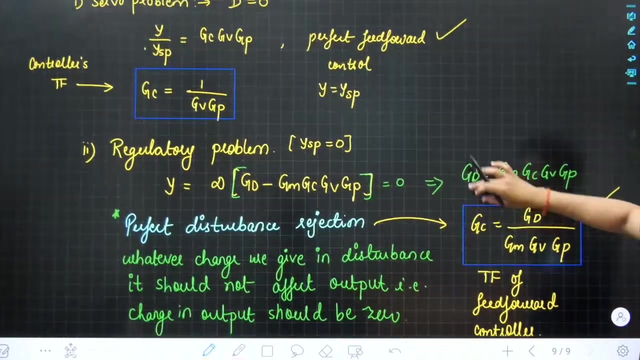 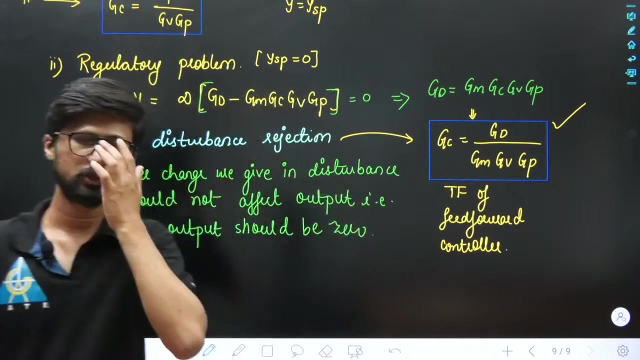 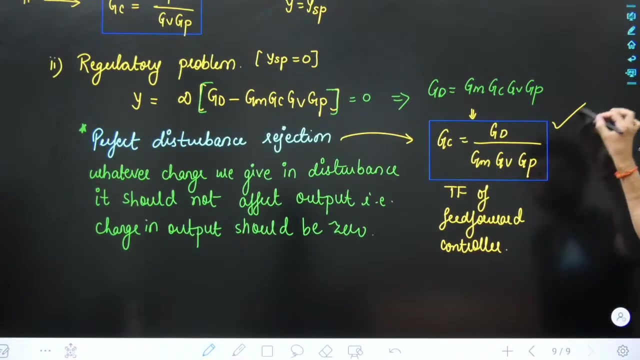 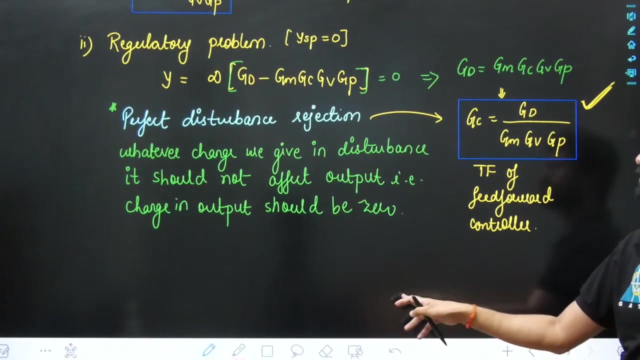 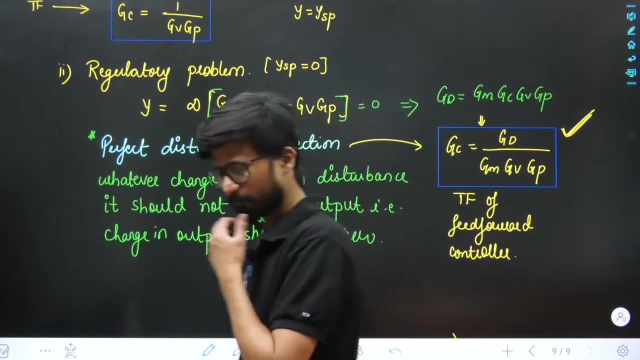 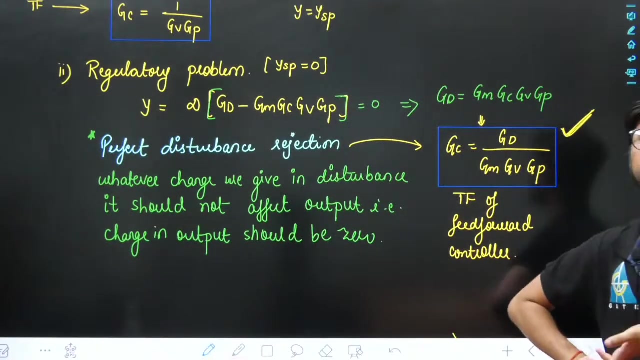 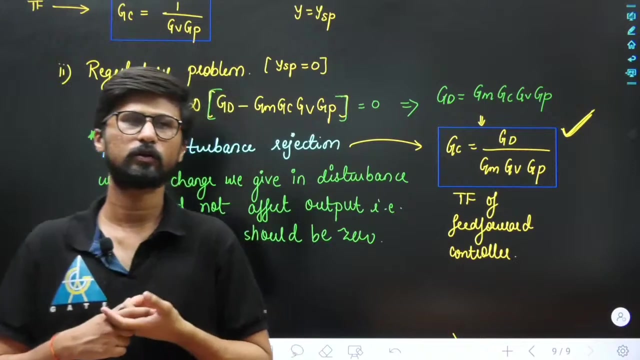 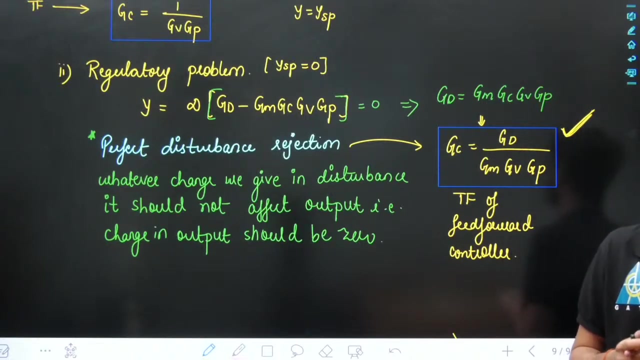 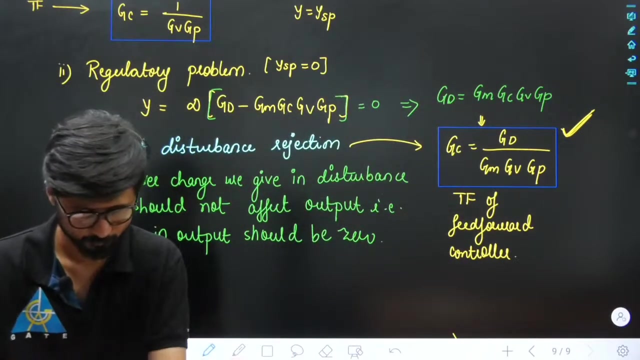 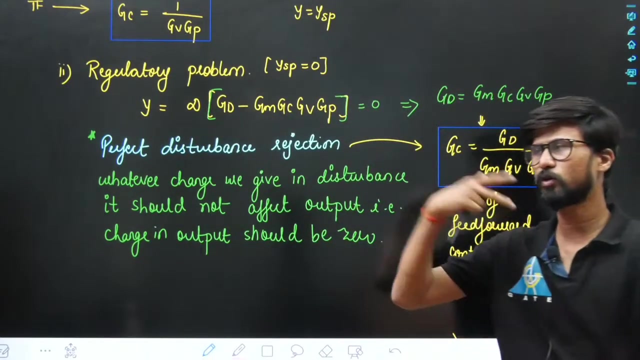 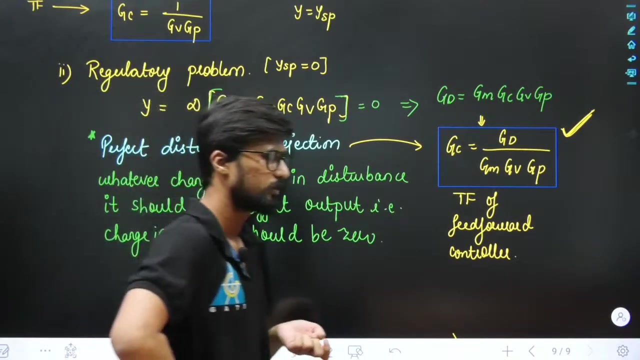 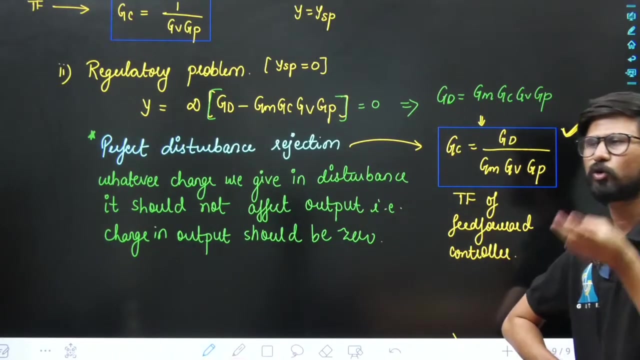 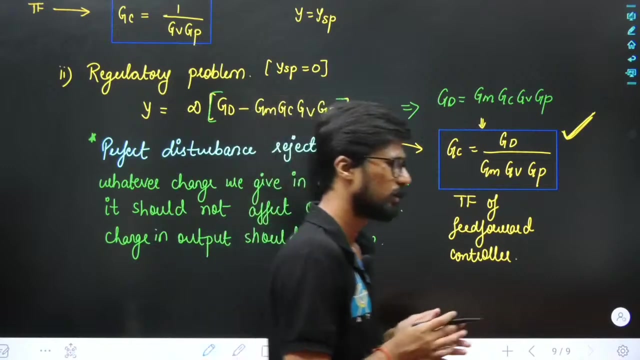 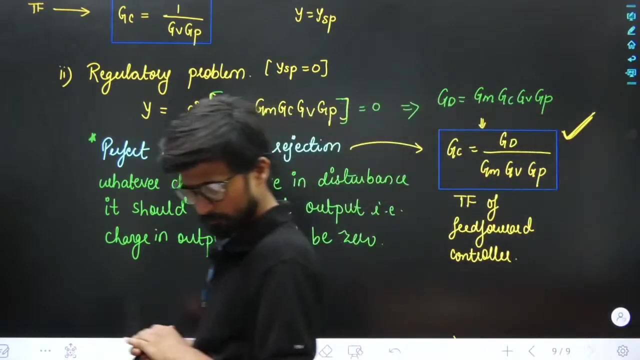